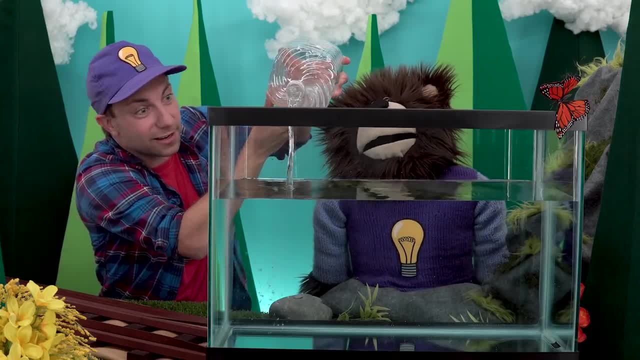 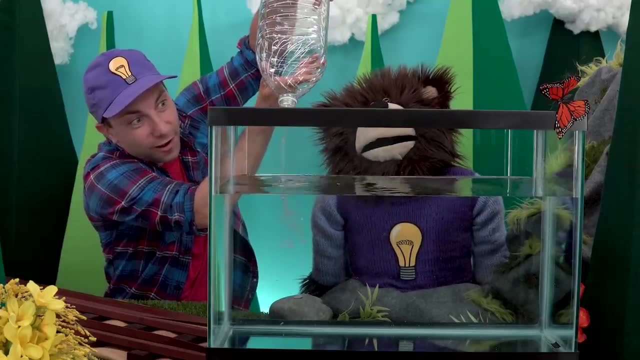 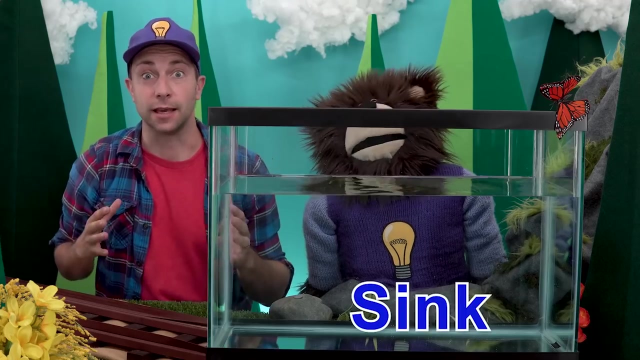 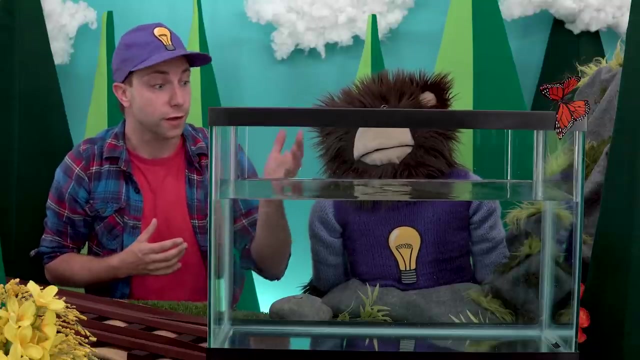 All right Made to. we are almost done filling up our tank with water, Just a little more. All right, Now we are ready to play the game Sink or Float. Wait, Do you know why some objects, when placed in water, sink to the bottom and other objects float on the top? 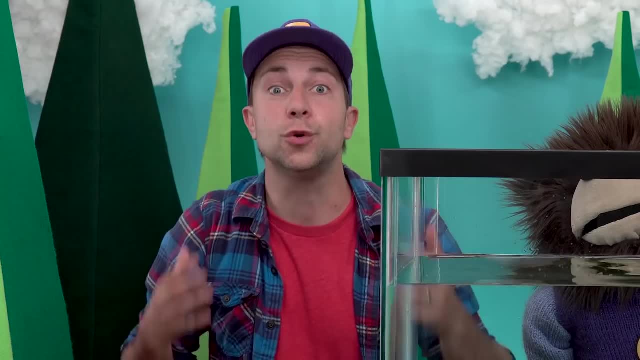 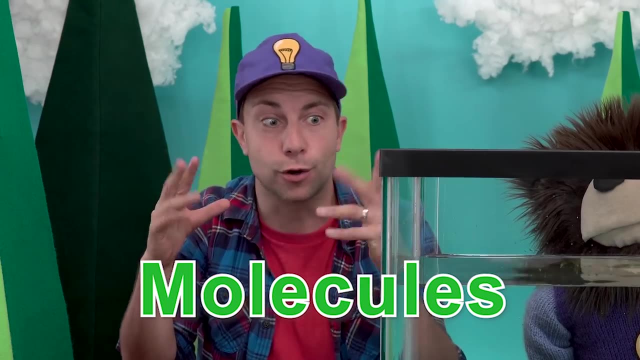 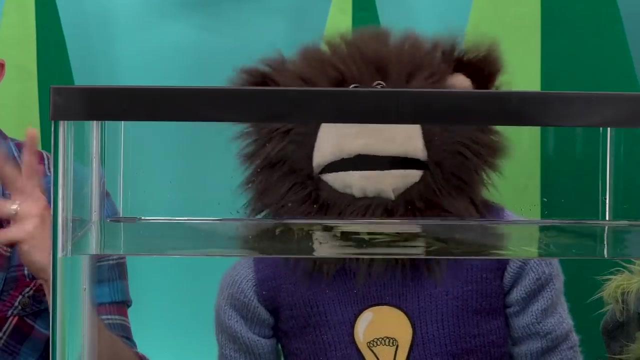 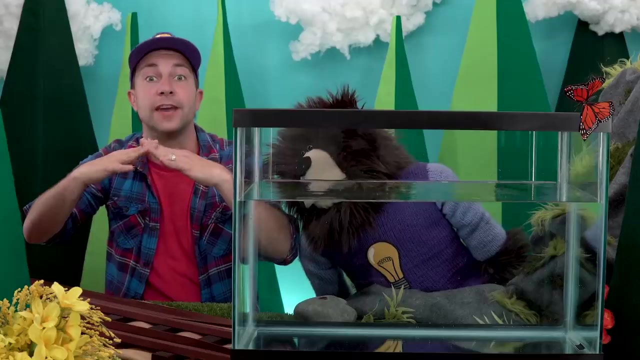 Well, I'll tell you, It has to do with density. You see, every object is made up of molecules, tiny little particles that are connected together. Let's pretend that my fingers are molecules. Now, if an object's molecules are farther apart, like this, the object is less dense and will most likely float on the top of the water. 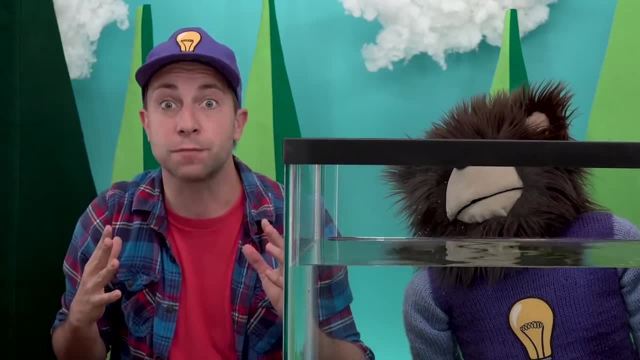 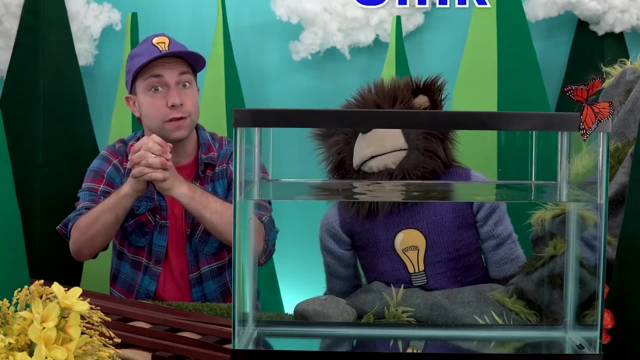 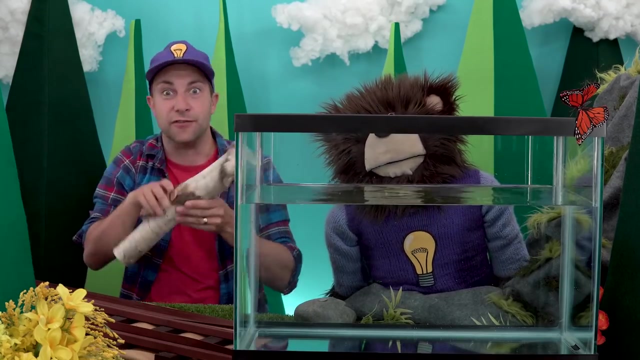 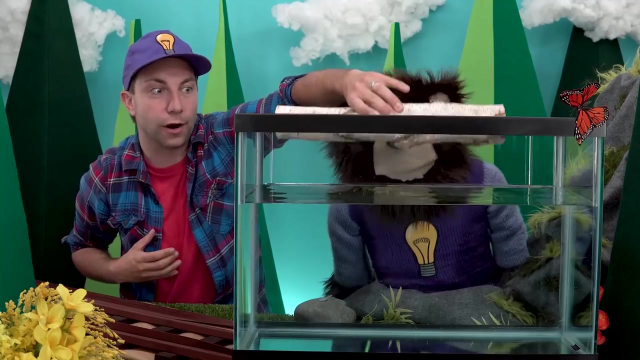 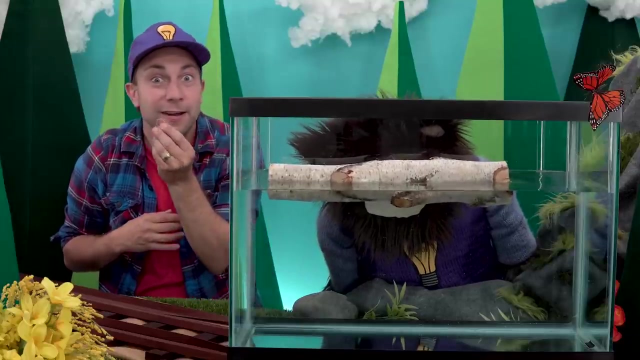 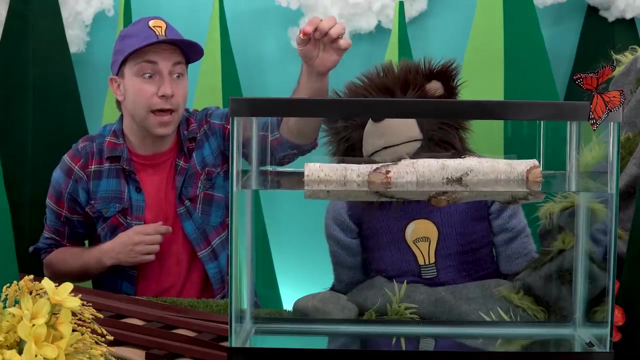 Now, if an object's molecules are tightly packed together like this, the object is more dense and most likely will sink to the bottom. That explains why a very heavy log like this will float on the top of the water Like that, While a little penny like this, when placed in water, will sink to the bottom. 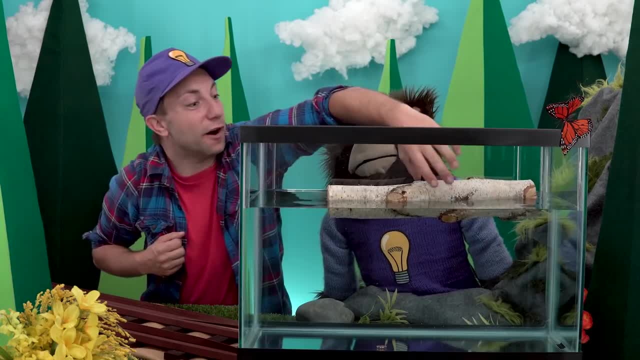 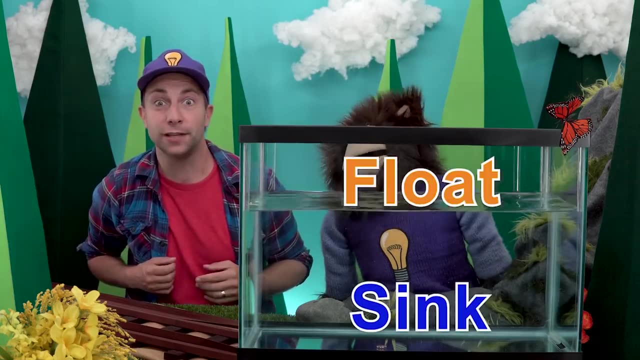 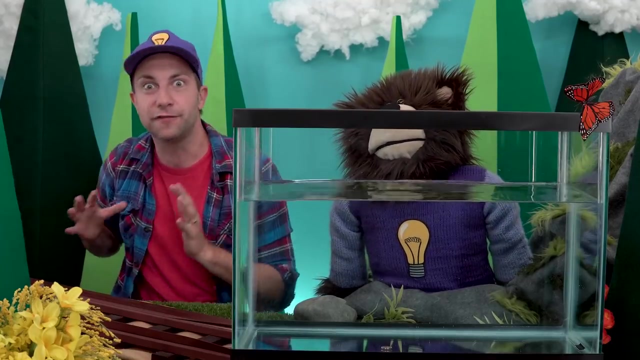 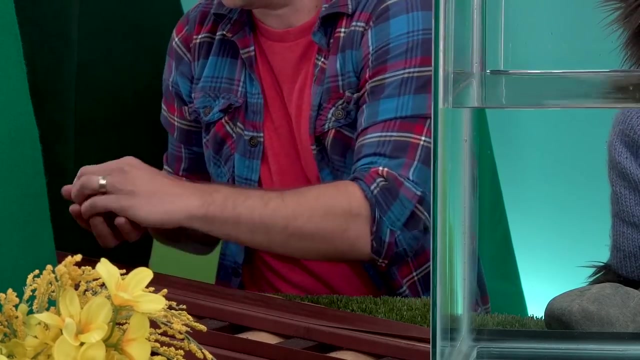 Wow, Okay, let's remove our log. Are you ready to play Sink or Float? You are. Are you ready? Yes, Okay, We've gathered a bunch of different things to see if they sink or they float First we have. 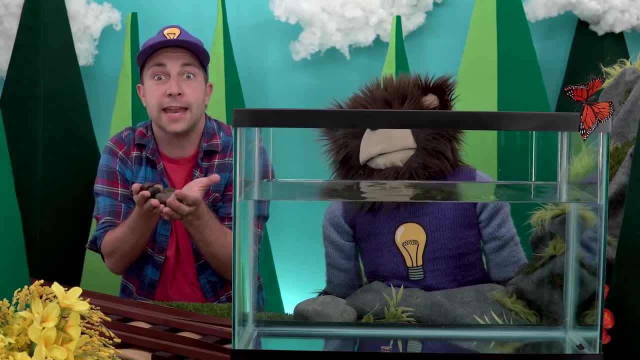 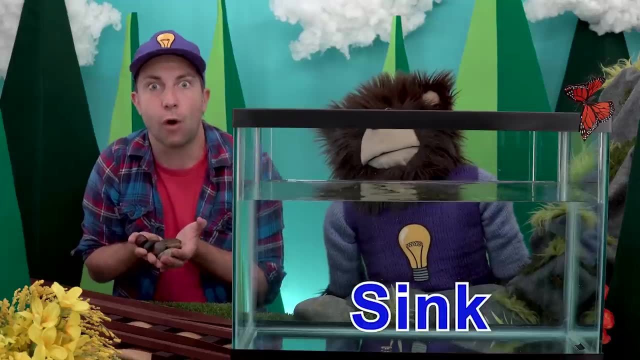 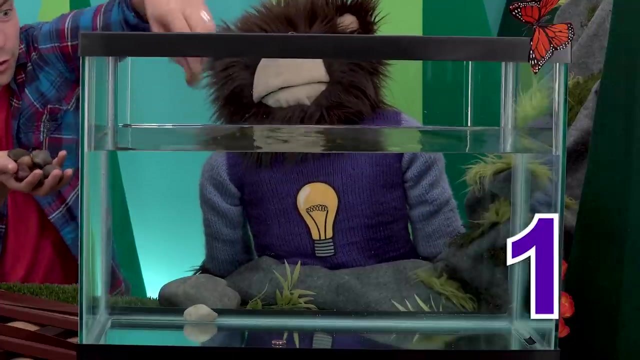 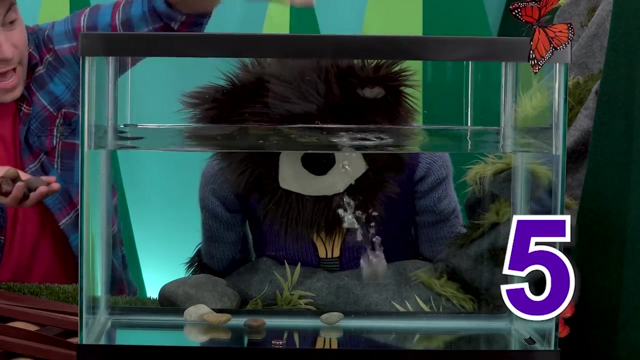 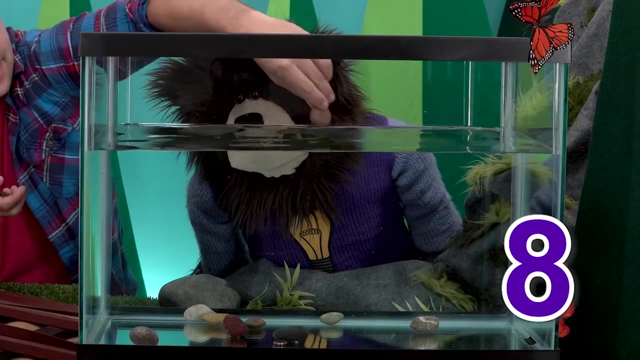 Whoa got to get them all Ten rocks. You see these rocks. Do you think they will sink to the bottom or float on top? Let's see All right. One, two, three, four, five, six, seven, eight, nine, ten. 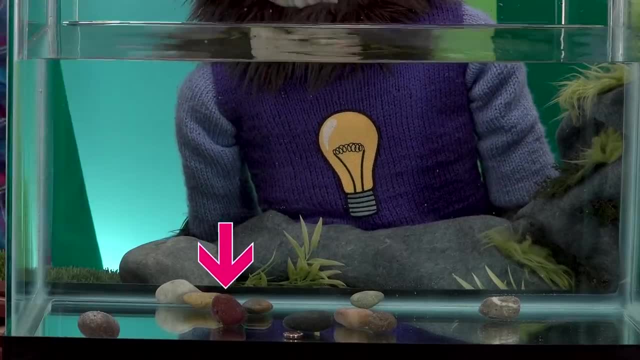 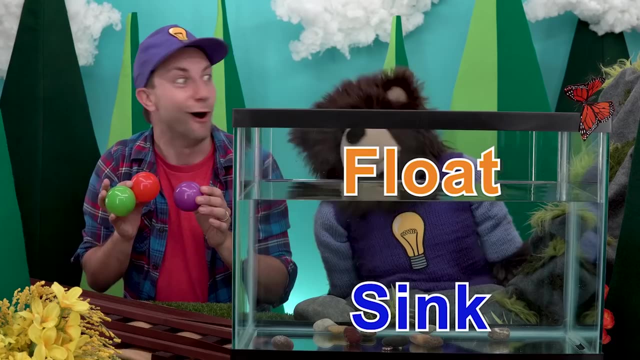 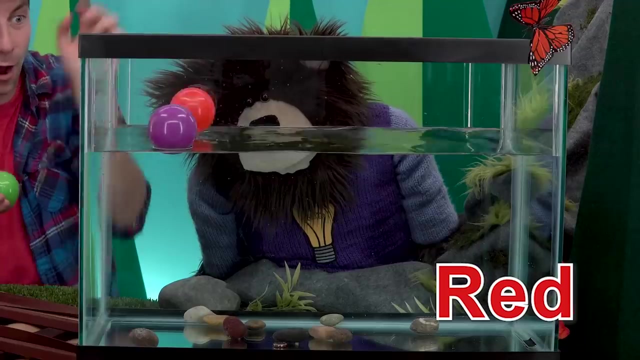 They all sank to the bottom. Wow, All right. Now we have three plastic balls filled with air. Do you think they will sink or float? Let's see, Mayta First, our purple ball and our red ball and our green ball. 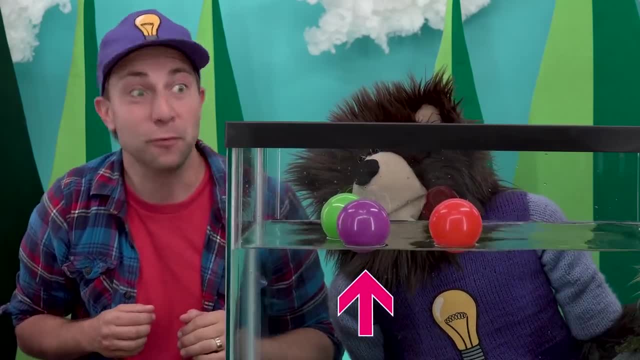 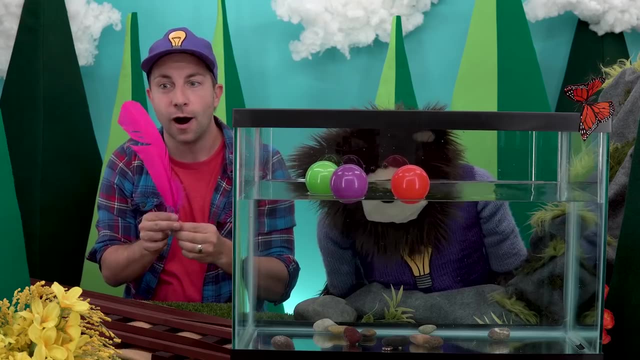 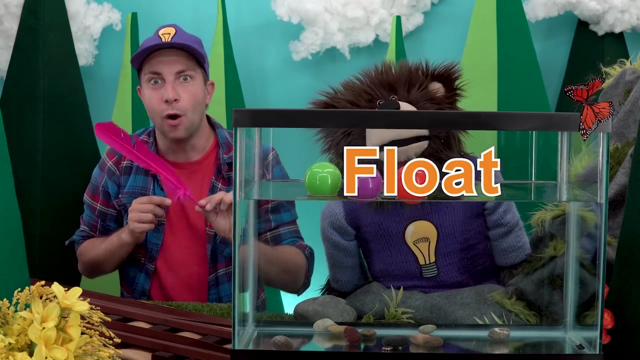 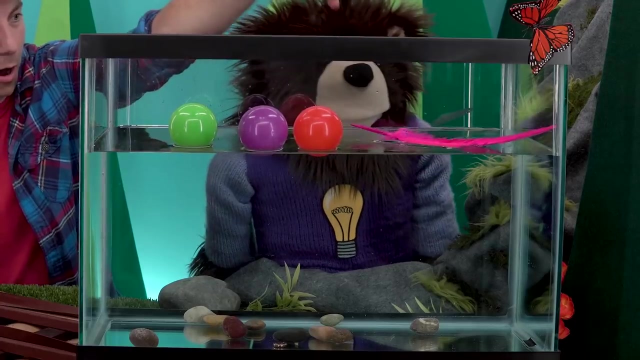 Mayta, they all float on the top of the water. Okay, Our next object is a pink feather. Do you think this feather will float on the top or sink to the bottom? Let's see. Oh, wow, Mayta. 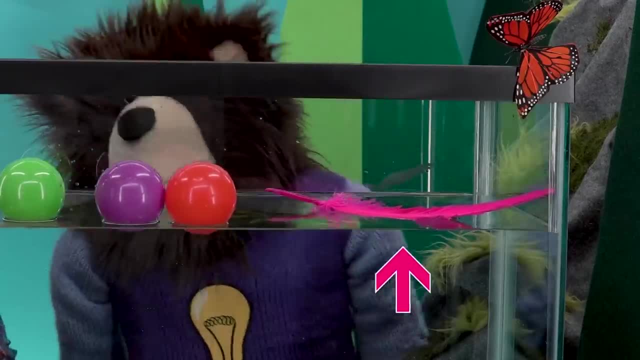 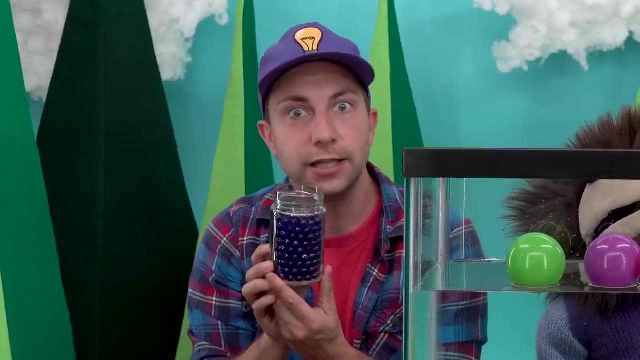 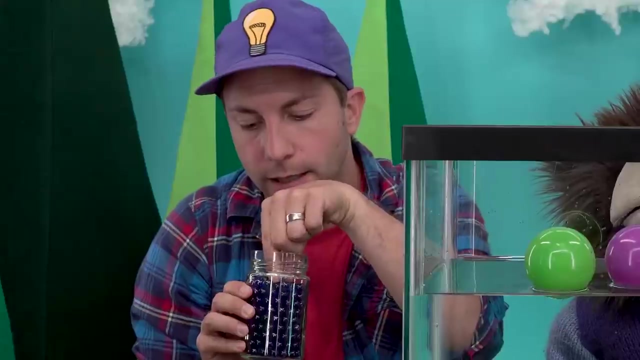 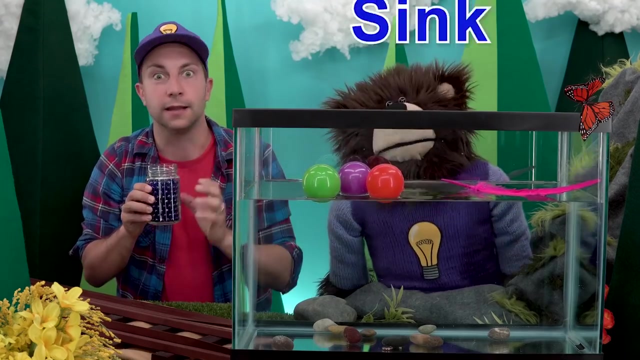 The feather is floating on the top of the water. All right, What do we have next? Whoa, We have a jar of little blue marbles. Now, Mayta, these marbles are very tiny, but they are very dense. 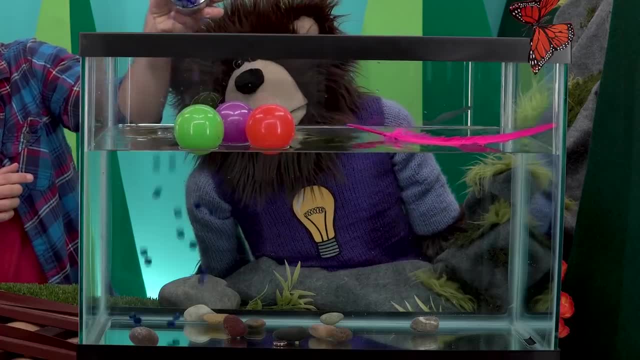 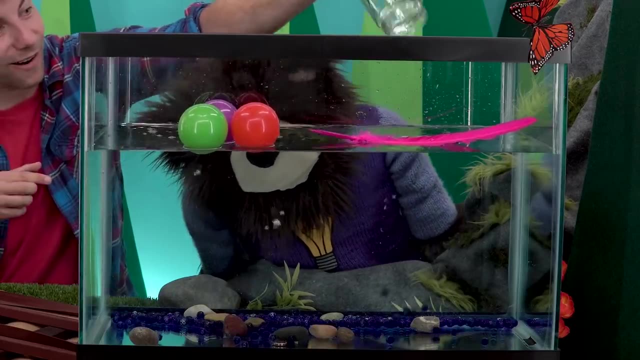 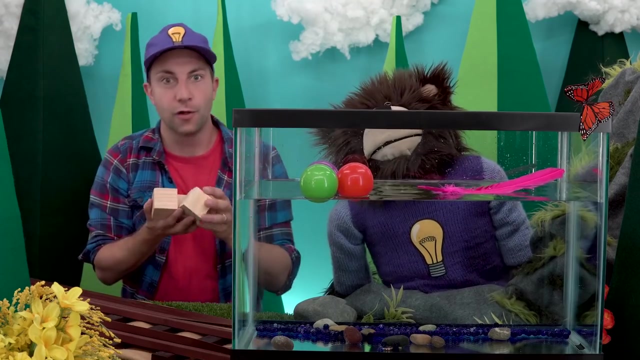 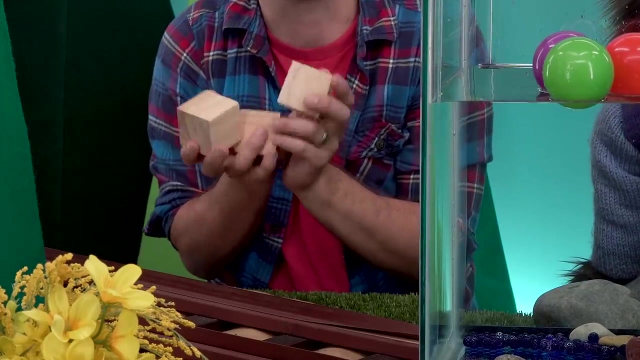 Let's see if they sink or float. Whoa, Mayta, all the marbles sank to the bottom. Okay, What do we have next? Three wooden blocks. Oh, Mayta, do you think that these three wooden blocks will sink or float? 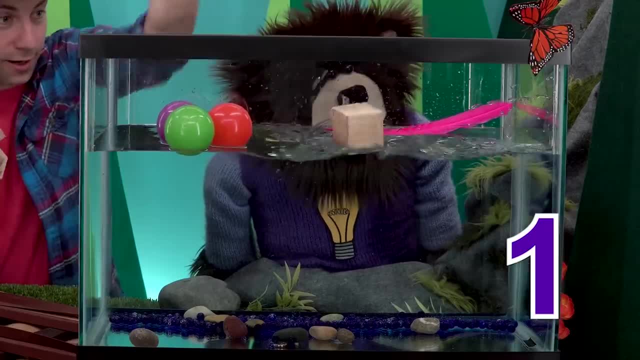 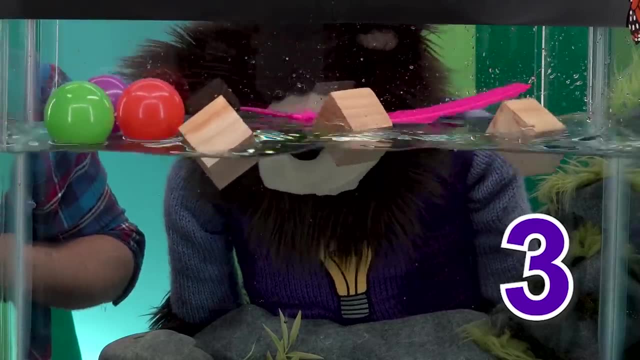 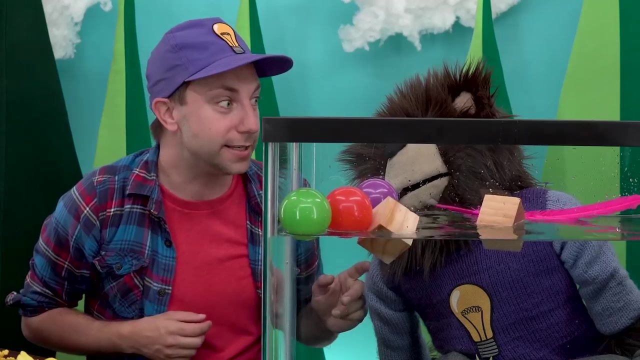 Okay, Let's see One, Two, Whoa, Three, Wow, All three wooden blocks are floating on the top of the water. Okay, What do we have next? Mayta, you are going to love what I have next. 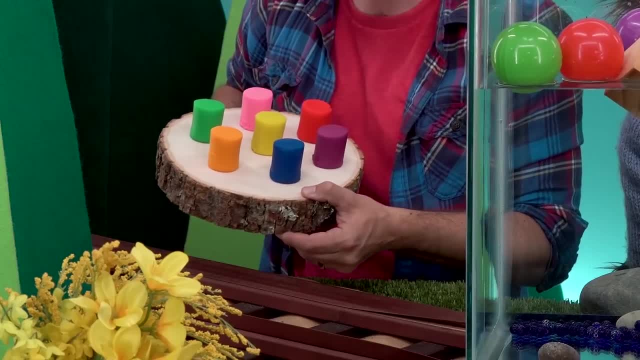 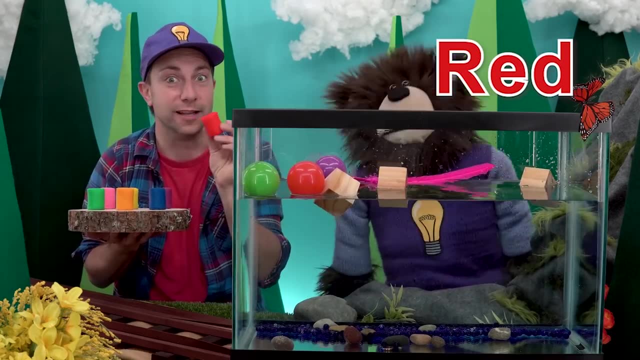 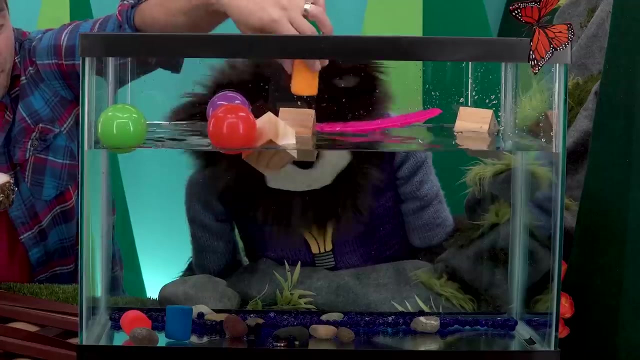 It's a bunch of colorful play-doh. Look at that. All right, Let's start with the red play-doh. Will it sink or float, Oh? Blue play-doh, Orange play-doh, Yellow play-doh, Green play-doh. 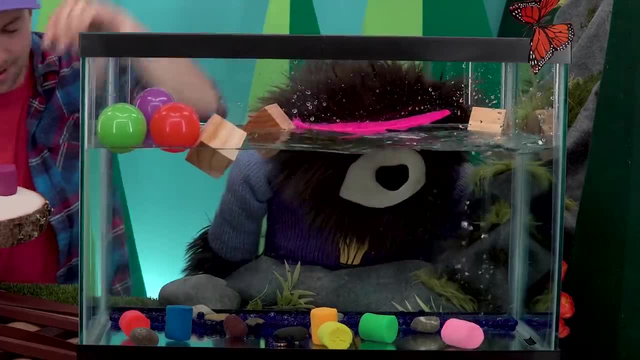 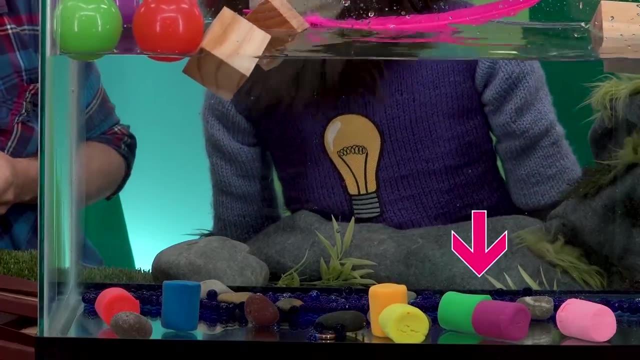 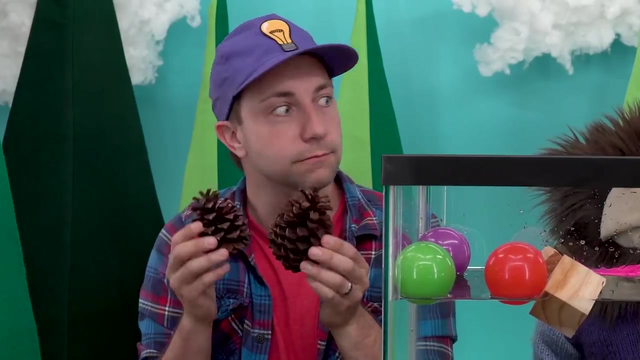 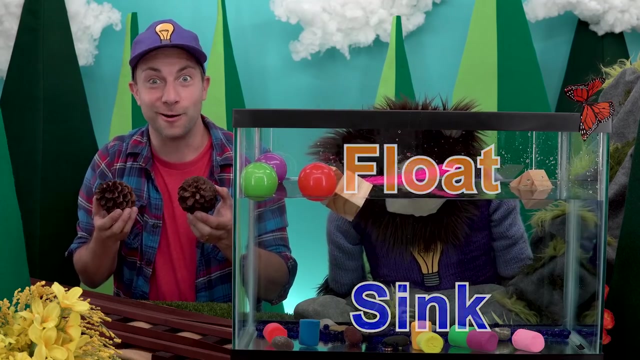 Pink play-doh And the purple Play-Doh. Mayta, all the Play-Doh sank to the bottom. Okay, next we have two pine cones. Hmm, do you think these pine cones will sink or float? Okay, let's see. 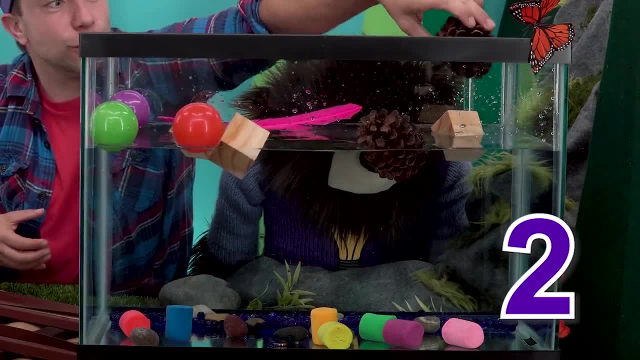 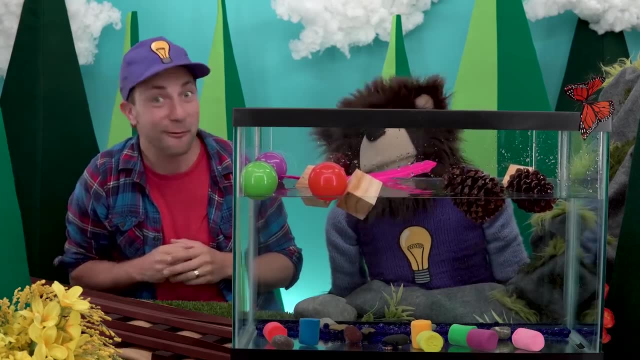 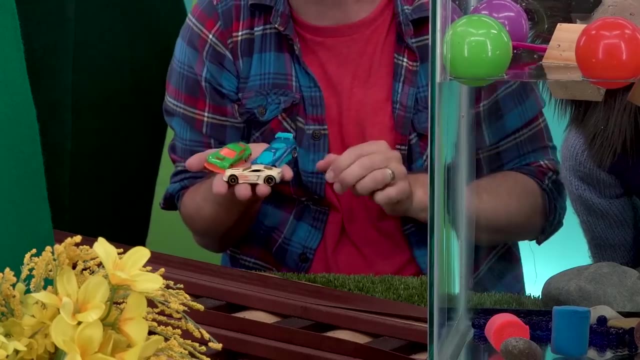 One, Two, Oh, the two pine cones are floating on the top of the water. Hmm, Wow, Okay. what do we have next? Oh, Mayta, look, we have three metal cars. Do you think these three metal cars will sink or float? 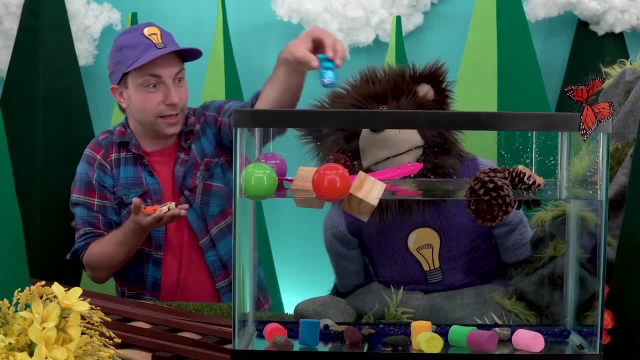 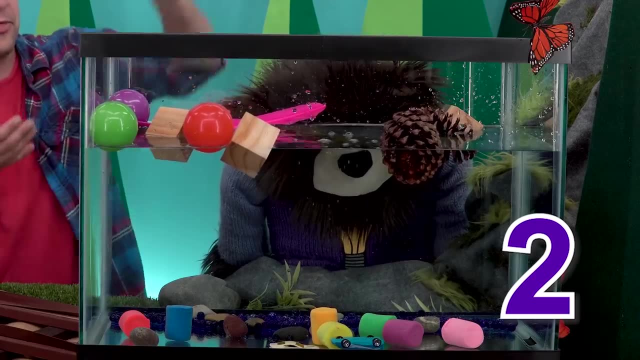 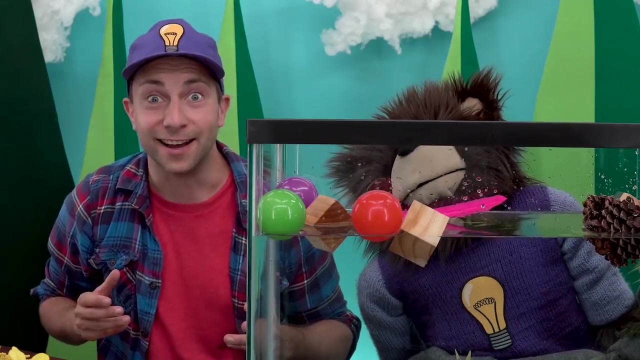 Oh, let's see One Whoa, Two Whoa And three. Oh, they're floating on the top of the water. Hmm, All three cars sank to the bottom. Mayta, look what I have next: a bottle of glue. 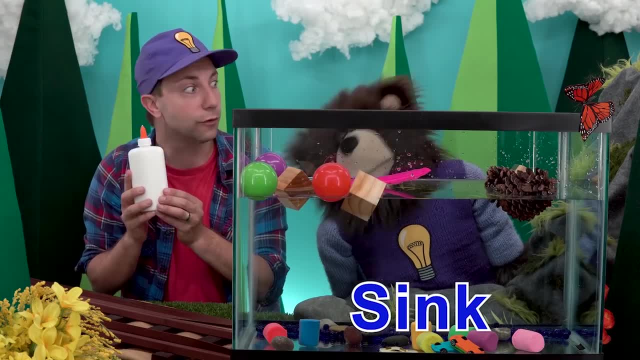 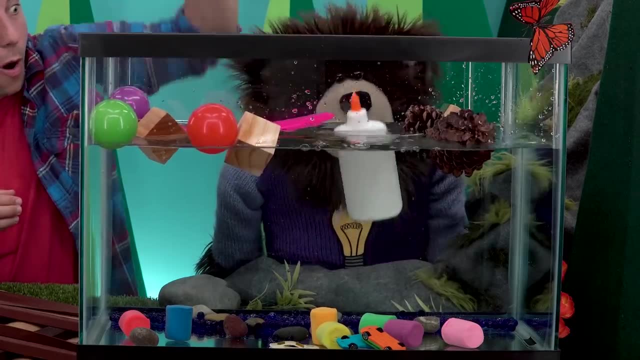 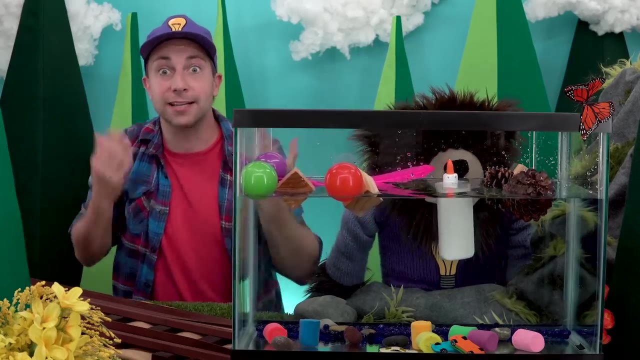 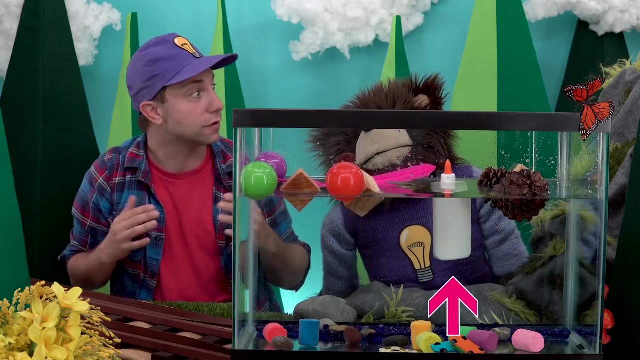 Do you think this bottle of glue will sink or float? Let's see. Oh, it's floating, Mayta. It first went all the way down but then floated back to the top. Mm-hm, that bottle has glue and air inside, which makes it less dense than the water, so it floats. 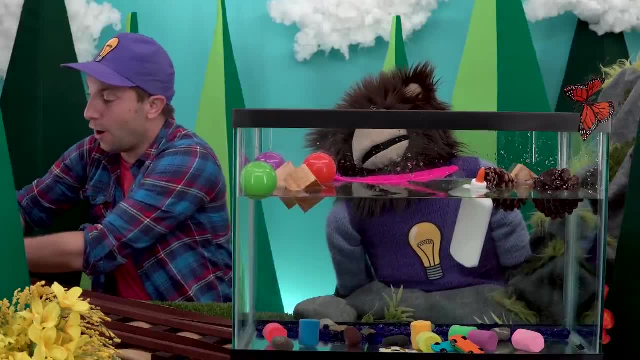 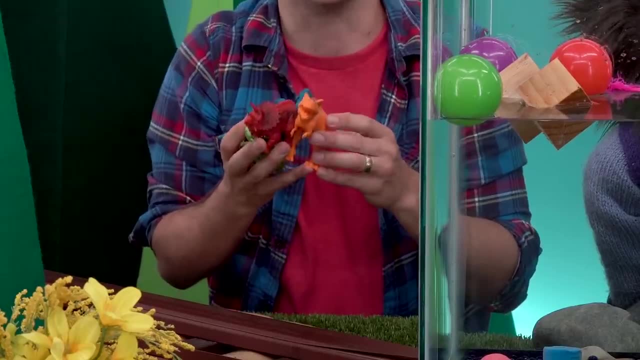 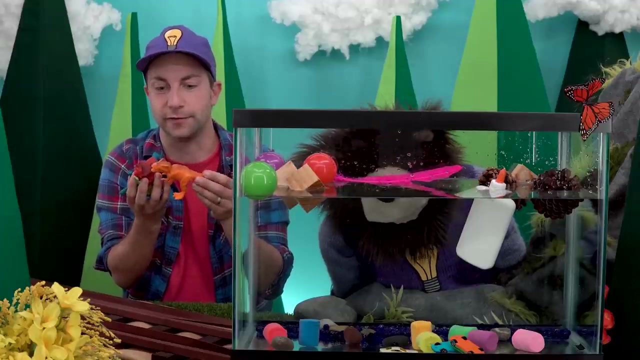 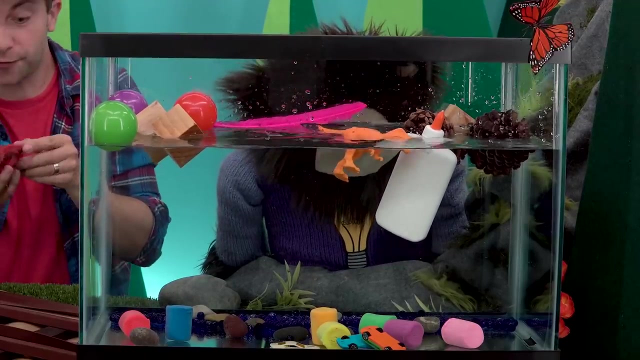 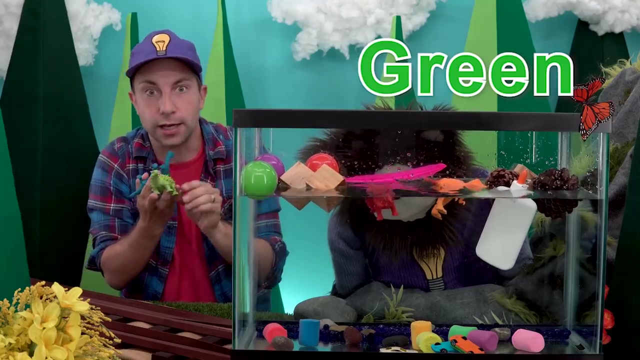 okay, mayta. next we have four toy dinosaurs. now these dinosaurs are made of plastic. do you think they will sink or float? all right, first we have a orange t-rex- oh, the t-rex floats. and a red triceratops- he floats too. and a green ankylosaurus. 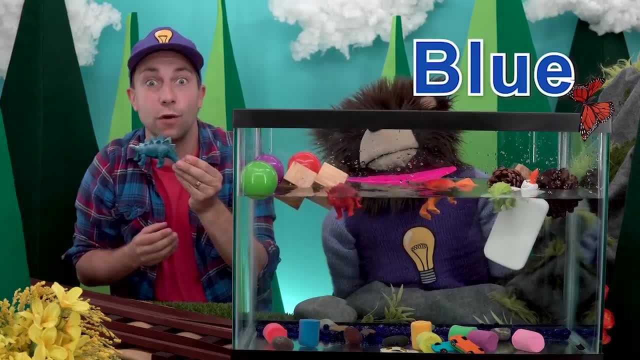 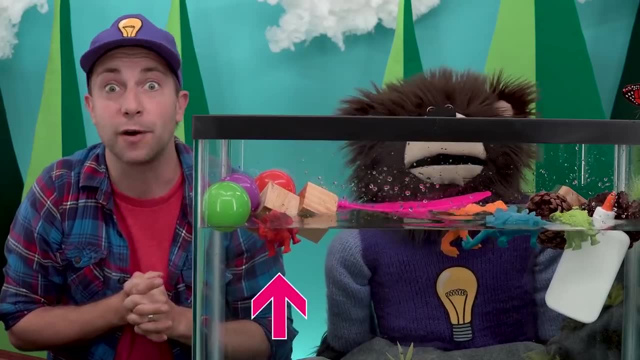 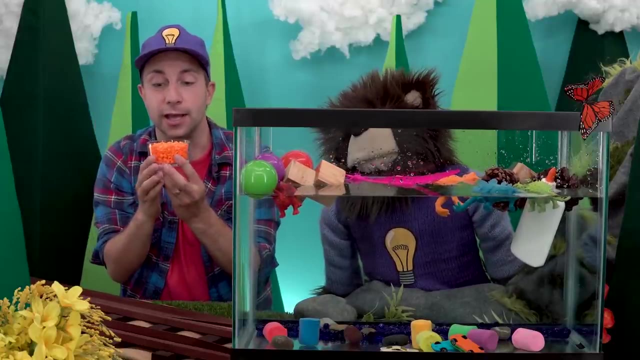 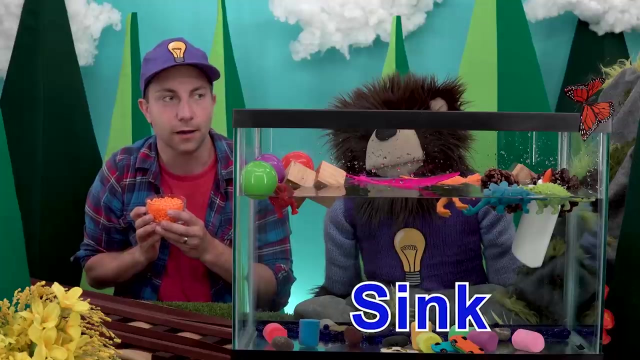 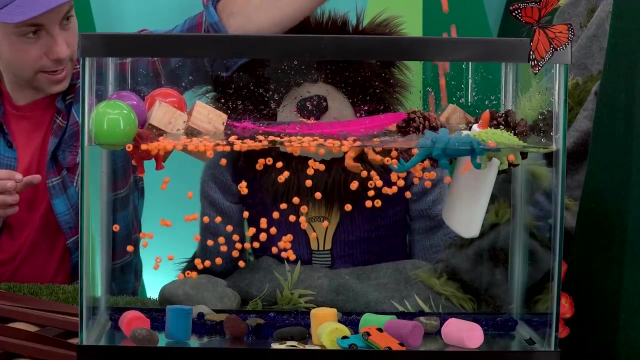 she floats. and a blue stegosaurus: she floats too. all four dinosaurs are floating on the top of the world. water, mayta, look what i have. it's a jar full of orange beads. do you think these beads will sink or float? let's see. oh, look at that, mayta. some are floating and some are sinking. 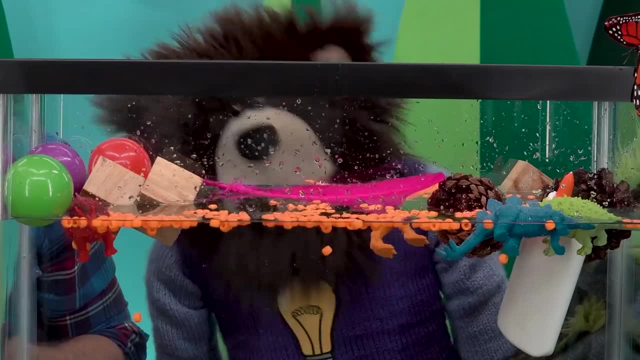 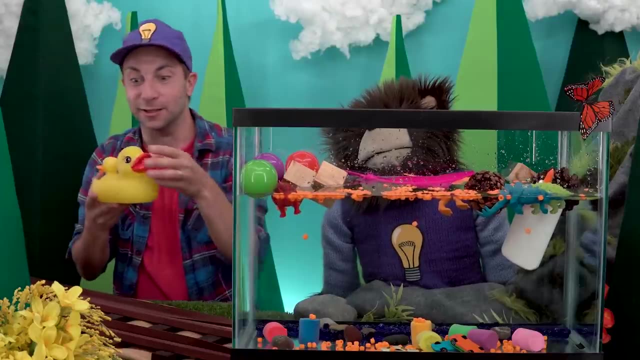 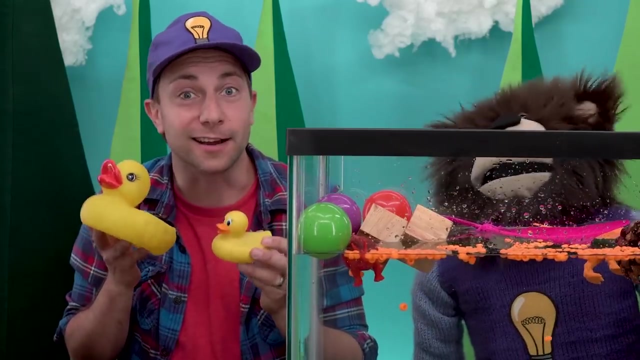 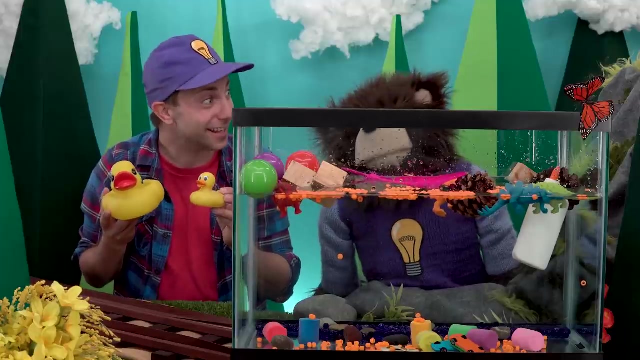 that is pretty neat, mayta. wow, okay, let's see what we have next, mayta. look, it's two rubber duckies, a mama ducky and a baby ducky. i bet you know what will happen when i put these rubber duckies in the water. should we do it, mayta? yes, should we put the rubber duckies in the tank? okay, first the 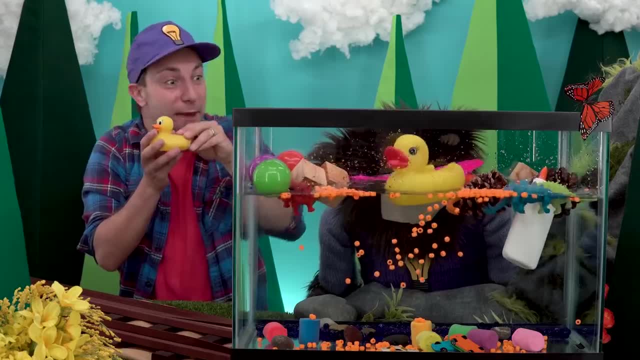 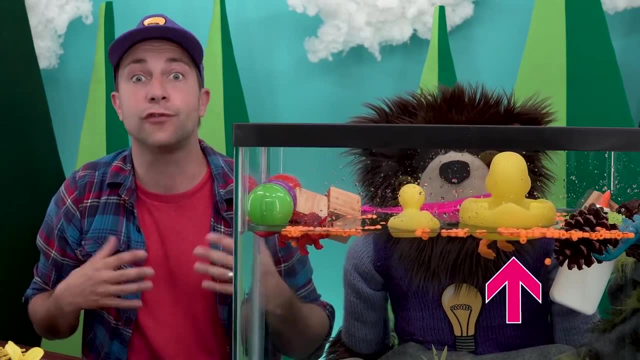 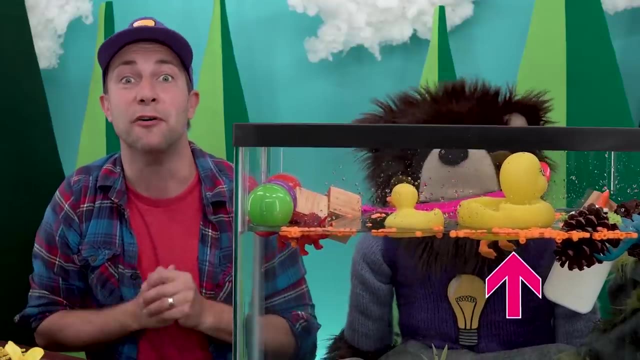 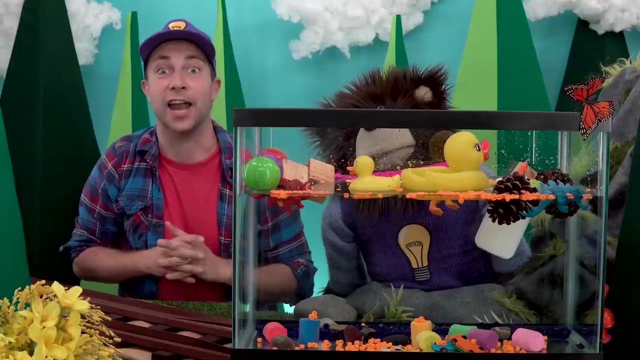 baby ducky and the mama duck, whoa, and then the baby duck. oh, look at them floating on top of the water. they are made of plastic and are full of air, so they are less dense than the water's density, which makes them float. wow, okay, before we go, i have one more thing that i want to put in our tank of water. are you ready, mayta? 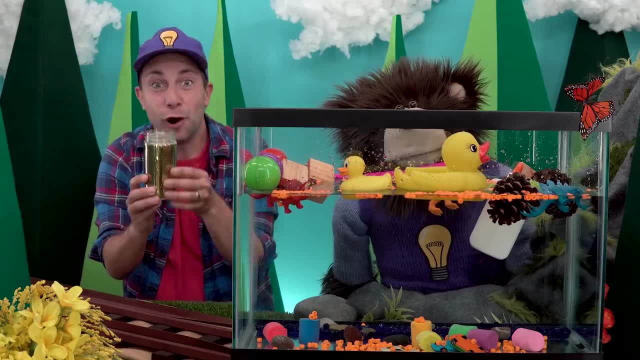 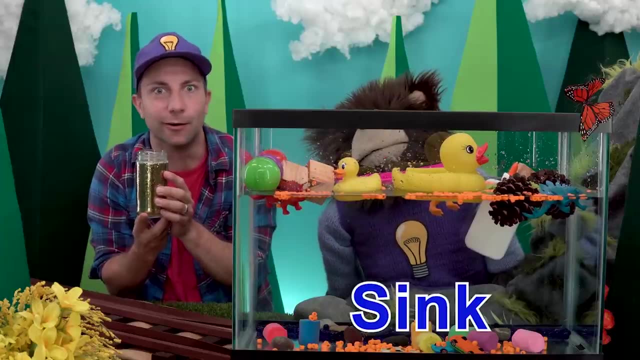 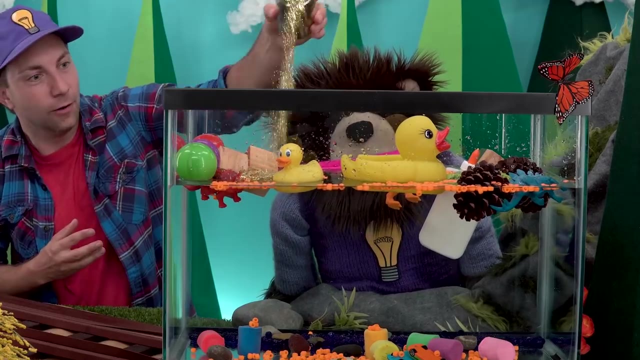 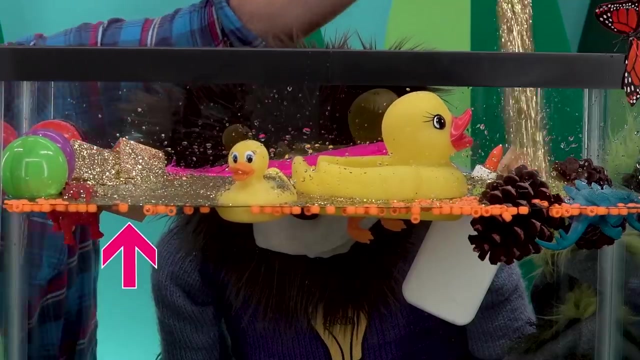 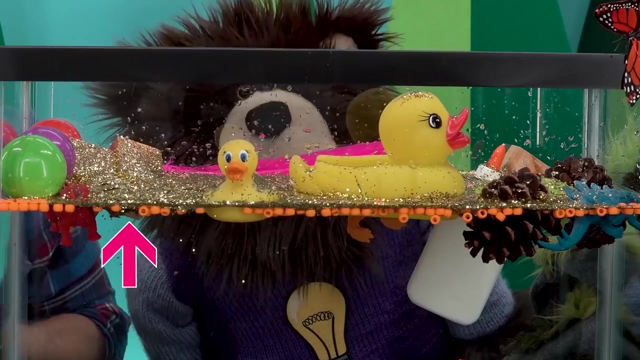 are you ready? i have a jar of gold glitter. do you think this glitter will sink or float? are you ready to see? okay, let's do it. wow, mayta, look, the glitter is floating on the top of the water. whoa, that is really neat. hey, what happens if we stir it up? 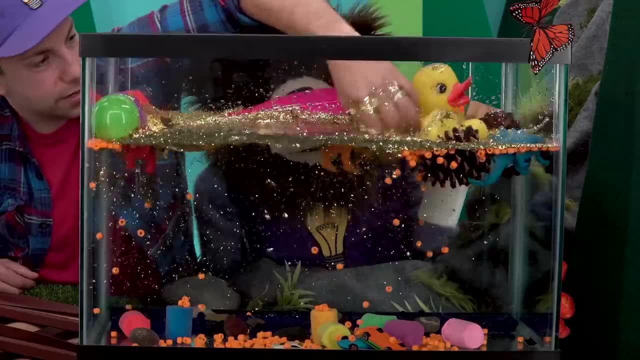 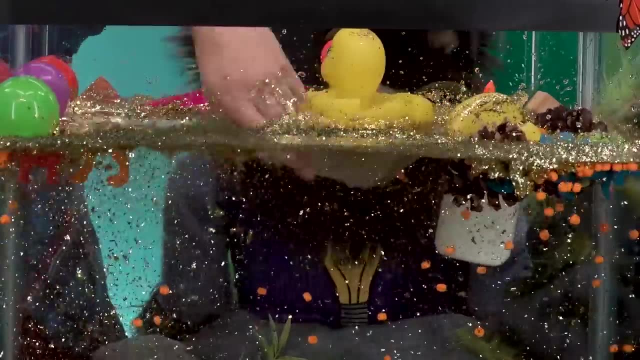 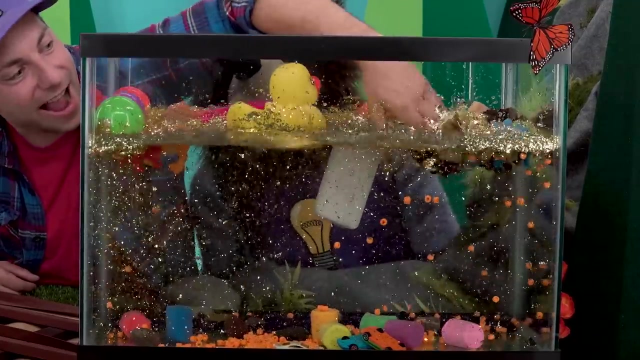 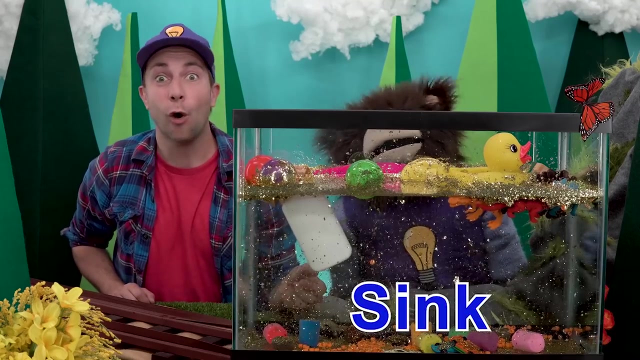 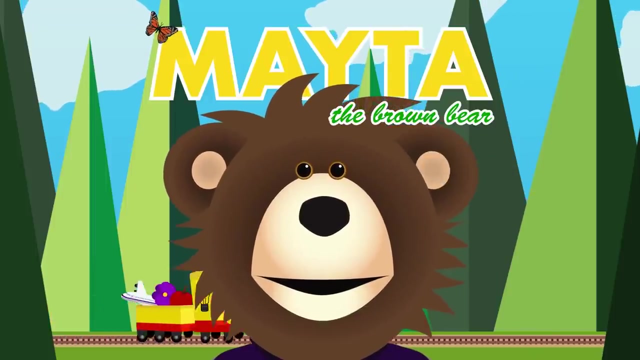 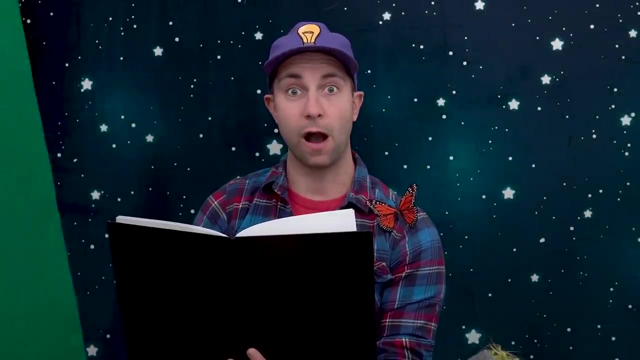 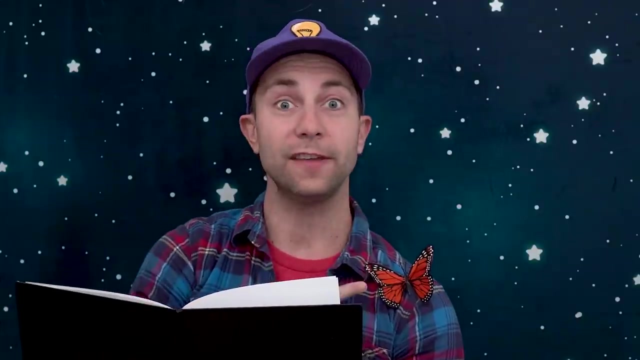 oh look, mayta, the glitter is going everywhere. that is so cool. it's floating and sinking. whoa, look at that. wow, that was a lot of fun playing the game sink or float. abby wants to go to space. oh hi, my name is b, like the letter b and this. this is mr butterfly. 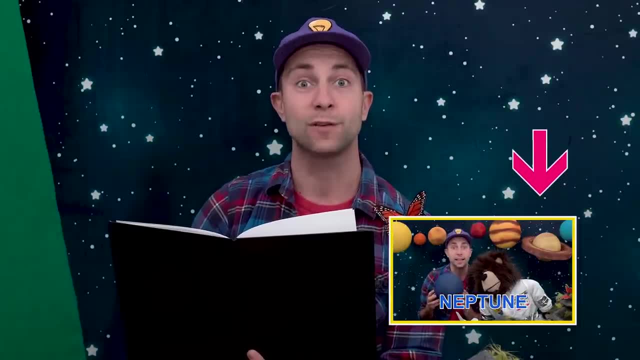 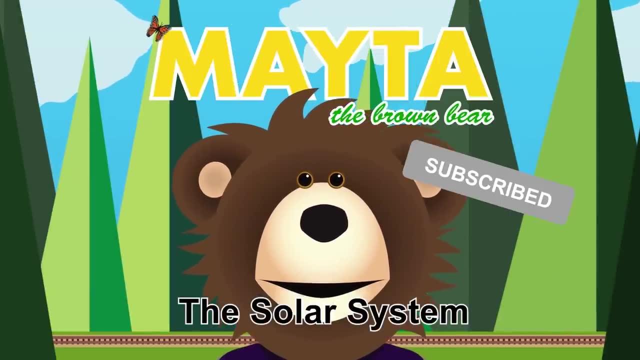 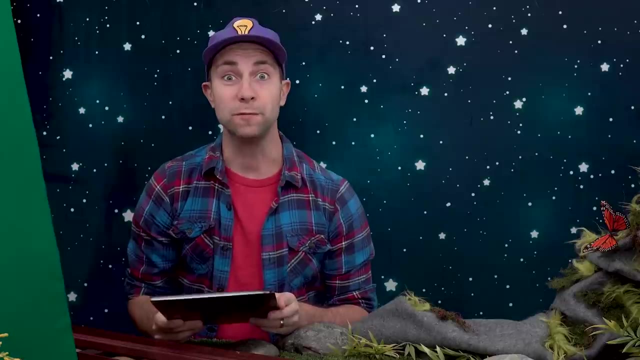 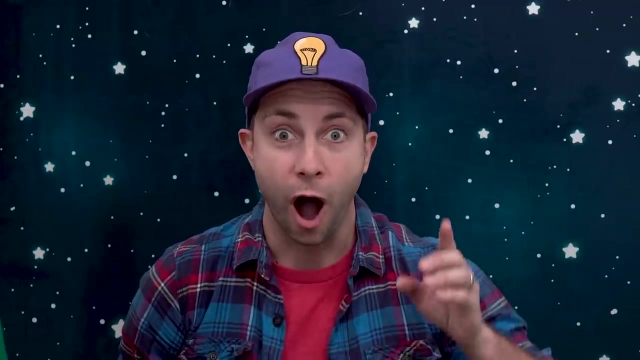 and we're waiting for our friend mayta to wake up from his nap so we can learn about the solar system. The brown bear. do you know who mayta is? mayta is a brown bear that lives in this forest. i have an idea. why don't? 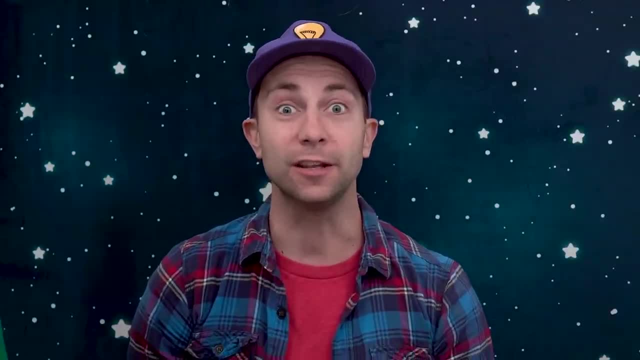 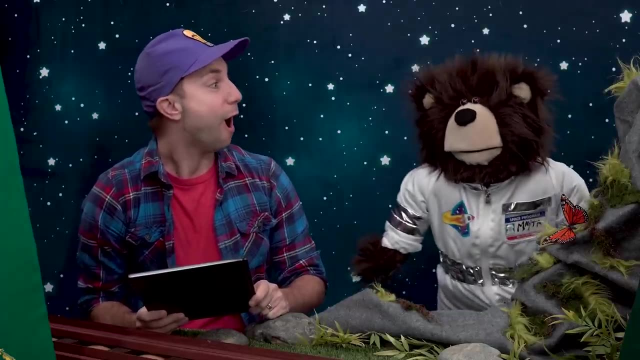 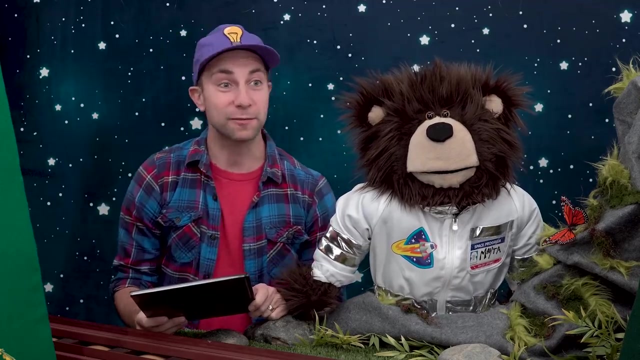 we wake made to up from his nap and together we can learn about the solar system. mayta, oh, Are you up from your nap yet? Where are you, Mayta? It's Mayta And look, Mayta, you are ready to go to outer space. 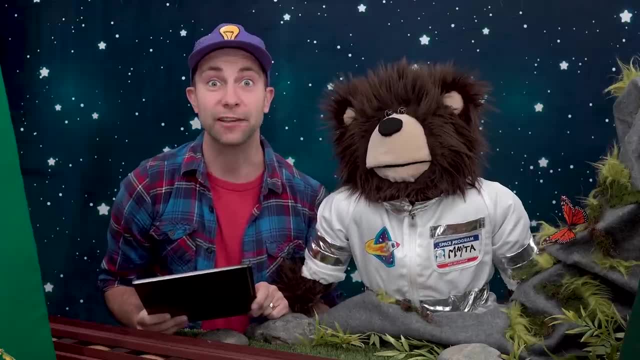 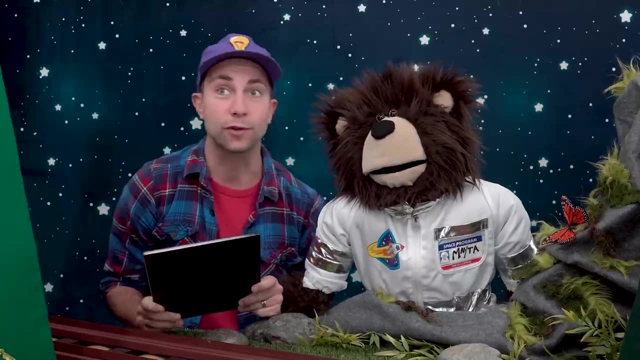 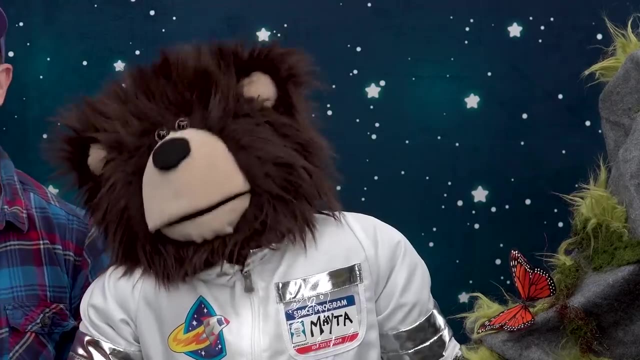 Wow, Mayta is dressed up like an astronaut. Do you know what an astronaut is? An astronaut is someone who travels all the way up to space in a rocket or a space shuttle. Wow, Mr Butterfly and I just finished our book about space. 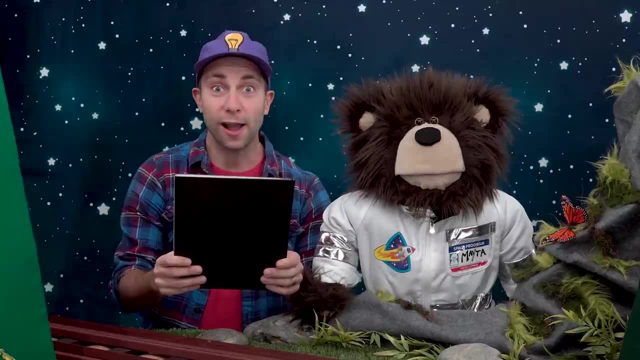 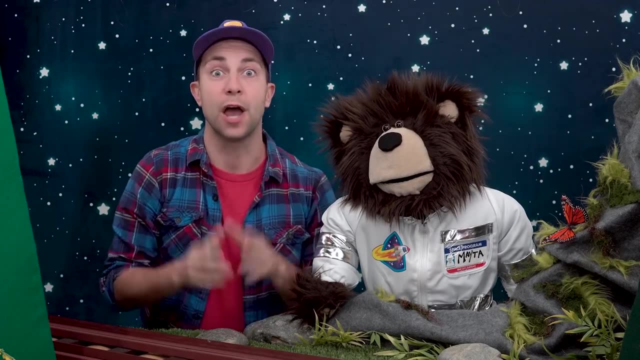 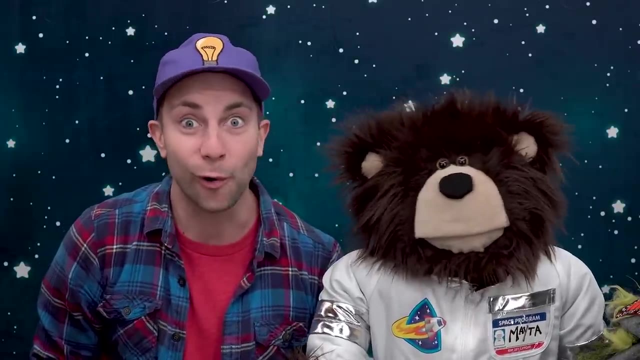 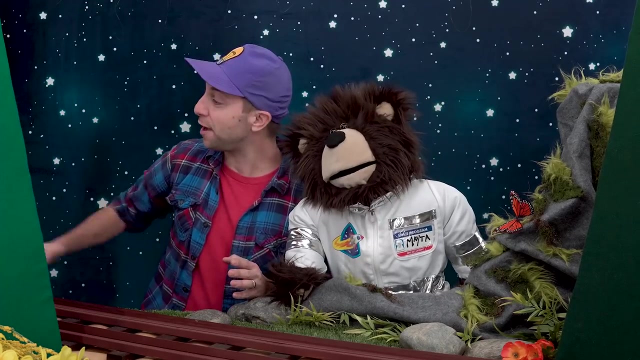 Do you know what color this book is? That's right, it's black. Well, together we are going to learn about the solar system. Do you hear that? No, Well, listen harder. Do you hear that? It's the Idea Train? 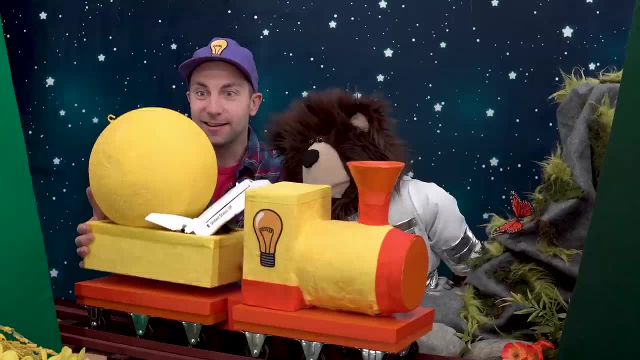 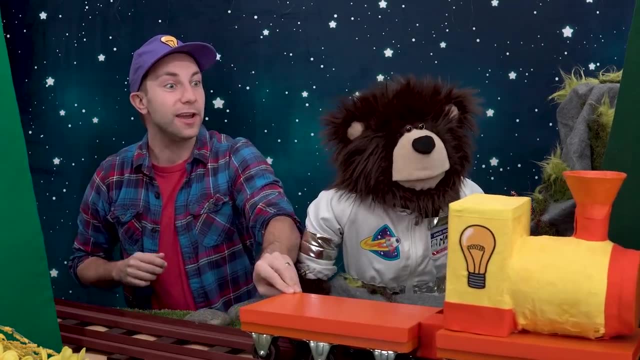 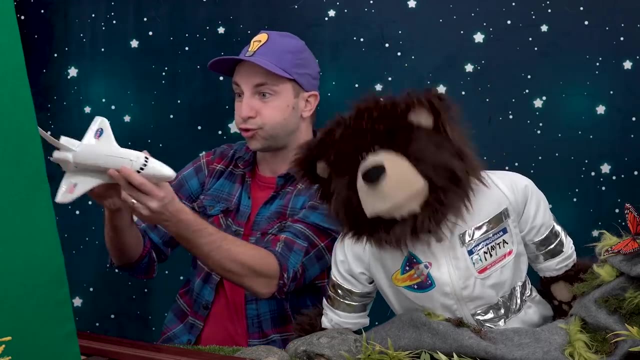 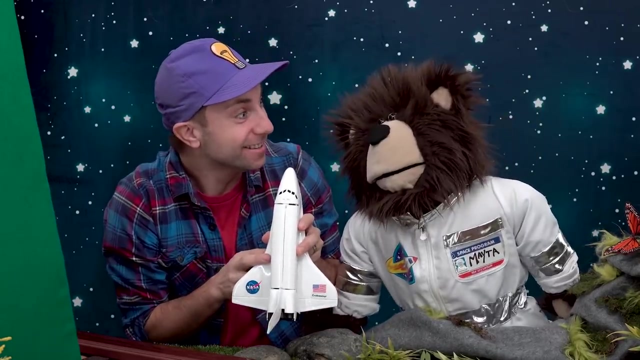 Whoa Mayta, look what's in the box. All right, we'll put this over here. Thank you, Idea Train. Whoa Mayta, Do you know what this is? Mm-hmm, yes, Do you know what this is? 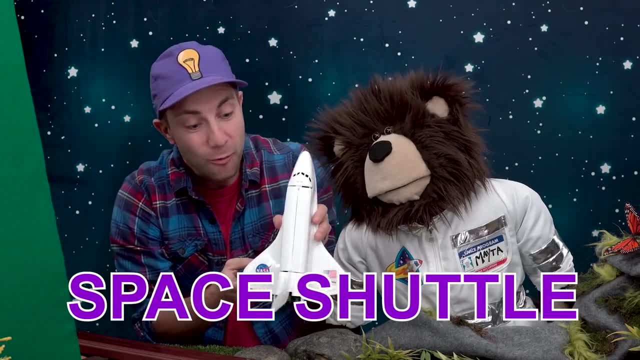 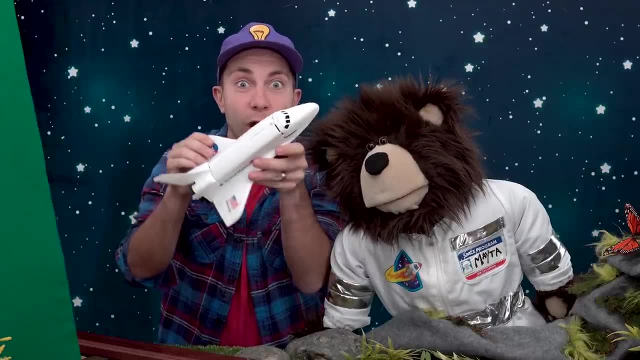 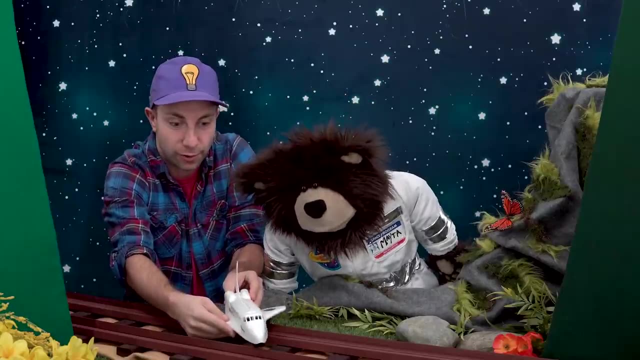 That's right, it's a space shuttle. Wow, Astronauts ride inside a space shuttle when they're up in space. Whoa, okay, let's put our space shuttle right here, All right? Hmm, Wow Mayta. 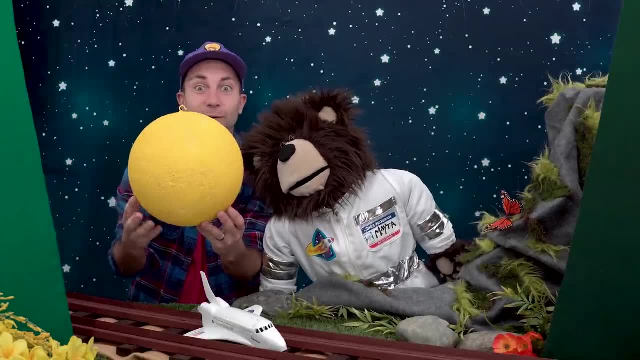 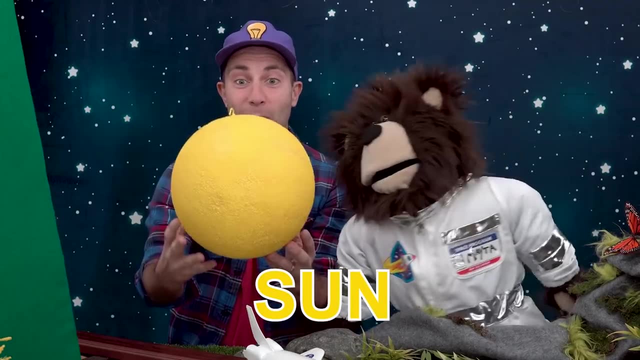 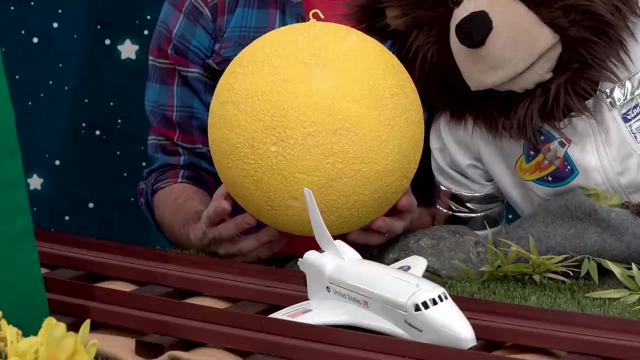 Do you know what this is? Whoo Whoa, it's the sun. Wow, The sun is a very big star found of the center of our solar system. Wow, look at that, Mayta. I have an idea. why don't we use our space shuttle? 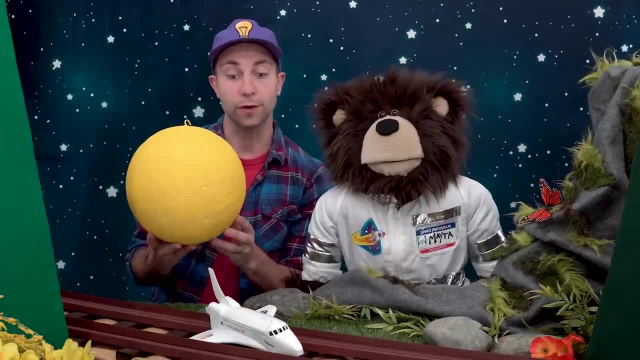 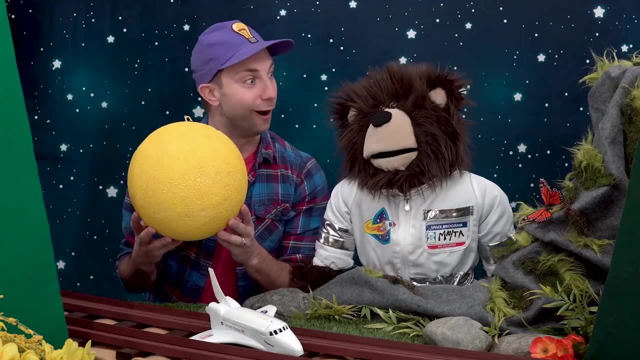 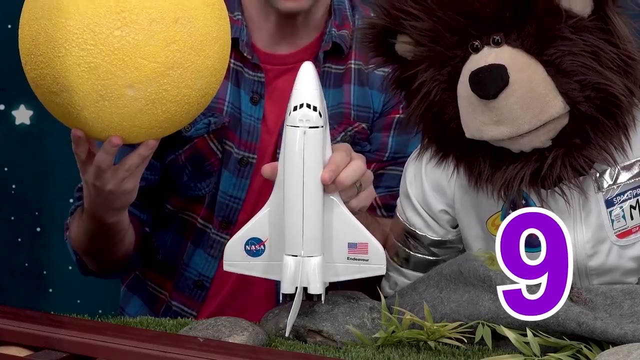 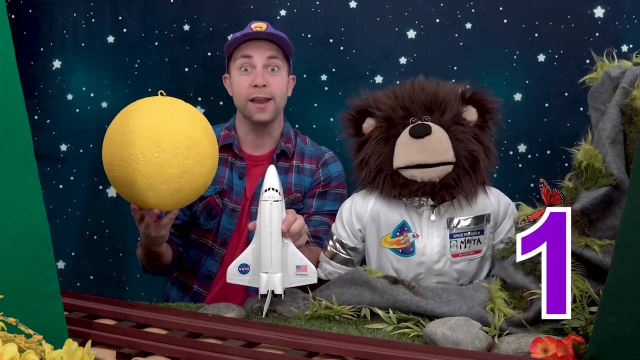 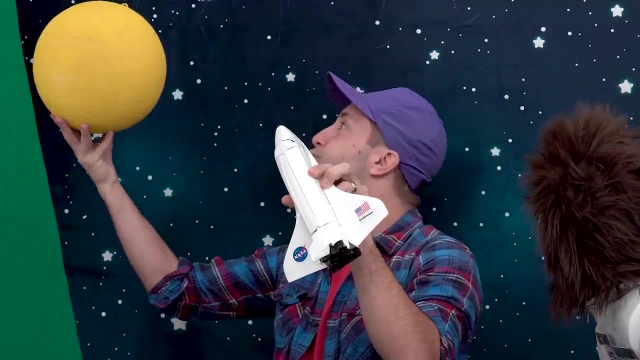 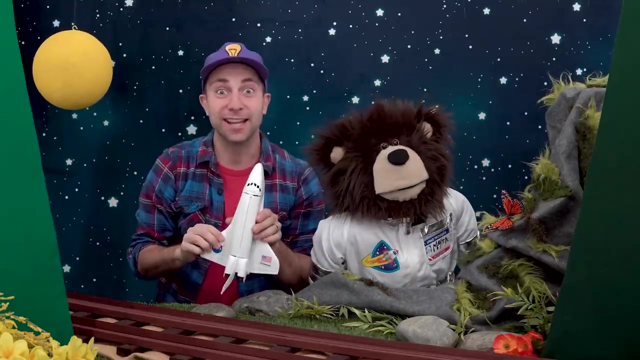 to fly the sun all the way up to outer space and put it outside of our solar system. Yeah, Yay, put it where it belongs. should we do that? yeah, okay, ready, ten, nine, eight, seven, six, five, four, three, two, one. blast off, we did it. the sun is back in space, the sun mate. 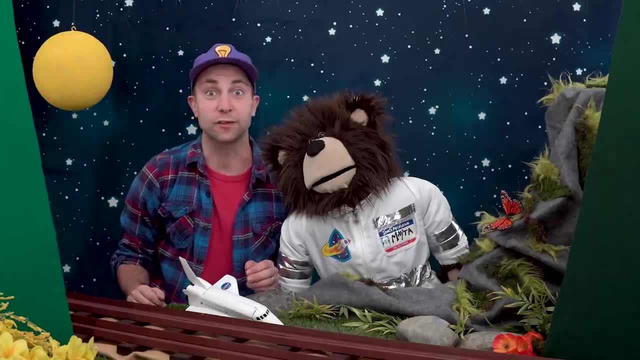 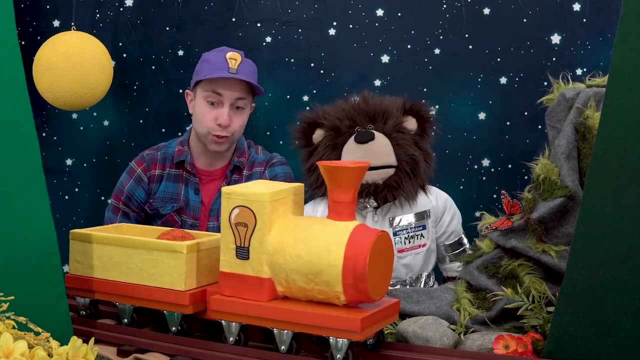 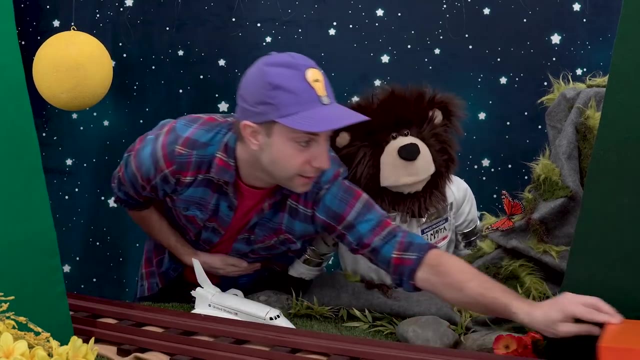 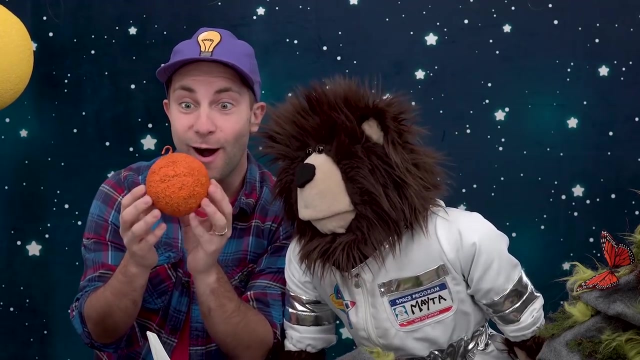 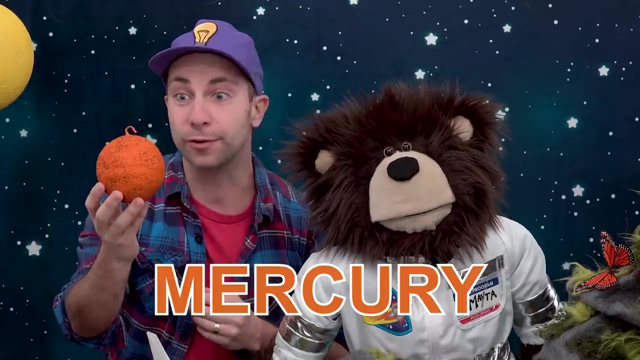 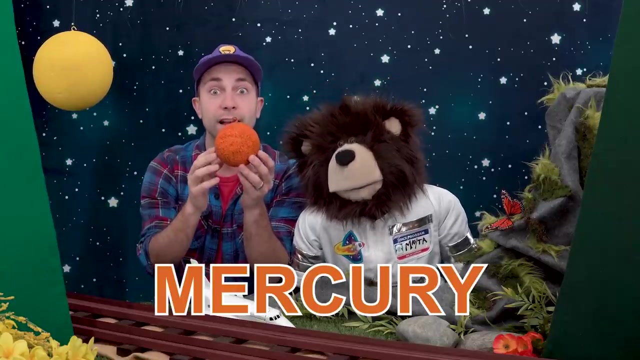 are you ready for the idea train to bring our first planet in the solar system? yes, okay, all right, thank you, idea train. whoa, look at this little planet, mayta. do you know what planet this is? that's right, it's mercury. wow, mercury is the closest planet to the sun. 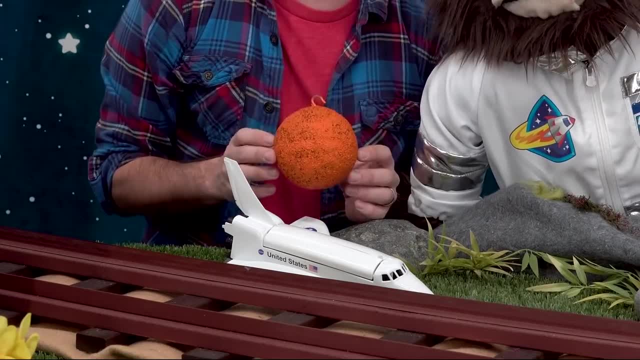 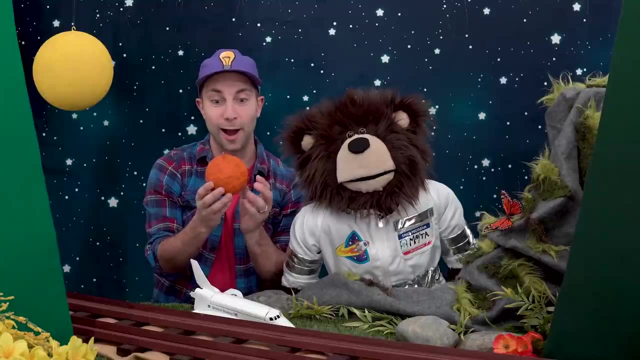 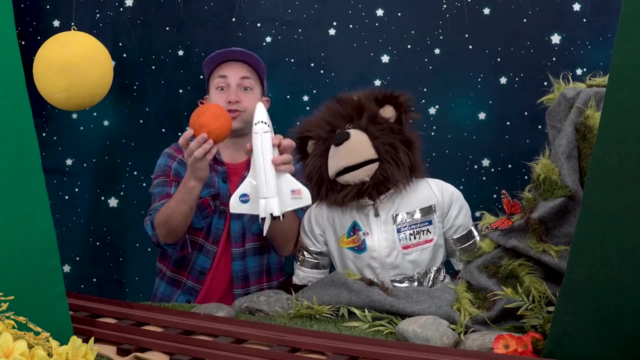 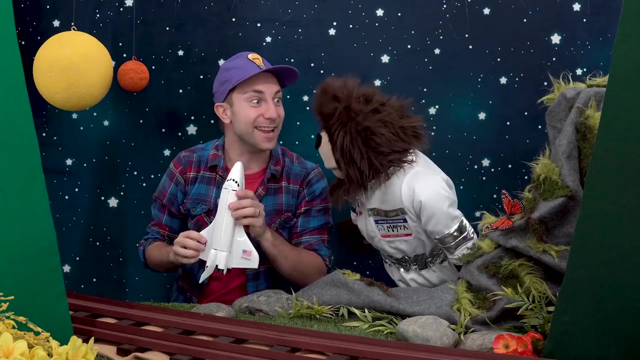 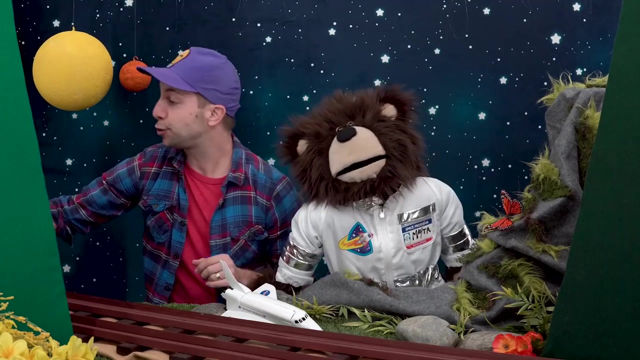 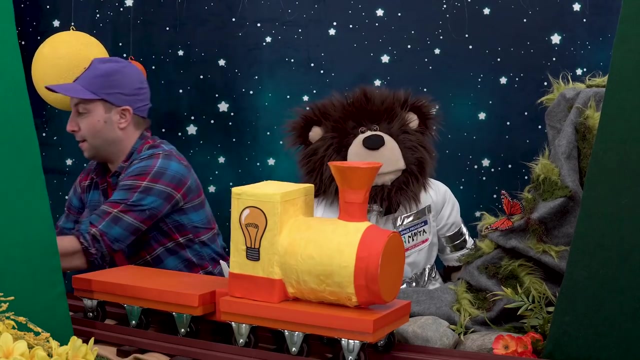 this planet does not have an atmosphere. it's a ball of iron covered by a very thin layer of rock. wow, mayta, let's fly mercury up into space. we did it. mayta, mercury, mayta. here comes the idea train with the next planet. wow, thank you, idea train. 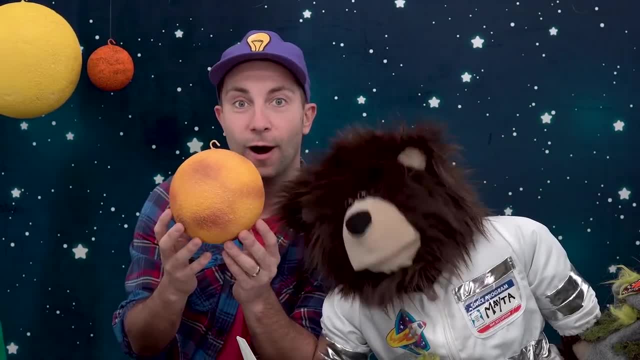 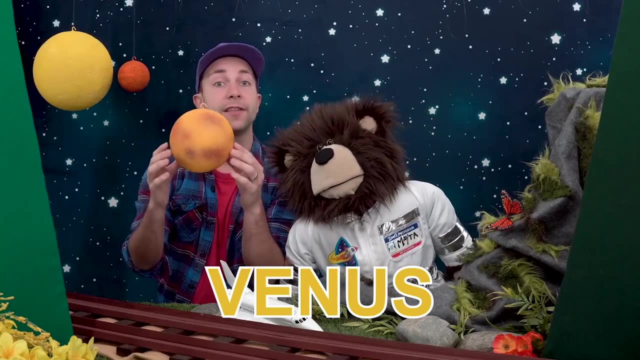 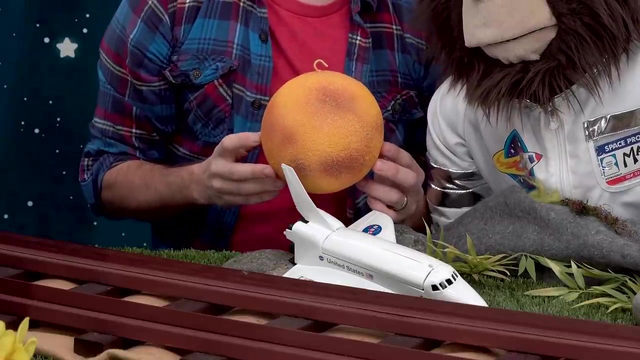 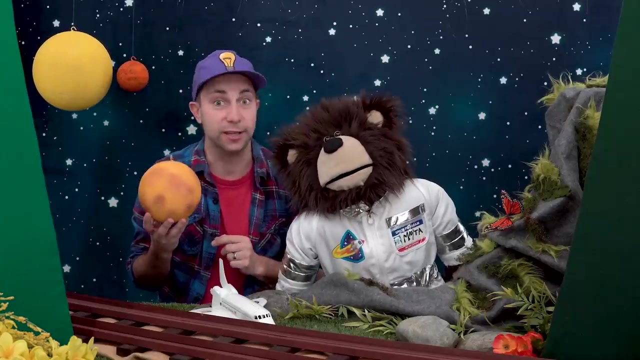 oh, mayta, look at this planet. do you know what the name of this planet is? it's venus. venus is the second planet from the sun and it's the second brightest object in the sky after the moon. mayta, let's blast this planet up. 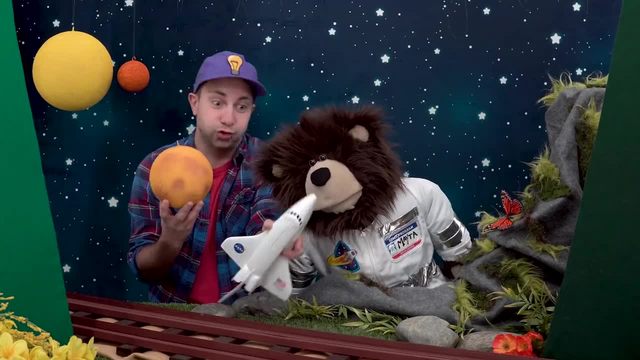 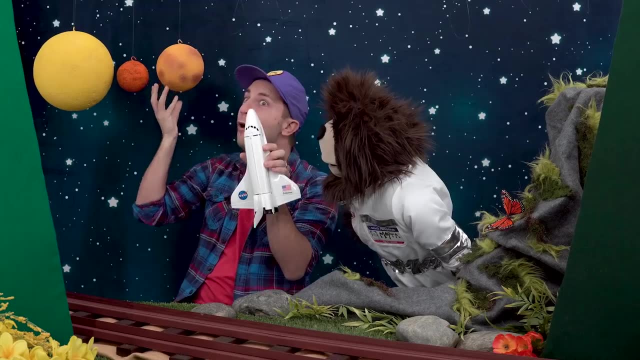 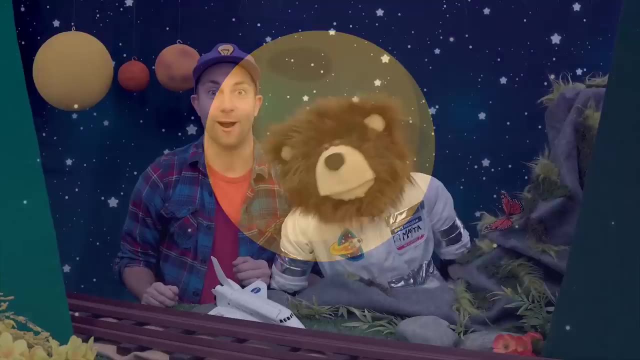 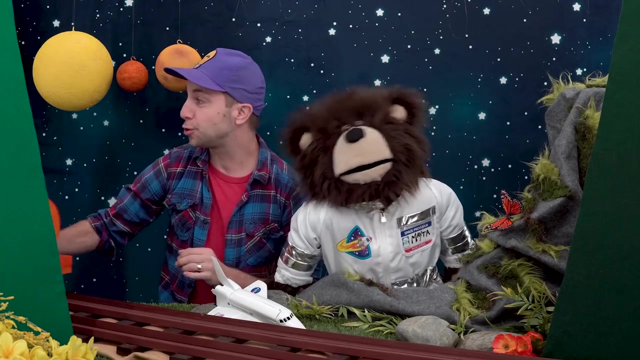 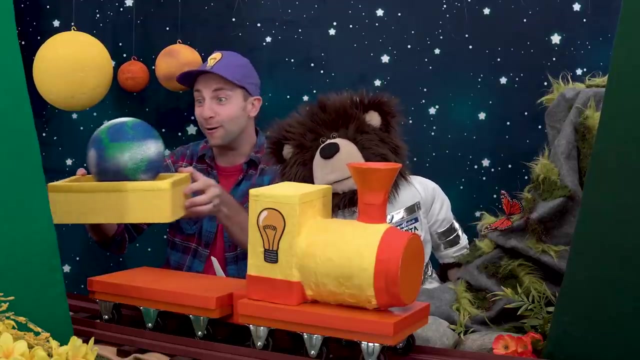 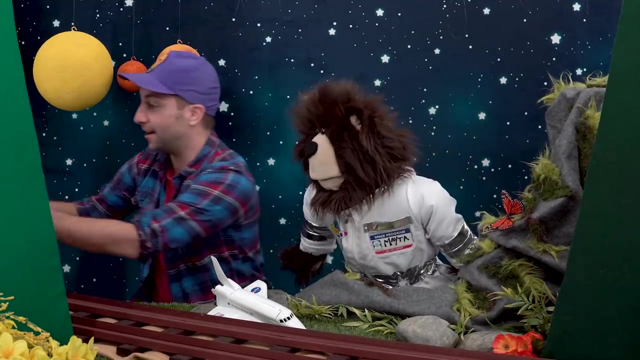 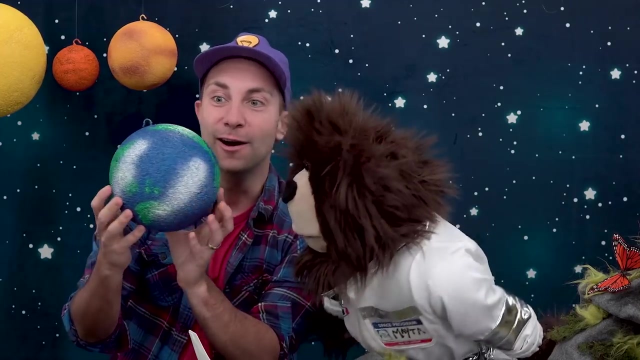 into space. here we go. whoa, we did it. mayta, venus is now in space. venus, Meta, here comes the Idea Train with another planet in our solar system. Whoa, Meta, look at this planet. Wow, Do you know what this planet's name is? 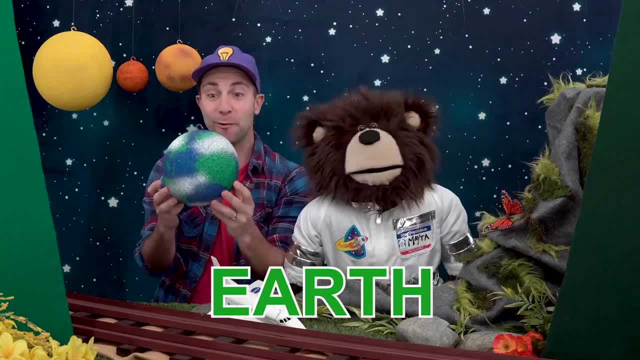 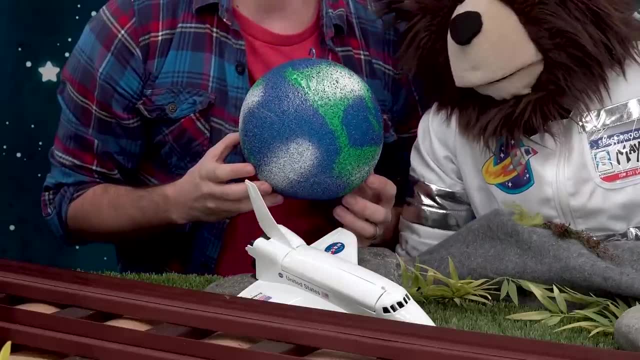 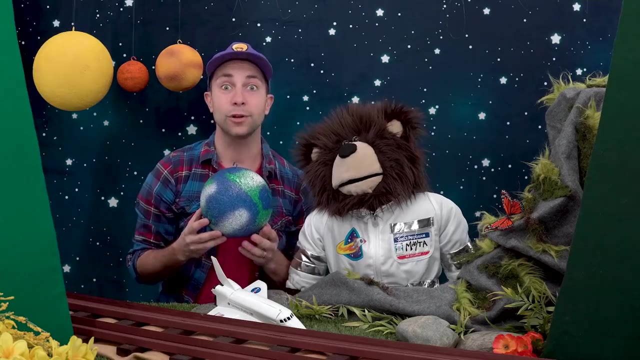 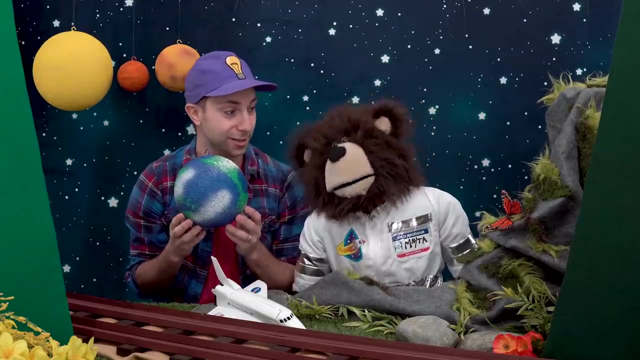 That's right, It's Earth. Wow, This is planet Earth. Earth is the only known planet that we know of that supports life. It's where you and Meta live. We live on Earth, Meta. should we deliver this Earth back up into space? 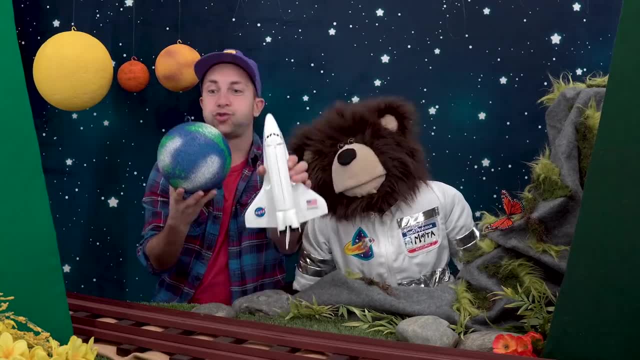 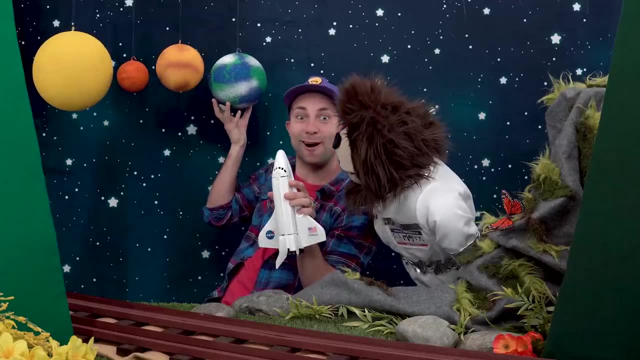 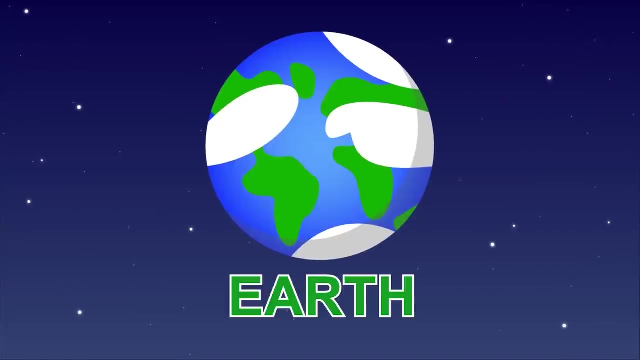 Yes, Okay, Whoa, That's pretty neat Earth. Here comes the Idea Train: Chugga-chugga-chugga-chugga-chugga-chugga-chugga-chugga-chugga-chugga-chugga. 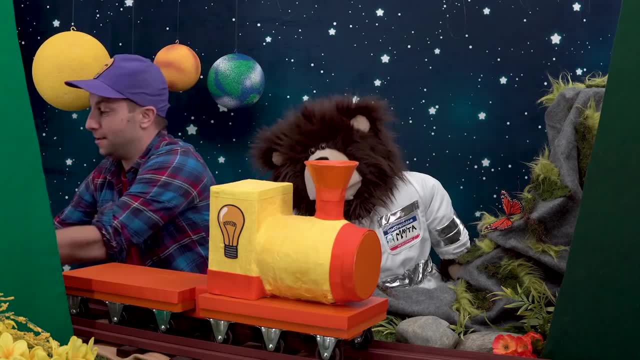 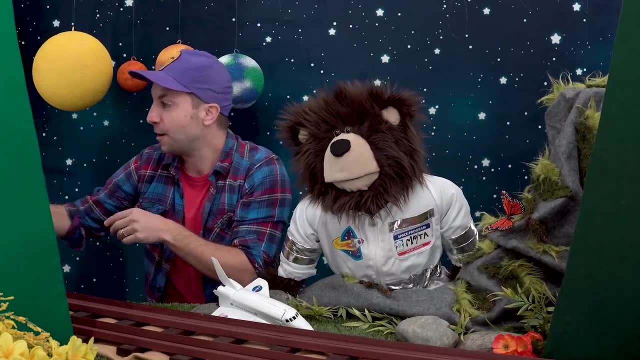 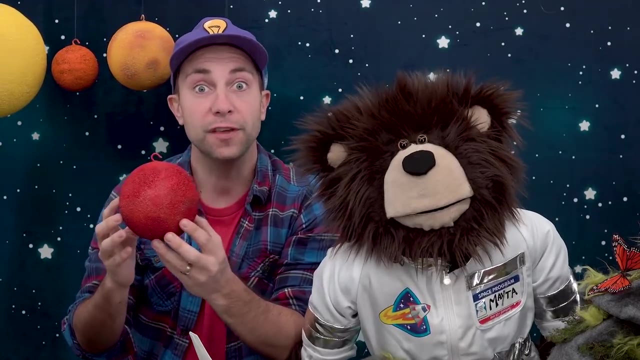 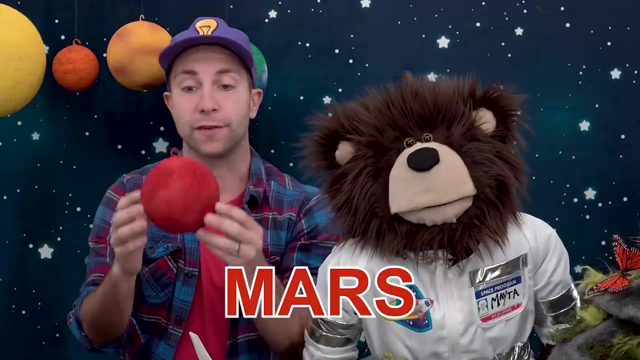 Oh, Thank you, Idea Train. Thank you, Whoa Meta. Look at this little red planet. Do you know what this planet is named? That's right, Mars. Mars is the fourth planet from the Sun and the second smallest planet. 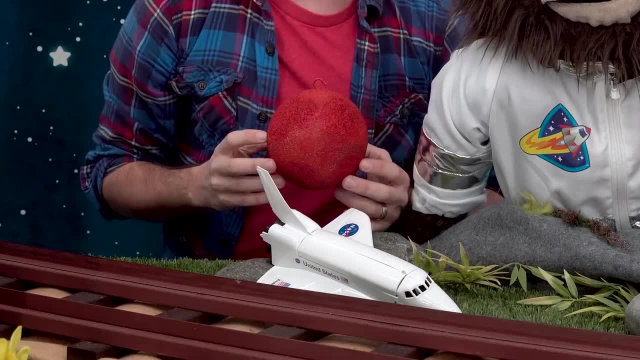 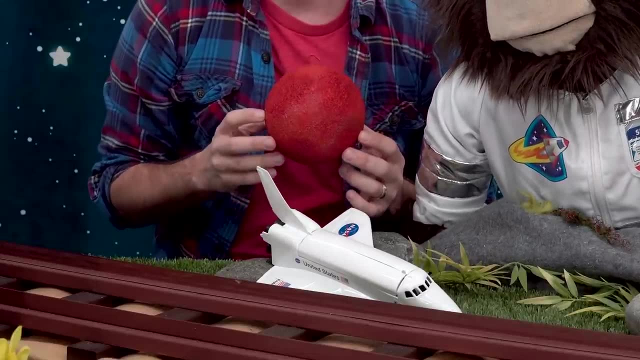 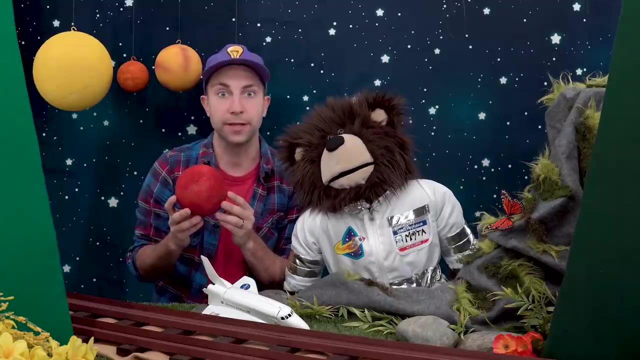 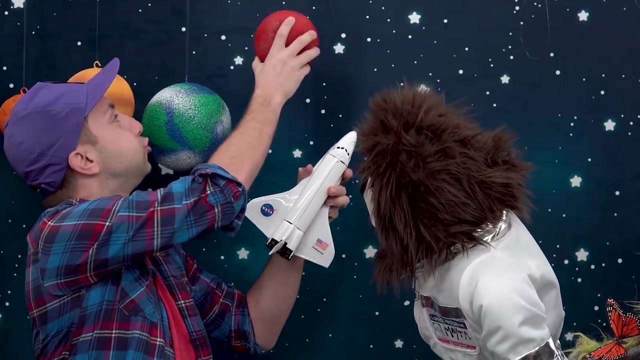 in the solar system. Did you know that the largest volcano in our solar system is found on this little red planet? Wow, Meta, should we blast Mars back up into space? Yes, Okay, Pffft, Whoa, We did it, Meta. 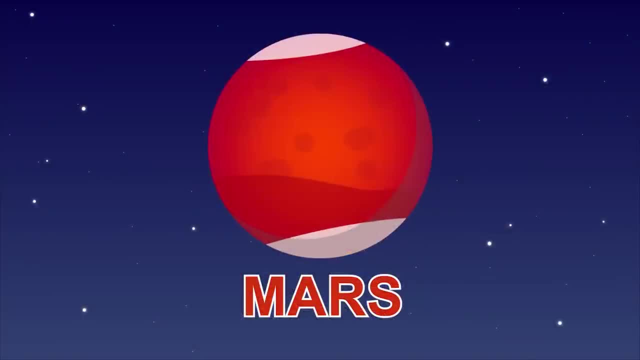 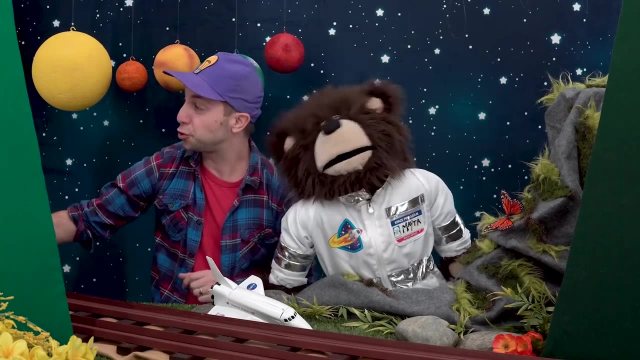 Mars is back in space. Mars, Are you ready for the next planet in our solar system? All right, Chugga-chugga-chugga-chugga-chugga-chugga-chugga-chugga-chugga-chugga-chugga-chugga-chugga-chugga-chugga-chugga-chugga. 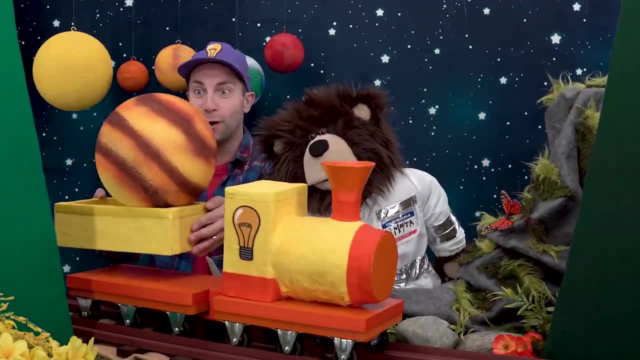 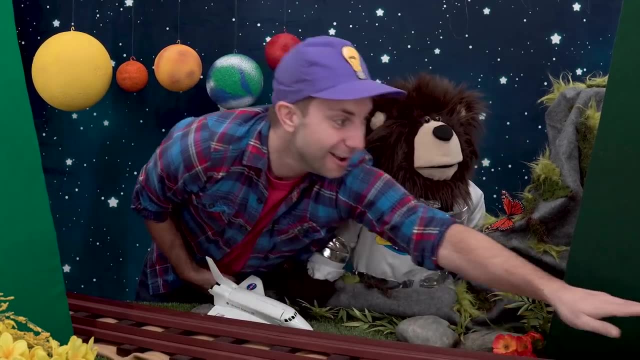 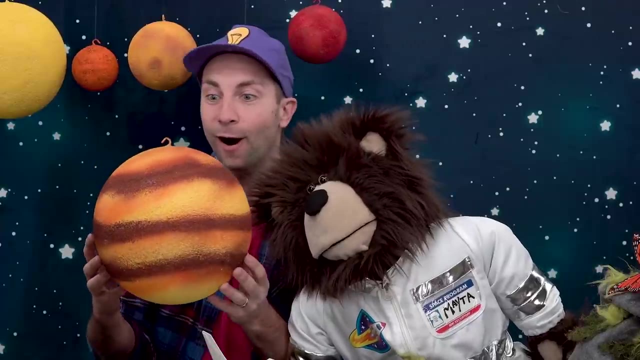 Shhh, Whoa, I've got to be careful, Meta, Mm-hmm, Mm-hmm, Wow, Wow. look at this planet, Mayta. This is a very big planet. Do you know what this planet is? 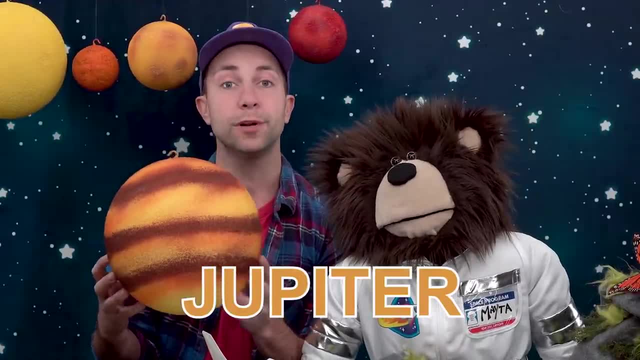 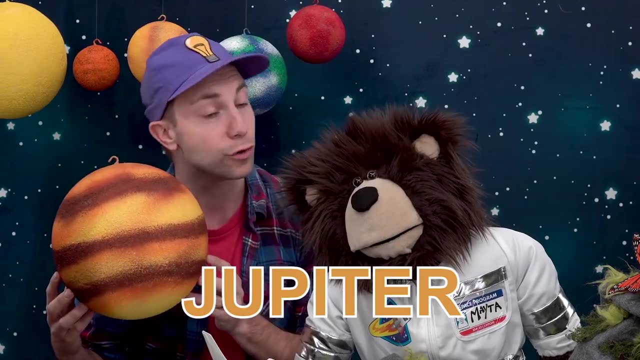 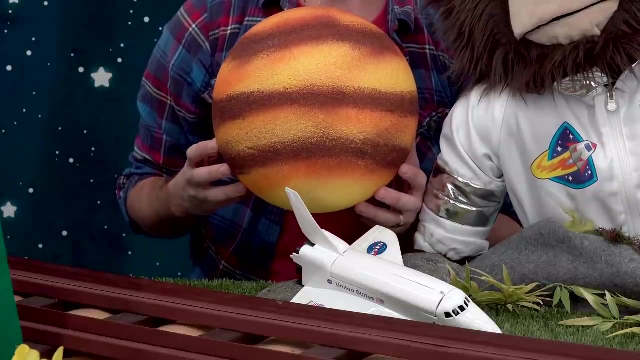 That's right, it's Jupiter. Jupiter is the fifth planet out from the sun and the largest planet in our solar system. Jupiter is known as the gas giant because it is made mostly of gases. Mayta, let's blast Jupiter back into space. 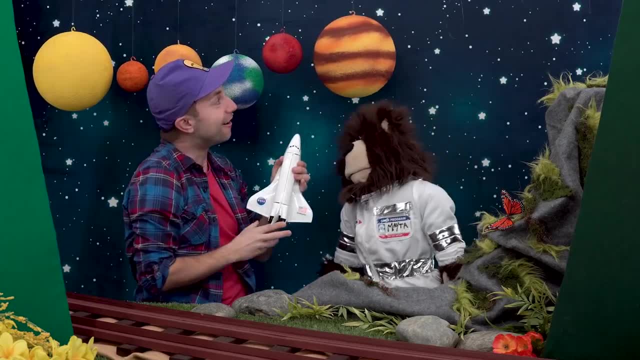 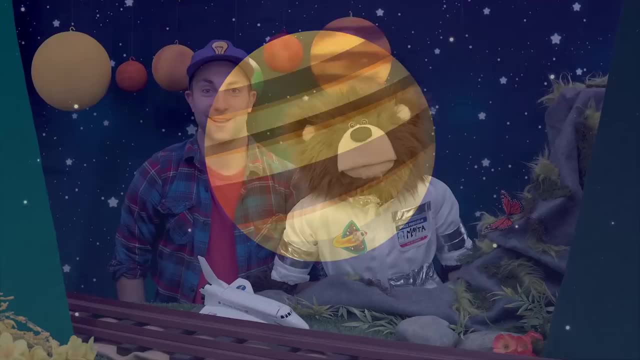 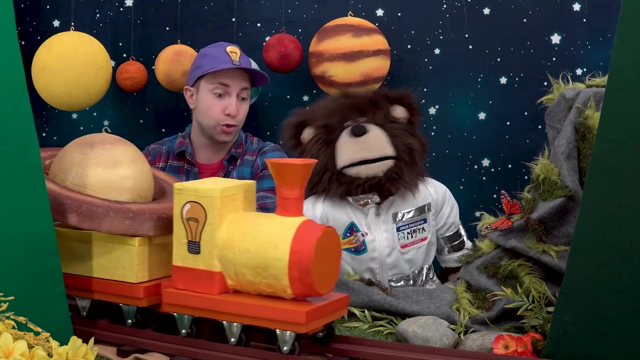 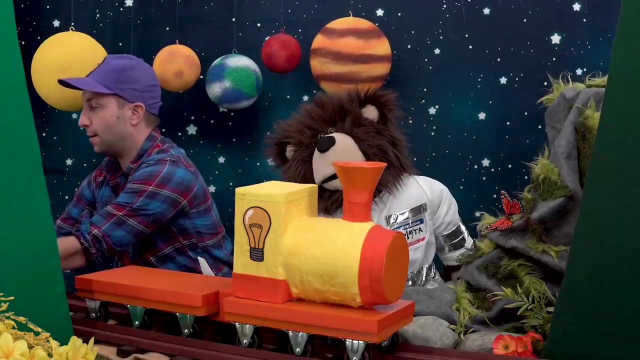 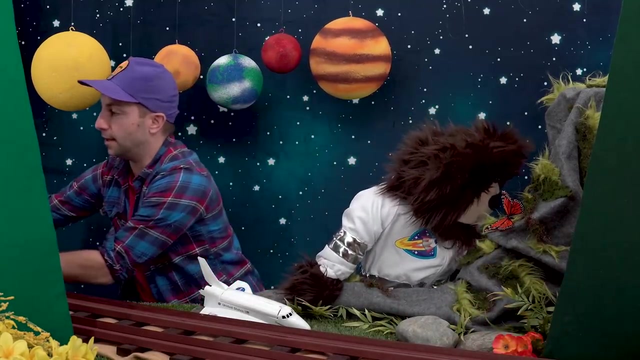 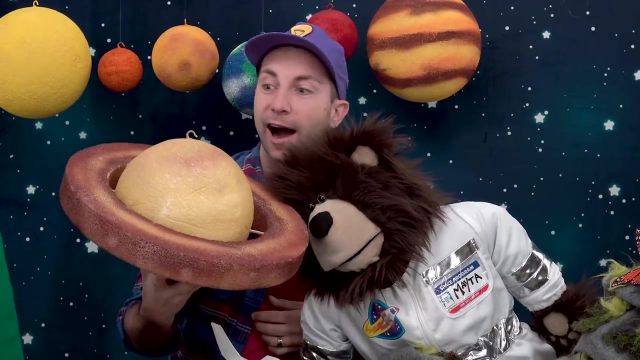 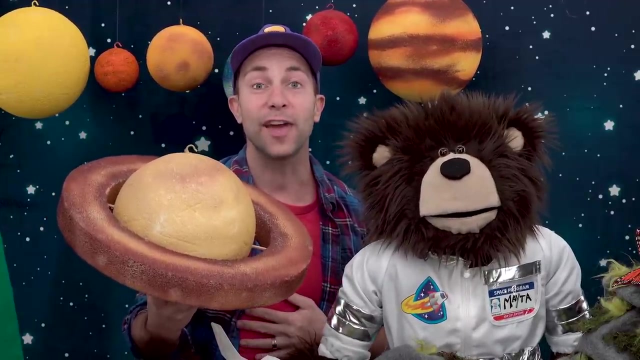 Whoa, All right. Jupiter is a big planet. Jupiter, Here comes our next planet. Whoa, Thank you, Idea Train Mayta, Look at this planet. Hmm, Wow, Do you know what this planet is? That's right, it's Saturn. 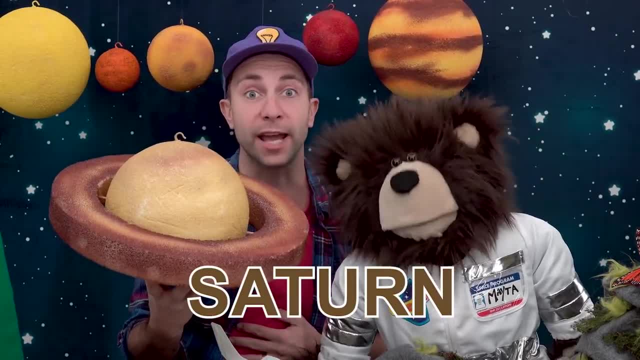 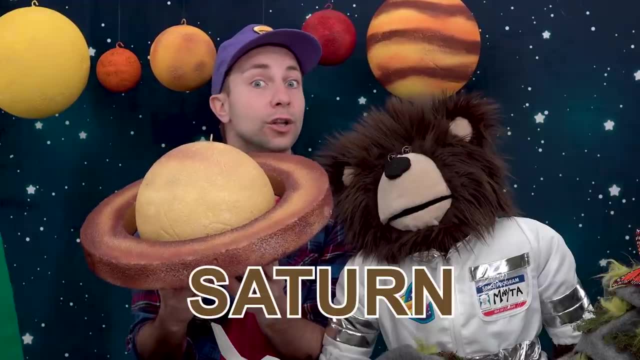 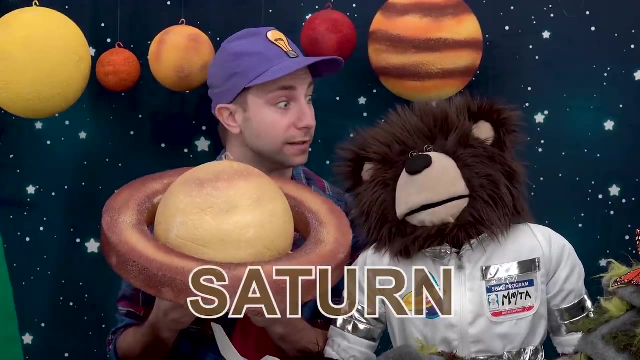 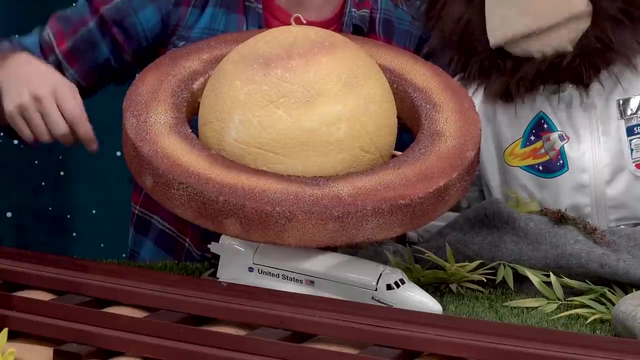 Hmm, Saturn is the sixth planet out from the sun, Wow, And Mayta, it is the second largest planet in the solar system, Mm-hmm- And the lightest planet. Hmm, It's best known for its amazing rings that go around the planet. 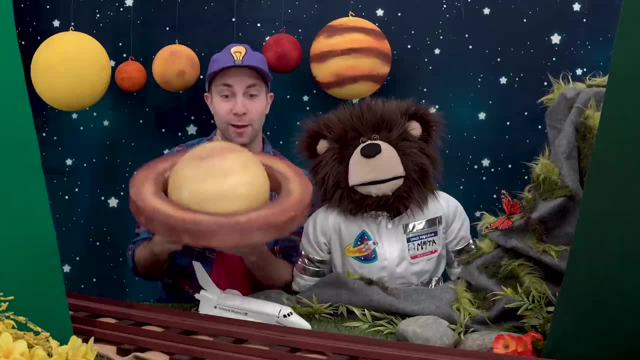 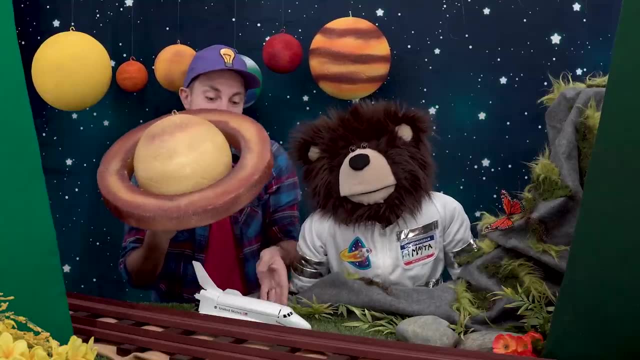 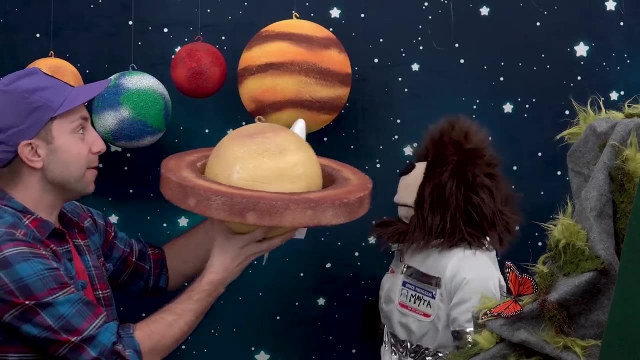 Saturn is also a gas planet. Wow, Mayta, Should we put Saturn back up in space? Mm-hmm. Okay, Here we go. Watch out, Mayta, We're coming through Shh Mm-hmm. 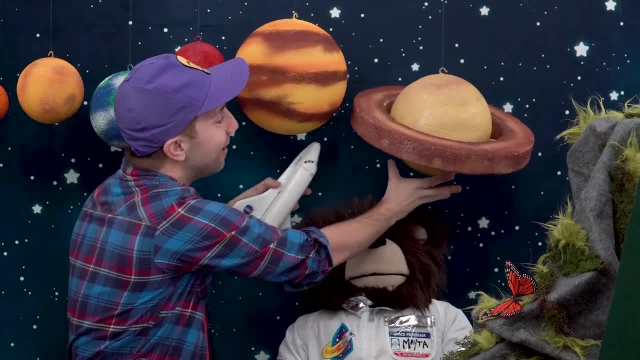 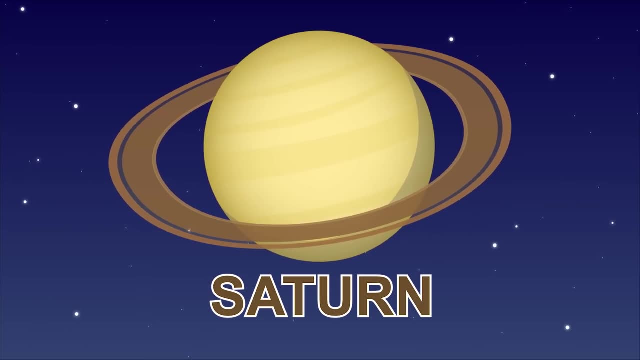 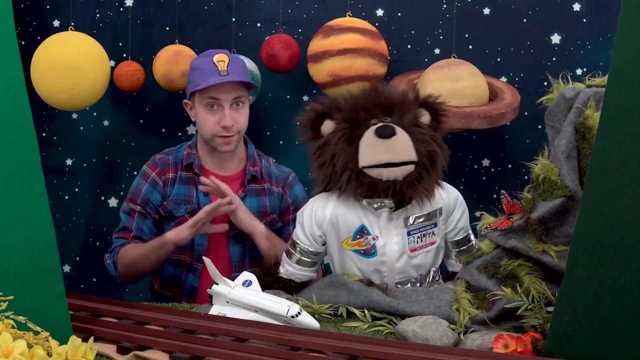 Ooh Whoa, We did it. Mayta, Saturn. Oh, Do you know what time it is? It's time to dance. We should dance. This is where we stop what we're doing. stand up and dance. 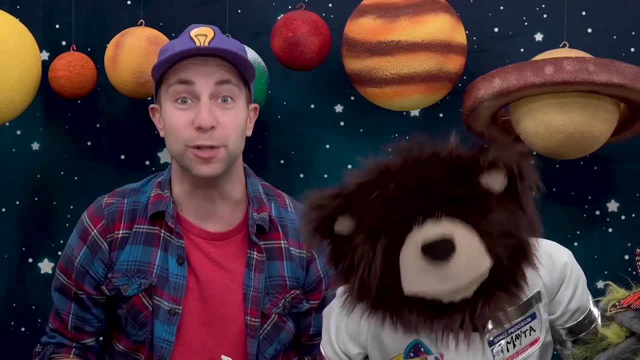 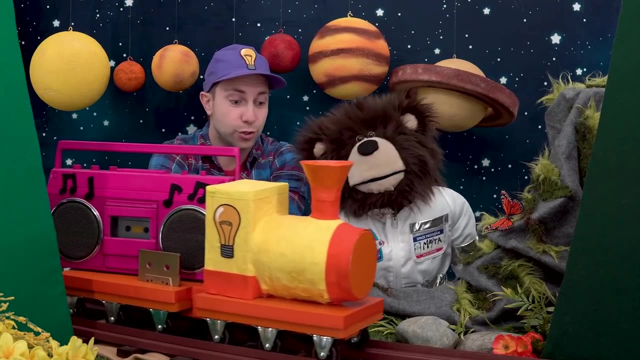 You can do whatever dance move you feel like doing. Oh, it's the Idea Train: Chka-chka-chka-chka, Chka-chka-chka-chka-chka, Chka-chka-chka-chka, Chka-chka-chka-chka. 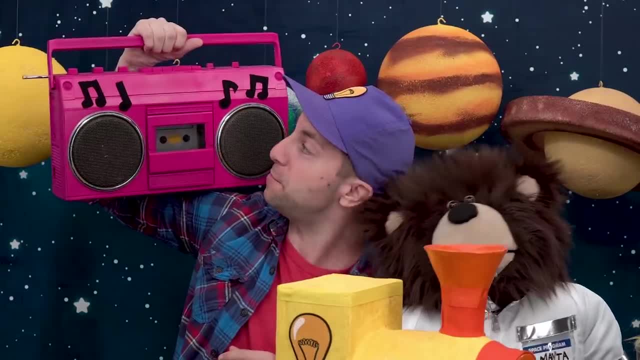 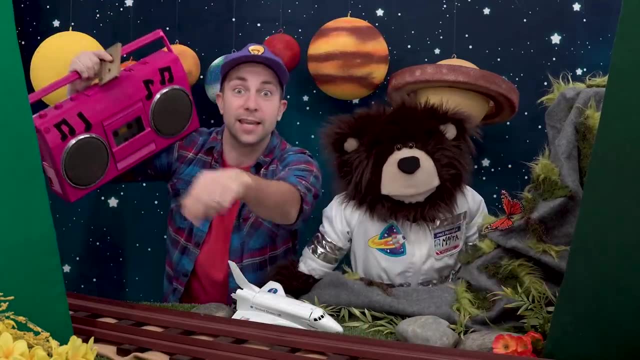 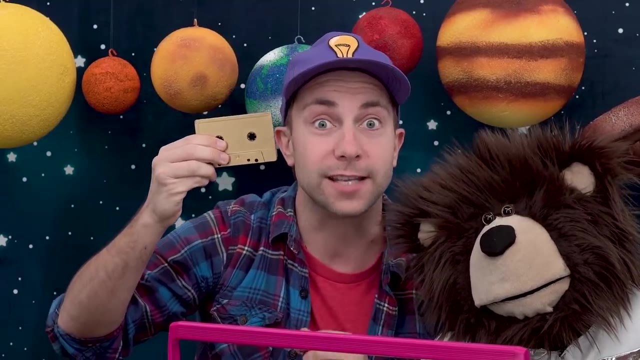 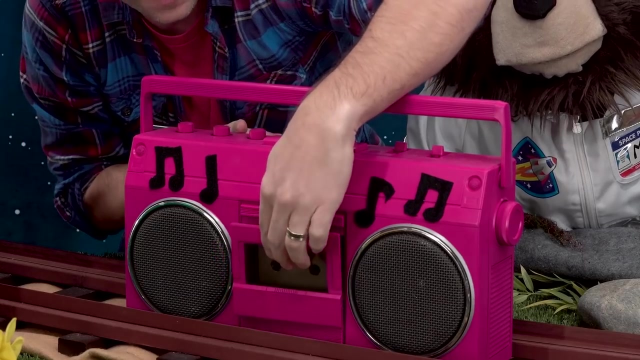 And look, it's Pinky the Boom Box. Woo hoo, Hi, Pinky the Boom Box. All right, Thank you, Idea Train. Woo hoo, Pinky the Boom Box played a very, very good performance, our music. we take this golden cassette tape and put it in here, and then we push. 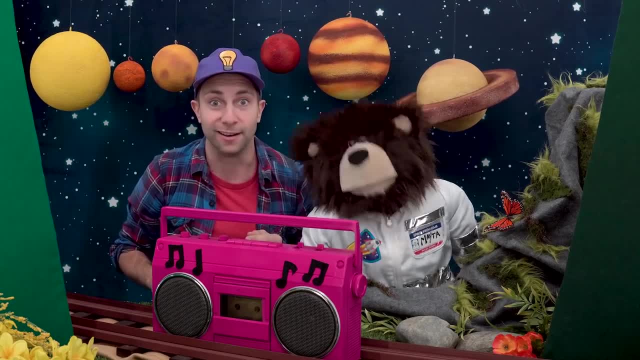 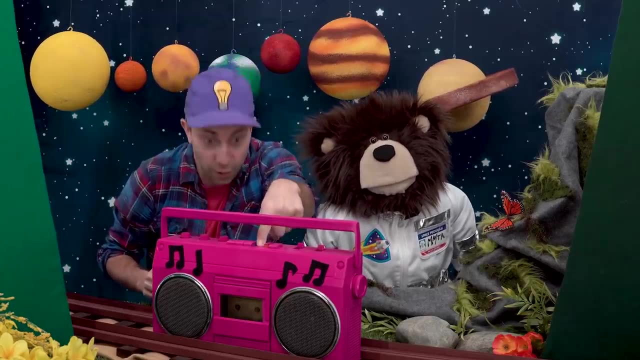 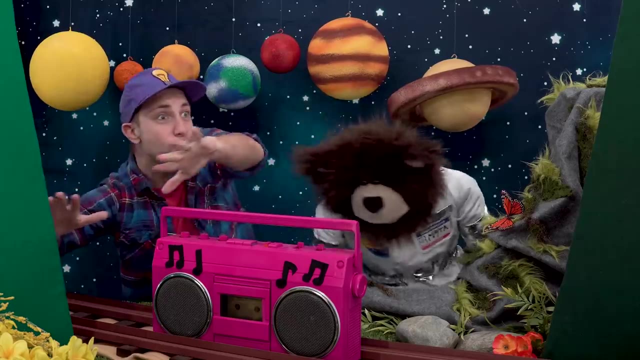 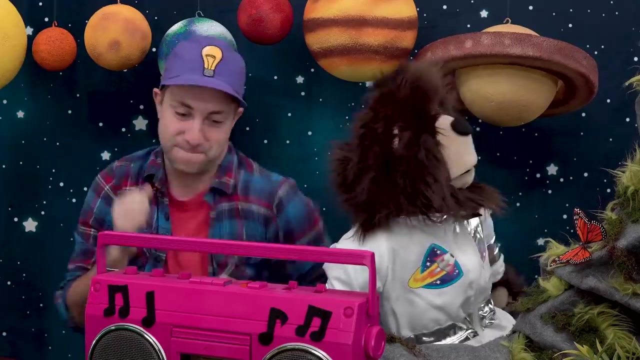 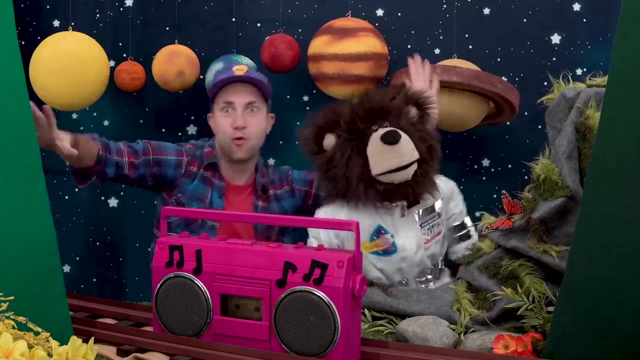 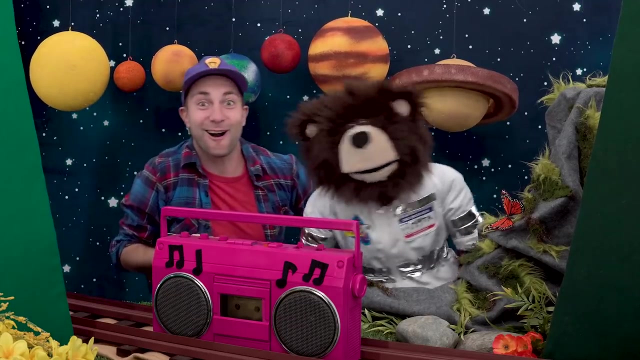 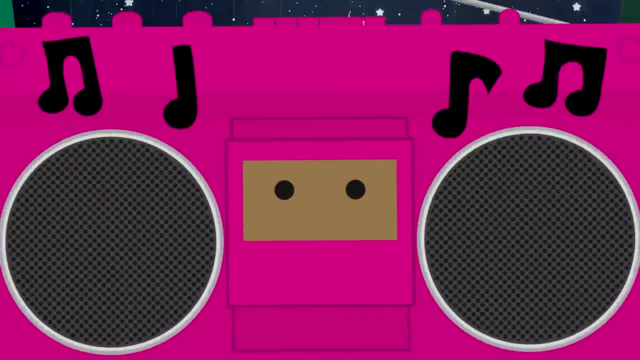 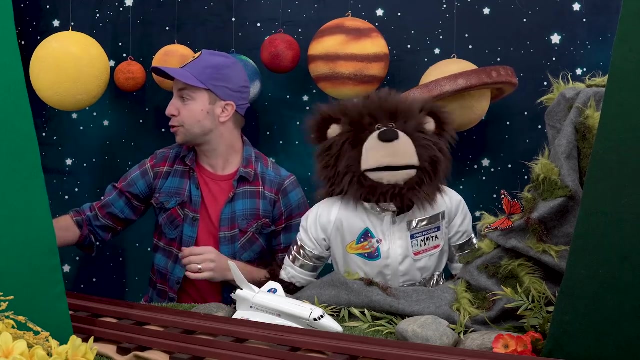 the button with the triangle on it, the play button. are you ready to dance? yes, okay, I'm going to push the button now. that was a lot of fun. okay, let's get back to what we were doing. doing. Are you ready for the next planet in our solar system? You are All right. 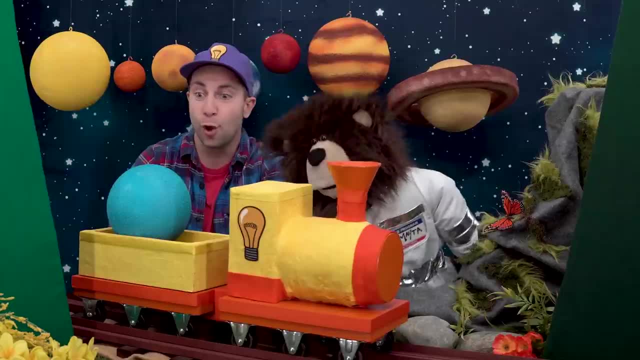 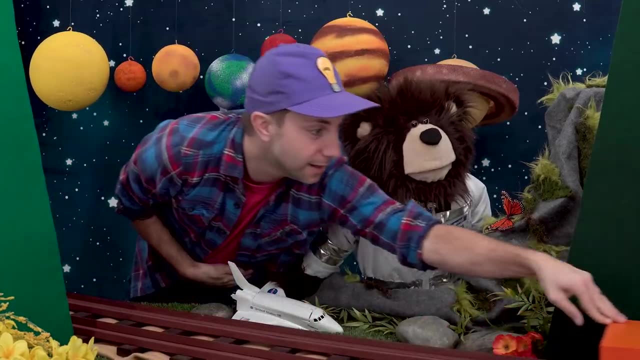 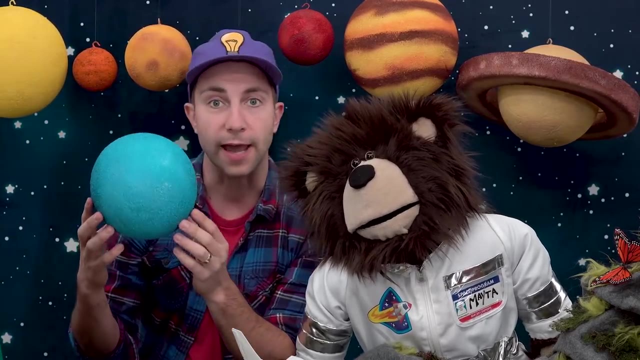 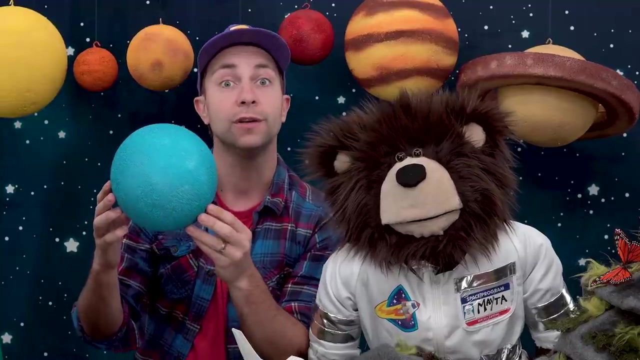 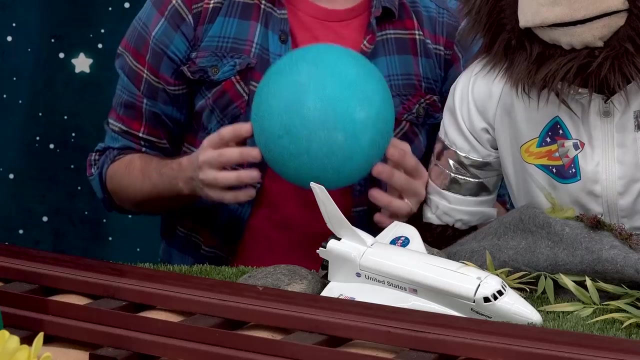 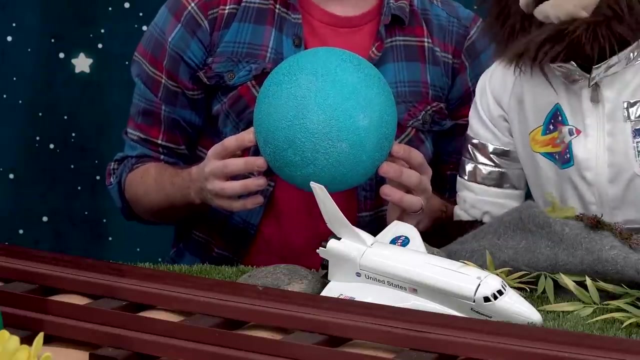 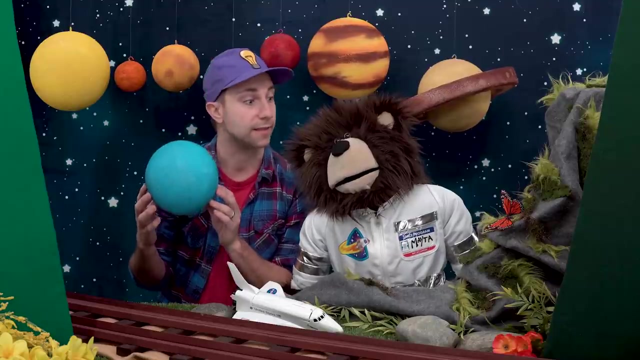 Wow, mate, Look at this blue planet. This planet is called Uranus. Uranus is the seventh planet from the Sun. Did you know that this planet orbits at an angle lying on its side And it's blue, not because it's made of water, but because of the gases that make it blue? Wow, mate, Let's. 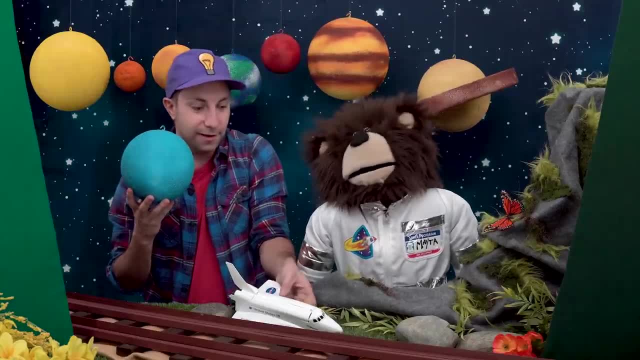 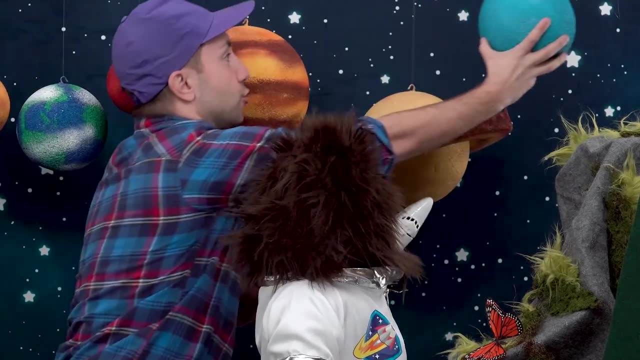 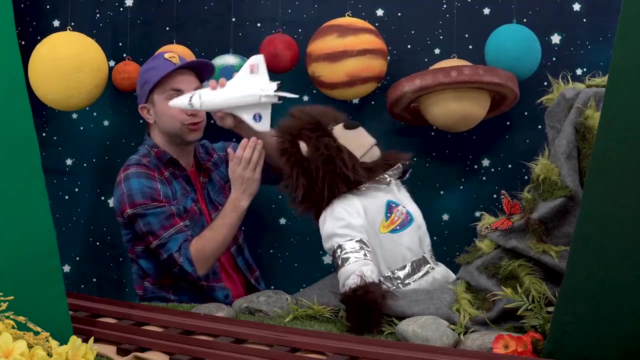 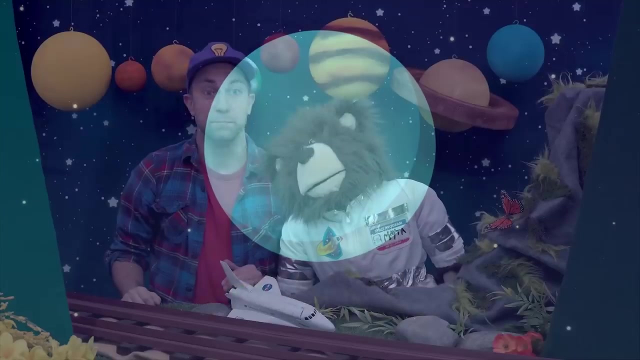 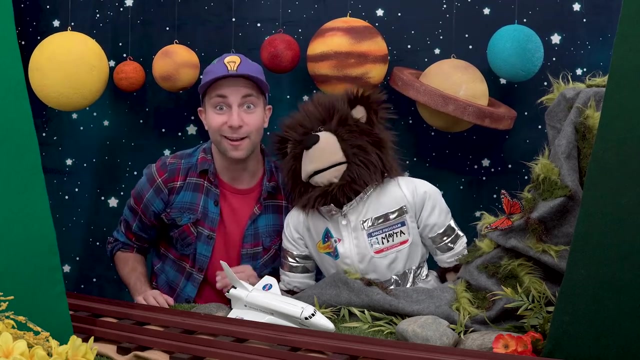 shoot this planet back up into space. Here we go. Whoa, We did it, Meta. Uranus is back in space. Uranus, Meta, are you ready for the last planet in our solar system? You are, Are you ready? 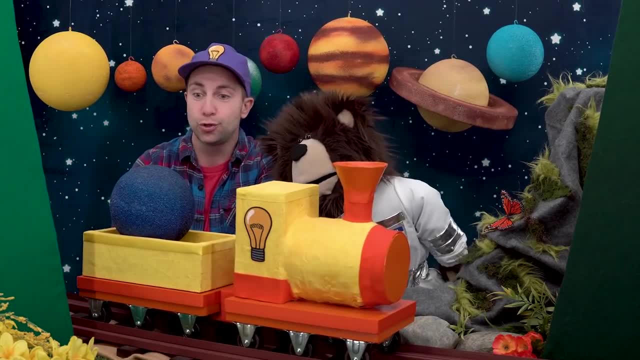 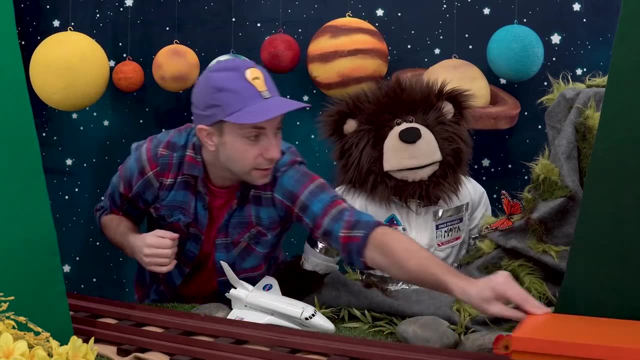 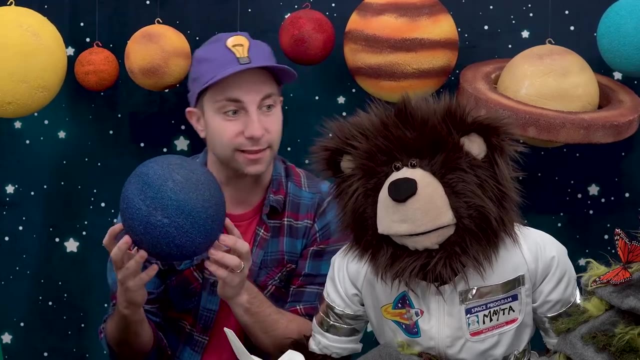 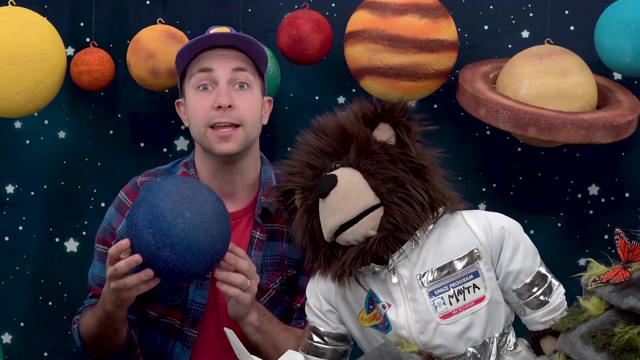 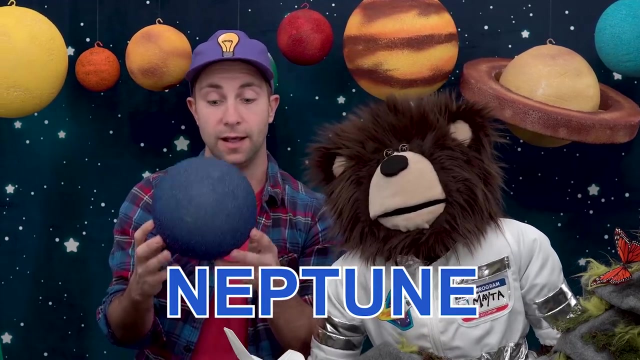 Okay, Shhh, Thank you, Idea Train. Wow, Look at this planet, Meta. This planet is called Neptune. Neptune is the eighth planet out from the Sun, making it the farthest planet from the Sun. Wow, Wow, Wow. 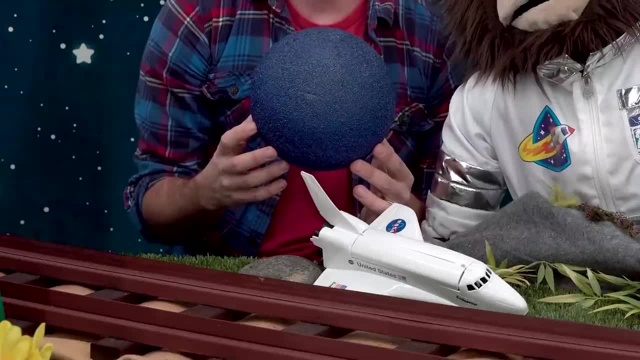 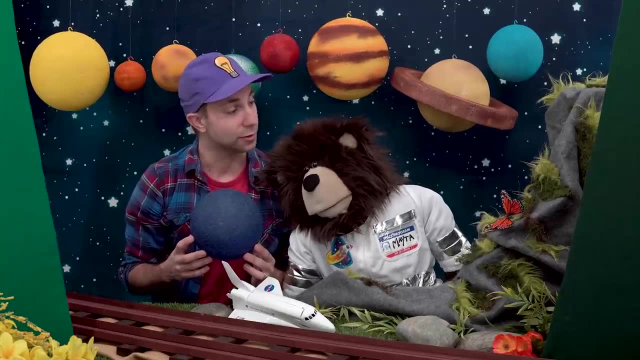 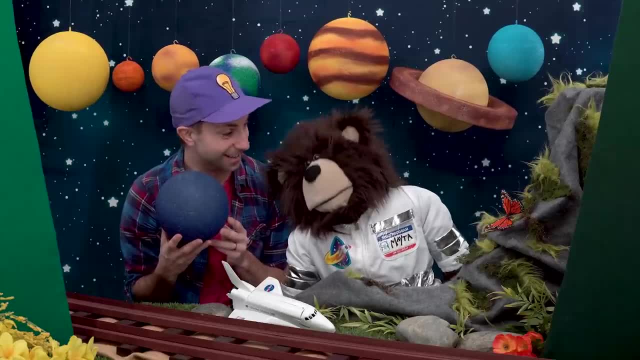 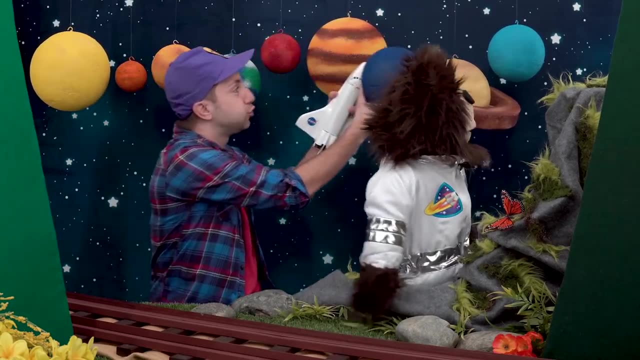 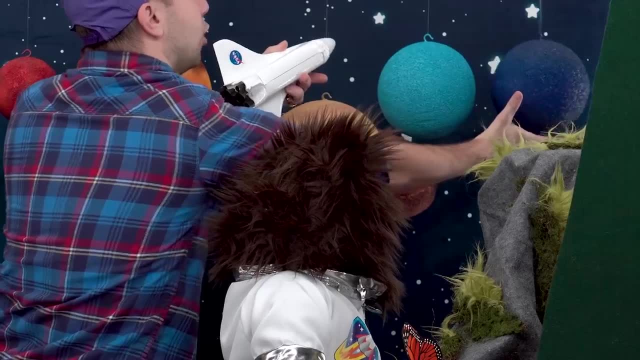 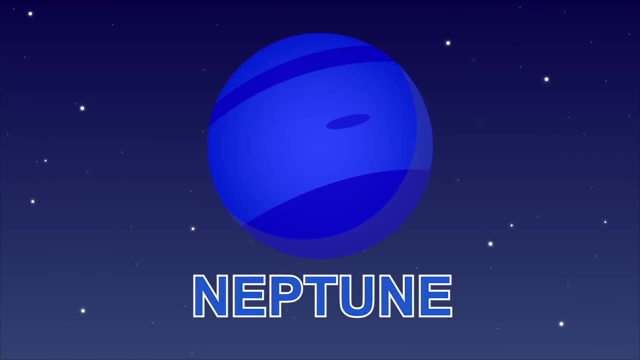 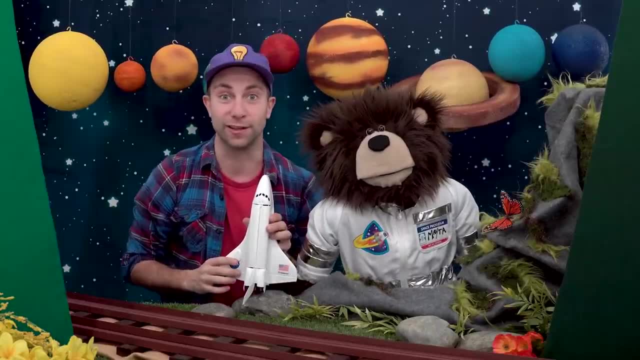 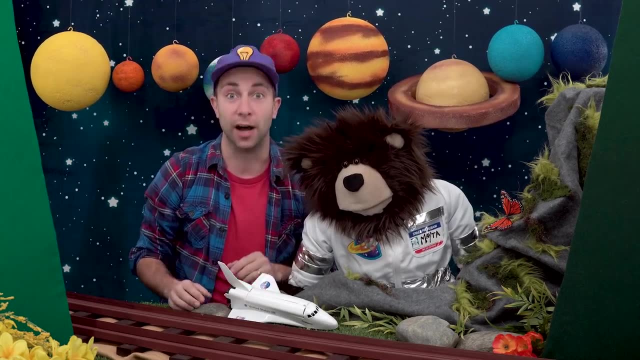 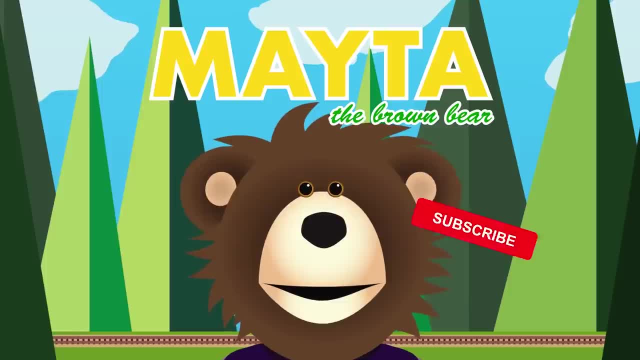 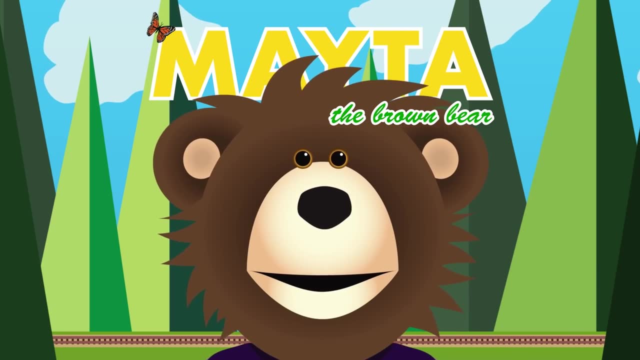 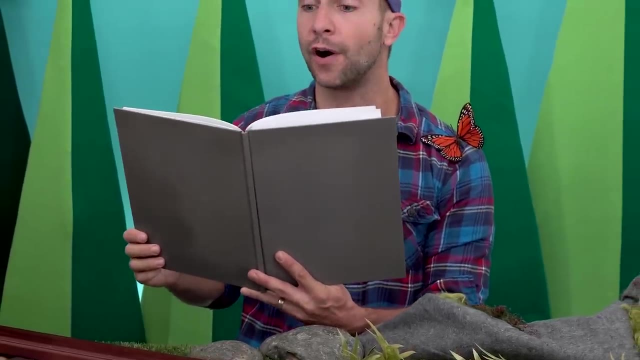 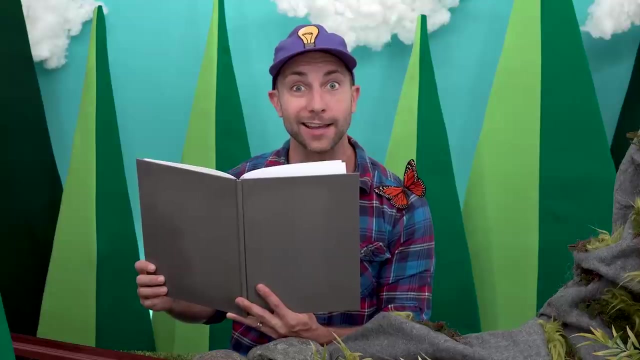 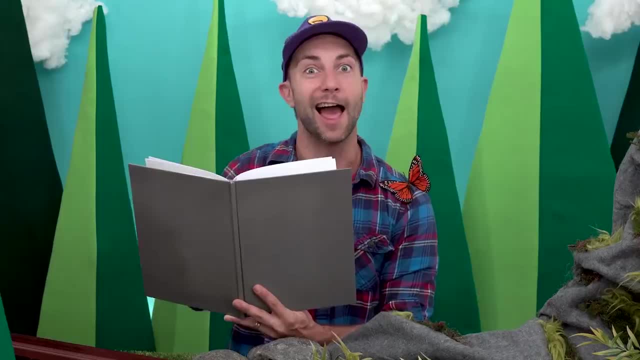 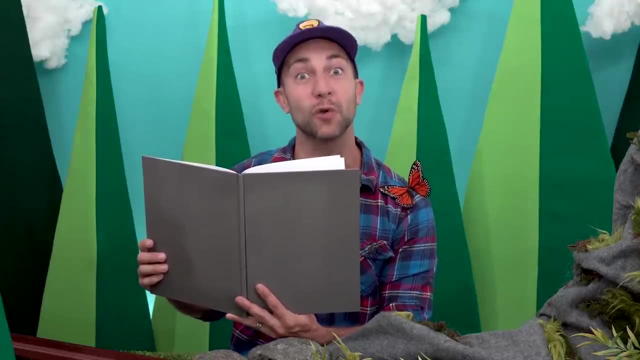 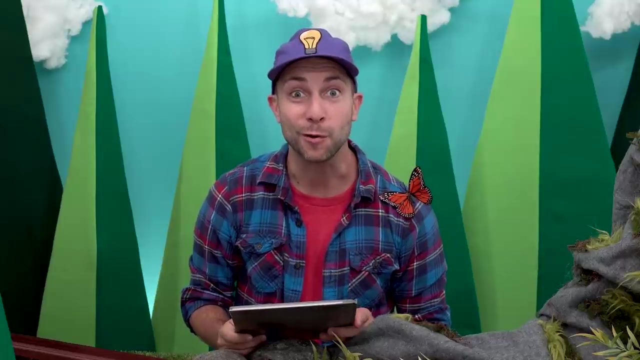 And this. this is Mr Butterfly And we're reading a book. Do you know what color book this is? That's right, it's gray. Well, we are waiting for our friend Meta to wake up from his nap. Do you know who Meta is? 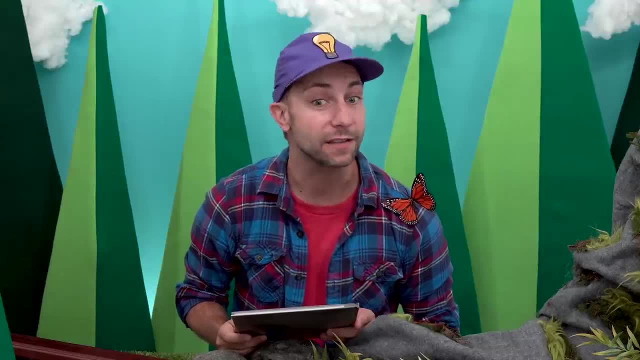 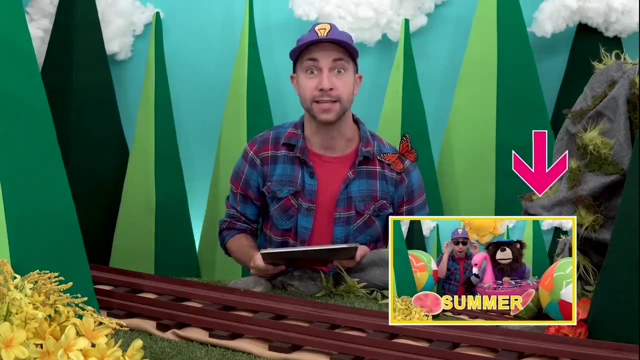 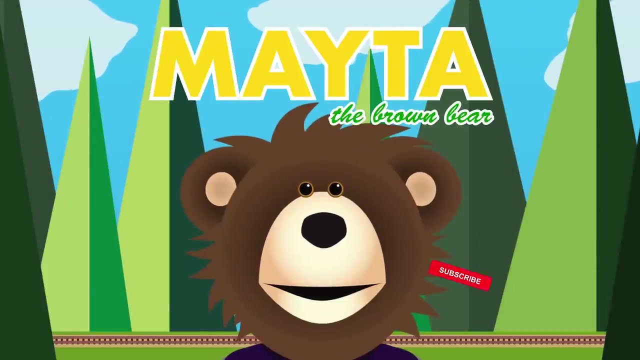 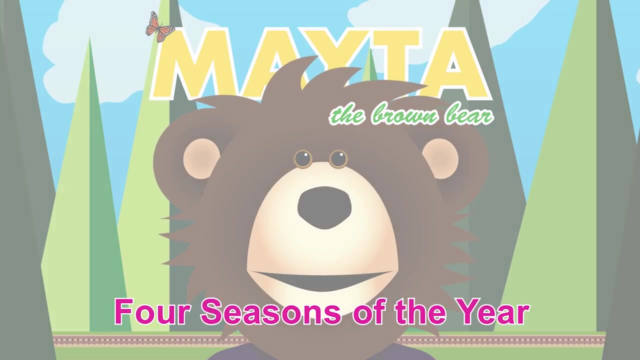 Meta is a brown bear that lives in this forest. I have an idea. Why don't we wake Meta up from his nap and together we can learn about the four seasons of the year? Meta, Meta, Meta, the brown bear, Meta, are you up from your nap yet? 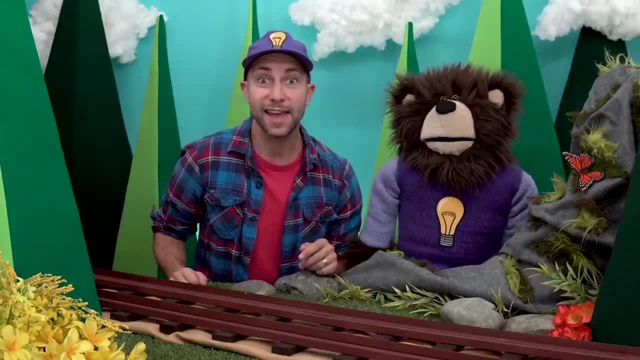 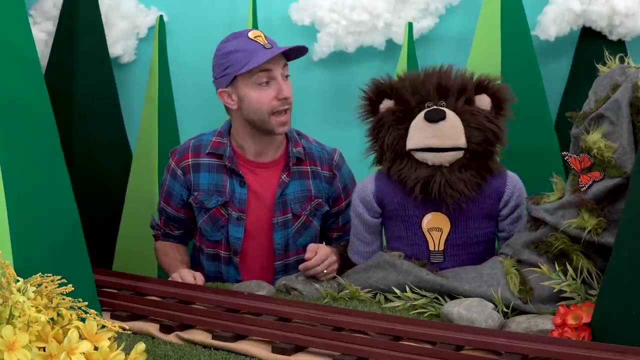 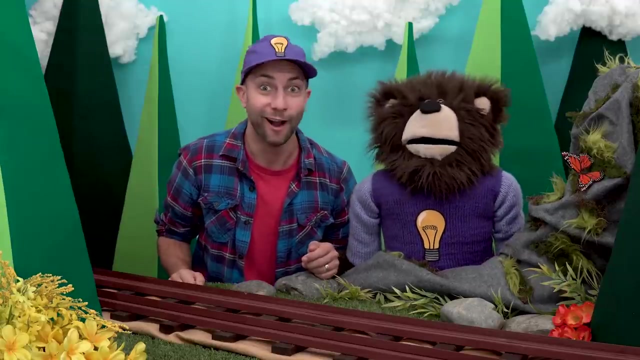 Where are you, Meta? It's Meta. Did you have a good nap? Yes, Hey, listen, we have some friends here today and together we are going to learn about the four seasons of the year. Do you want to do that? 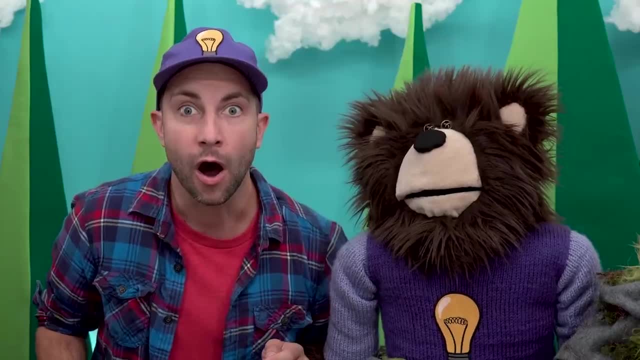 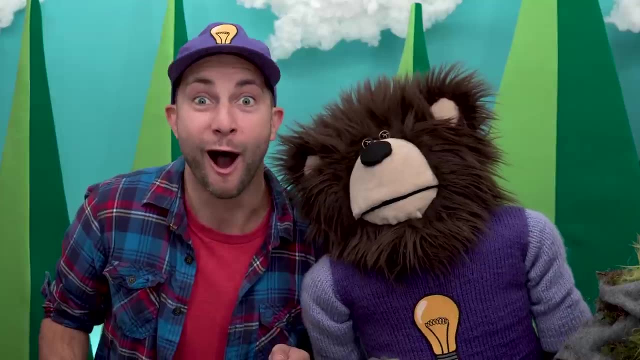 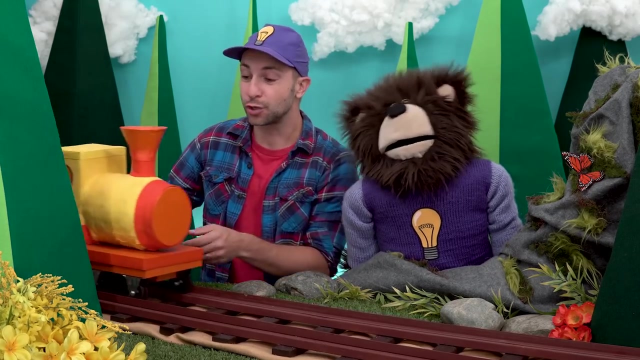 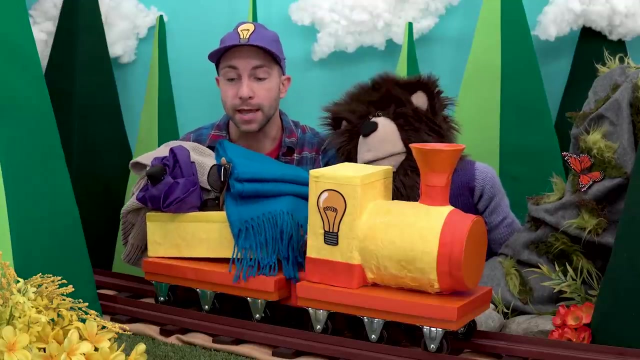 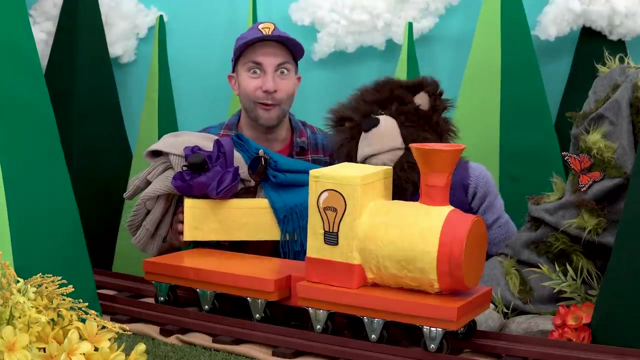 Yes, Okay, Do you hear that? No, Well, listen harder. Do you hear that? It's the idea train? Oh wow, Meta, There are four different things in this box. Oh, all right, Let's put the box over here. 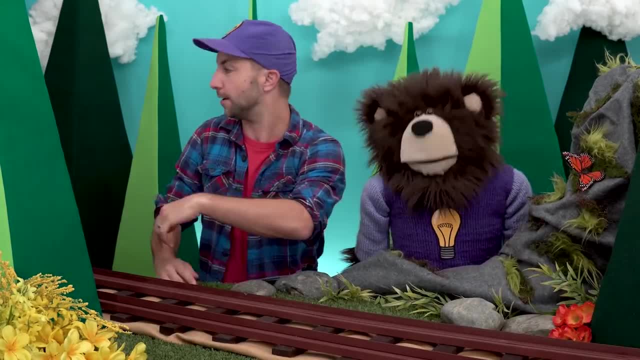 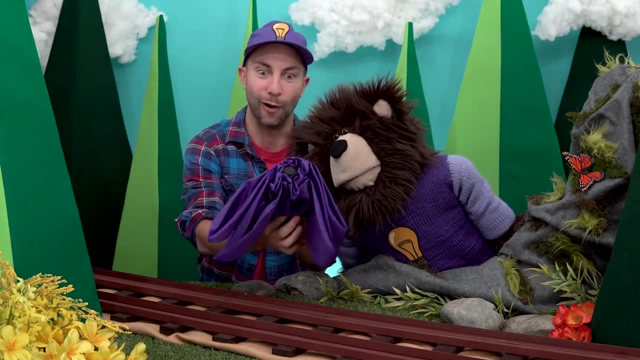 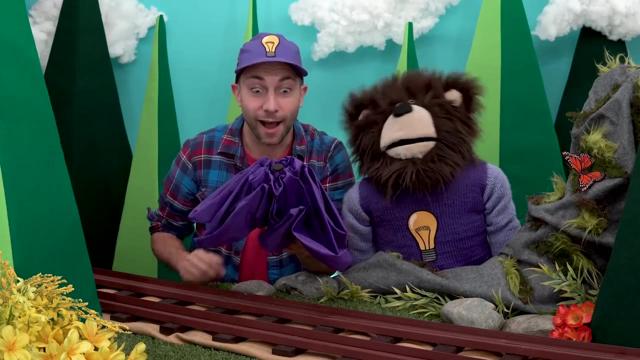 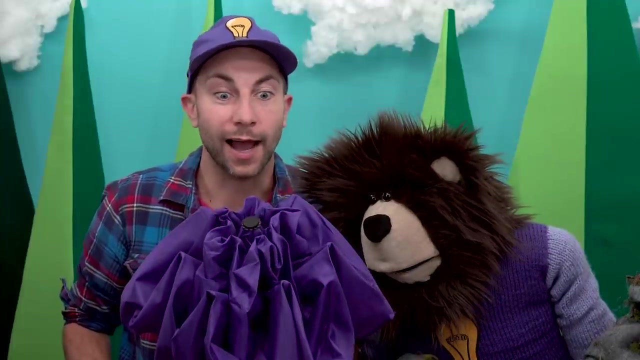 Thank you, idea train. All right, First we have. Oh, do you know what this is? That's right, It's an umbrella. Oh wow, Meta. when I open this umbrella, I wonder what season it will be. 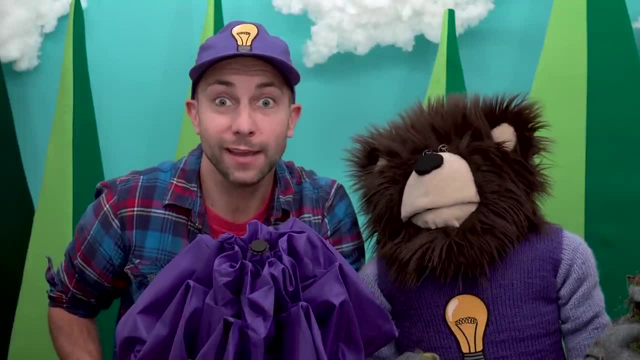 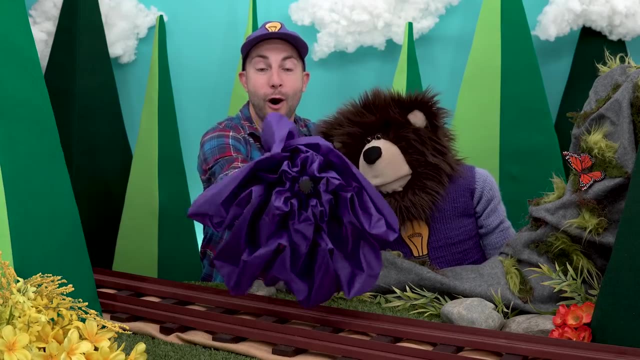 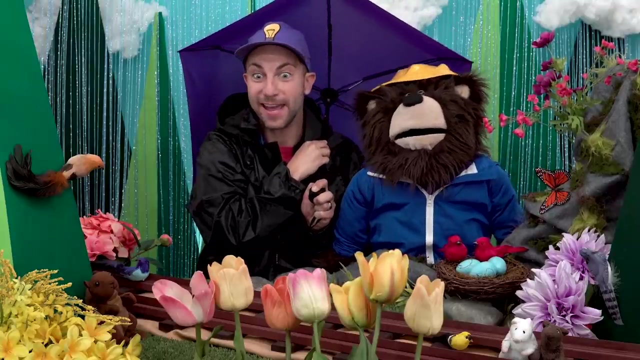 Oh, do you want to see what season it will be? You do, You do? Okay, let's open the umbrella. Oh, oh, oh, oh. Wow, Meta, You are wearing a rain jacket And a rain hat. 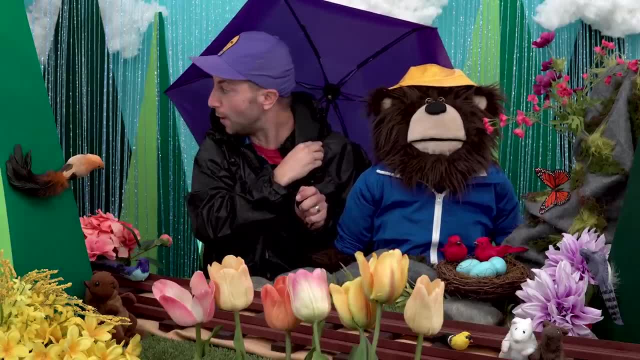 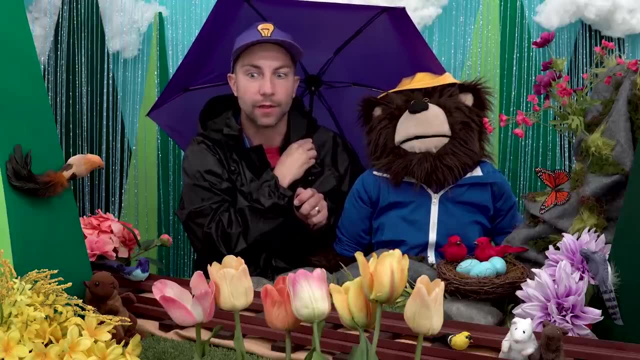 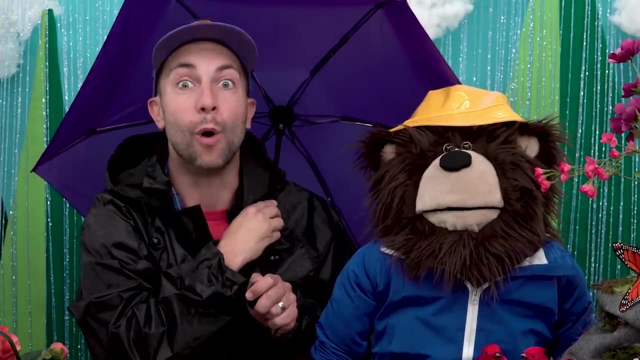 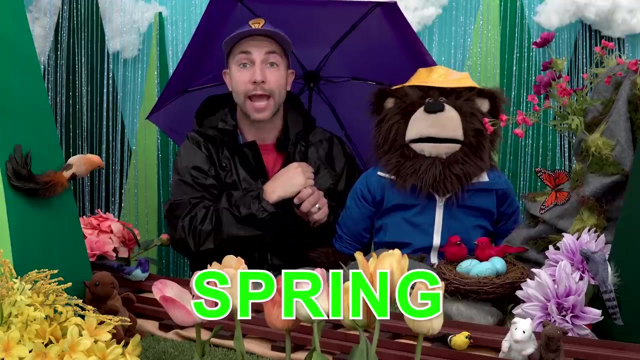 Oh, and look at all the rain falling from the sky. Wow, Oh and Meta, look, the plants and flowers are growing. Do you know what season this is? Oh, that's right, It's spring. And do you know what happens in the spring? 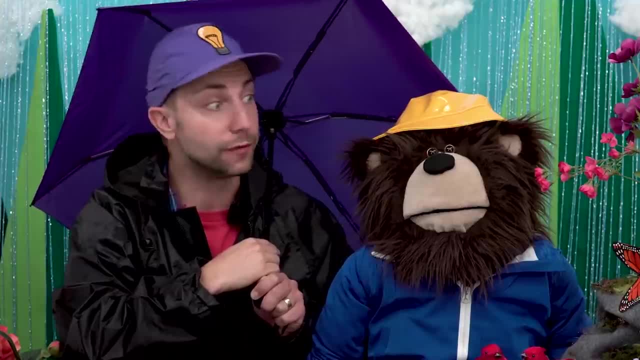 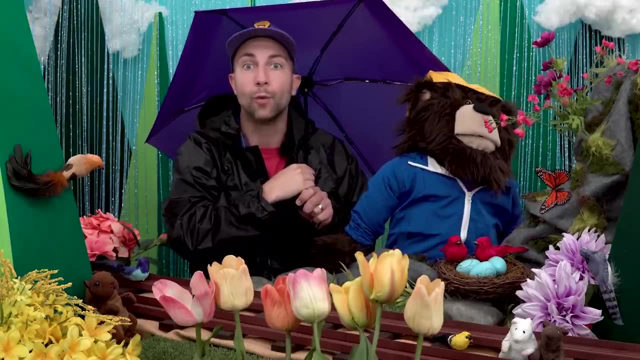 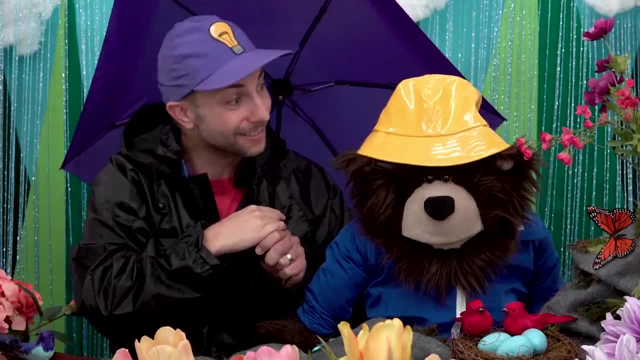 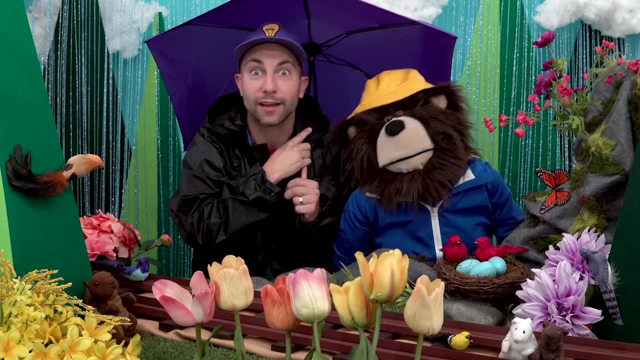 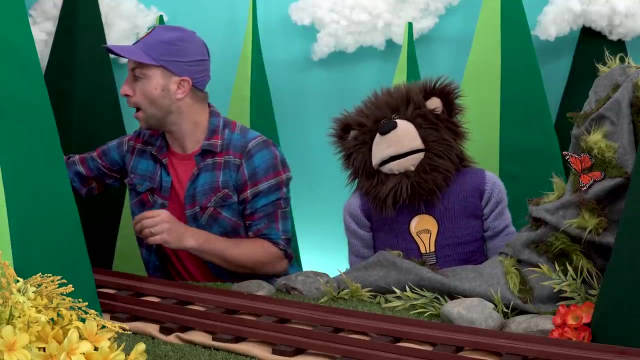 return to the warmer weather, often with little babies. Oh, look at those little red birds in their nest. This is the spring. Oh, Meta, are you ready to see what else is in the box? Yes, Okay, Let's go. 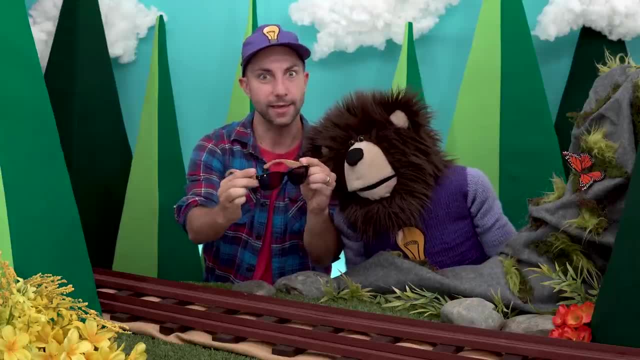 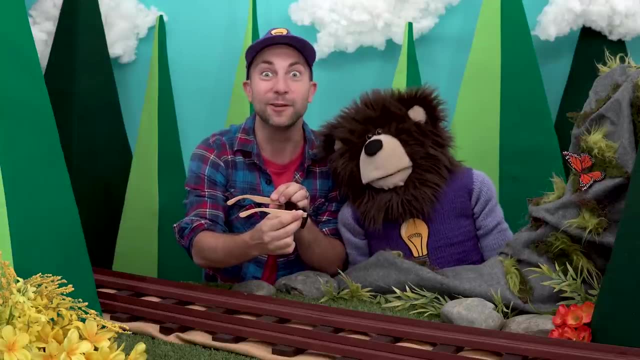 Let's go, Let's see. Oh, look at these. Hmm, Meta, do you know what these are? Mm-hmm, Do you know what these are? That's right, They're sunglasses. Hmm, I wonder, when I put these on, what season it will be. 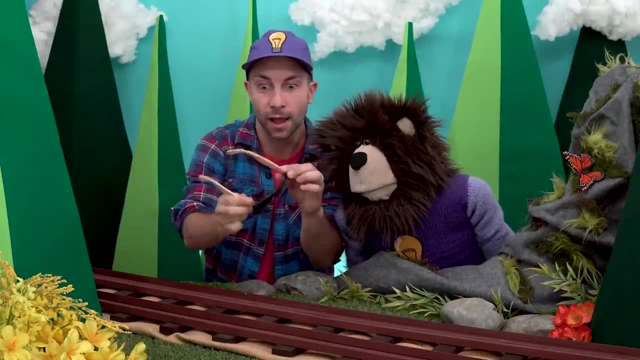 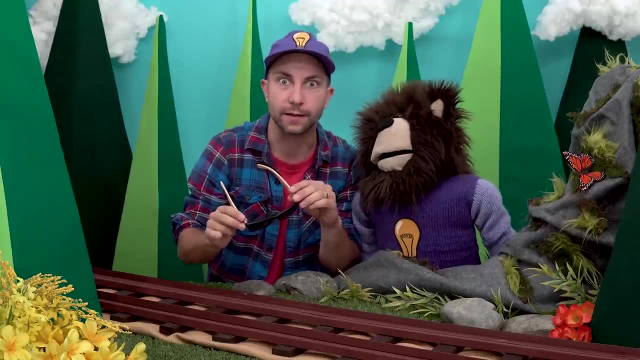 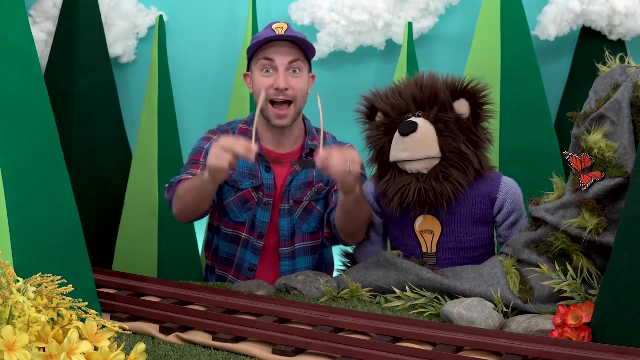 Hmm, Do you want to see what season it will be? Mm-hmm, You do? Yeah, I wonder. Oh, look at that, Look at that. Wow, Look at that. Look at this, Look at that. Okay, let's put them on. 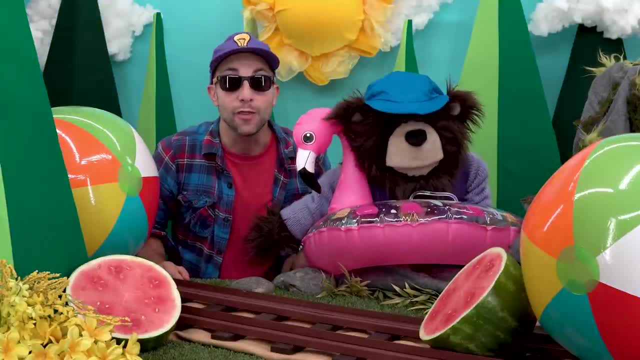 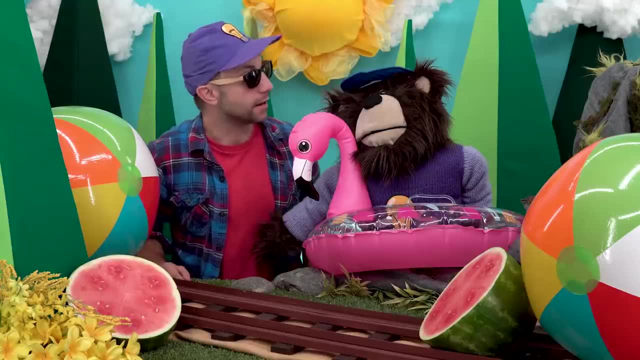 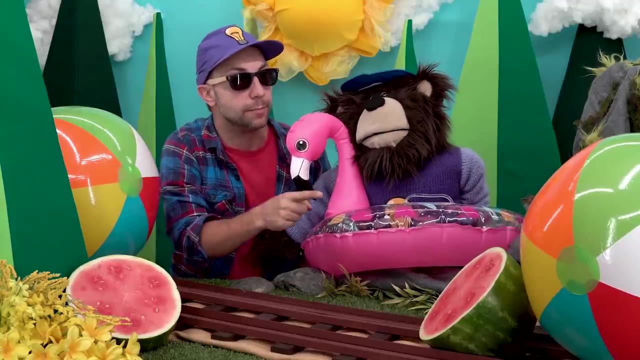 Whoa, Mayta, The sun is out. Whoa And you? You are wearing a sun hat and it looks like you're ready to go to the beach And you're flamingo floaty. Oh, Mayta, look at the beach balls and the watermelon. 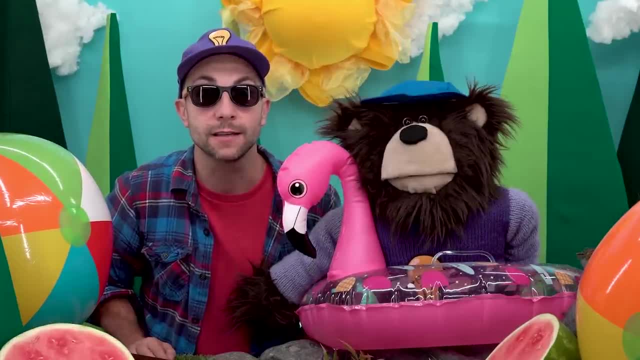 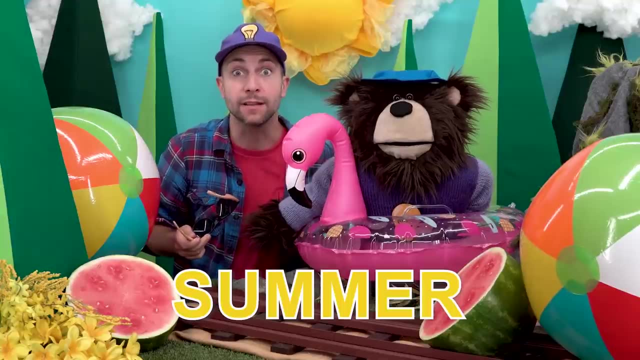 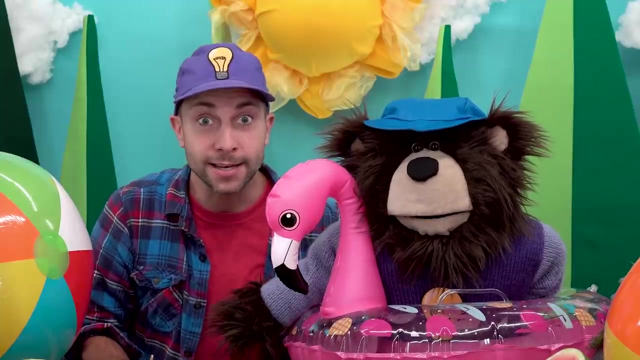 Do you know what season this is? That's right, it's summer. And do you know what happens in summer? Well, if you're in school, you're probably on summer break, And the weather is usually very, very hot, depending on where you live. 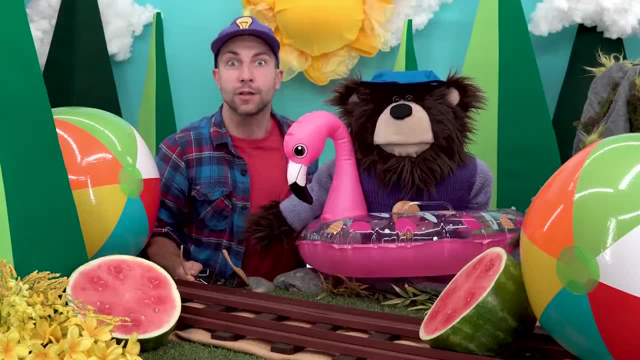 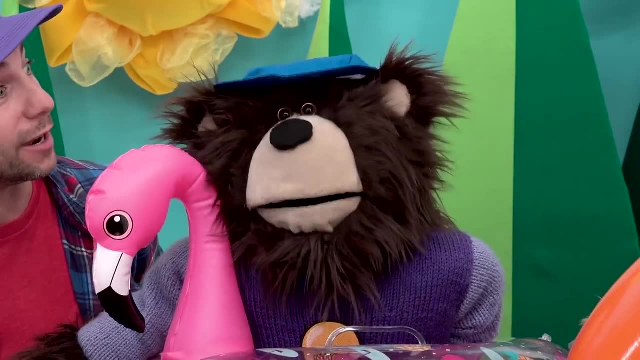 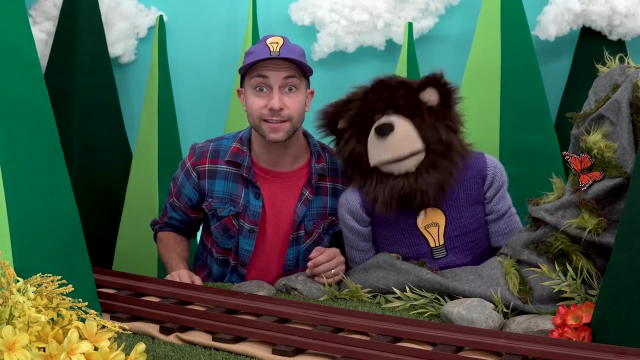 The sun is out, So it's a good idea to wear sunscreen when you're outside and maybe wear a sun hat, like Mayta's wearing. Awesome, I love the summer. Are you ready to see what else is inside the box? You are? 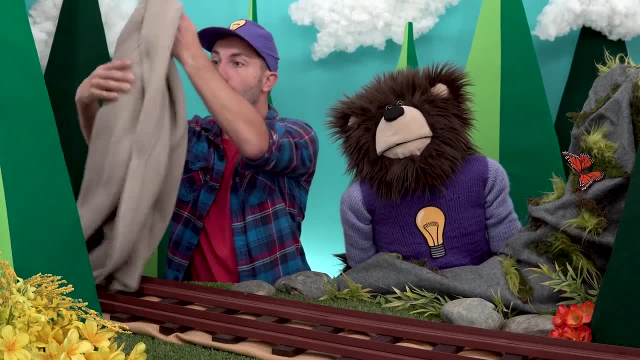 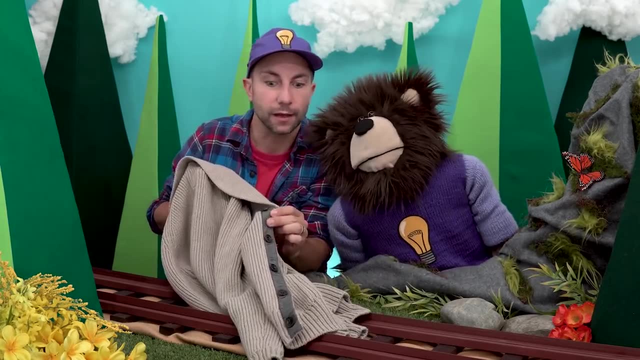 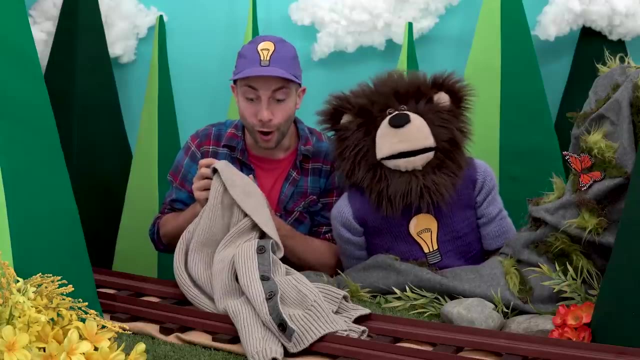 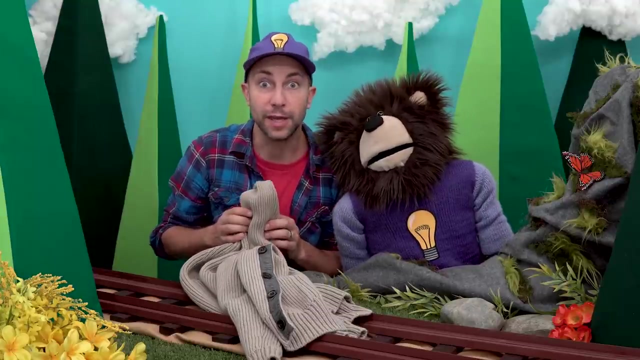 Okay, let's do it. Oh, Mayta, look, There's some buttons right here. Do you know what this is? It's a sweater. I wonder, when I put this sweater on, what season it will be. Do you want to find out what season it will be? 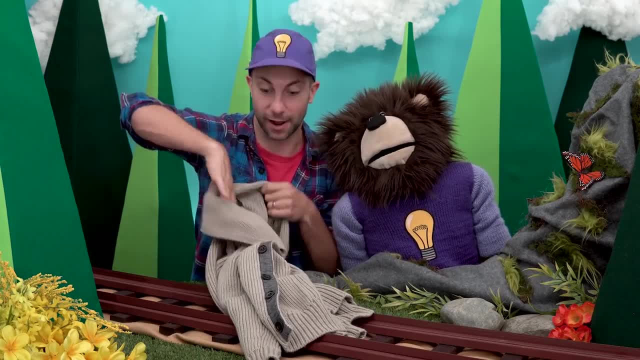 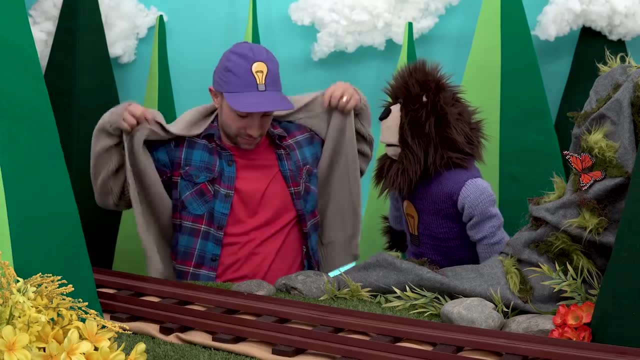 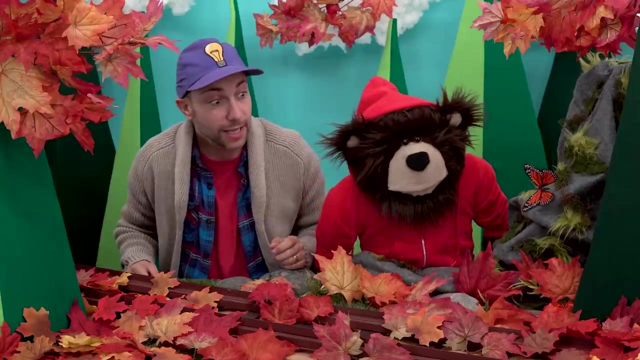 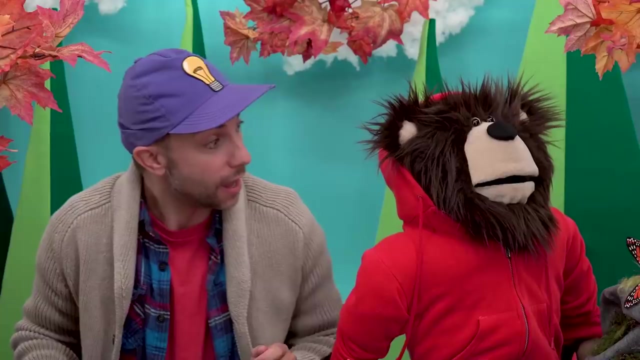 You do. Okay, let's put the sweater on. Okay, one arm in here. And Whoa, Mayta, look at all the fallen leaves. They're so colorful- Reds and yellows and oranges. And look, Mayta, you are wearing a hooded sweatshirt. 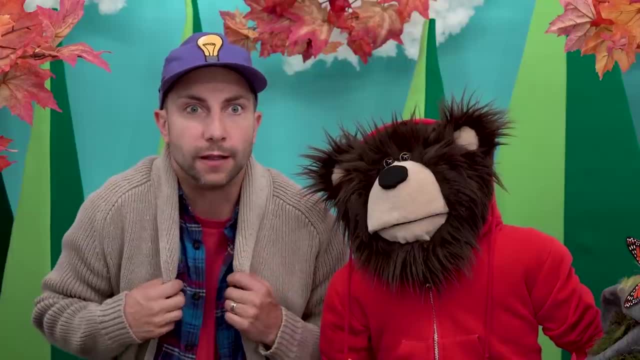 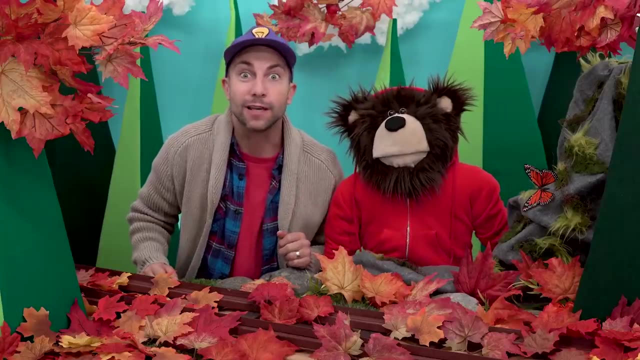 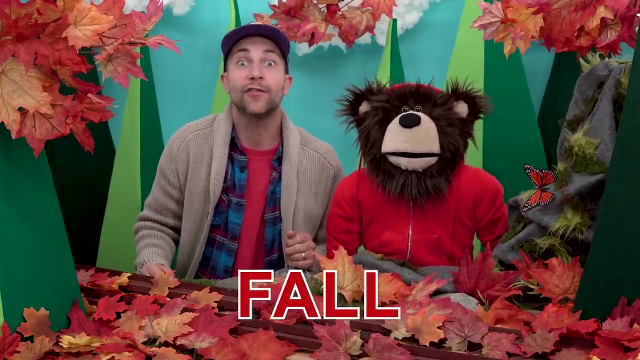 Oh, the weather is a little colder And it's a little windy. Do you know what season this is? You do, Mayta, Do you? That's right, It's fall, Or some people call it autumn. Do you know what happens in the fall? 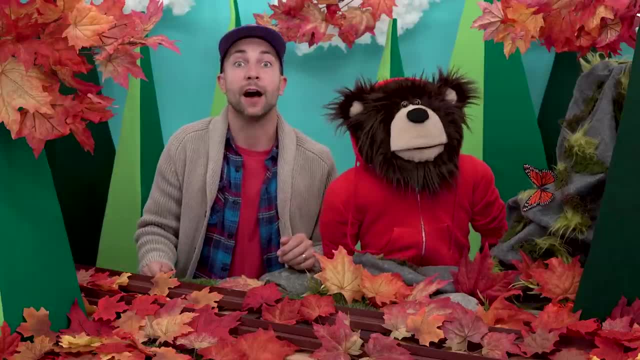 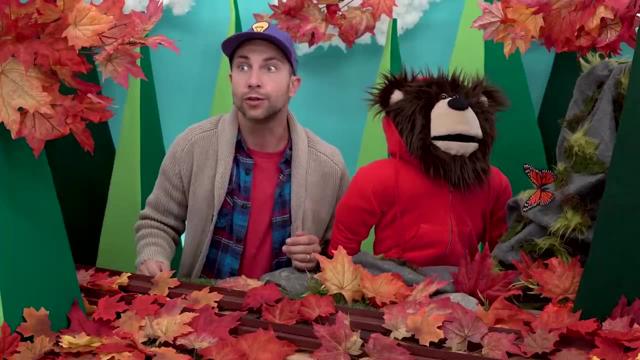 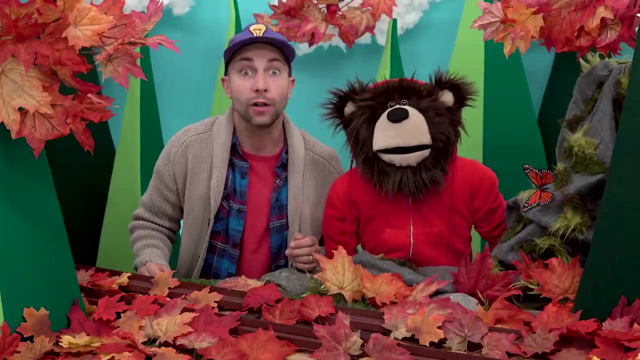 Well, the weather gets colder and all the leaves up in the trees change colors. That's right, Mayta. They turn from green to orange or red or yellow, And then the leaves fall to the ground Like this, Mayta, Wow. 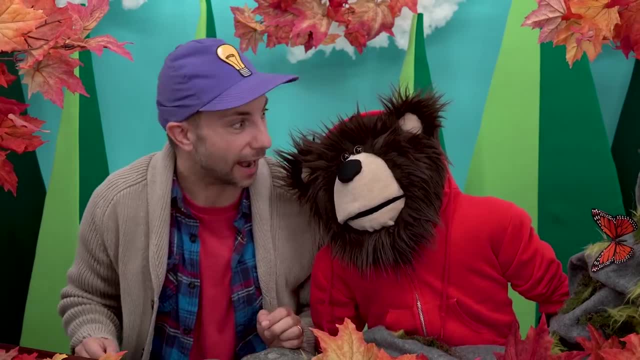 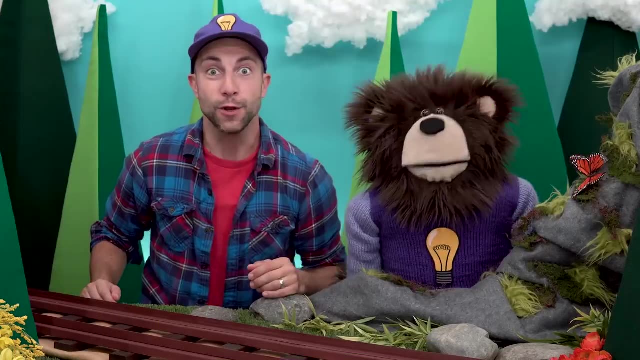 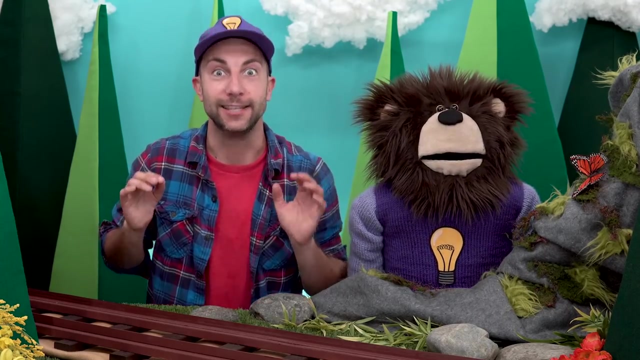 Hey Mayta, we could make a leaf pile and jump into it. The fall is fun. You know what time it is. It's time to dance. This is where we stop what we're doing. stand up and dance. You can do whatever dance move you feel like doing. 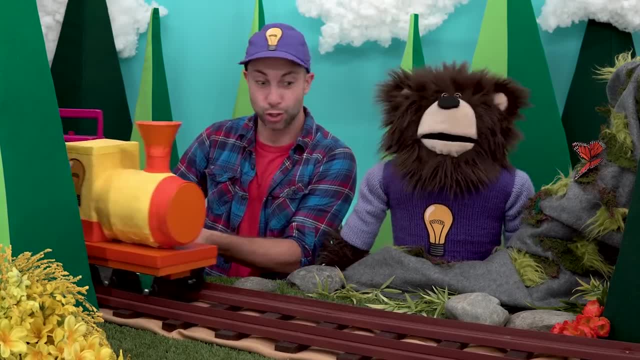 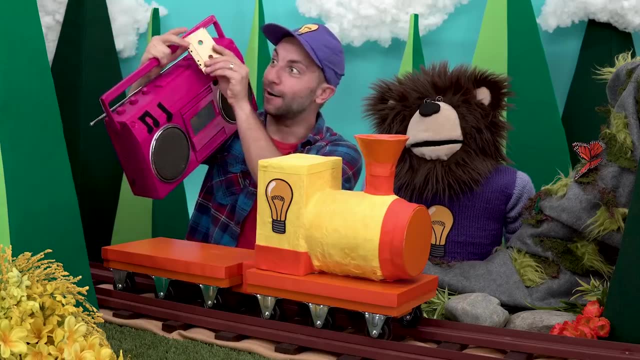 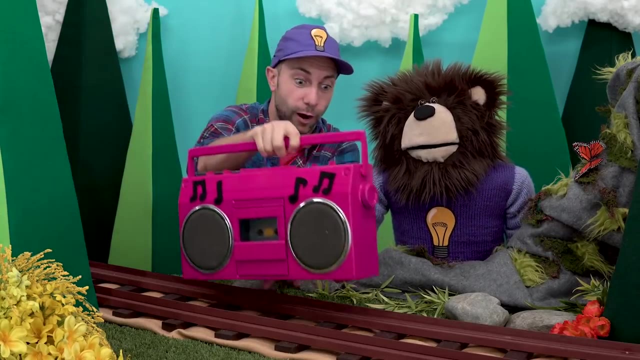 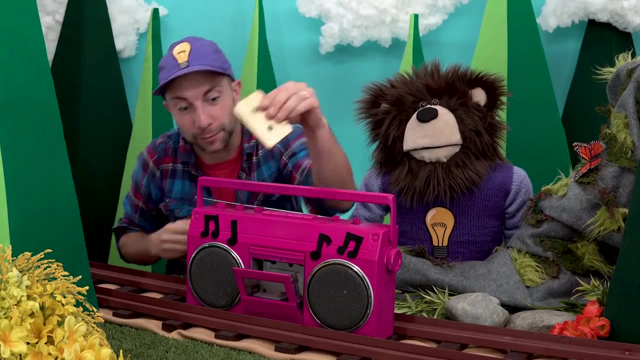 Look, It's the Idea Train. It's Pinky the Boom Box. Hi, Pinky the Boom Box. All right, See you later. Idea Train, Pinky the Boom Box plays our music. We take this golden cassette tape and put it in here. 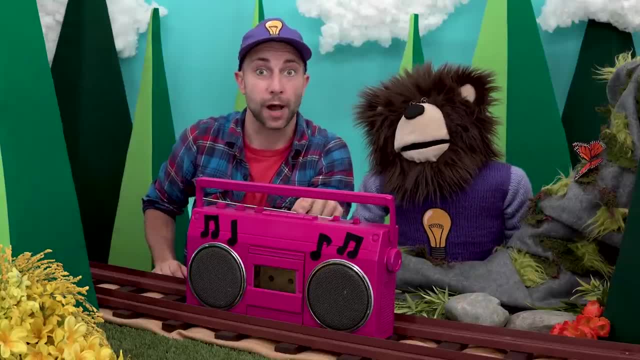 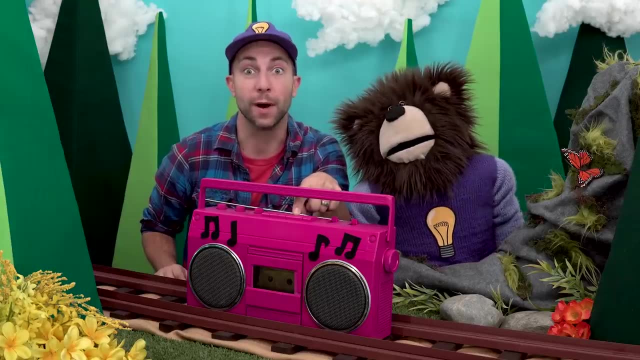 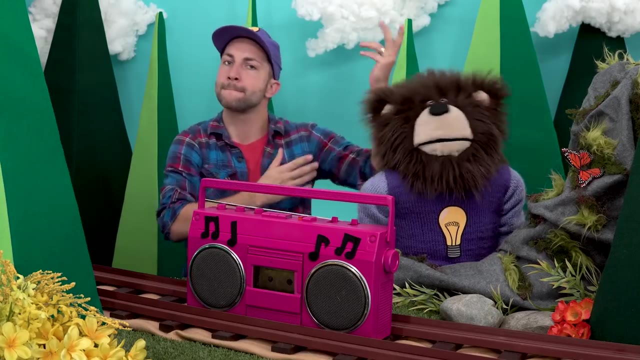 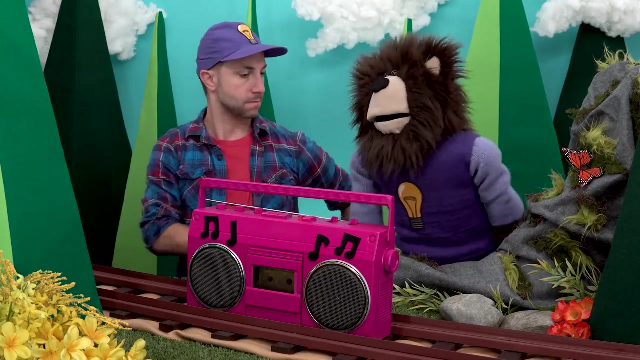 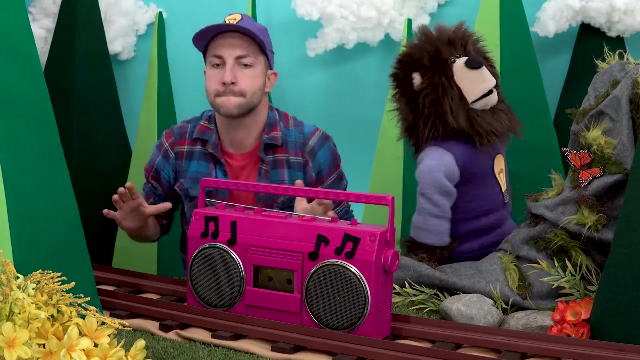 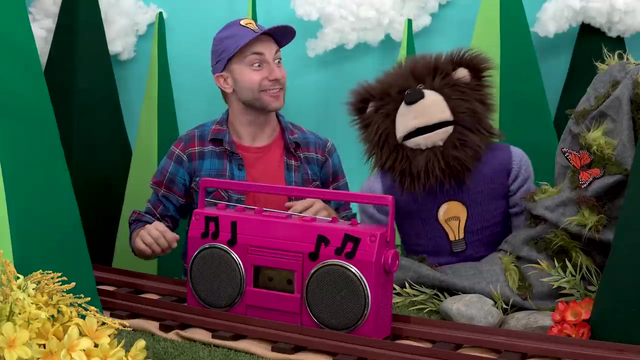 Close that up And then we push the button with the triangle on it, the play button. Are you ready to dance? Yes, I'm going to push the button now. Wow, That was a lot of fun, All right. All right, let's get back to what we were doing. 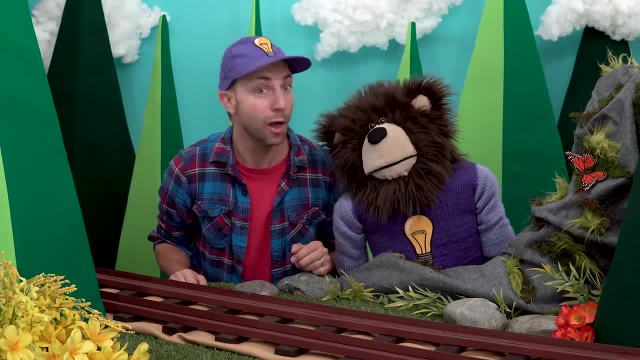 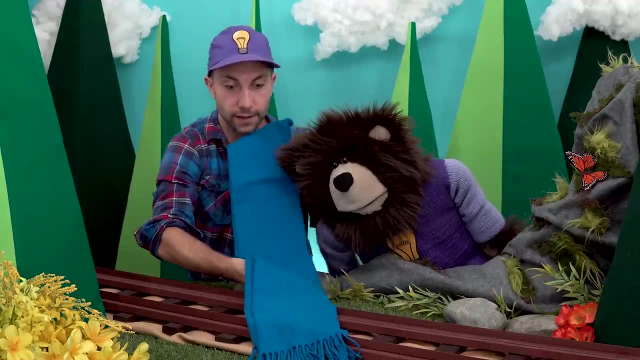 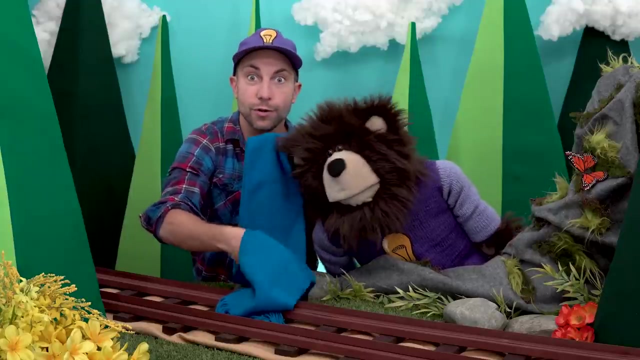 Mayta, are you ready to see what else is inside the box? Okay, Oh, look at this, Mayta. Oh, it seems very warm and soft. Do you know what this is? That's right, It's a scarf. 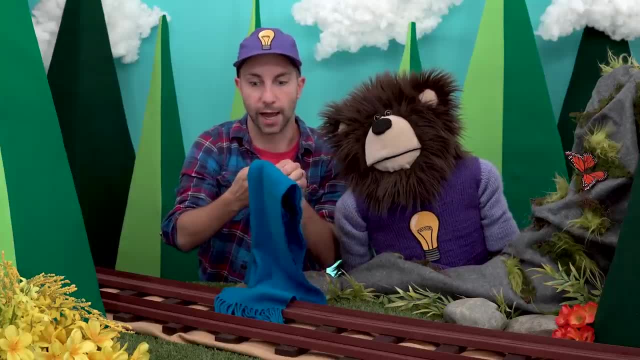 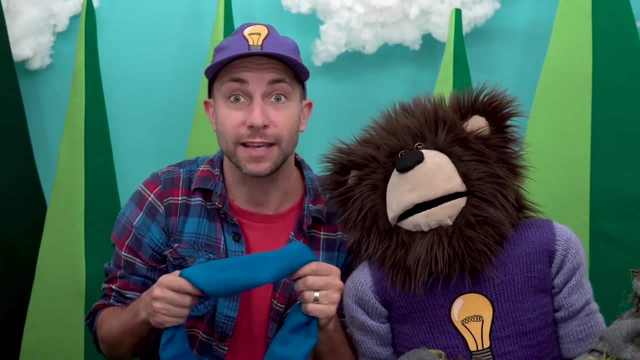 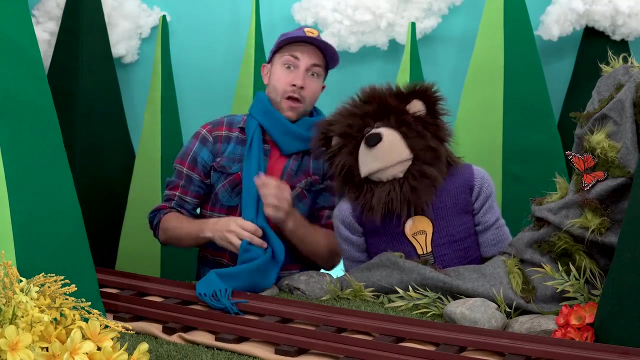 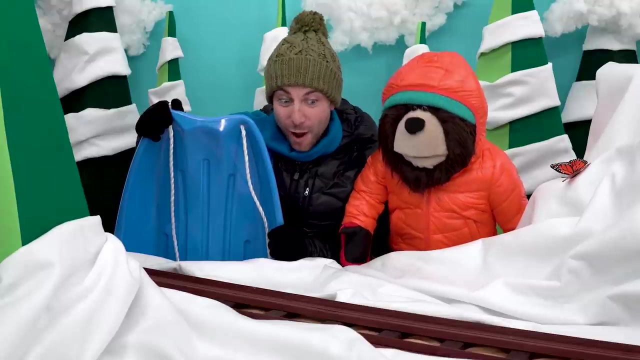 Oh, I wonder, when I put this scarf on, what season it will be. Do you want to find out what season it will be when we put this scarf on? Yes, Okay, let's find out. Whoa Mayta, look at all this snow. 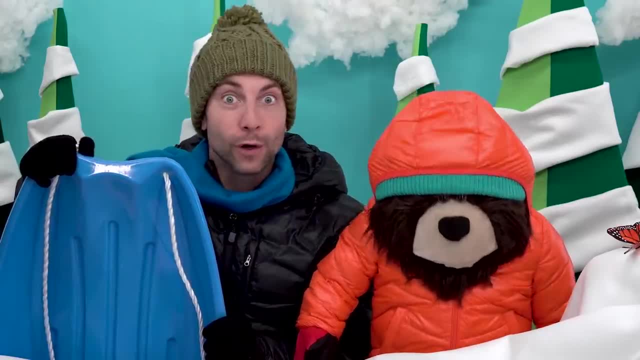 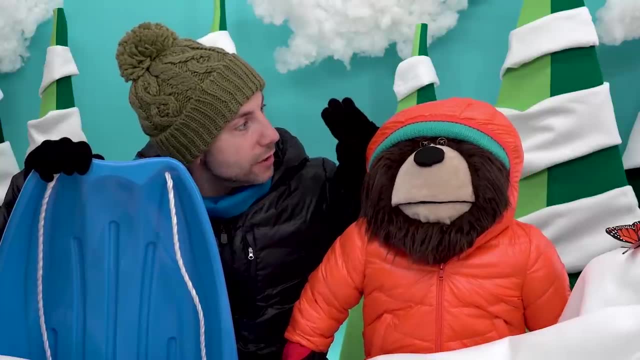 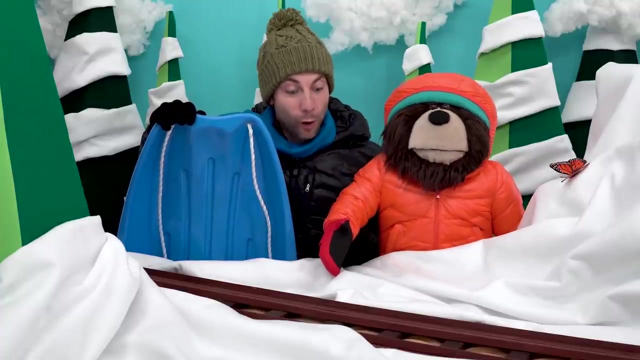 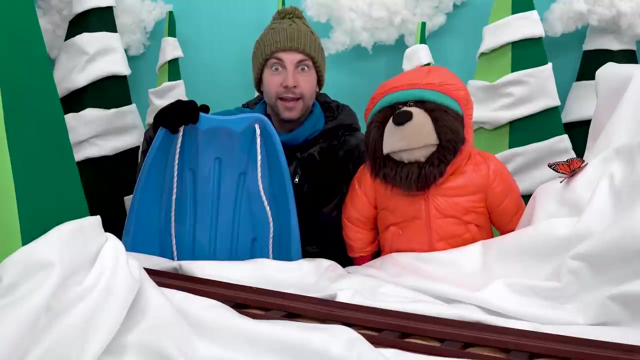 Oh, and you're wearing an orange warm coat with a hood over your head, and underneath the hood I see a warm hat and you have some red warm gloves. and look it. I'm wearing a warm jacket too, with a hat and gloves. 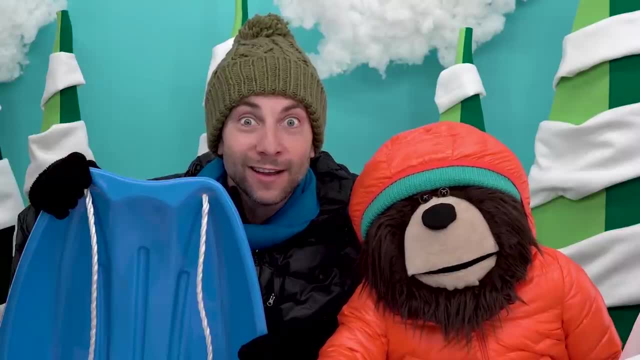 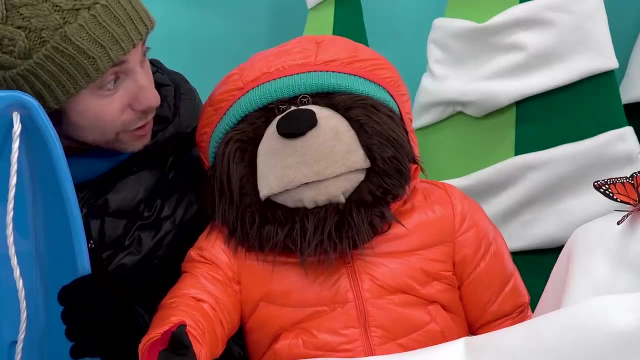 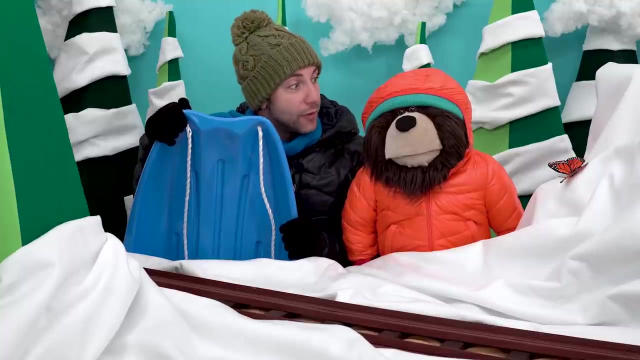 Do you know what season this is? Hmm, That's right, It's winter. Oh, Mayta, do you know what happens in the winter? Mm-hmm, Do you know what happens in the winter? Well, depending on where you live, the weather can get very, very cold, so cold that it snows. 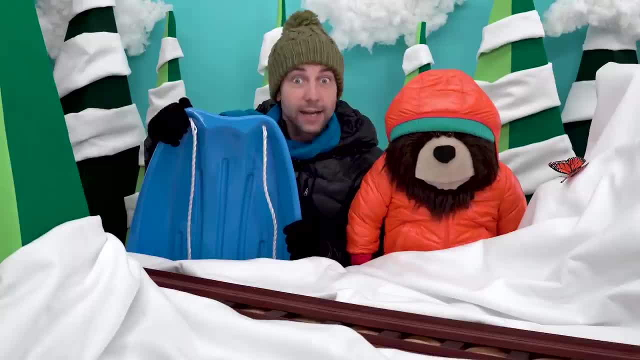 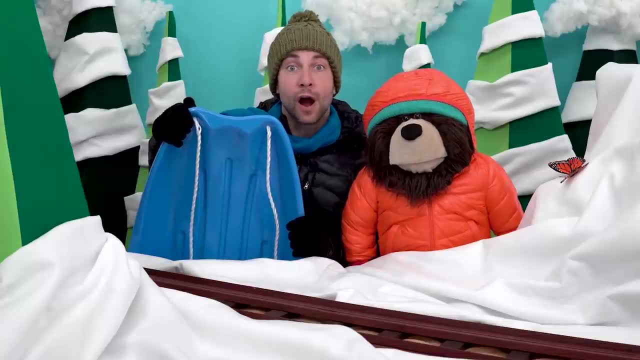 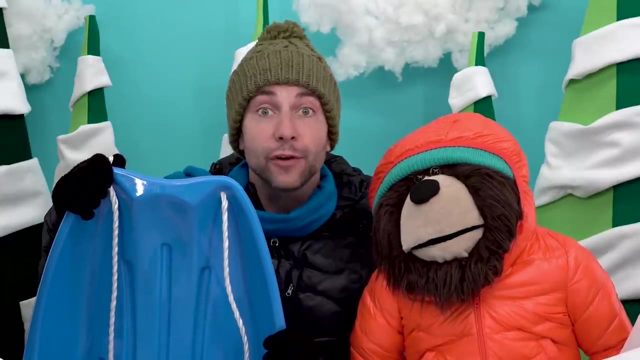 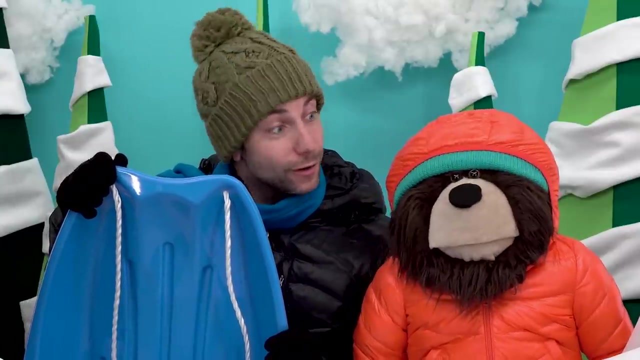 Oh, you can go outside and go sledding on a hill, or you can make a snowman and all the animals start to hibernate. Oh, do you know what that means? That means all the animals gather food and find a nice, safe, warm place to stay during the winter. and you should stay warm too if you go outside. so wear a winter hat, some gloves and a nice warm coat. 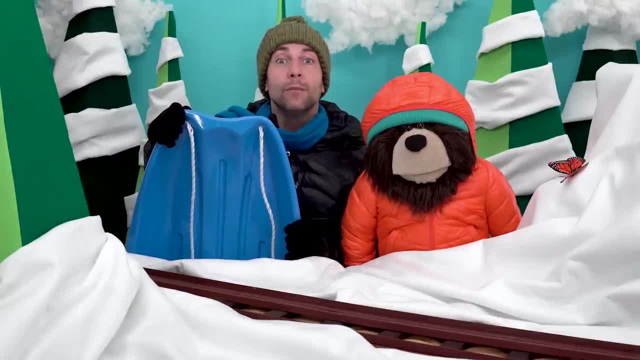 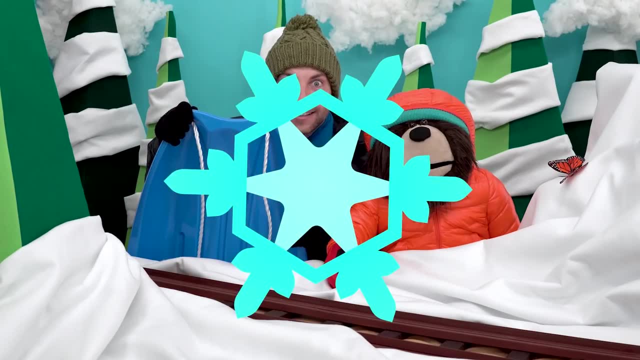 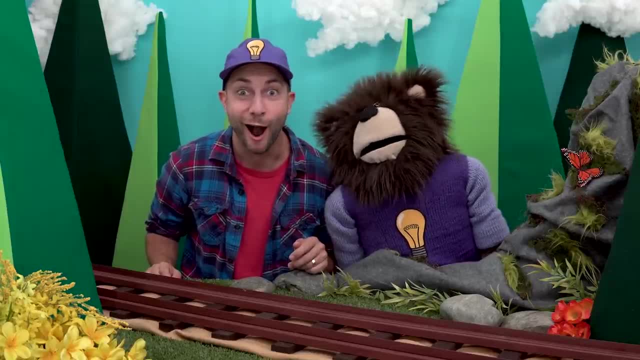 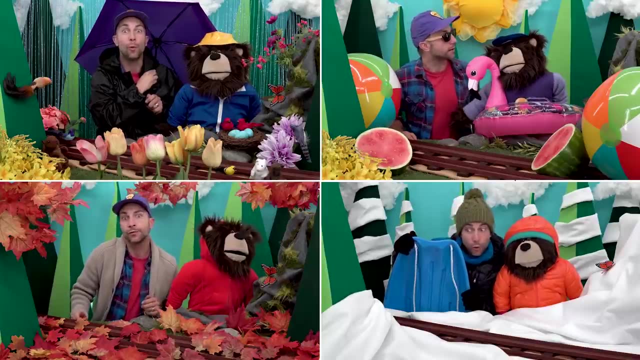 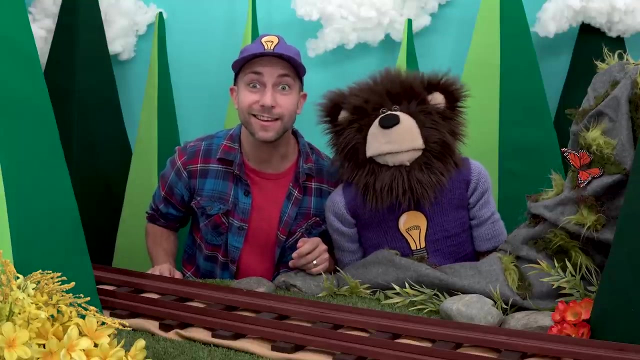 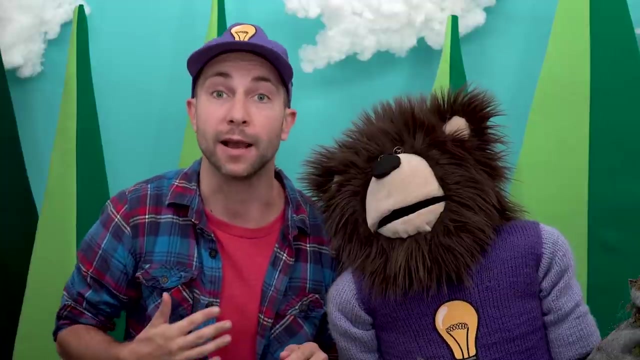 Wow, We just learned the four different seasons of the year: Spring, summer, fall and winter. Wasn't that fun, Mayta Mm-hmm, Did you have fun learning about the four different seasons? Yes, Well, thank you so much for spending your time with Mayta and myself and learning about. 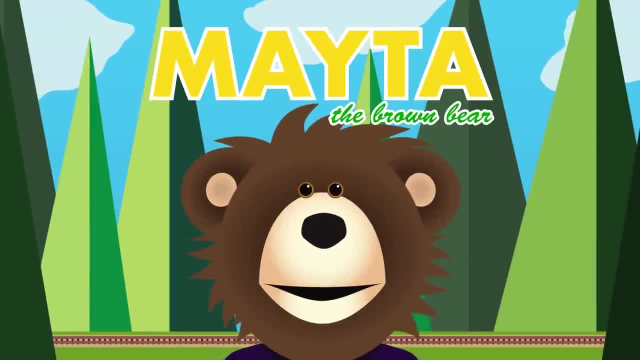 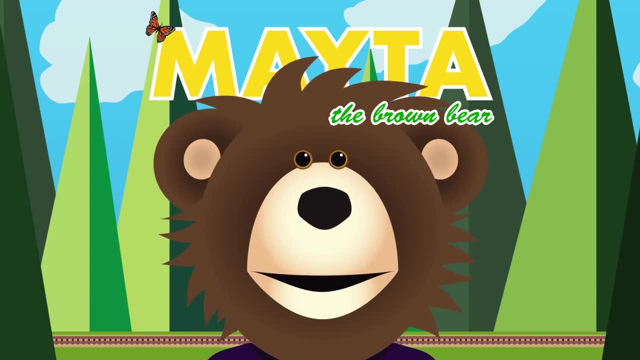 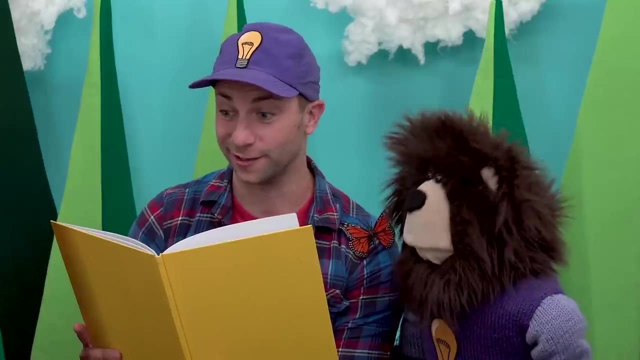 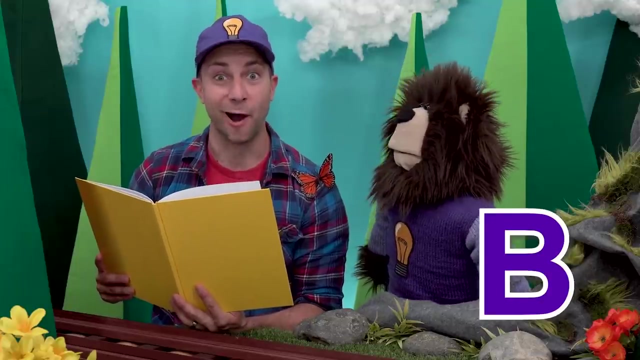 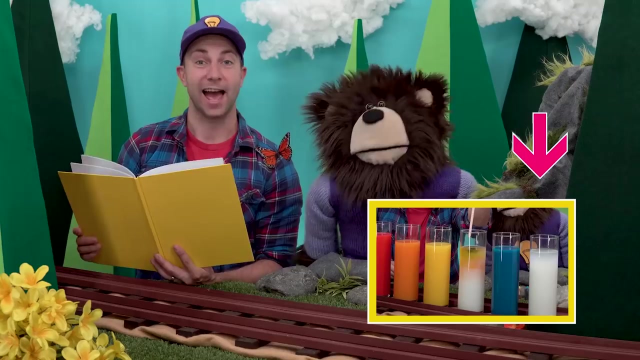 the four seasons. Adison and Everest love mixing colors to make new colors. Oh hi, my name is B, like the letter B. This is Mr Butterfly and this is Mayta the brown bear. After we are done reading our book, we are going to mix colors to make new colors. 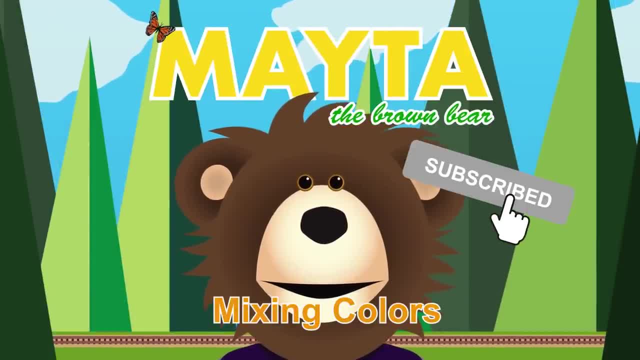 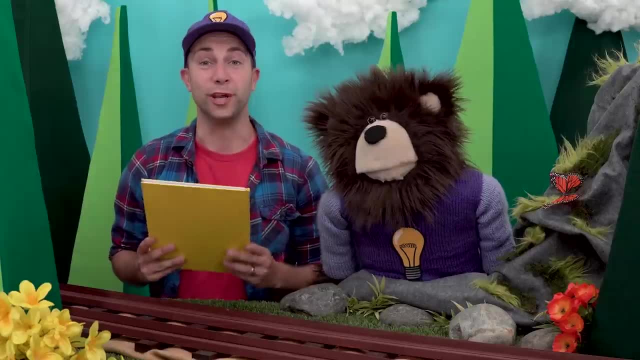 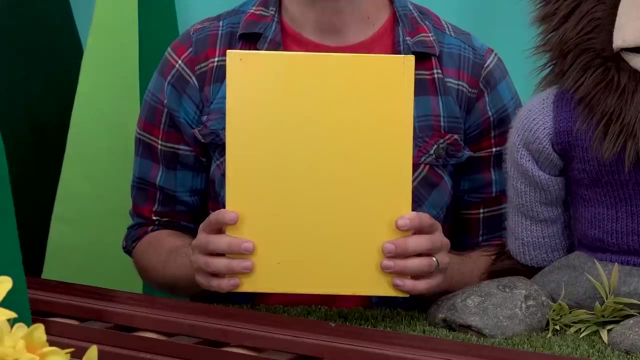 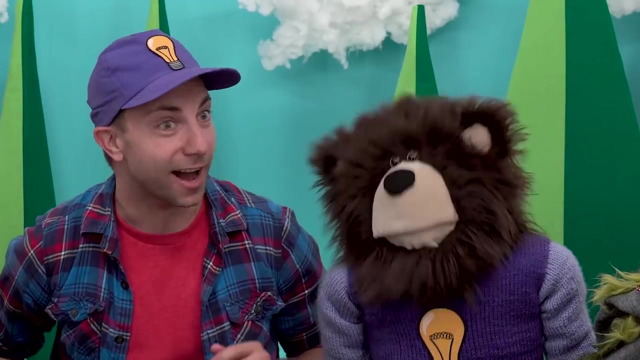 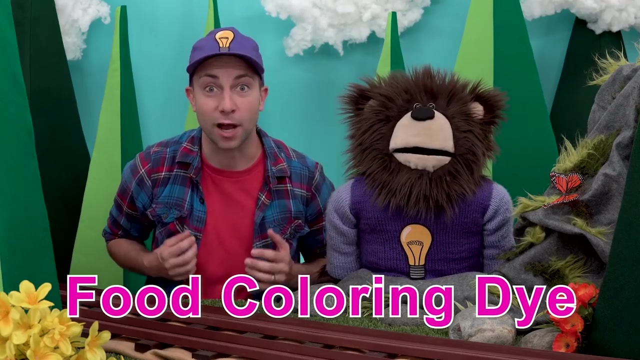 Mayta, Mayta, Mayta, the brown bear. We just finished reading our book about making colors with Addison and Everest. Do you know what color this book is? It's yellow, Mayta. I have an idea. Why don't we do an experiment using water, milk and food coloring dye to make colors? 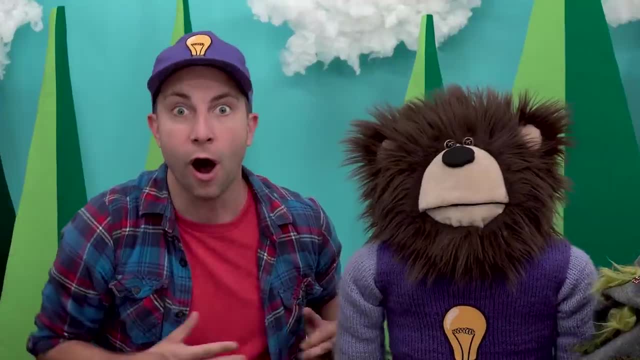 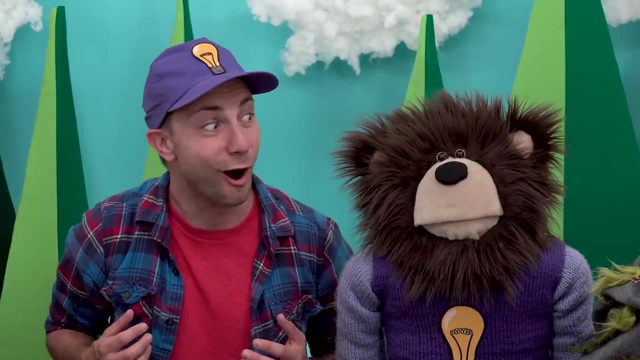 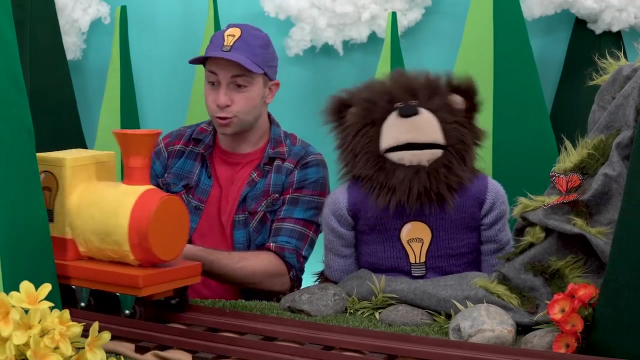 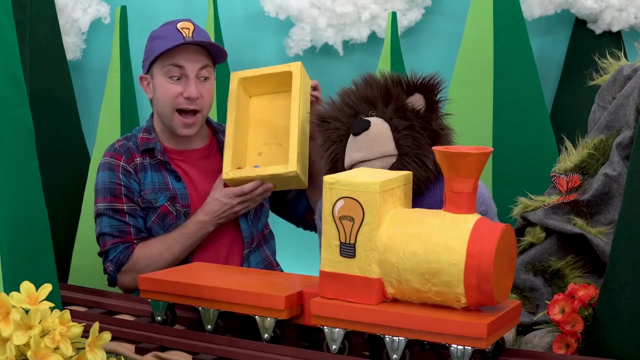 Would you like to do that? Yes, Do you hear that? No, Well, listen harder. Do you hear that? It's the Idea Train. Oh Mayta, look what's inside the box. All right, Put that right there. 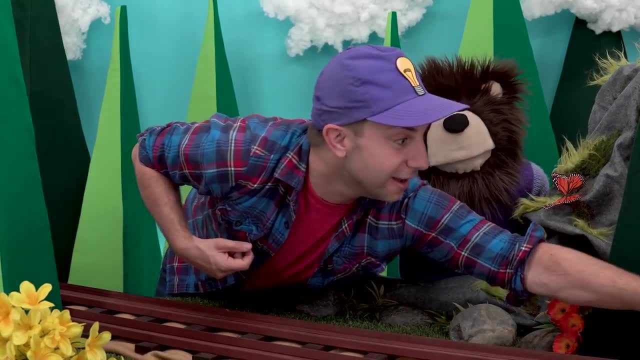 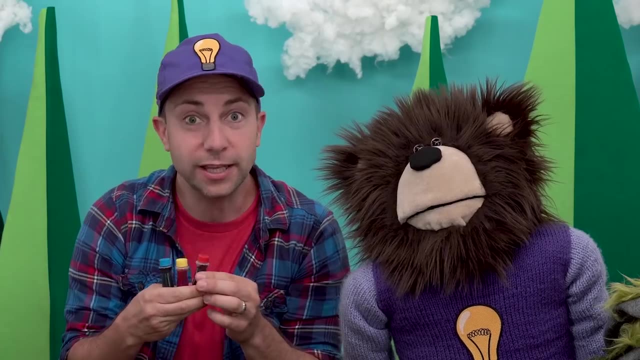 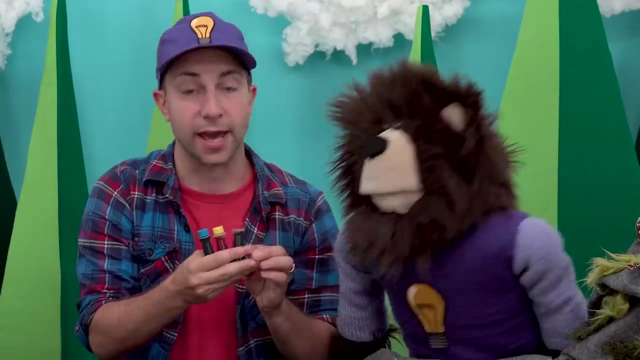 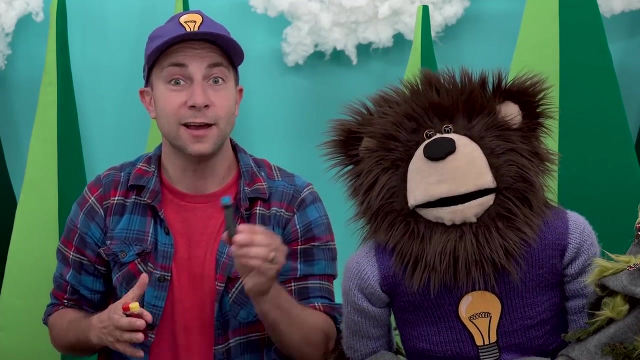 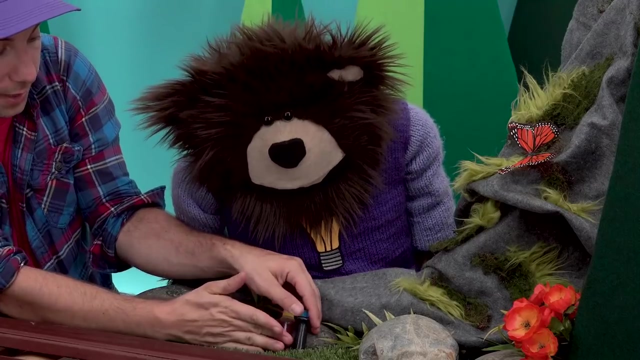 Thank you, Idea Train: Okay, Mayta, We have three little plastic containers. We have three containers filled with food coloring dye. See that We have red, yellow and blue. Okay, I'm going to put the food coloring dye right here in front of Mayta. 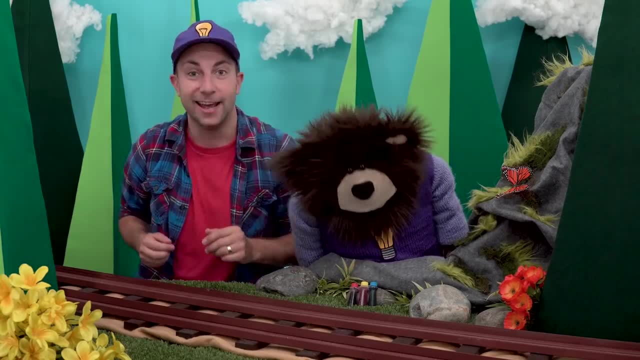 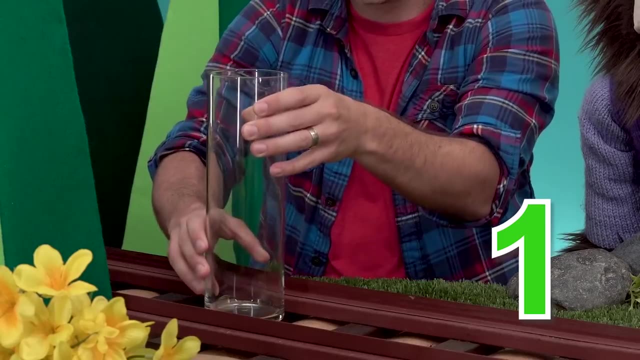 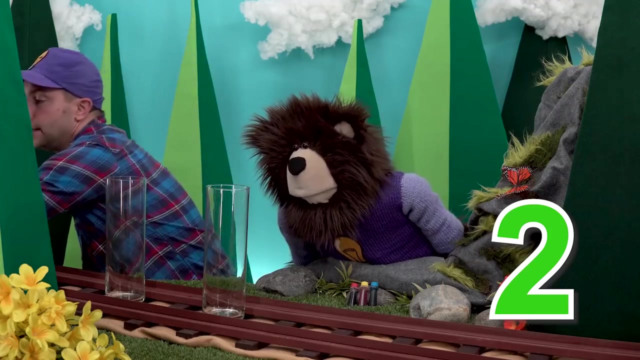 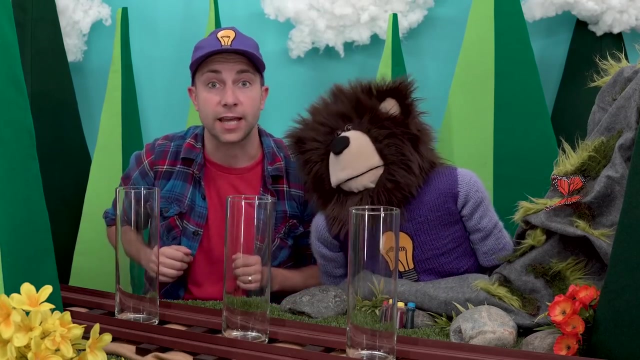 Oh, it's falling over. Wow, Okay, Mayta, over here. I have three glass containers: One, two and three. First, we are going to fill each of these containers up with water. Okay, let's do it. 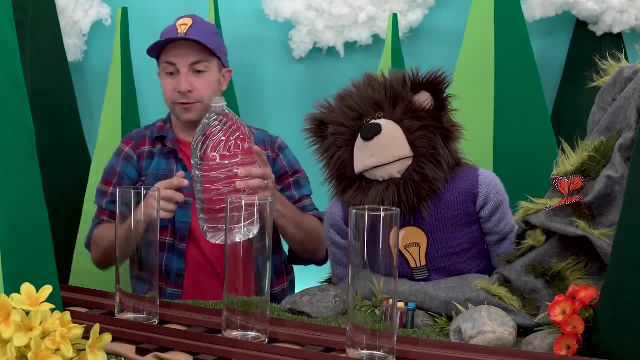 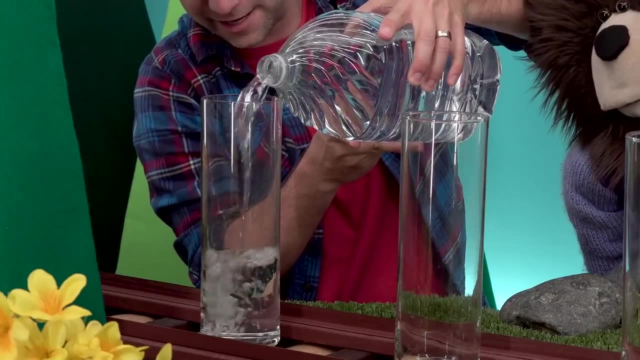 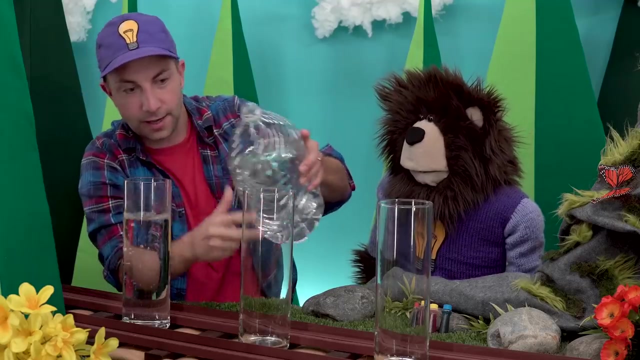 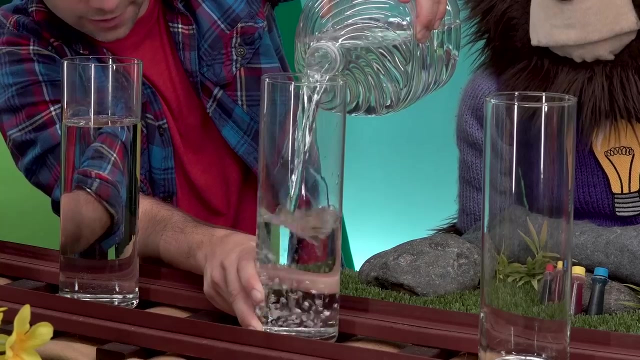 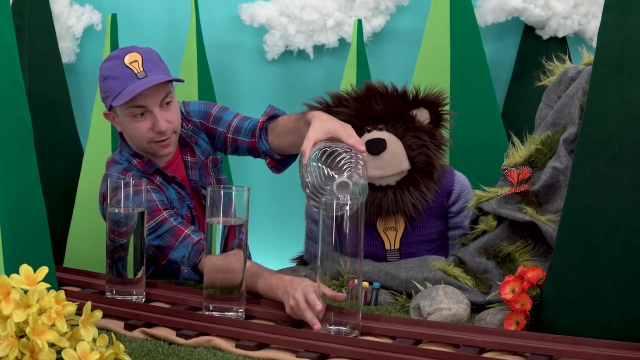 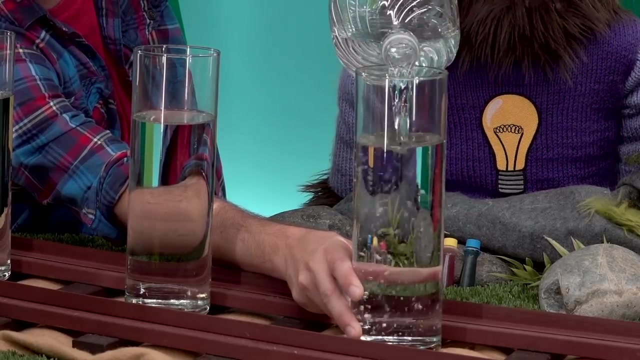 I have some water right here And we'll fill the first container. Okay, Whoa Mayta, look at that. Okay, We'll do the second container. Okay, Then we'll do the last container. Okay, All right. 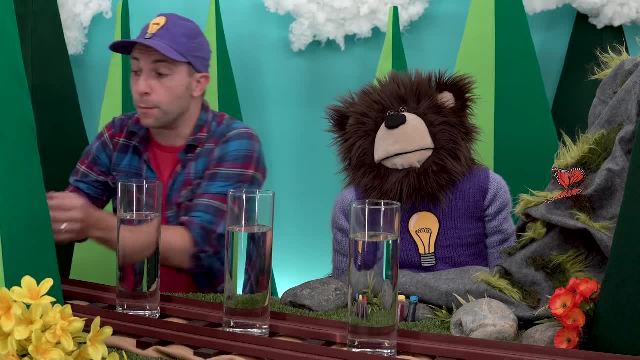 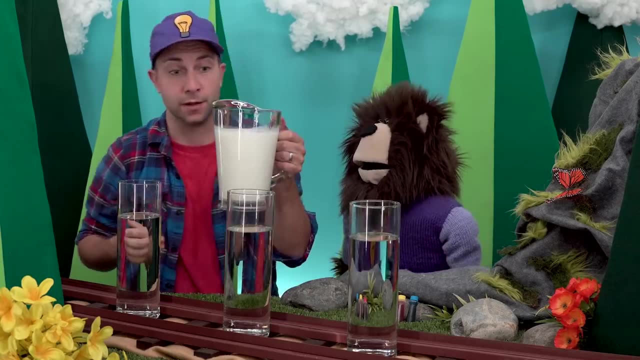 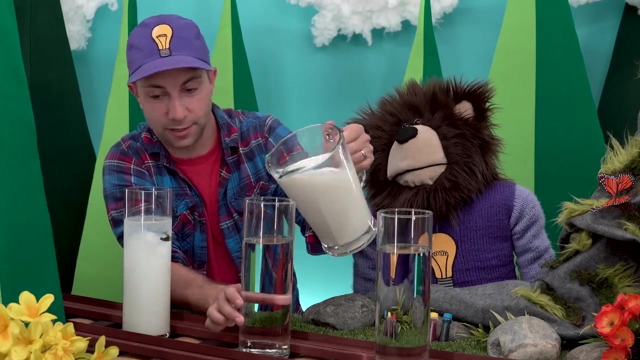 Now we are going to take our milk. We're going to add just a splash of milk to each one of these containers. Are you ready, Mayta? All right, Here we go. Whoa, And this one, Whoa. 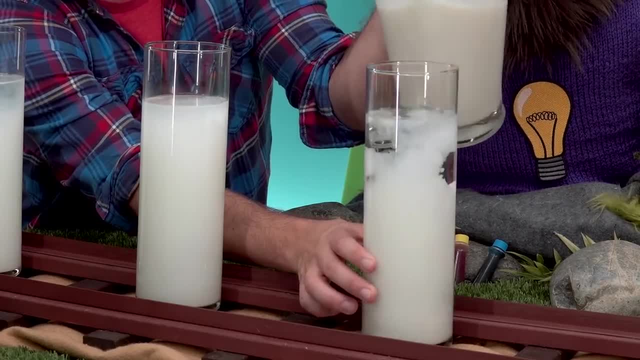 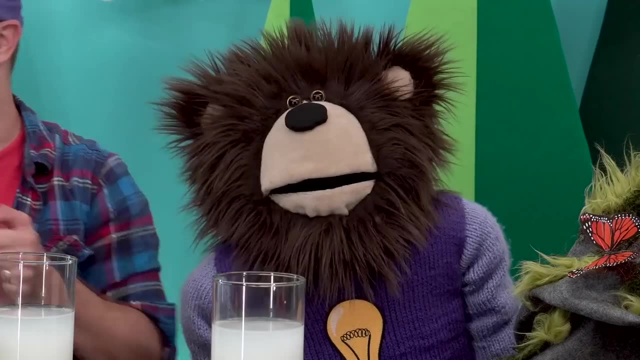 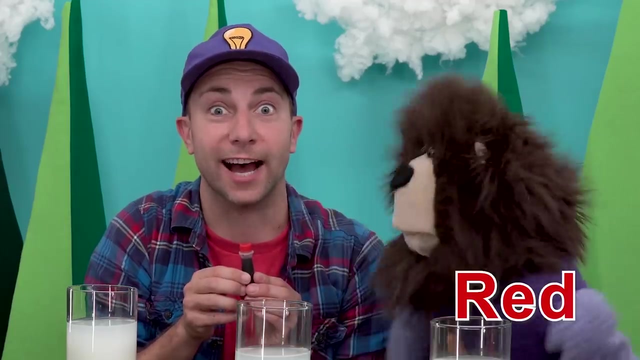 And this one: Whoa, Whoa. Look at that, Mayta. Adding milk will help our colors be nice and bright. Okay, Now we are going to add the dye. First, the red dye. All right, Let's open it up, Mayta. 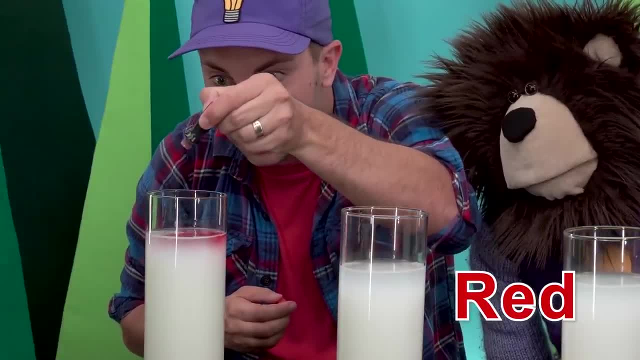 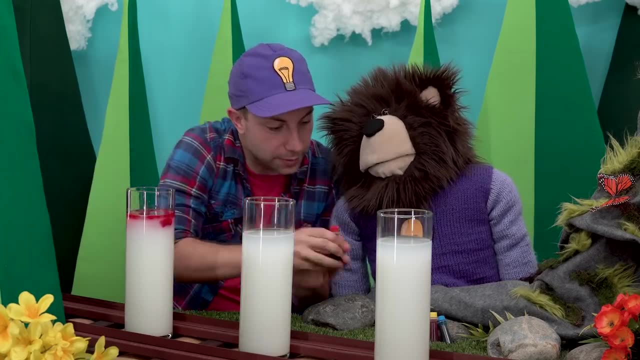 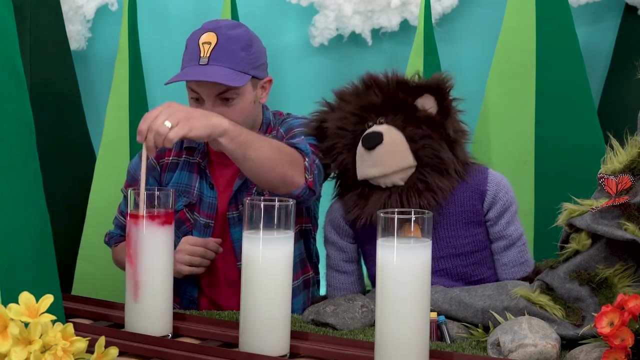 And we'll put a few drops in here. Whoa, Look at that, Mayta. Wow, Okay, Close it up. Then we will take a wooden stick and stir it up. You ready, Mayta? Okay, Here we go. 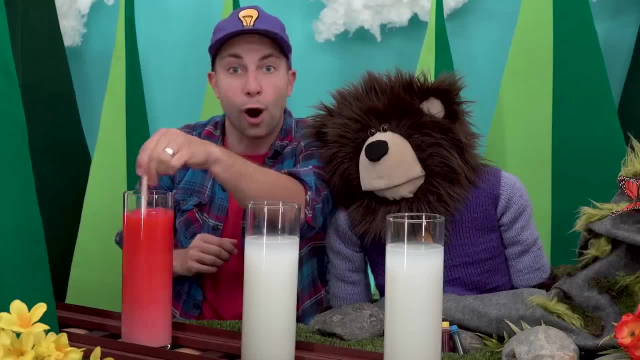 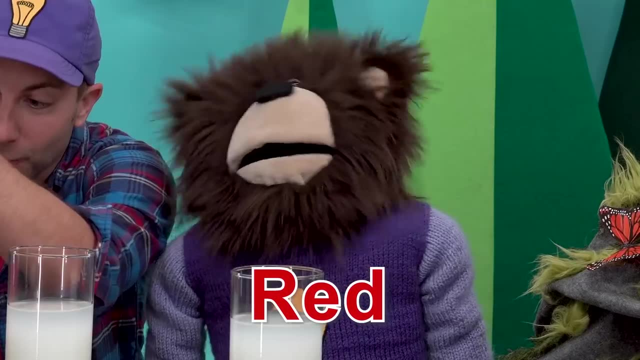 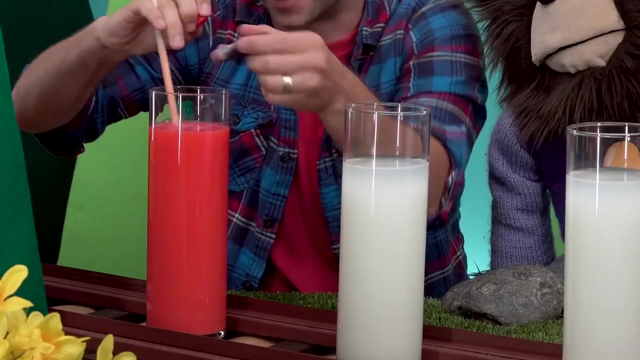 Whoa, Look at that, Mayta. The water, milk and the red dye are mixing together to make the color red. Wow, That is pretty neat. Hey, Mayta, let's add a few more drops of red dye. 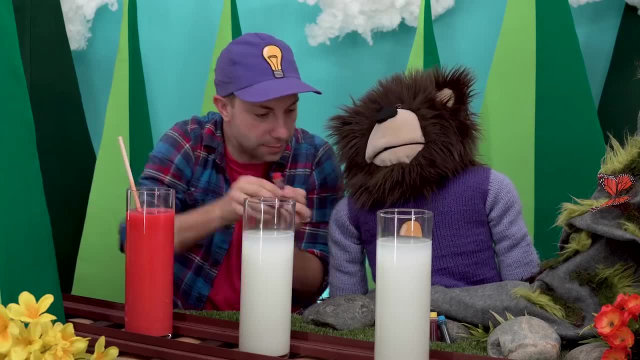 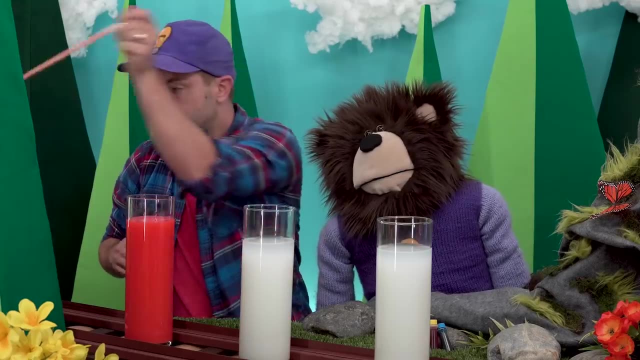 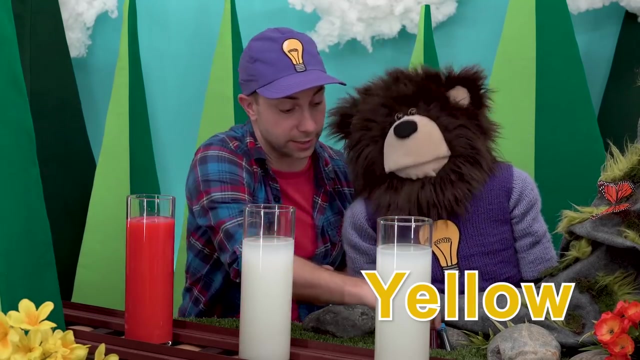 Boop boop, boop, boop boop. Close that up and stir again. There we go. It's nice and bright, Wow. Okay, Mayta, let's add the yellow dye to the second container, All right? 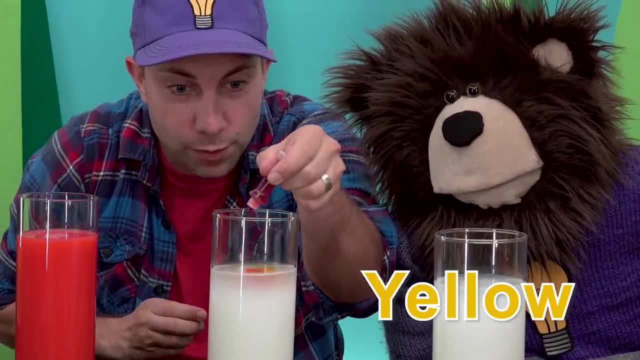 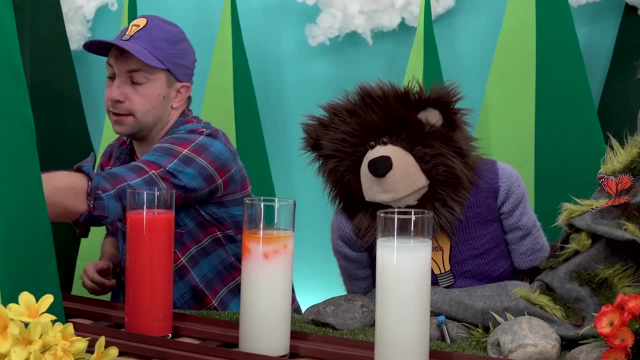 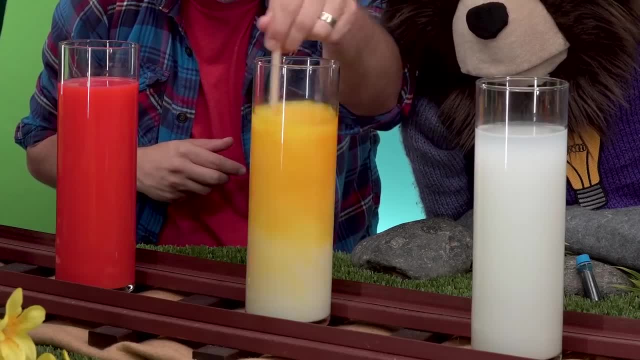 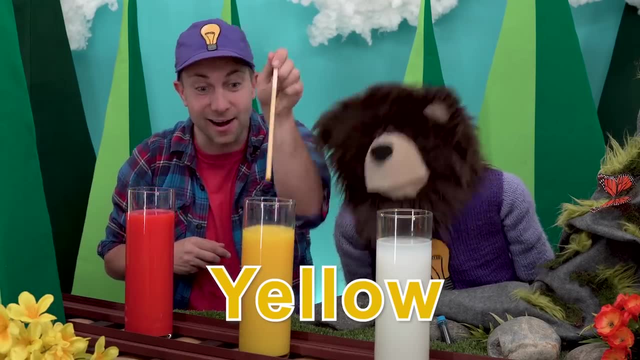 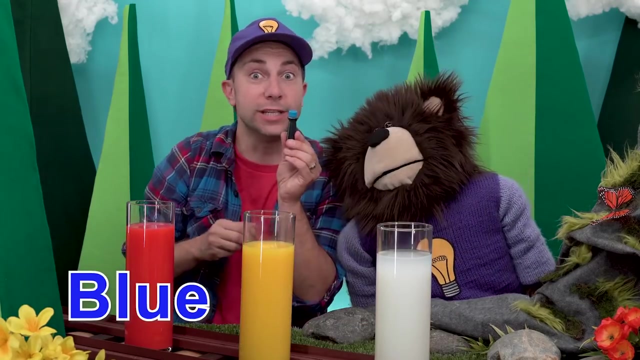 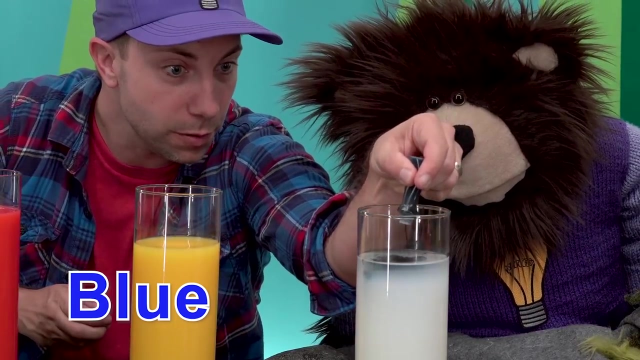 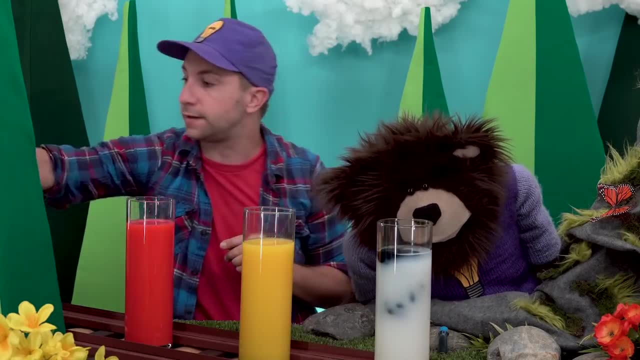 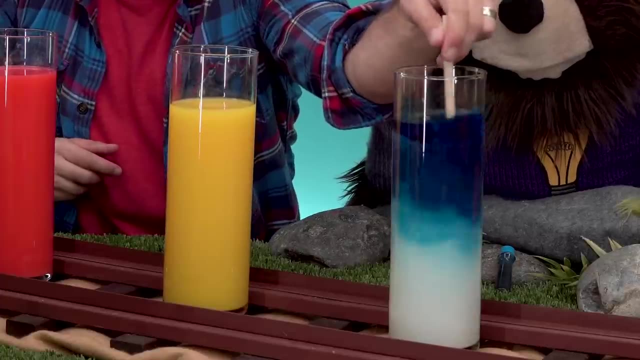 Okay, Boop. And then take a wooden stick and mix it up. Are you ready, Mayta? Yes, Okay, Here we go. Whoa, Look at that, Mayta, It's turning blue. These three colors are called primary colors. 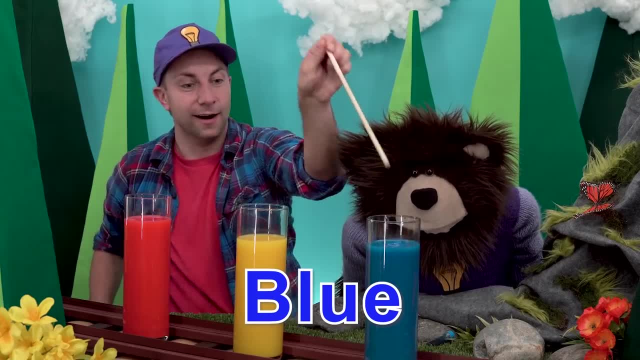 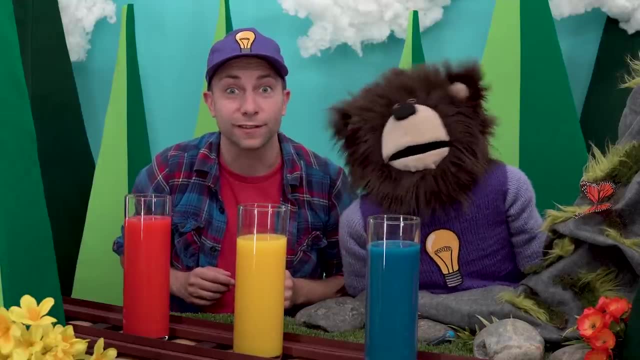 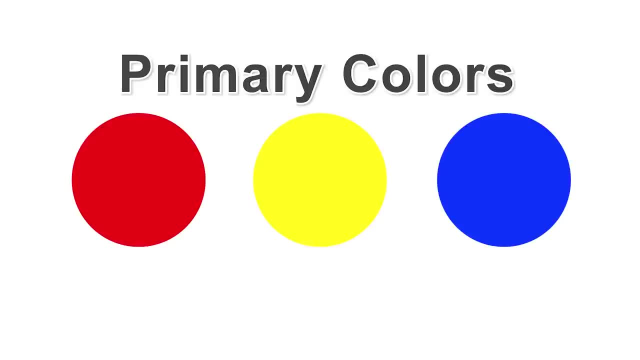 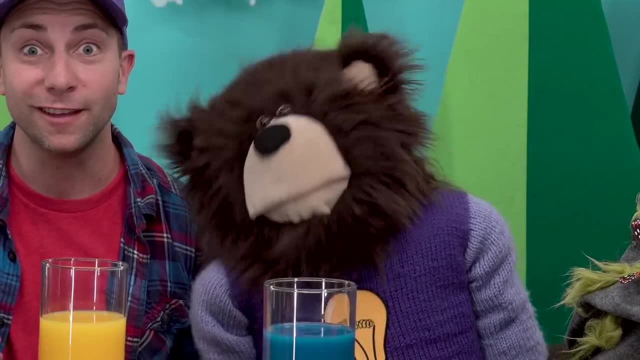 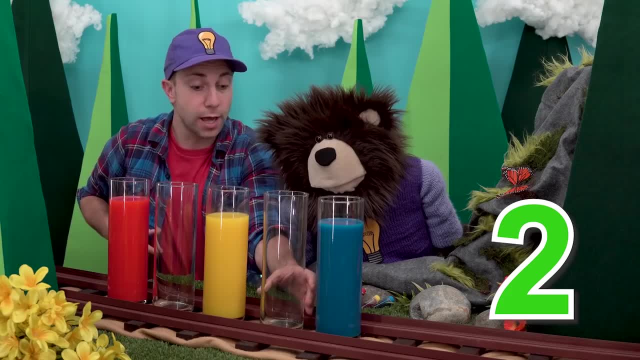 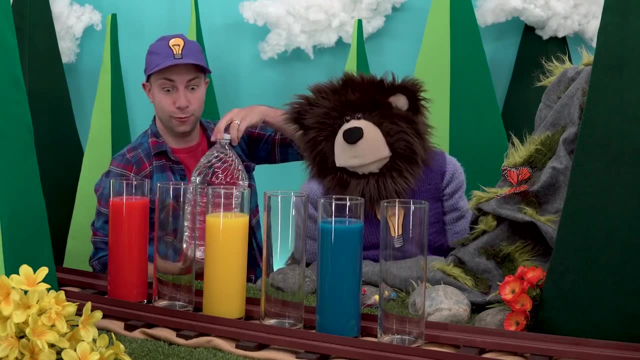 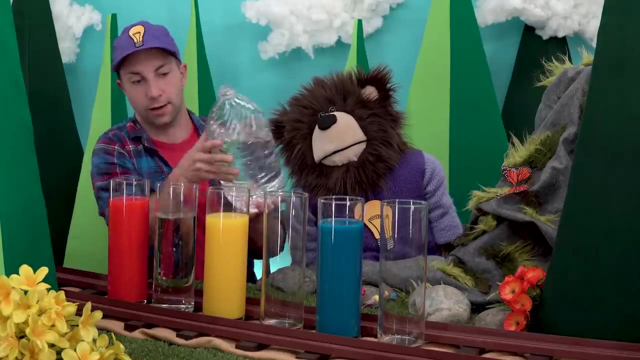 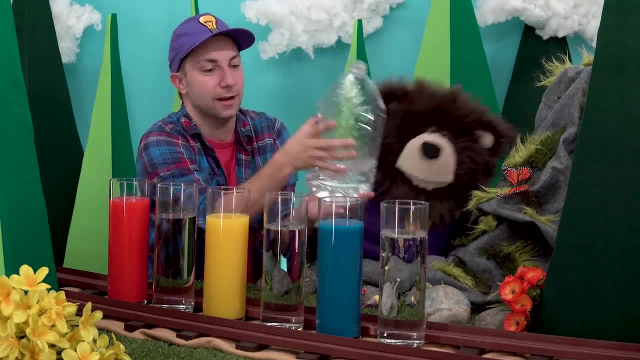 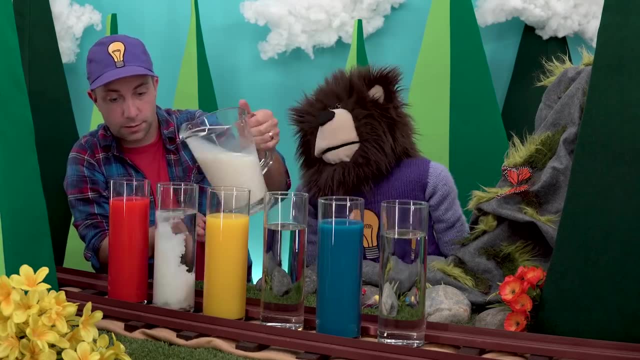 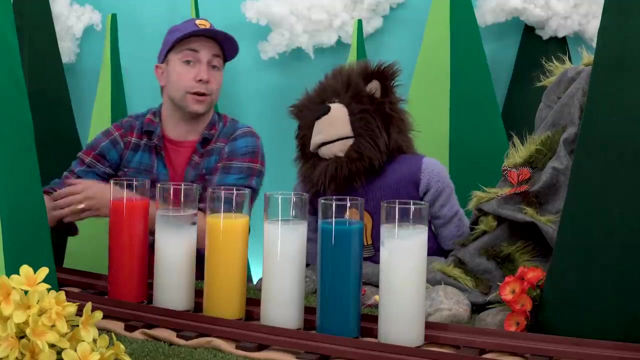 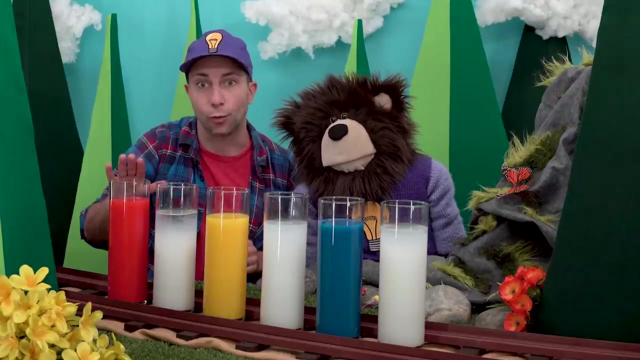 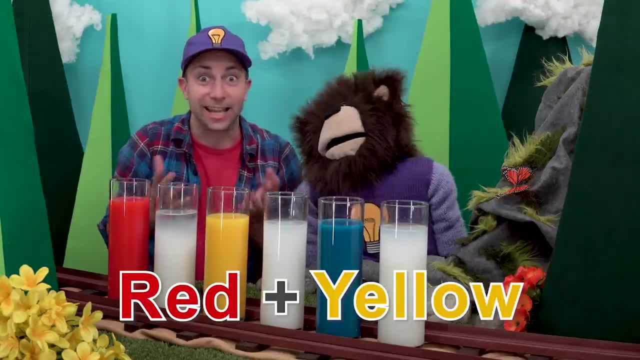 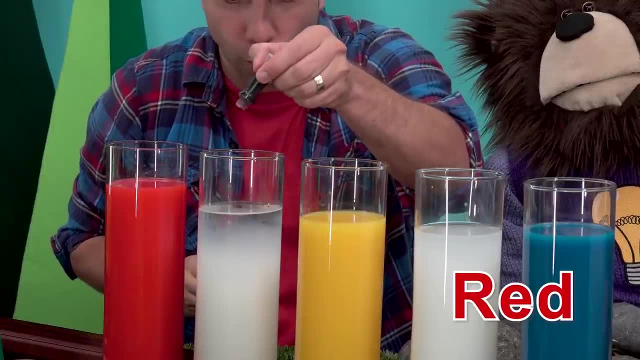 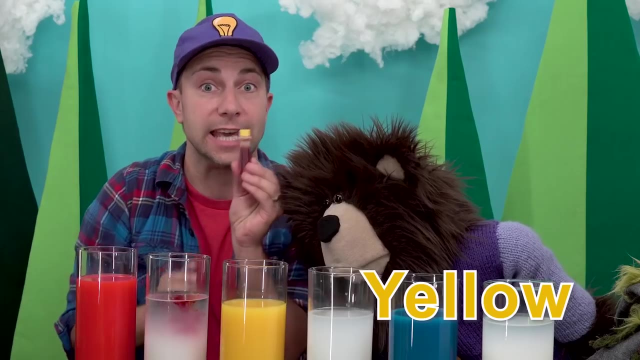 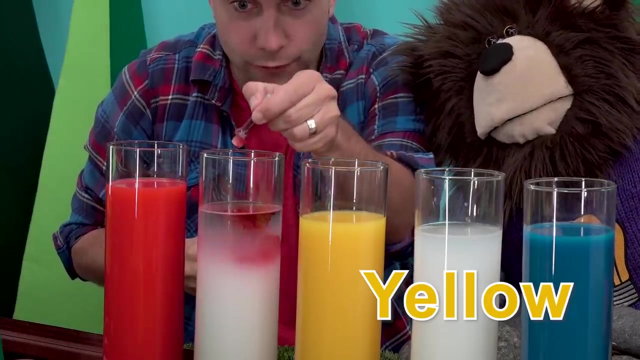 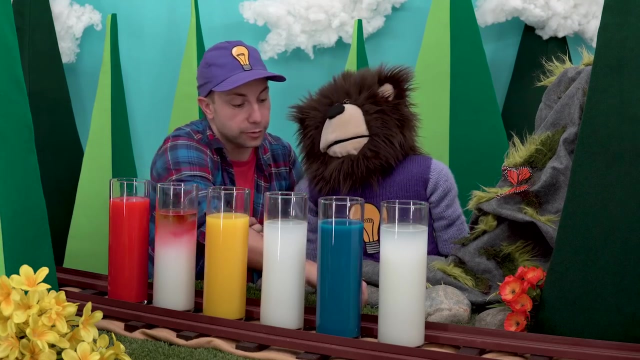 All right with yellow, let's find out. all right, so first we will take our red dye and add two drops: one, two, all right. next we will take our yellow dye and add five to six drops: one, two, three, four, five, six, one more seven. okay, now we will take the wooden stick and mix it up. are you ready? here we go. 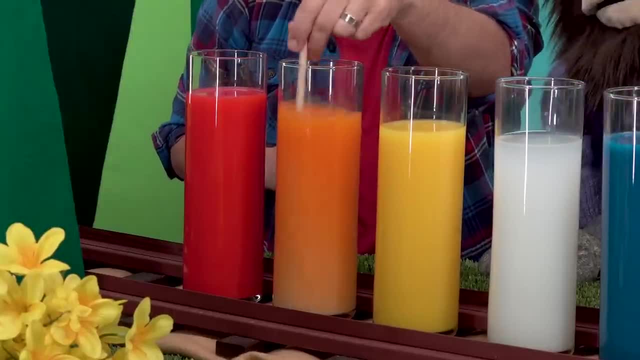 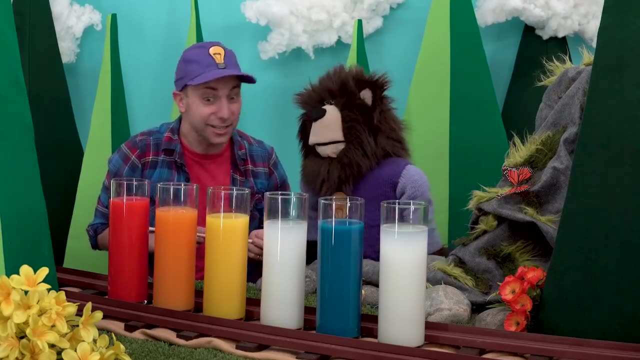 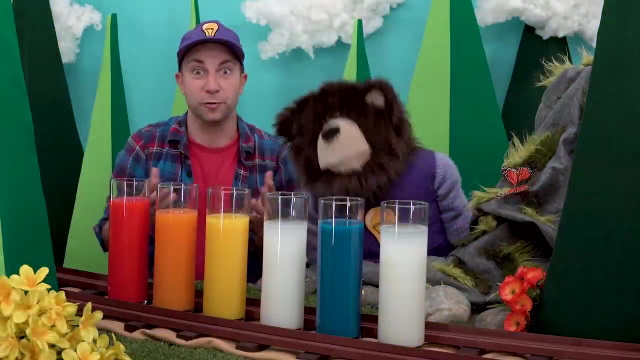 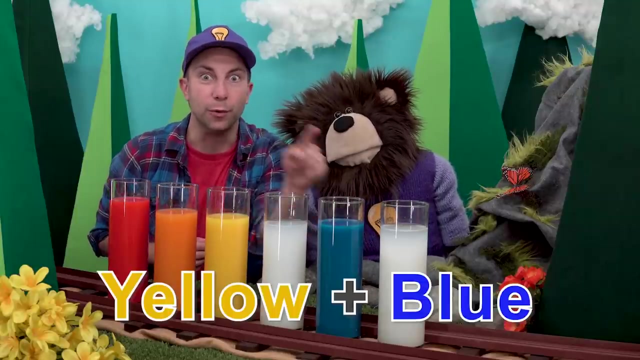 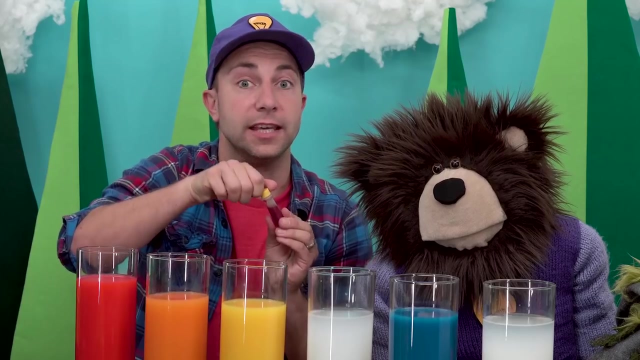 whoa mayta. look at that: mixing red with yellow makes orange. that is really neat. red mixed with yellow makes orange. are you ready to make another color? all right, what do you think will happen if we mix yellow with blue? let's find out. first, we will take the yellow dye and add about five to six drops. 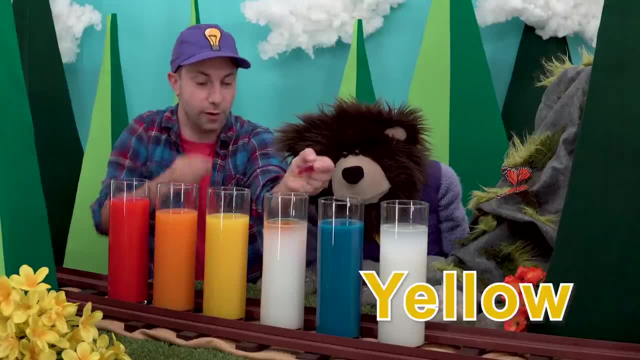 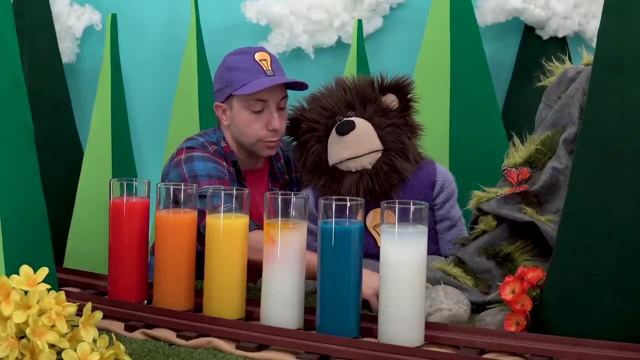 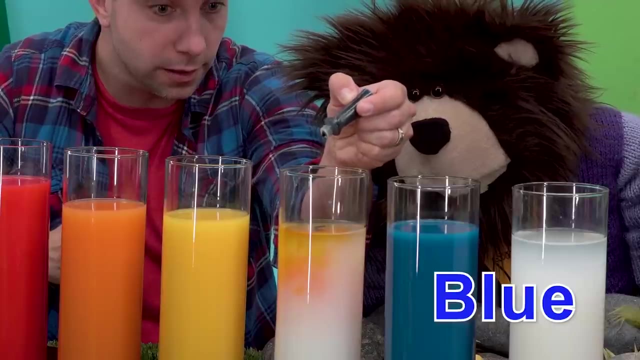 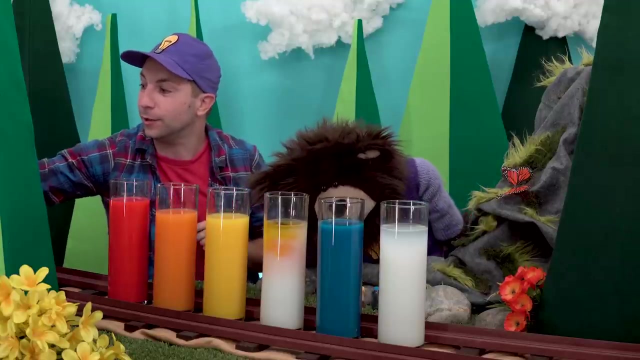 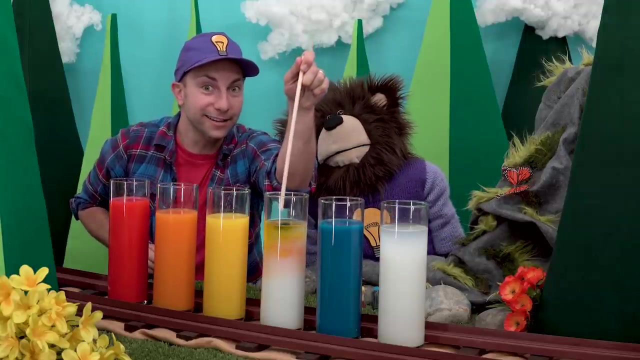 one, two, three, four, five, six. okay, let's add another drop, mayta. all right, now we will take our blue dye and add two drops: one, two. okay, we will take a wooden stick and mix it up. are you ready to see what color we are making? yes, okay. 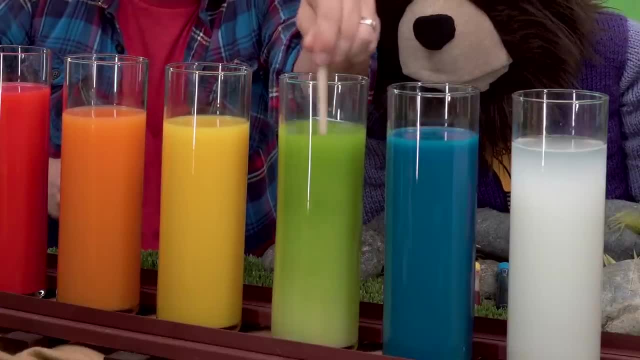 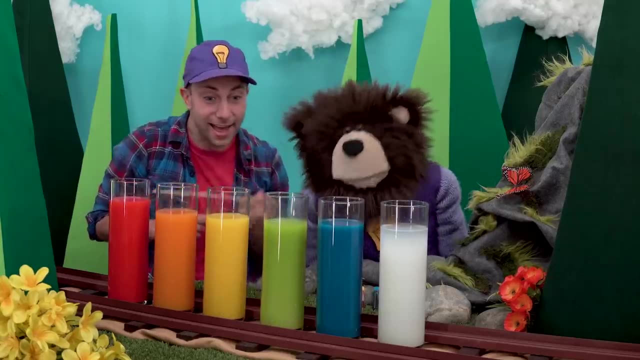 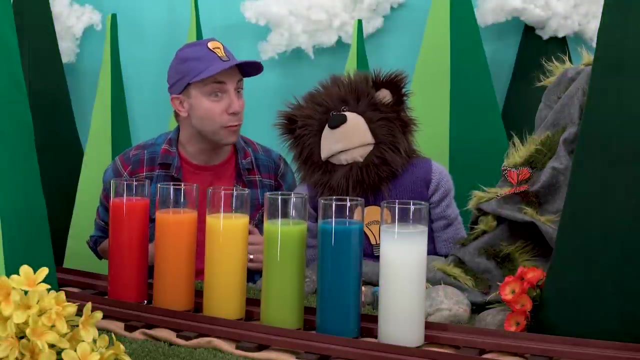 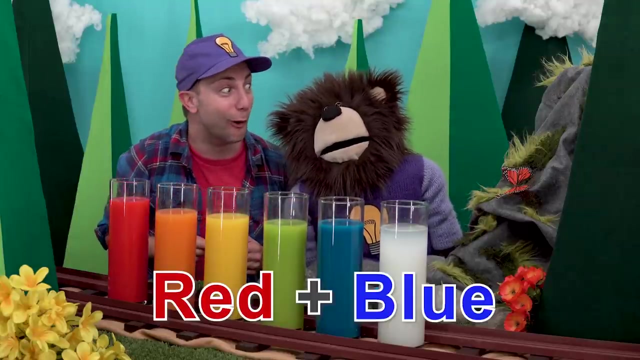 whoa mayta. Mixing yellow and blue makes green. Wow, look at that. Yellow mixed with blue makes green. Let's make one more color. What do you think will happen if we mix red and blue? Oh Okay, so let's take our red dye. 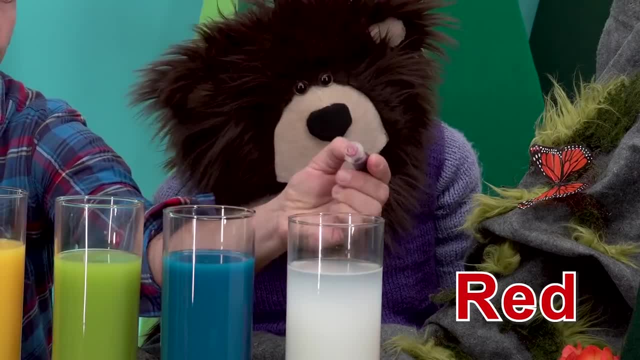 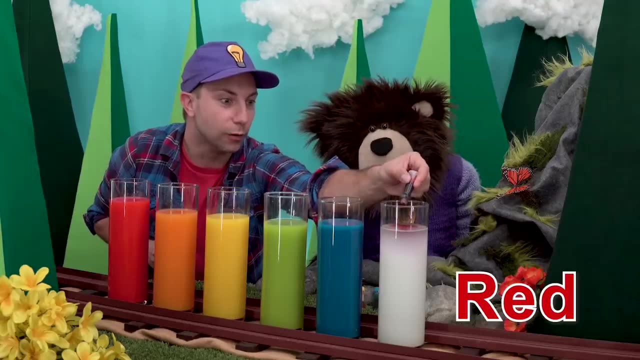 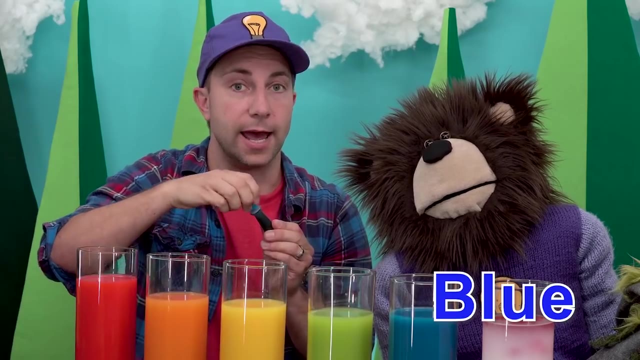 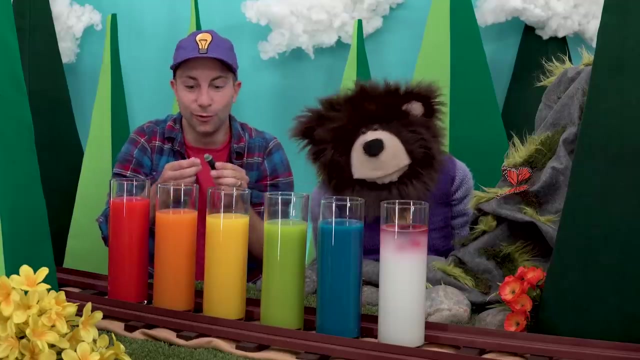 and we will add about four to five drops: One, two, three, four, five. All right, one more. And then we will take our blue dye and add two drops, One, two. What color do you think we are going to mix? 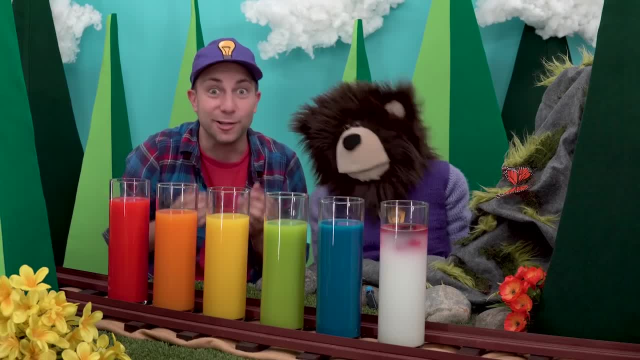 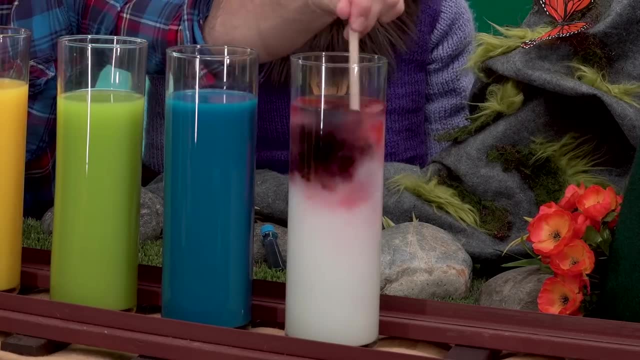 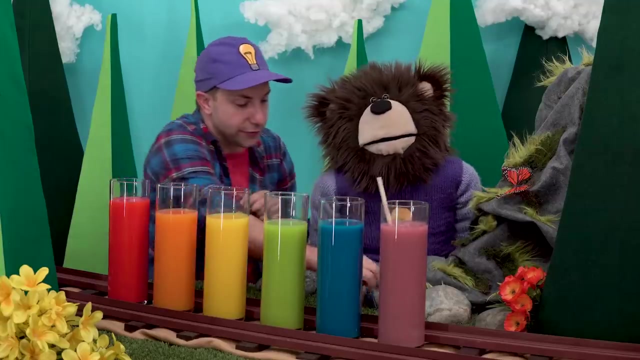 We are making, Mayta, Do you know? Let's find out. Okay, take the wooden stick and mix it up. Whoa, look at that, Mayta. Let's add a few more drops of red to really make it nice and bright. 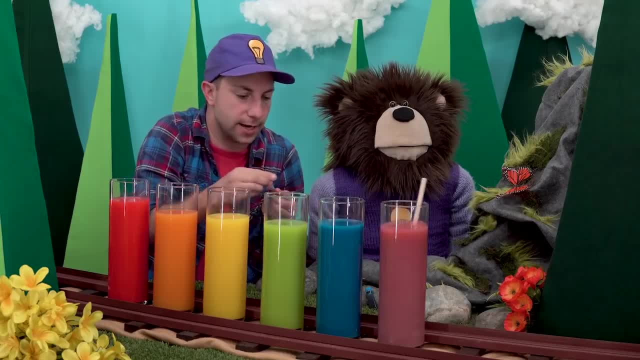 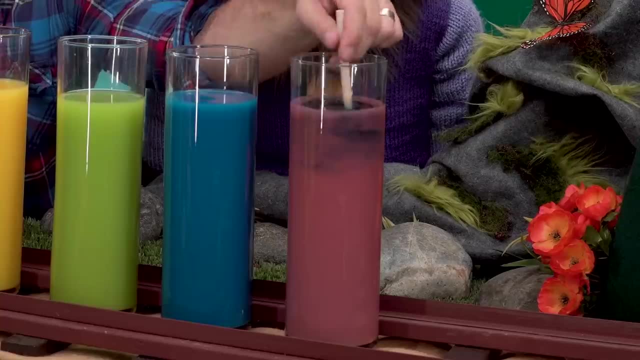 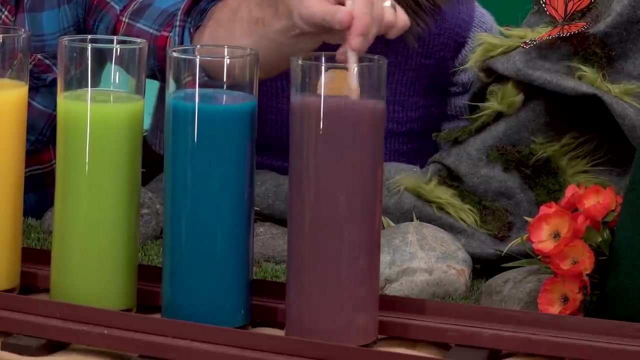 Okay, Oh, we're going to need to add a few more drops of blue Boop, boop, boop. Let's see, There it is, Mayta, Look at that. That is the color purple. Wow, Red mixed with blue makes purple. 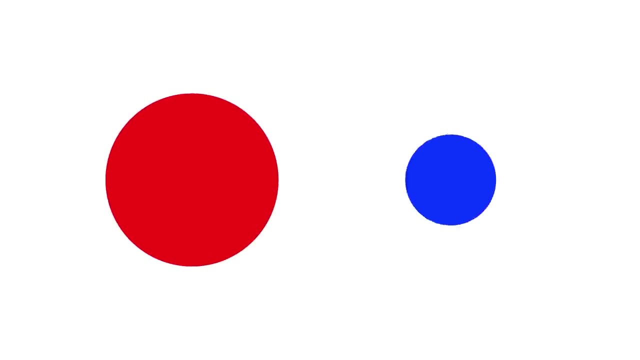 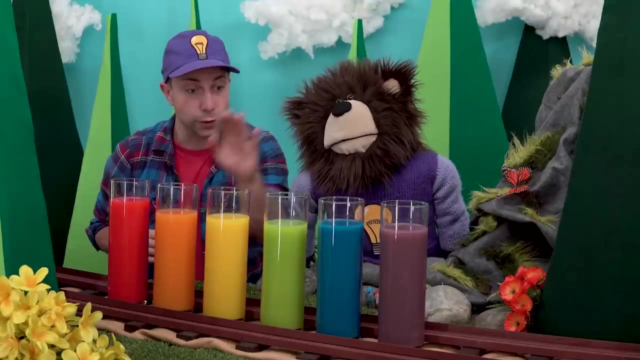 These three new colors- orange, green and purple- were made by me and Mayta And I'm going to mix them together. I'm going to mix it up, And then I'm going to mix it up, And then I'm going to mix it up. 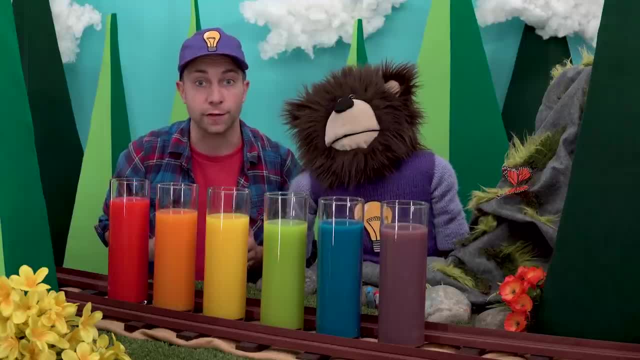 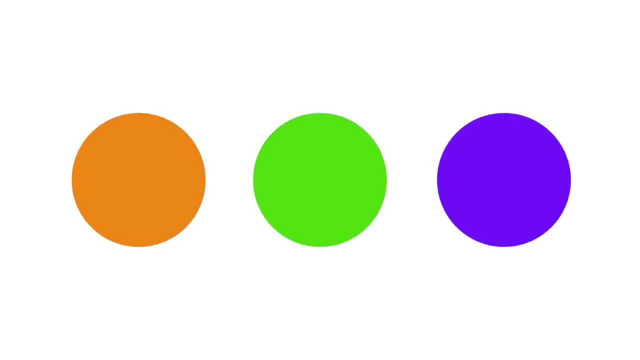 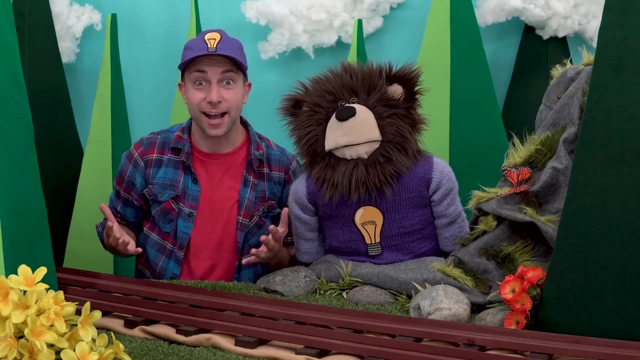 And then I'm going to mix it up By mixing primary colors. They are called secondary colors. They are called secondary colors. Orange, green and purple are called secondary colors. Do you know what time it is? It's time to dance. 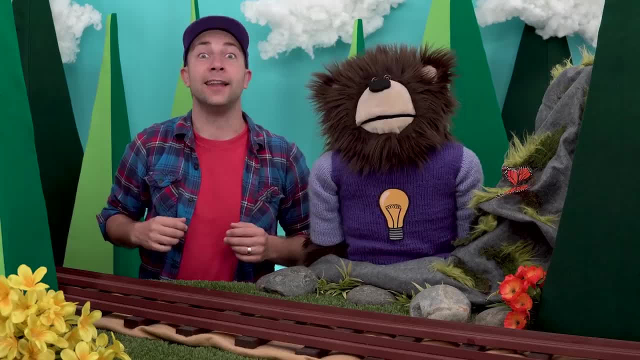 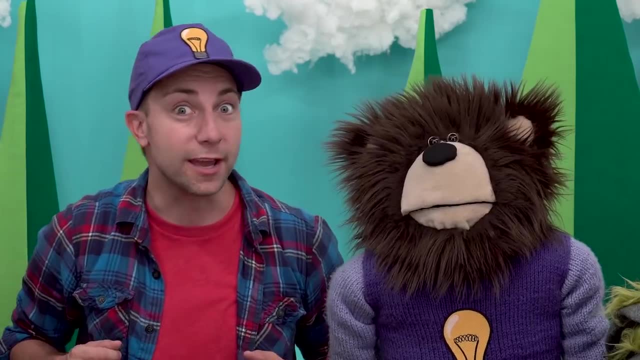 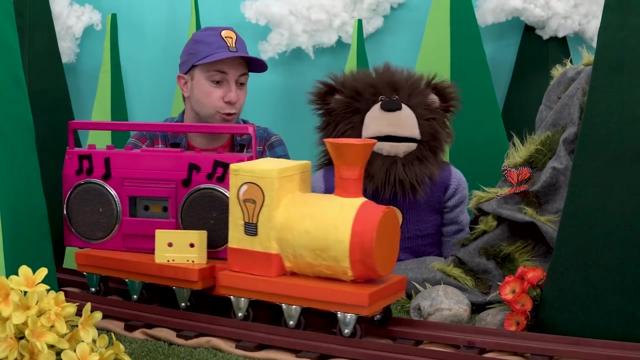 This is where we stop what we're doing. stand up and dance. You can do whatever dance move you feel like doing. You can do whatever dance move. Do you hear that? It's the Idea Train? And look, It's Pinky the Boom Box. 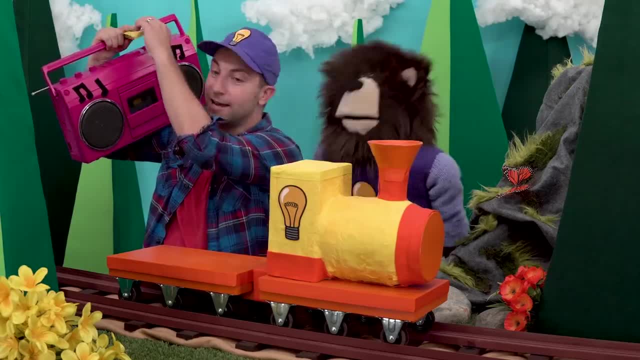 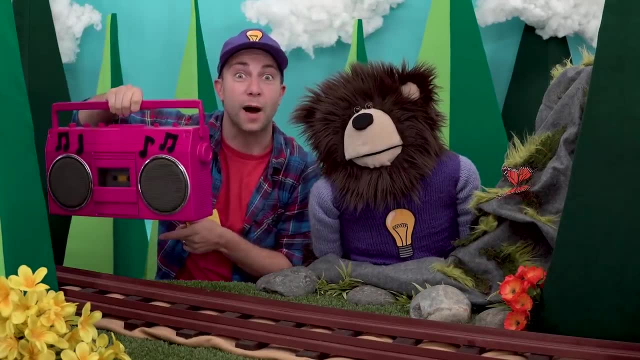 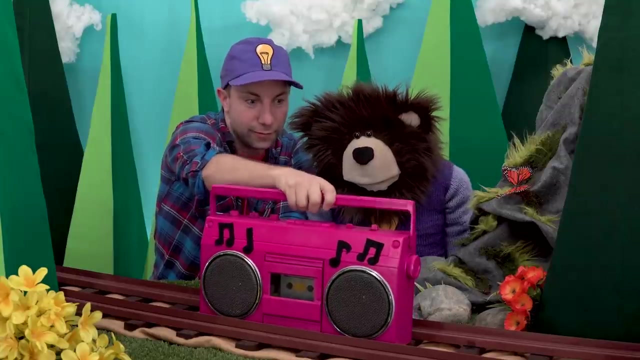 Hi, Pinky the Boom Box. All right, Thank you, Idea Train. Pinky the Boom Box plays our music. We will put Pinky right here. We will put Pinky right here, Then we will take this yellow cassette tape. Then we will take this yellow cassette tape. 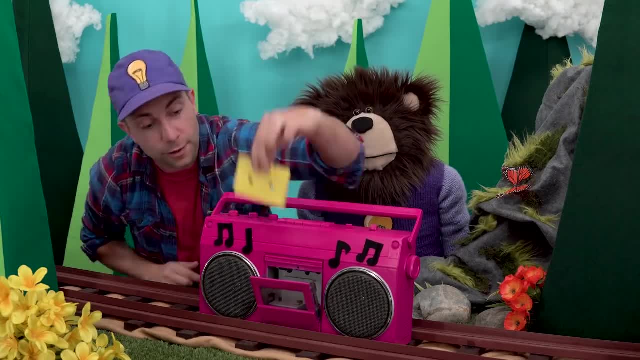 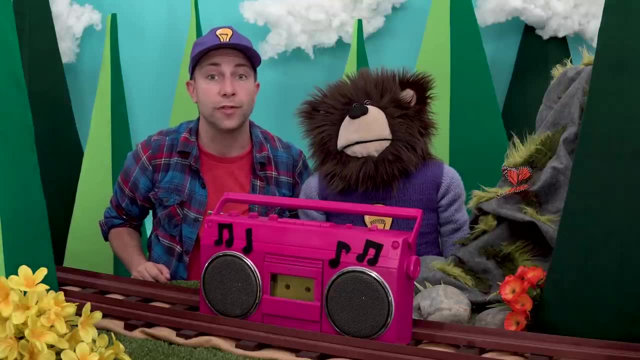 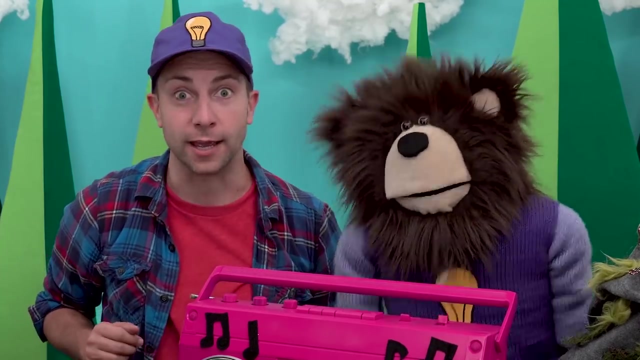 and put it in here. Okay, And then we will close it up. And then we will close it up, Then we will push the button. Then we will push the button with the triangle on it, The play button. Are you ready to dance? 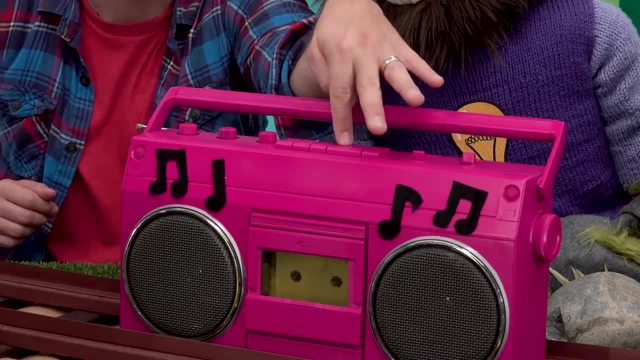 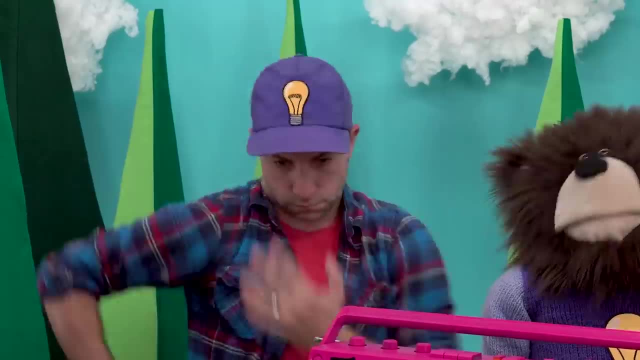 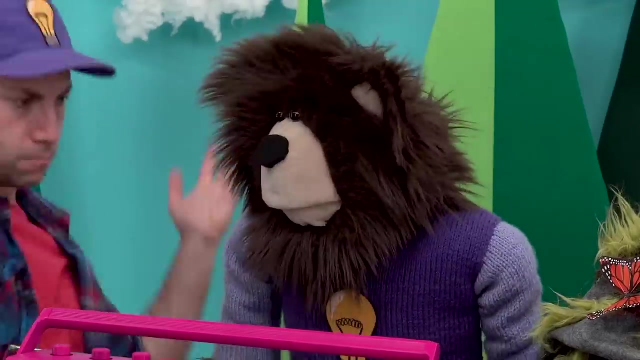 Yes, Okay, I'm going to push the play button now. Here we go. Here we go, Here we go. Are you ready to dance? Yes, Here we go, Here we go. We are ready to dance, Here we go. 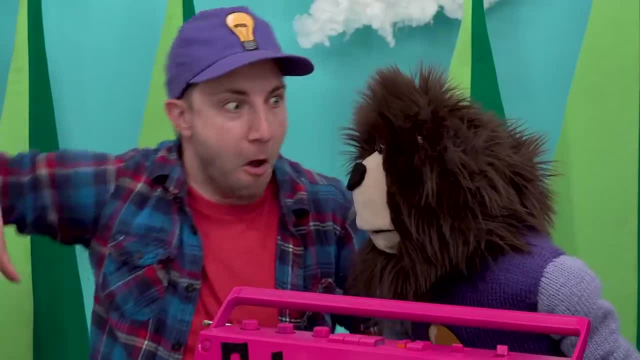 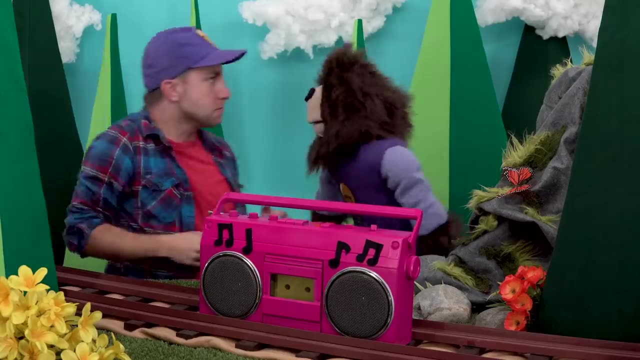 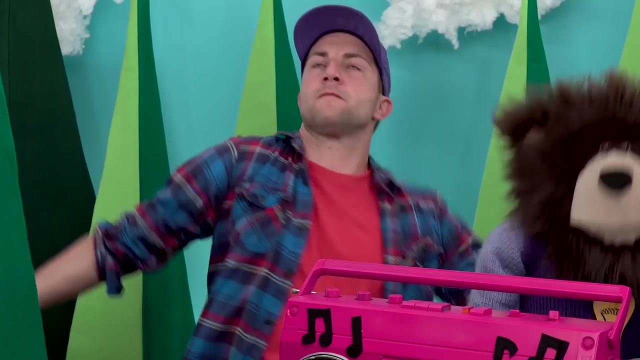 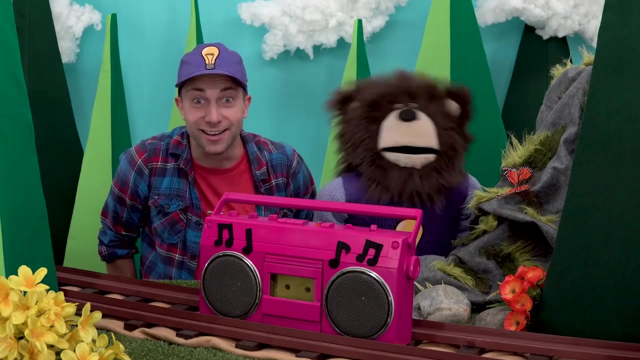 We are ready to dance. Come on, Hey, What's up, Pinky? Hey, What's up, Pinky. We are ready to dance. Whoa, that was a lot of fun. Okay, let's get back to what we were doing. 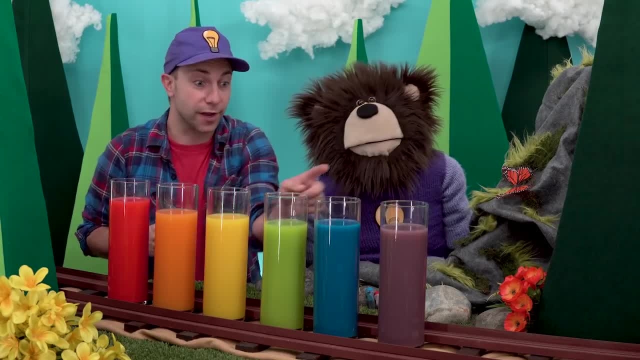 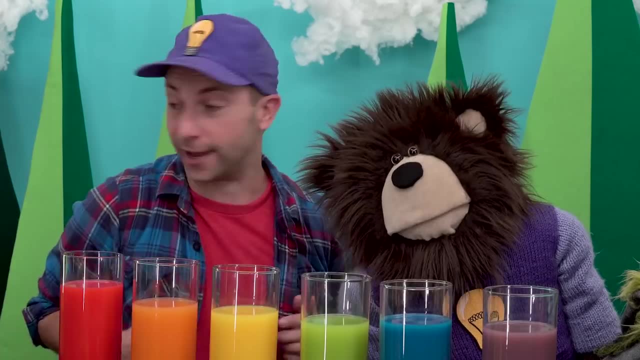 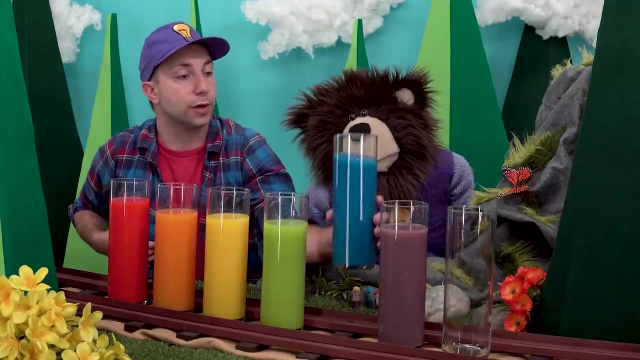 Before we go, what do you think will happen if we mix the color blue with the color purple? Should we find out, Meita, Yes, Okay, I have one last glass container. We will pour half of our blue color into this container. 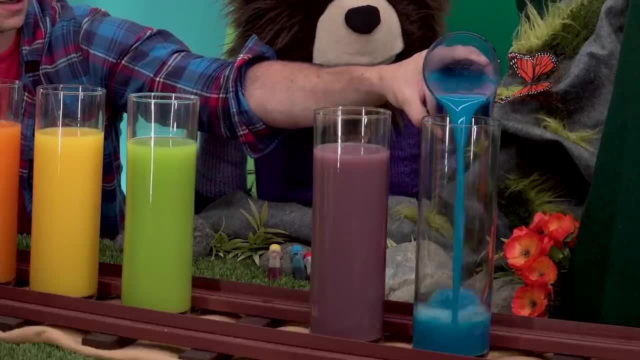 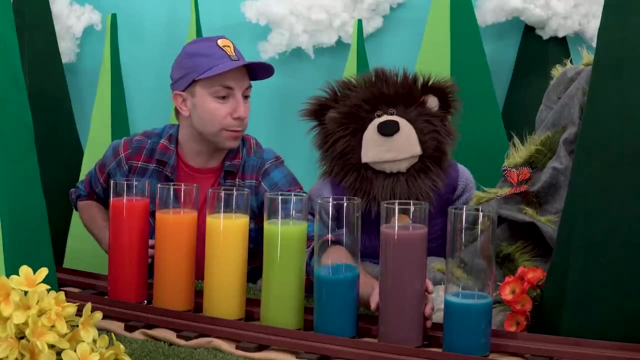 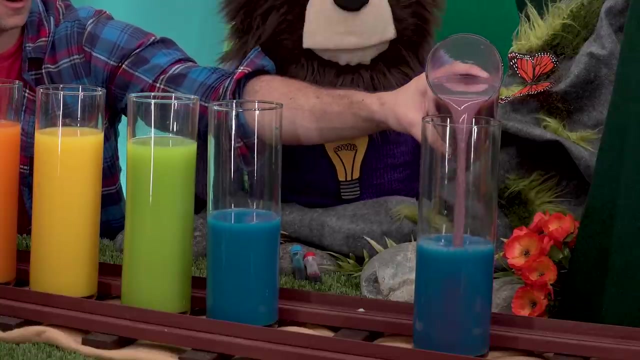 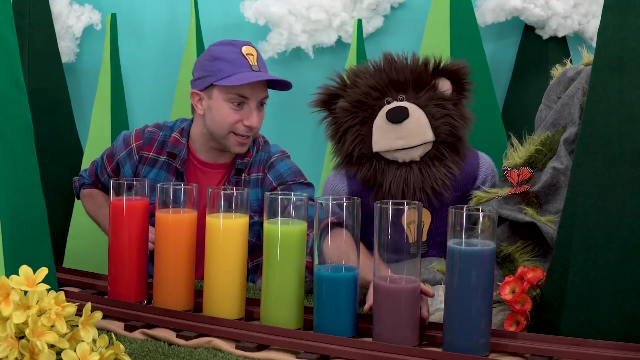 Are you ready, Meita? Here we go. Whoa, Now we will take our purple and pour half of the purple into the same container. Whoa, Whoa. look at that, Meita. Okay, now let's take a wooden stick. 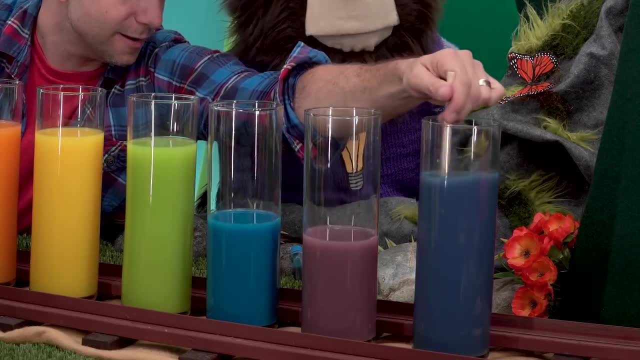 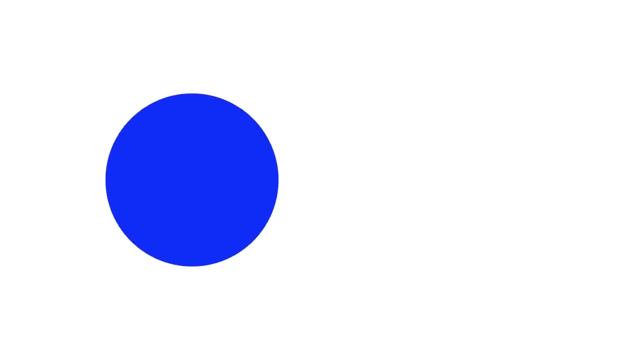 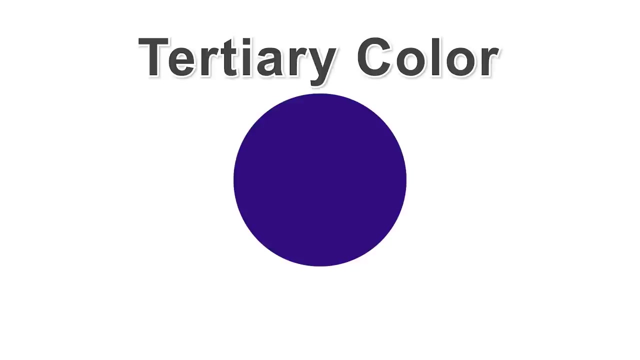 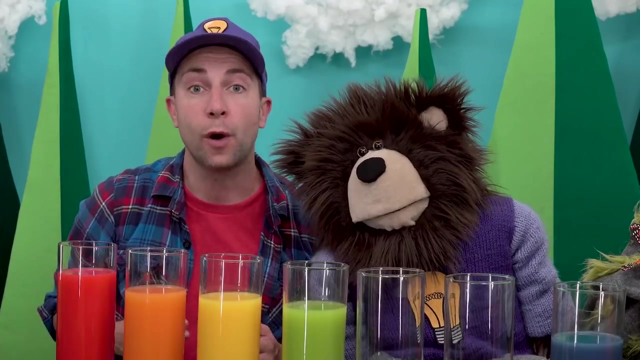 and really mix it up. Whoa, That is the color indigo. Blue mixed with purple makes indigo. Indigo is called a tertiary color. Wow, that was a lot of fun making all these colors. If you want to watch more Meita videos, 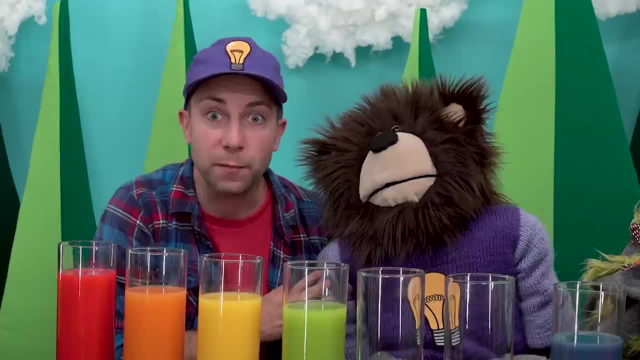 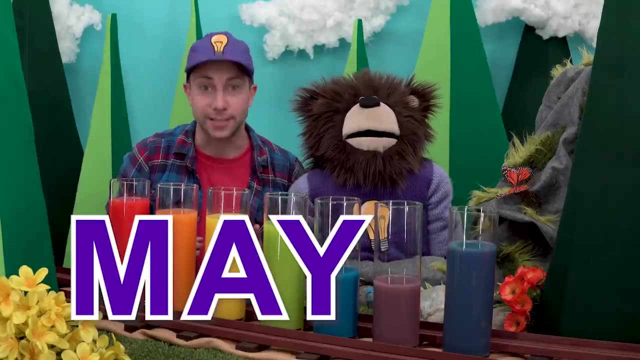 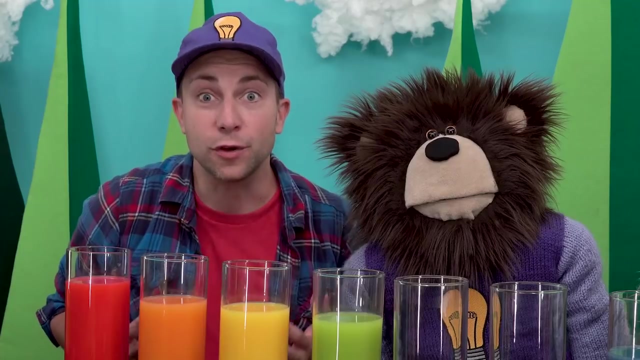 search Meita's name. Do you know how to spell Meita's name? Hmm, Let's do it together: M-A-Y-T-A. Hmm, Meita. Then type the brown bear. Thank you so much for spending your time with Meita and myself. 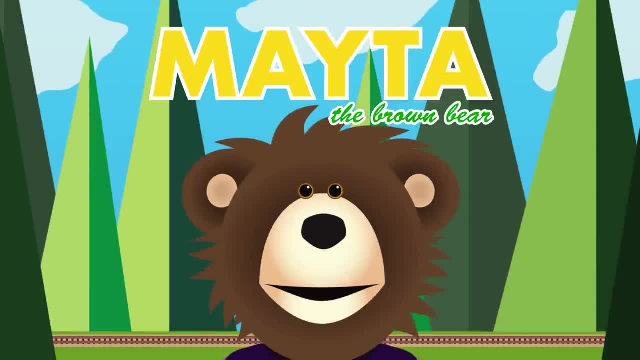 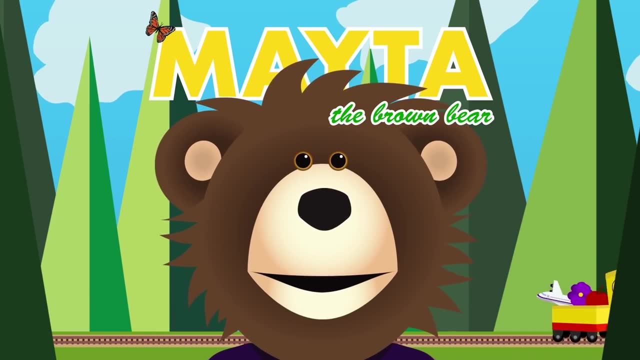 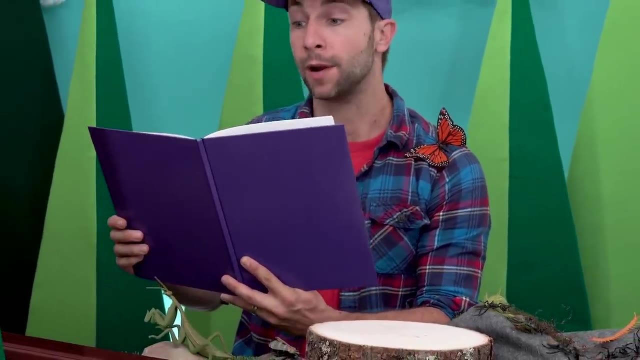 and learning how to make all these different colors. Meita, Meita, Meita, Meita, Meita. The brown bear. There are so many different kinds of bugs in the world. Bugs come in all shapes, colors and sizes. 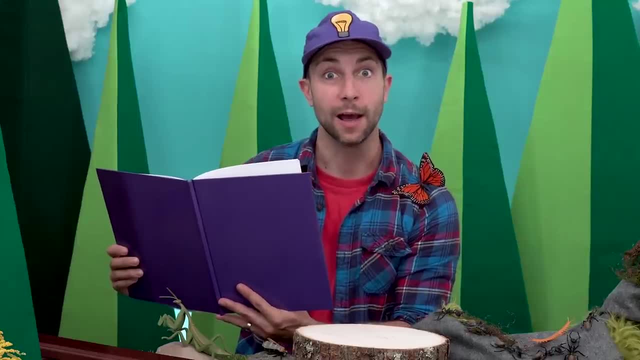 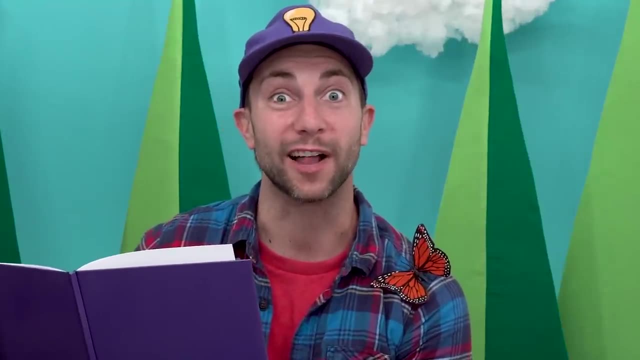 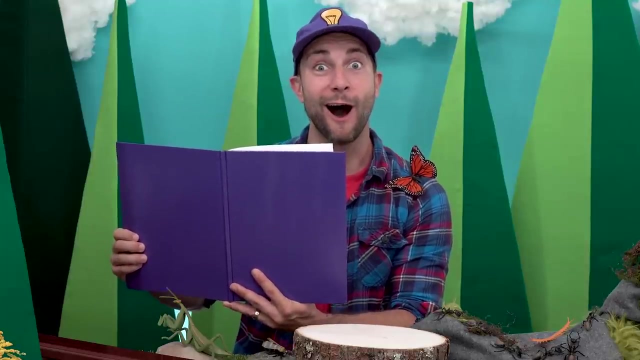 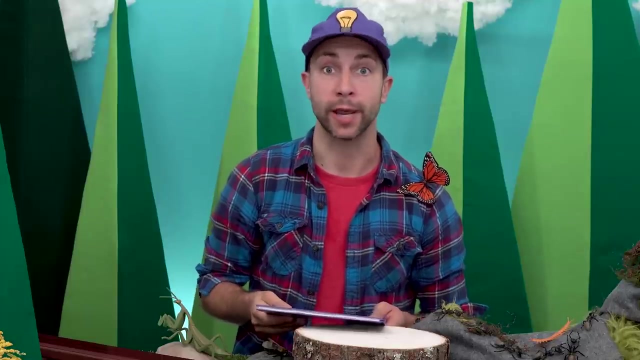 Oh hi, My name is B, like the letter B And this. this is Mr Butterfly and we're reading a book. Do you know what color this book is? That's right, It's purple. Well, we are waiting for our friend Meta to wake up from his nap. 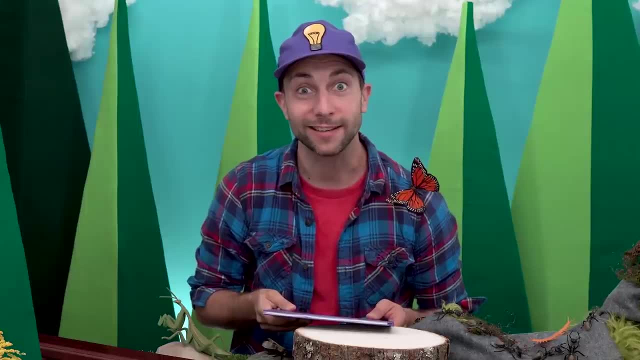 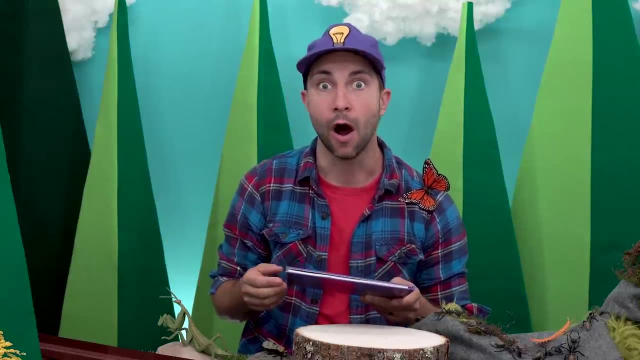 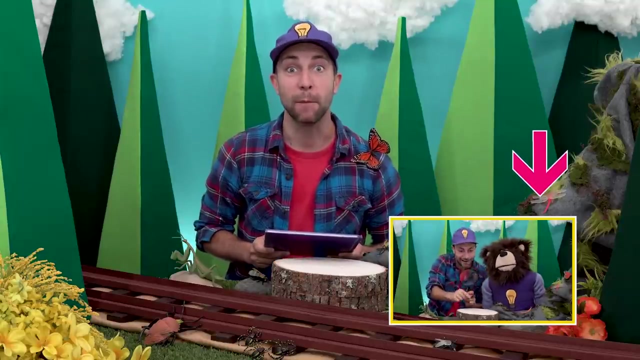 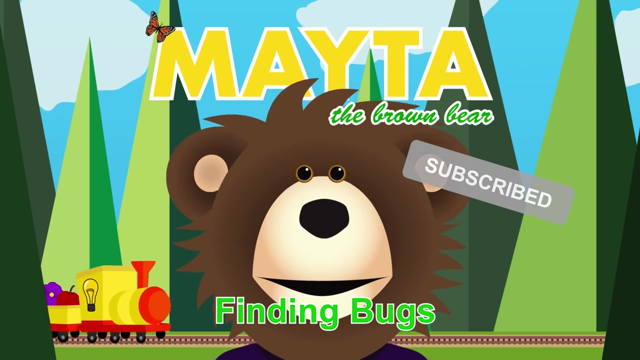 Do you know who Meta is? Meta is a brown bear that lives in this forest. I have an idea. Why don't we wake Meta up from his nap and together we can learn about bugs? Meta, Meta, Meta the brown bear. 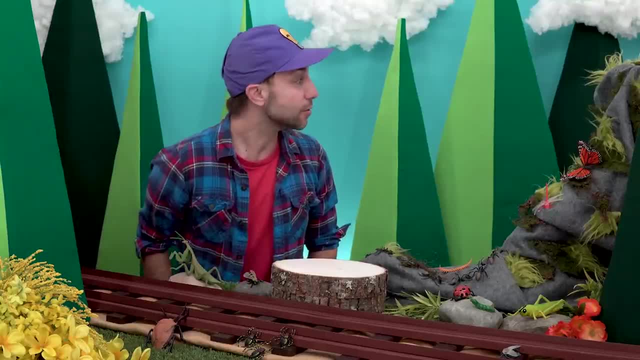 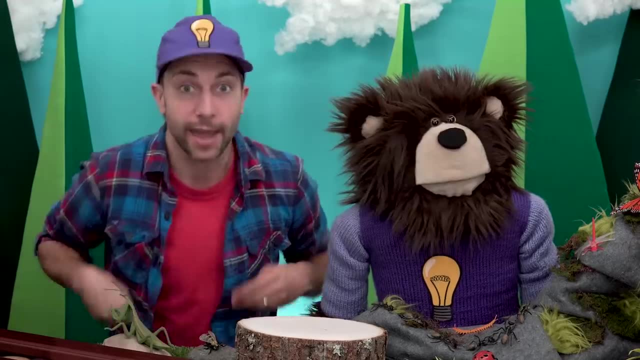 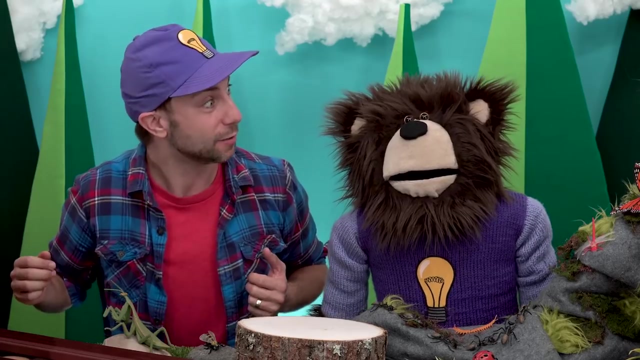 Meta, are you up from your nap? Where are you, Meta? It's Meta. Did you have a good nap? Yes, Hey, listen, we have a lot of friends here today and together we are going to learn about bugs. Do you want to do that? 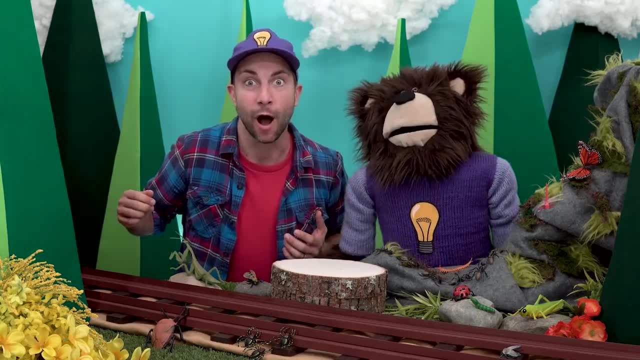 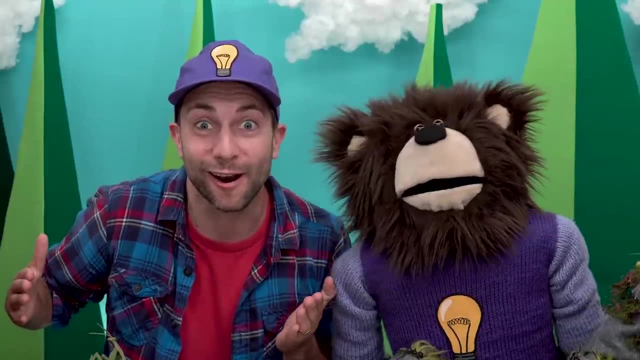 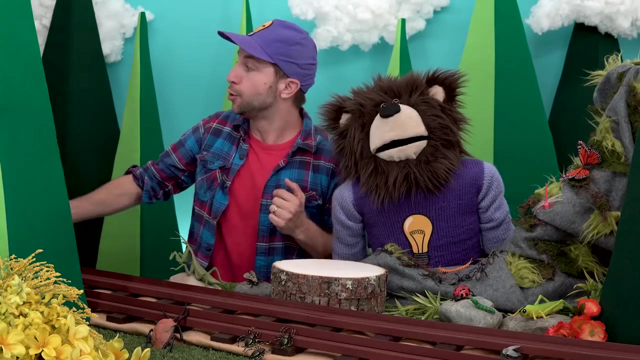 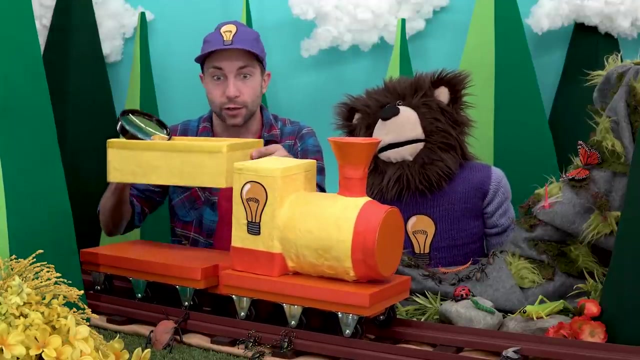 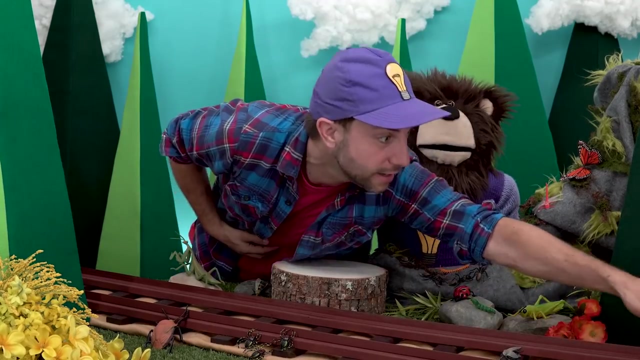 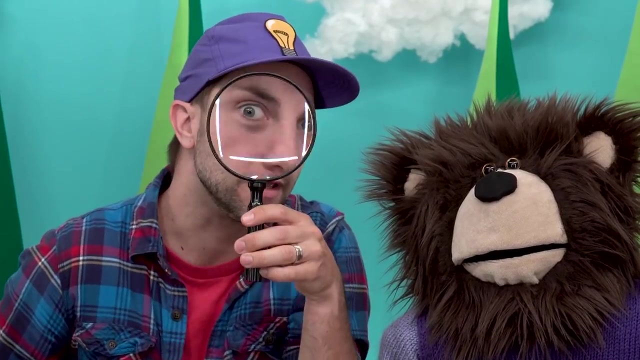 Yes, Okay, Do you hear that? No, Listen harder. Do you hear that? It's the idea train? Oh, Meta, look what's in the box Here. Thank you, idea train, Alright, Oh, Hmm, What is this? 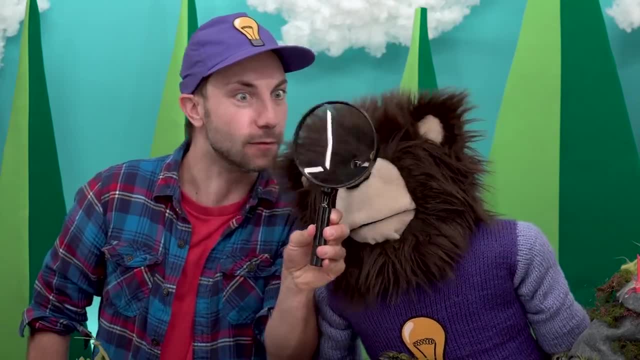 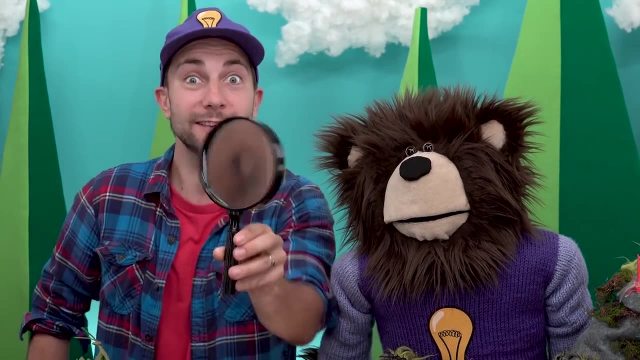 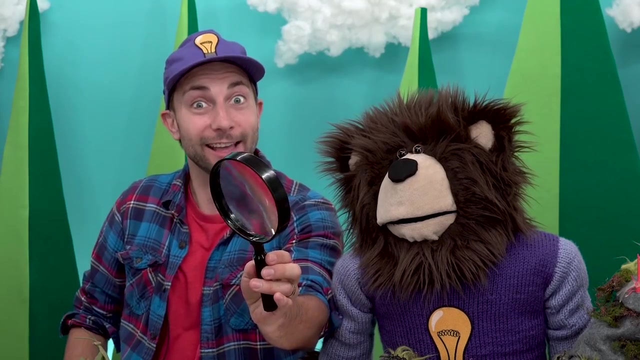 Wait to look through that. Do you know what this is? That's right, It's a magnifying glass. And do you know what a magnifying glass does? Yes, It makes objects look big. So when you look through the glass, 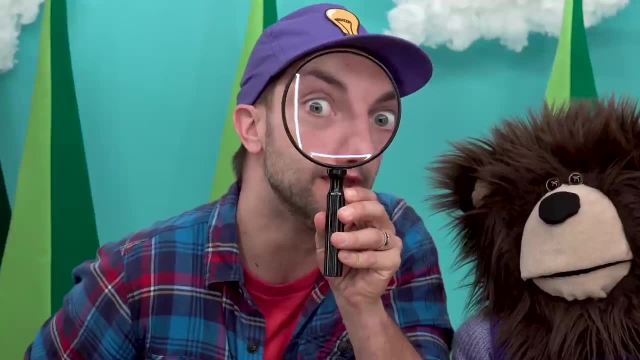 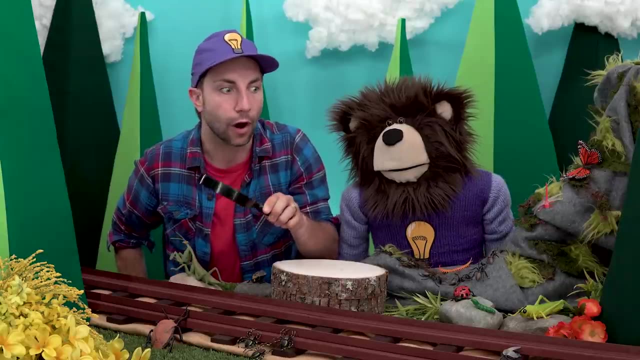 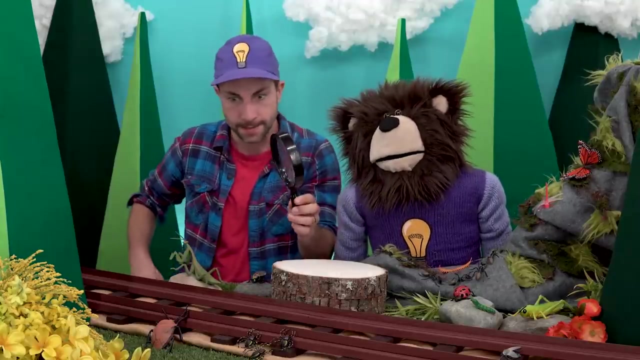 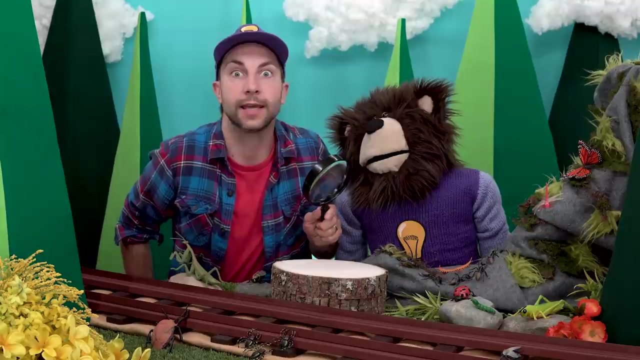 you can see things really big. I have an idea: Why don't we use the magnifying glass to look for all the different bugs in the forest? Should we do that? Yeah, Okay, Let's get started. Hmm, Oh, Meta, There is a caterpillar right in. 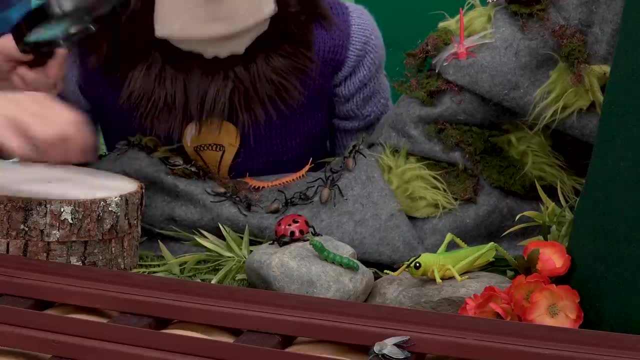 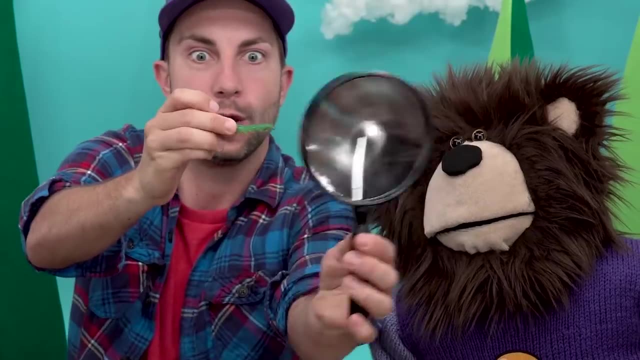 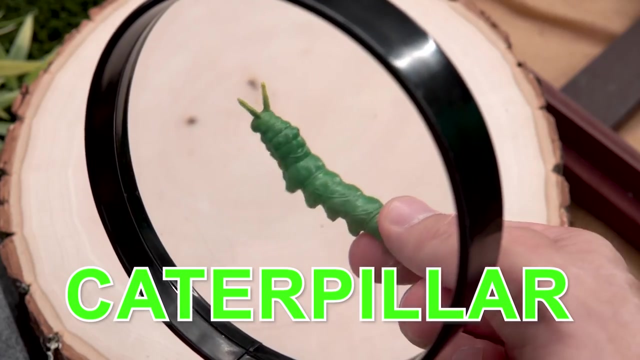 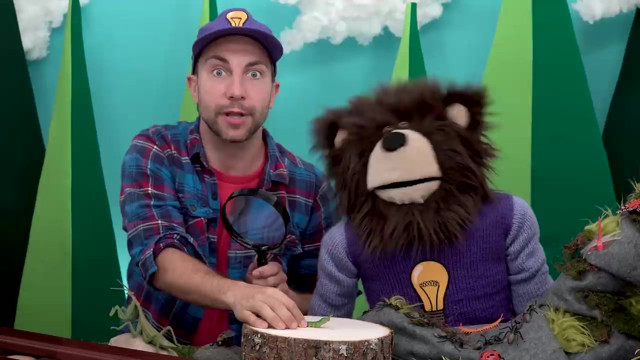 front of you. You see that There he is, Whoa, Take a look, Whoa. Did you know, Meta, that the main job of a caterpillar is to eat? That's right, A caterpillar has to eat a lot of food. so that the caterpillar. 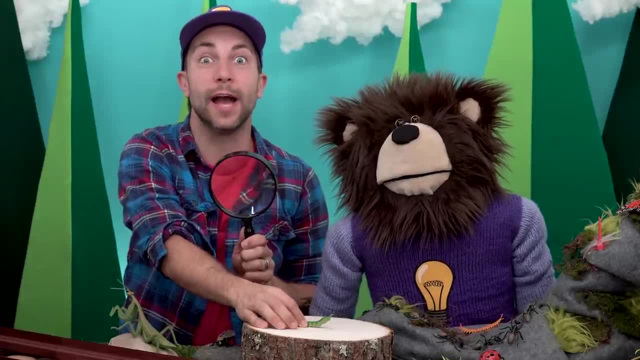 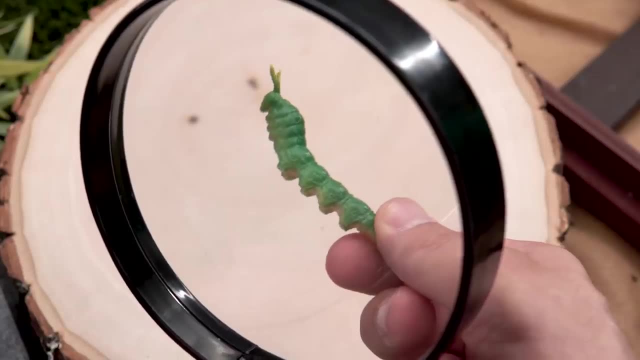 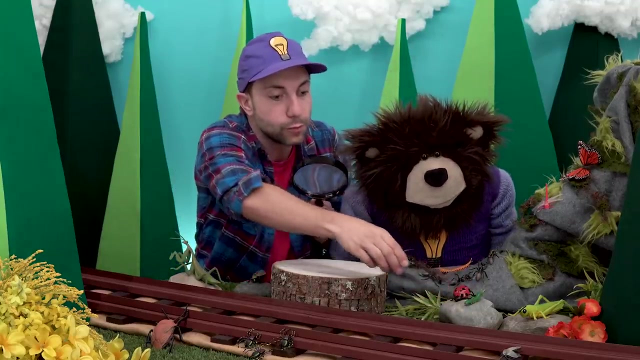 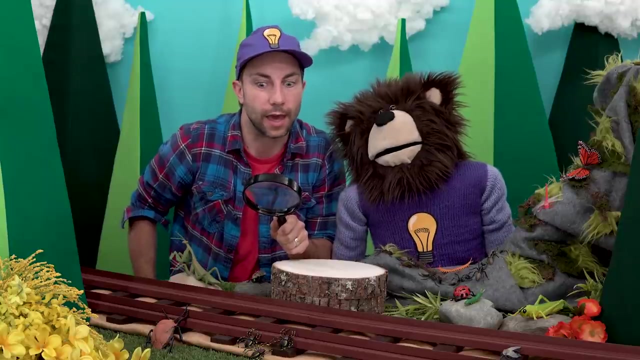 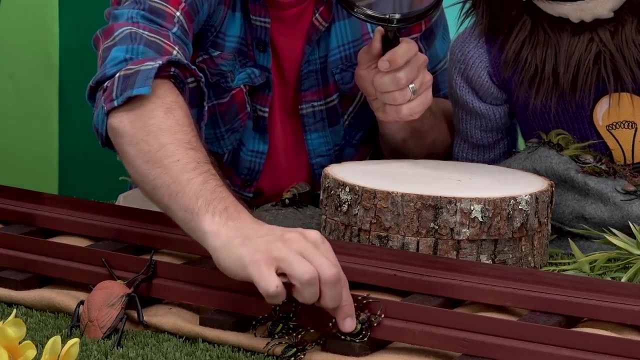 has enough energy to turn into a butterfly. That's right, Meta, A caterpillar transforms into a butterfly, Okay, Hmm, What other bugs can we find? Do you see a crawling spider right over there? Yeah, Here it is, Hmm. 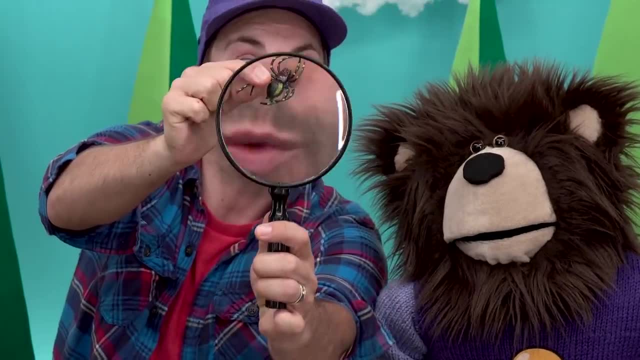 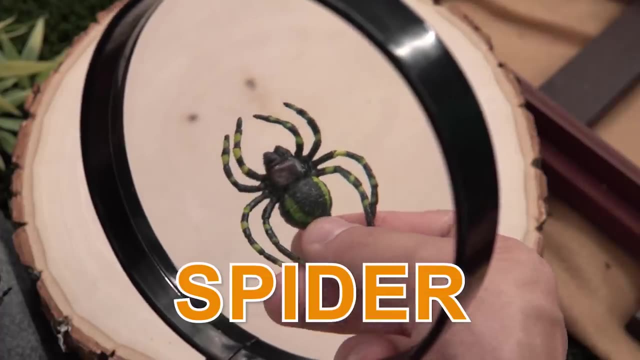 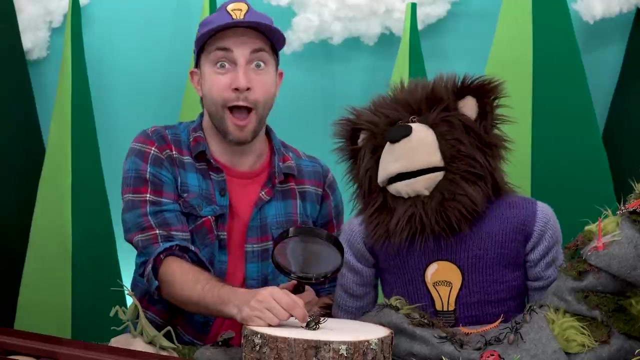 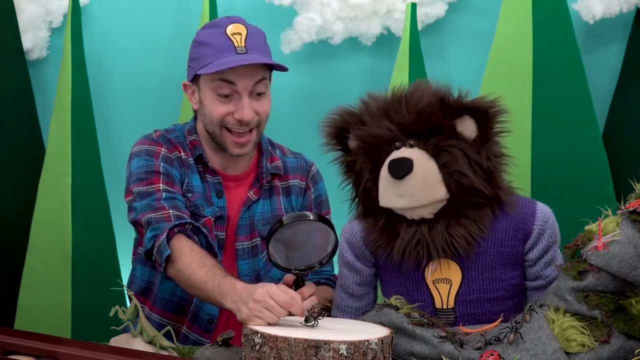 Hmm, Hmm. Spiders have eight legs. You know spiders, they keep to themselves and they make spider webs. Hmm, Have you seen a spider web? You have, Have you Meta? Yeah, So have I. All right, We'll put this. 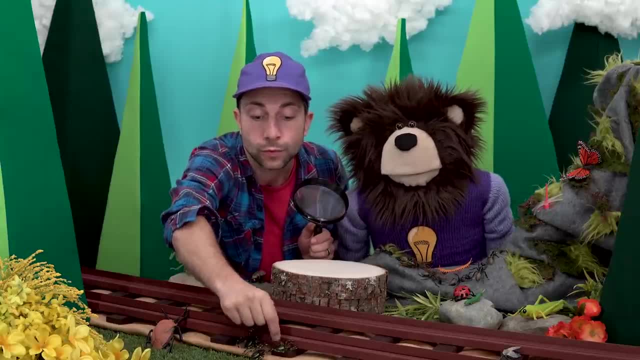 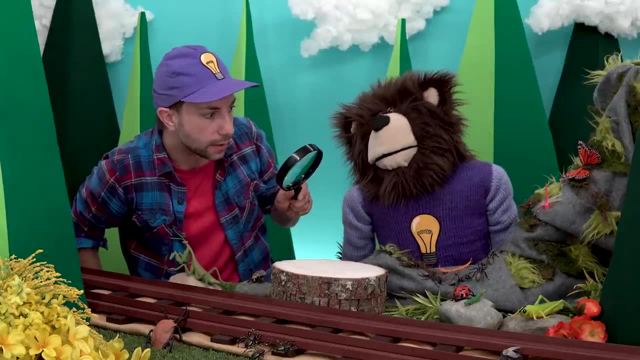 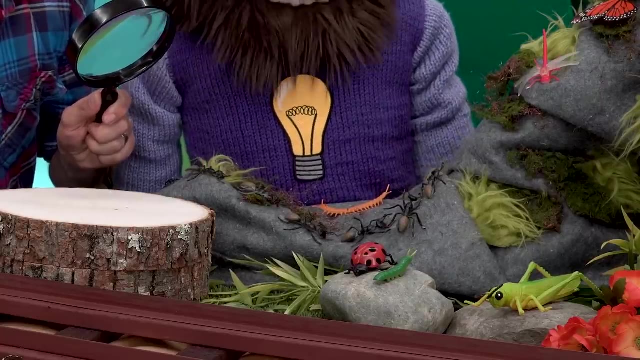 guy back. Hmm, Hmm, Okay, Let's continue to look. Oh, Meta, I see a line of marching ants. Do you see the ants? Hmm, That's right, Meta, they're right in front of you. Yes, Here I'll grab. 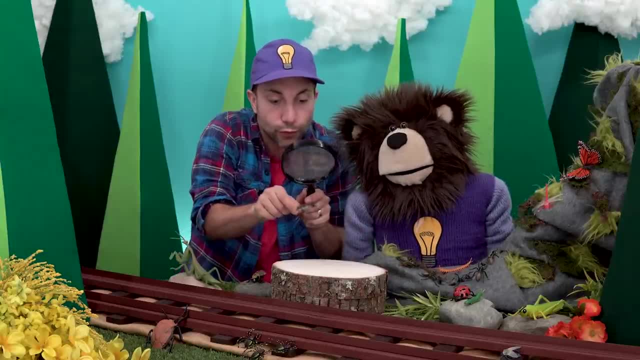 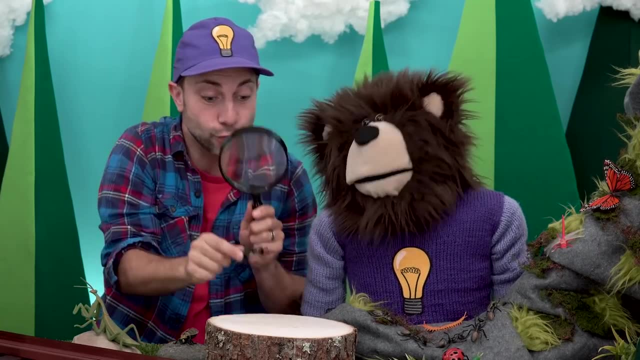 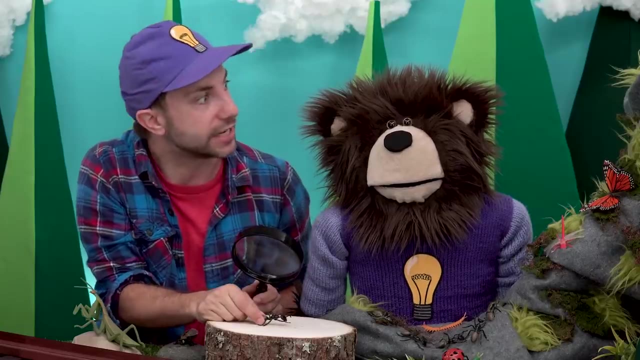 this guy right here? Whoa, Whoa. Oh, An ant is very, very strong. An ant can carry up to 10 to 50 times their body weight. Oh, that's a lot of weight, huh, And did you know? 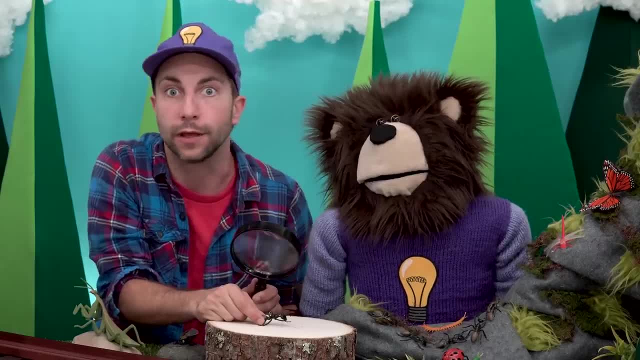 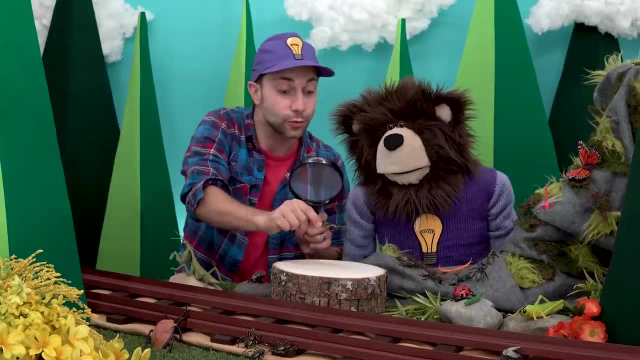 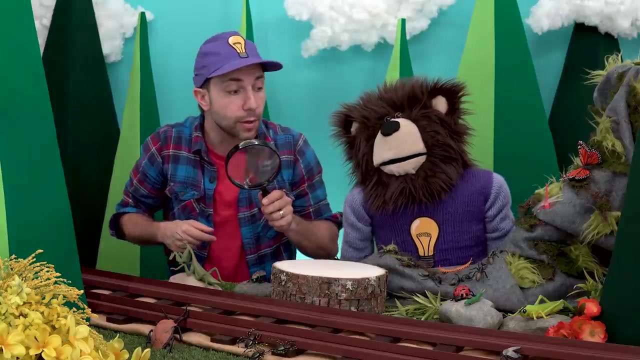 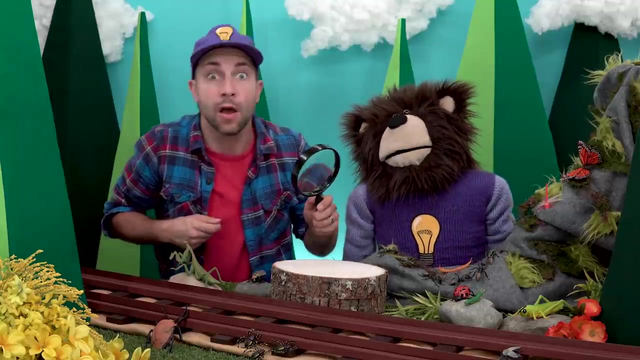 that an ant uses vibrations to feel around and to find food. Hmm, Oh Okay, Bye little ant. All right, Let's keep looking. Hmm, What are we going to Meta? There's a dragonfly right over there. 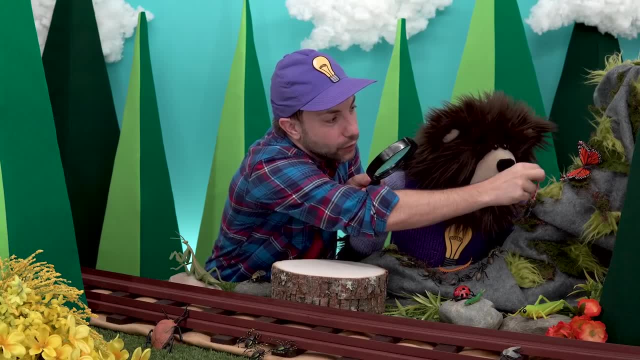 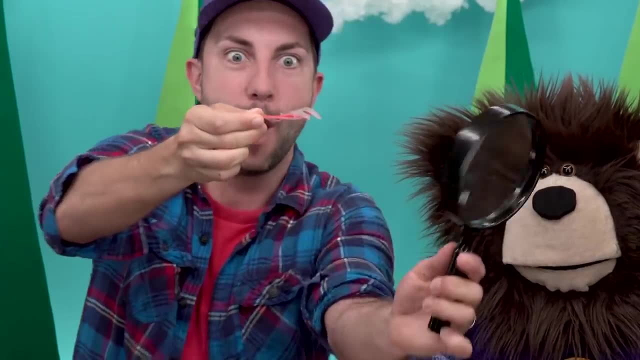 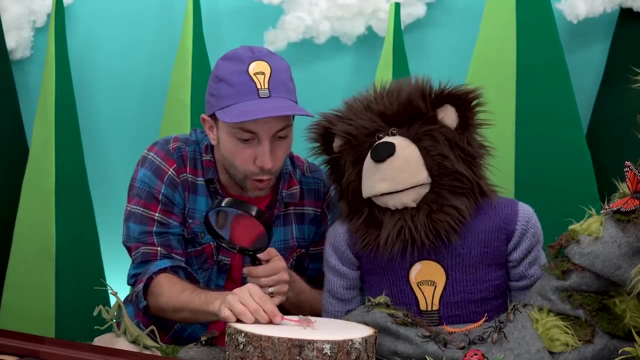 Whoa Here. Zzzz, Zzzz, Zzzz, Whoa. Take a look at that dragonfly. Zzzz, Zzzz, Dragonflies are really Here. Take a look again, Meta. Dragonflies are really. 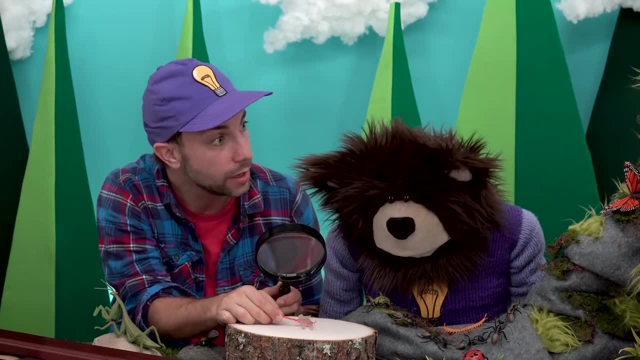 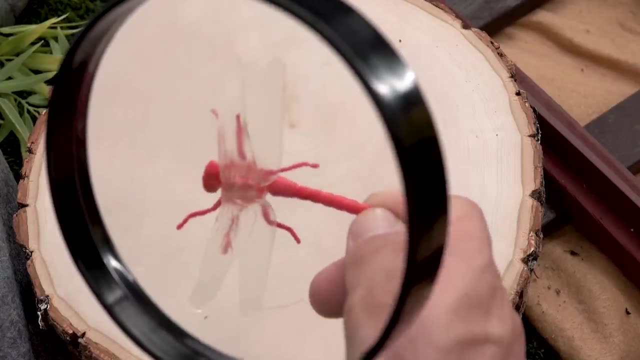 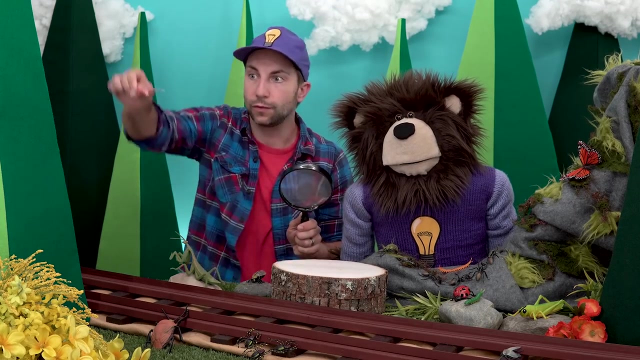 good flyers. They can fly up, They can fly down, They can even hover midair like a helicopter, And a dragonfly has a really big eye on their head so they can see really, really well. Zzzz, Zzzz, Zzzz. 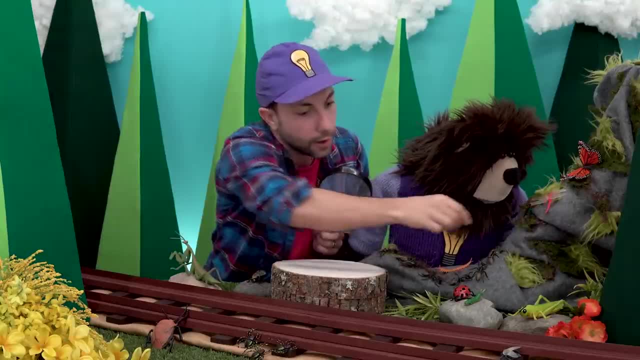 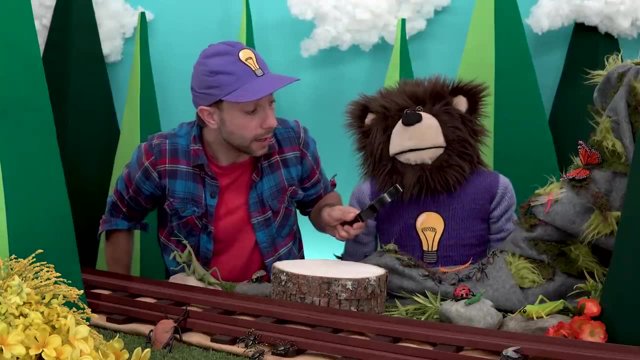 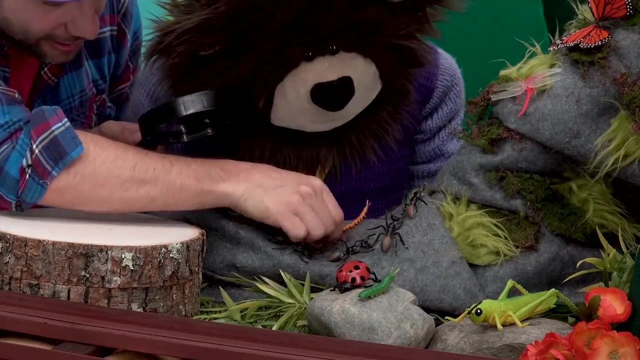 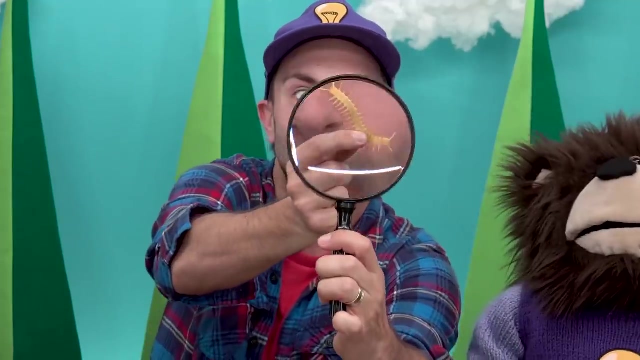 Zzzz. All right, What other bugs can we find with our magnifying glass? Meta, I see a orange centipede right in front of you. Whoa, It's right there. Zzzz, Whoa, Whoa. 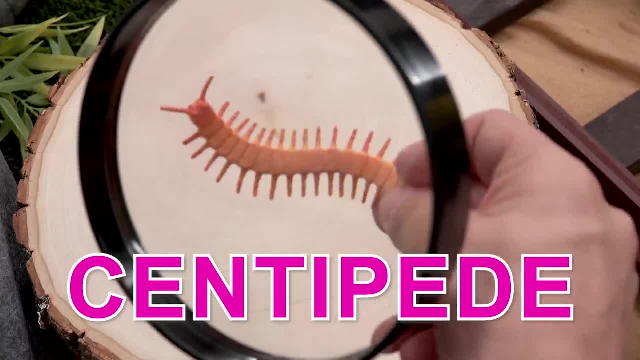 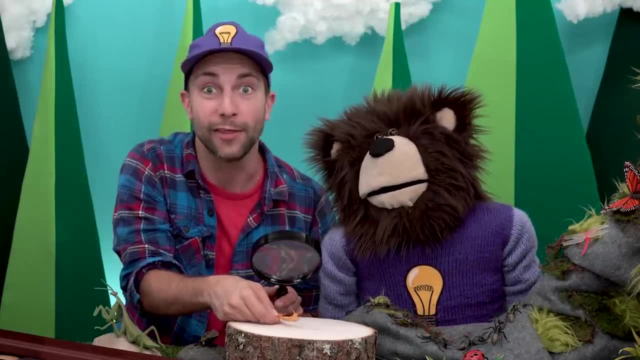 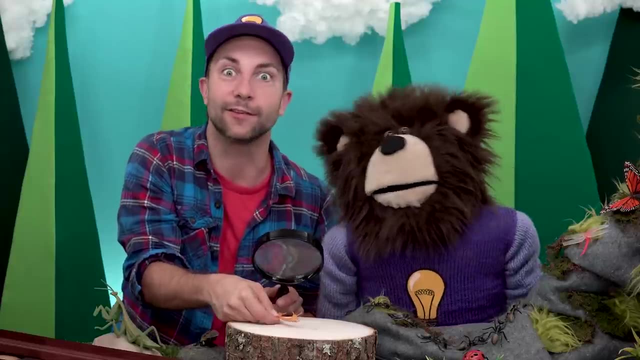 Centipedes have really long segmented bodies. Their bodies can sometimes range up to 12 inches long- Whoa, That's really really long. They have anywhere from 15 to 177 pairs of legs. Their legs are long and thin, so they can. 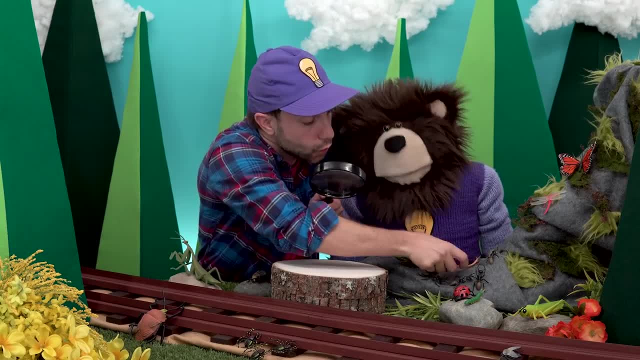 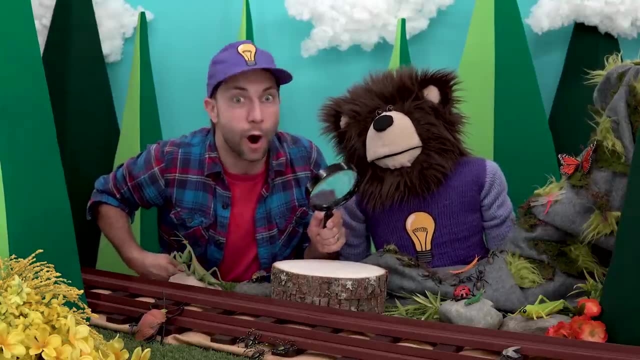 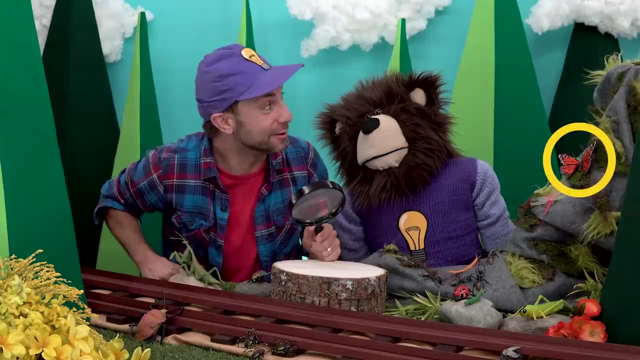 move really fast. Zzzz. All right, Let's continue to look for bugs. Zzzz, Zzzz. Do you see a butterfly? Zzzz, Zzzz. Meta, do you see a butterfly? Zzzz. 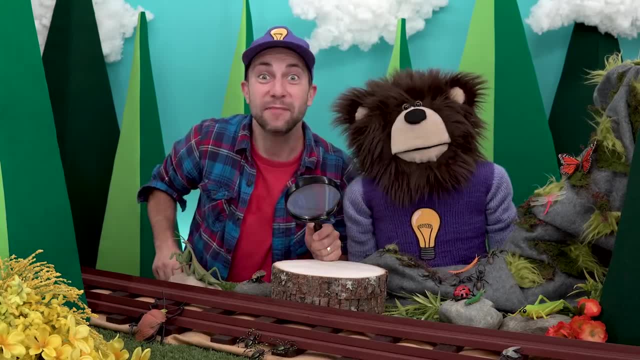 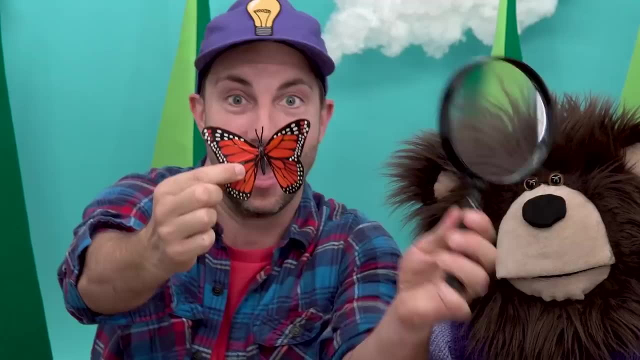 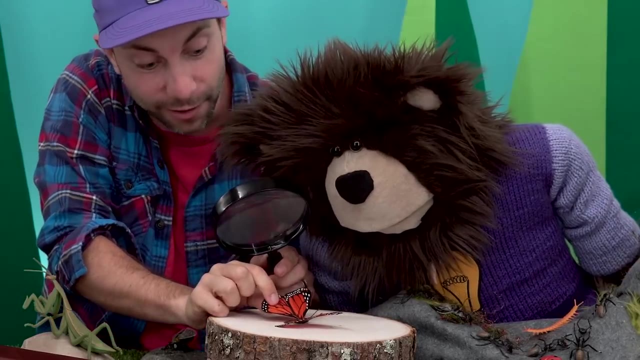 Zzzz, Zzzz, It's Mr Butterfly. Hi, Mr Butterfly, Whoa Zzzz, I like to look. Whoa, Mr Butterfly, how are you doing today? Good Yeah, All right. 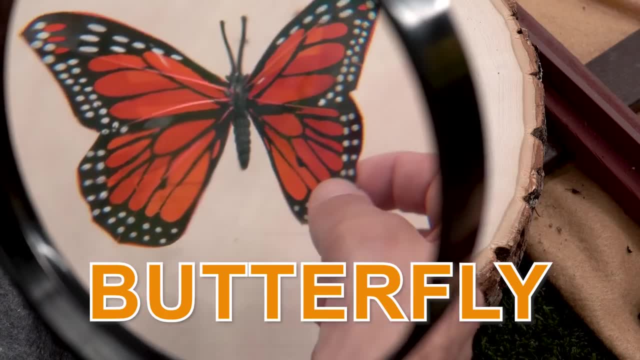 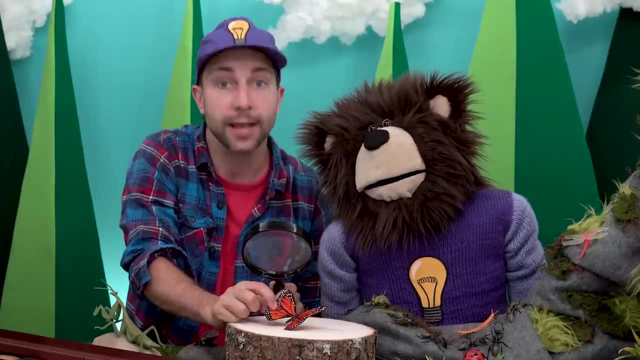 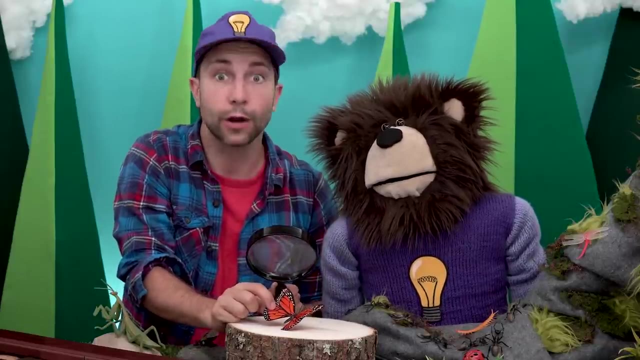 Did you know that butterflies taste with their feet? Isn't that silly? That's a fun fact. And, as we talked about before, a butterfly comes from a caterpillar. Did you also know, Meta, that a butterfly's wings are clear? 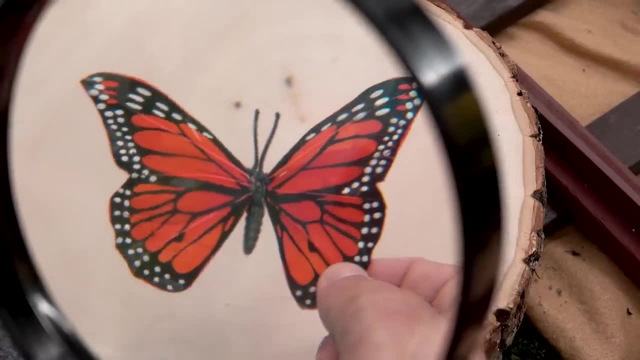 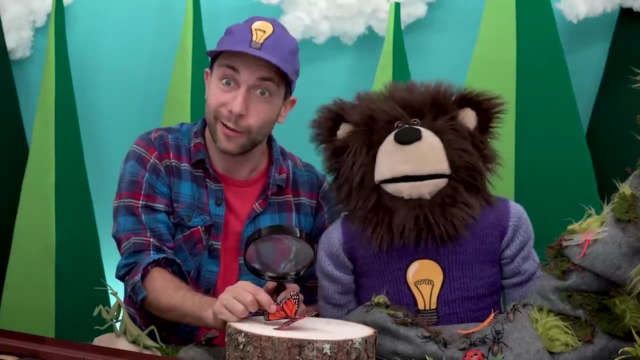 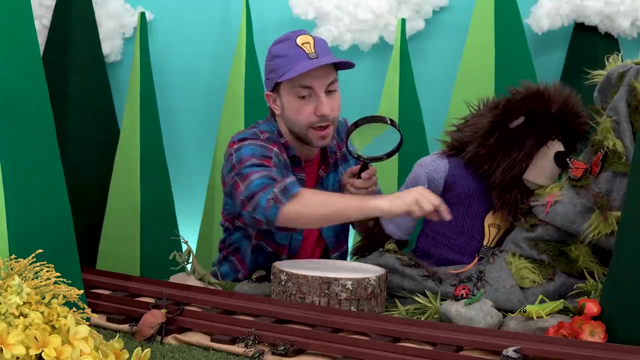 Zzzz, That's right. They have little tiny scales on their wings that reflect light. So all the colors and shapes that we see are actually reflections of light. Oh, that is very interesting. Okay, Let's put the butterfly right back there. 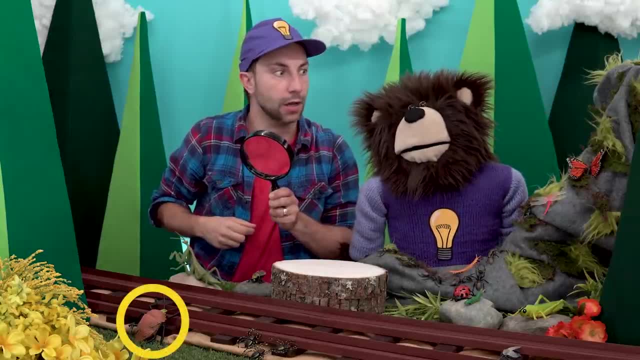 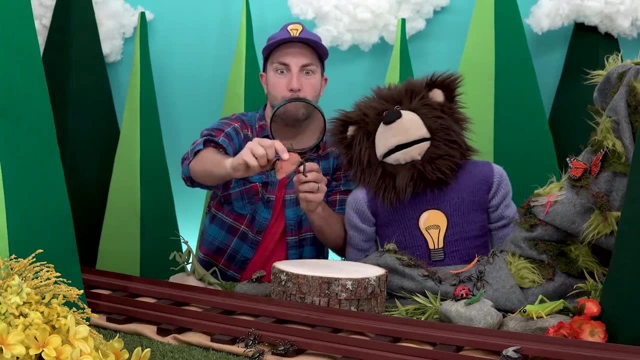 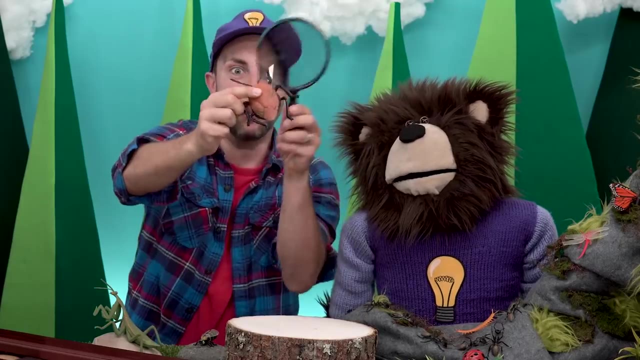 And Meta. I see a beetle. Look at this big beetle. Ba-boom, Ba-boom, Ba-boom, Ba-boom, Ba-boom, Ba-boom Here, Whoa Ba-boom, Ba-boom, Ba-boom. 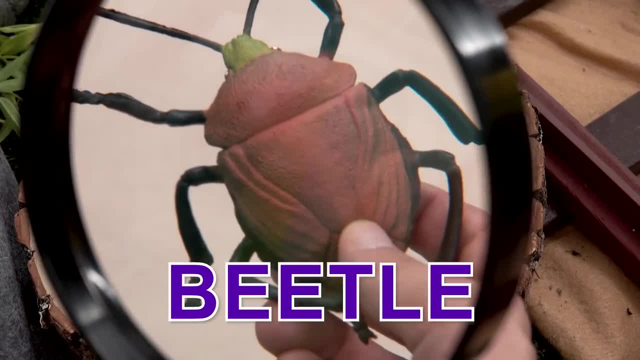 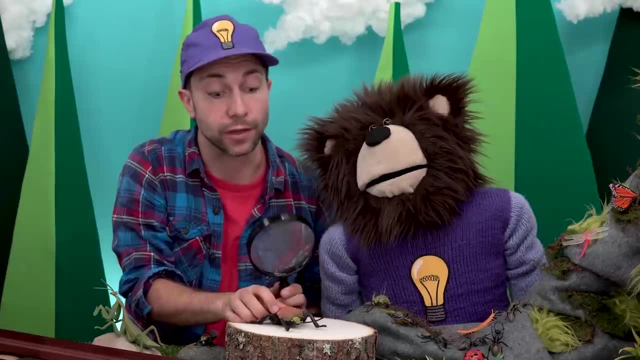 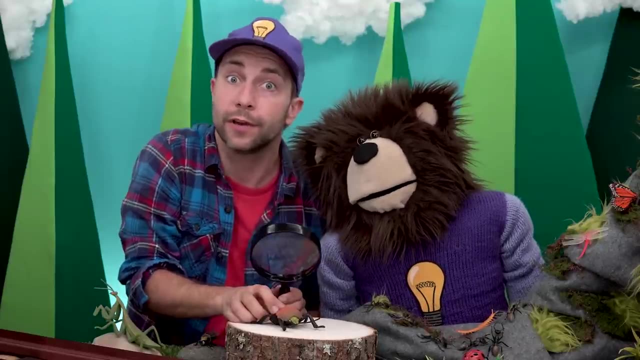 Ba-boom Beetles usually have two wings and they can't see very well, So they use a sense of smell and vibrations like ants to find food and feel their way around. Isn't that interesting? Mm-hmm, All right. 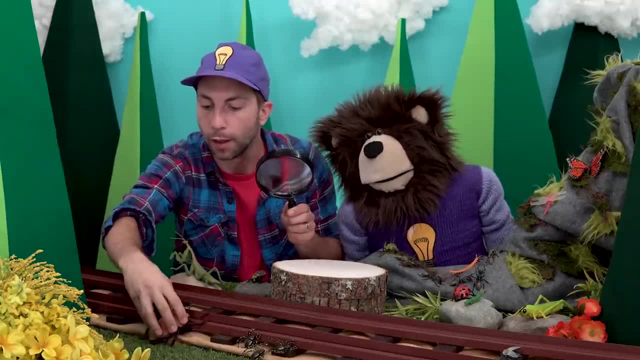 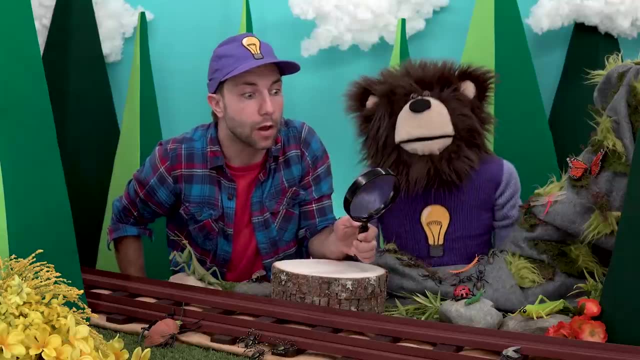 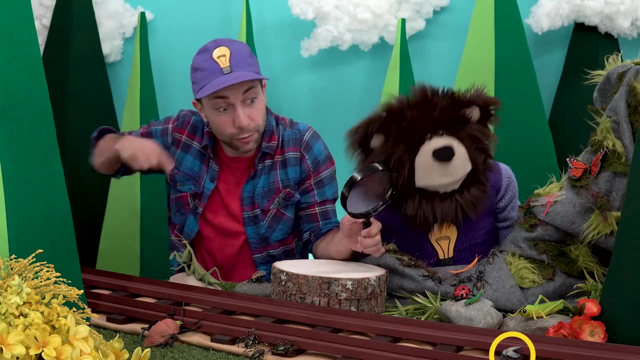 Ba-boom, Ba-boom, Ba-boom, Ba-boom, Ba-boom. There you go, little beetle. All right, Let's continue to look for more bugs. Do you see a housefly? Do you Meta? That's right. 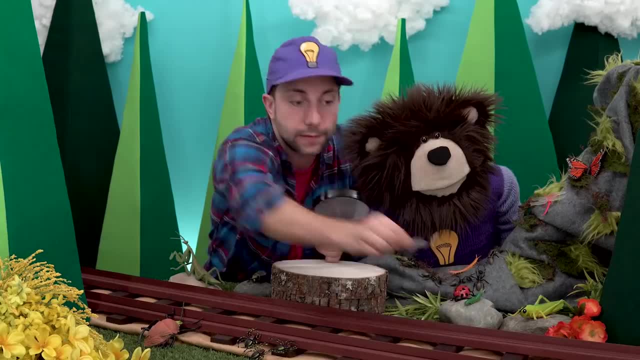 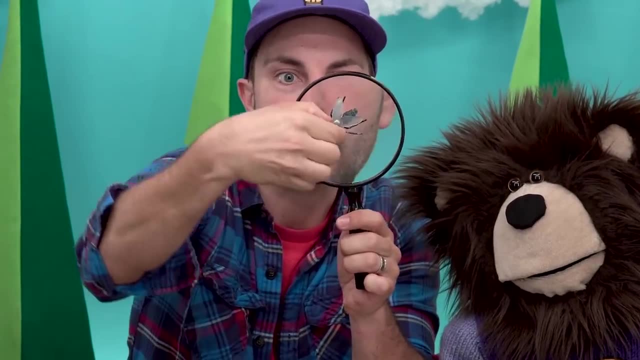 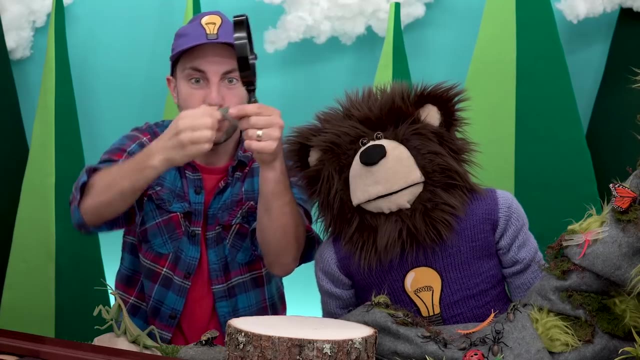 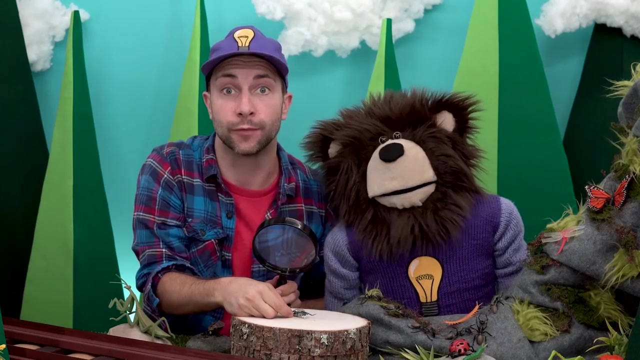 The housefly is over here on the train track. Whoa, Look at that housefly. Whoa, Here you go. Houseflies are really good flyers. A housefly can see in front of them. It can see the sides of them. 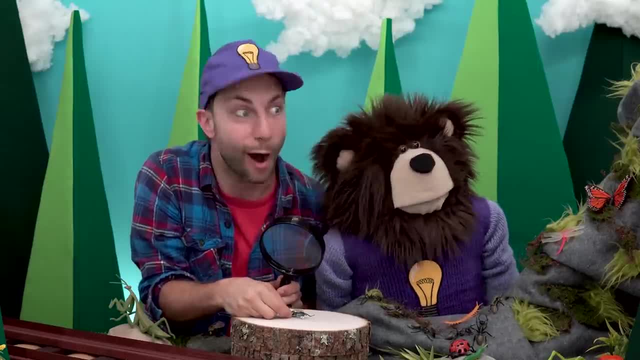 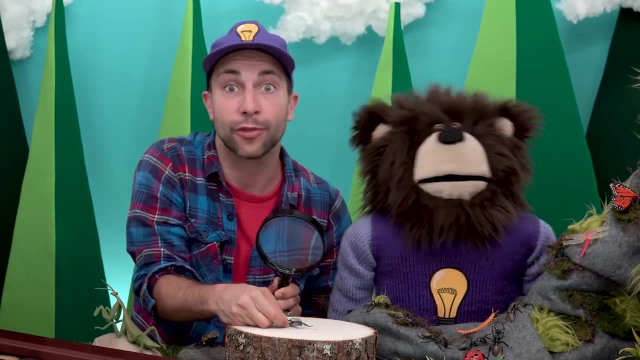 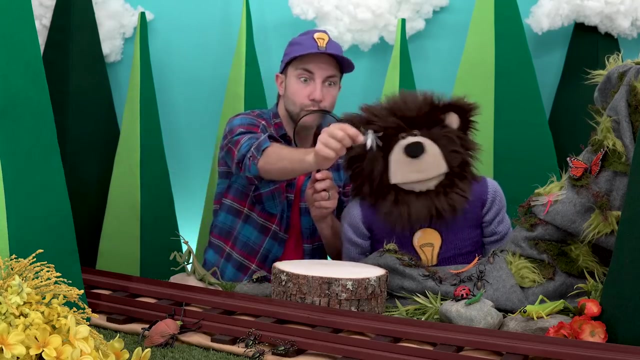 And they can see in back of them. That's right. A housefly can see all the way around. They have a 360 degree view of vision. Wow, That's pretty neat. Zzz, Zzz, Zzz. All right, Let's continue. 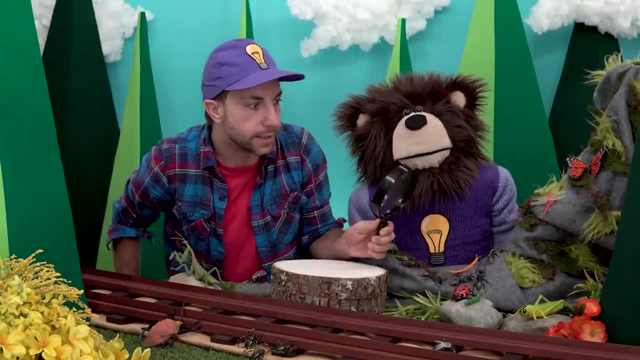 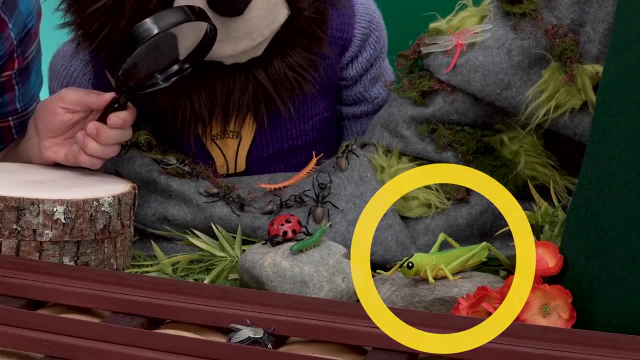 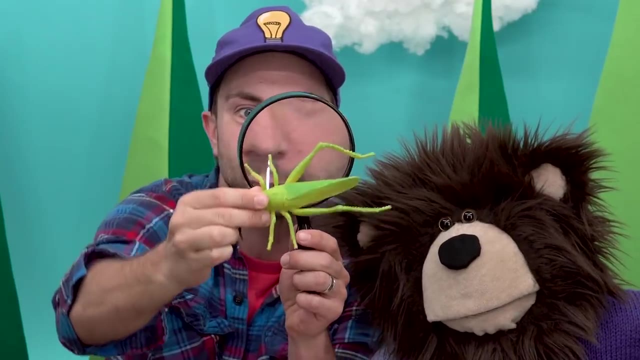 to look for our bugs. Meta, there's a grasshopper in front of you on the rock over there. Oh, A-boing, A-boing, A-boing, Whoa. Look at this grasshopper, Would you look? 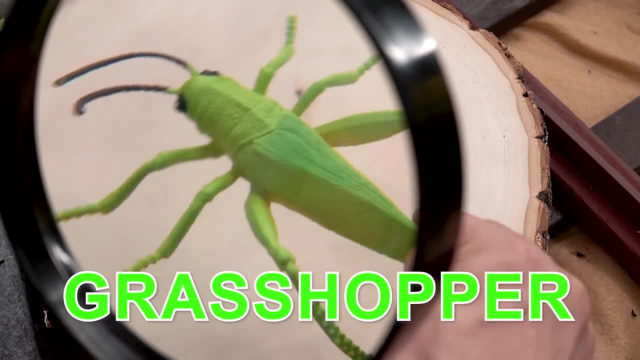 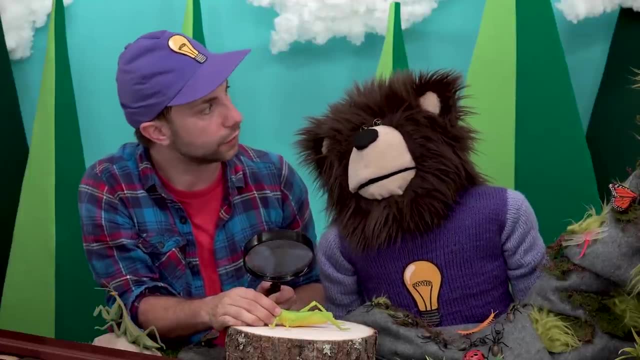 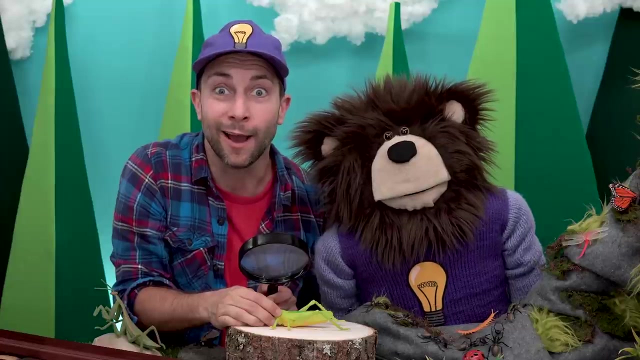 Whoa A grasshopper is a really good flyer and a really good jumper. They also make some interesting noises too, by rubbing their hind leg against their forewing. Have you heard a grasshopper at night? You have Meta. have you heard? 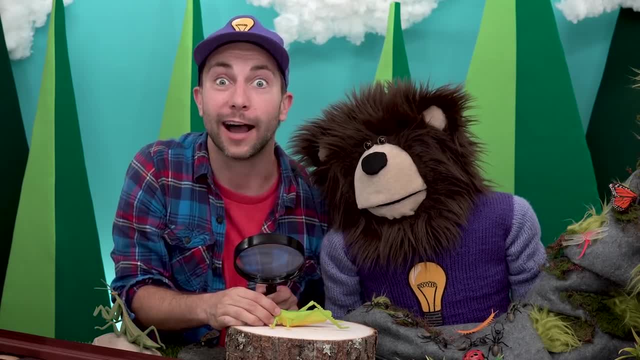 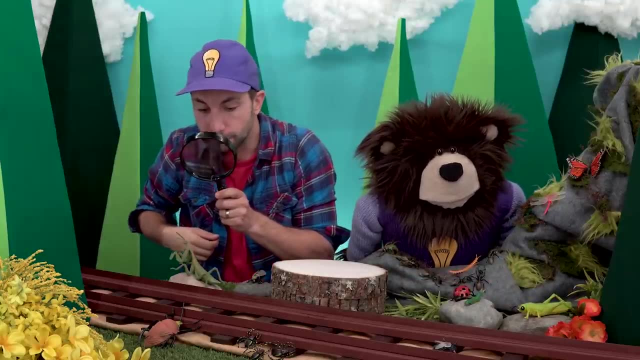 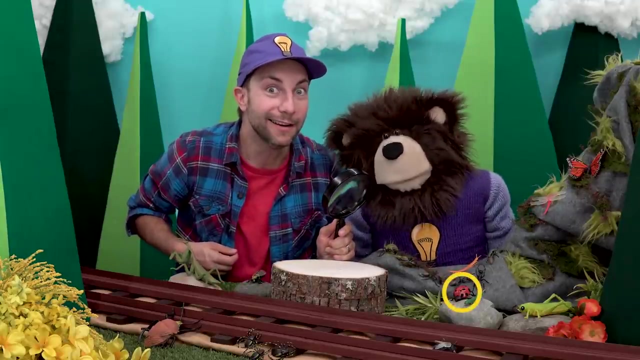 a grasshopper at night. Yeah Well, so have I. Boing Boing, Boing, Boing. Okay, Let's continue to search for some bugs. Do you see a ladybug? That's right, Right in front of Meta. 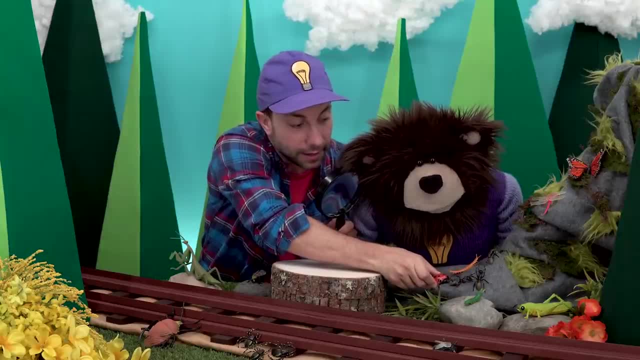 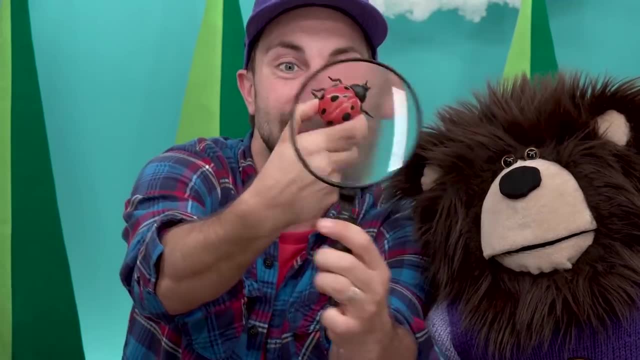 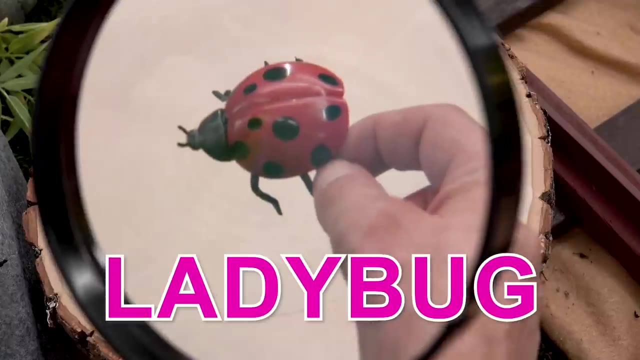 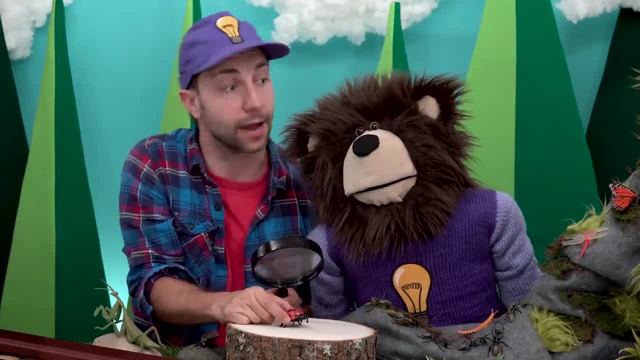 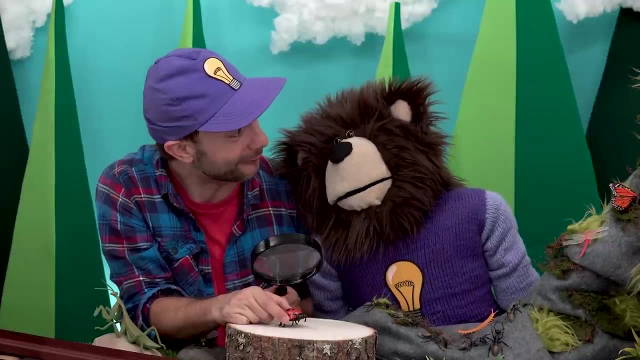 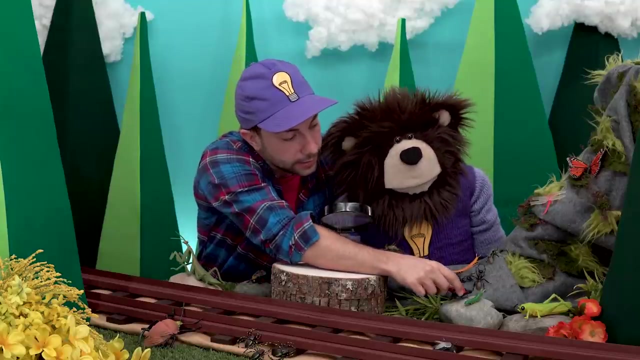 just like this one with red and black colors. But did you know that a ladybug can come in all colors of the rainbow? Wow, That is pretty, pretty neat. All right, Let's put this little ladybug back. Let's keep looking Meta. 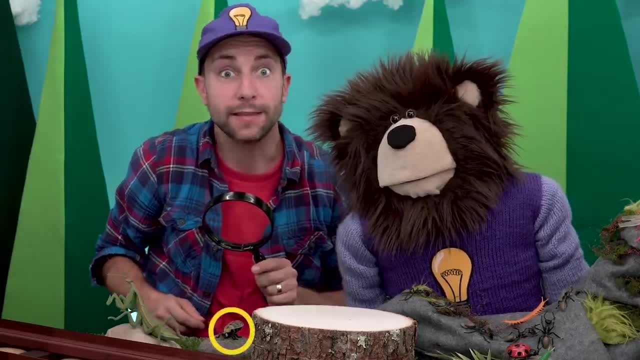 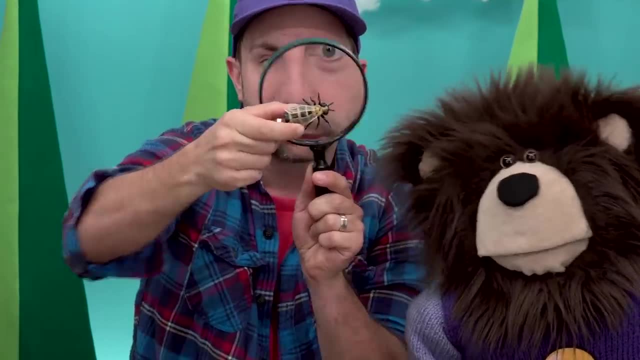 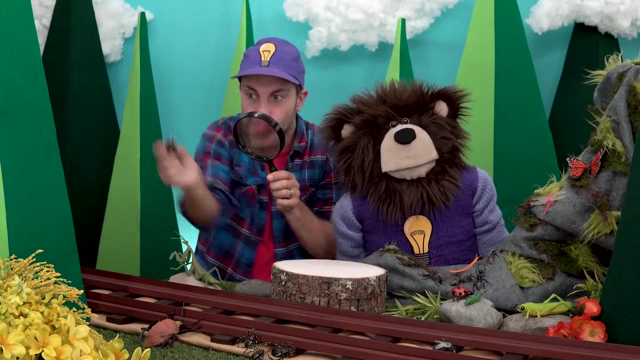 Whoa Meta. Right in front of me is a honeybee- Buzz, Buzz, Buzz, Buzz, Buzz, Buzz, Buzz, Whoa Whoa. Look at that honeybee Meta. Buzz, Buzz, Buzz Honeybees. 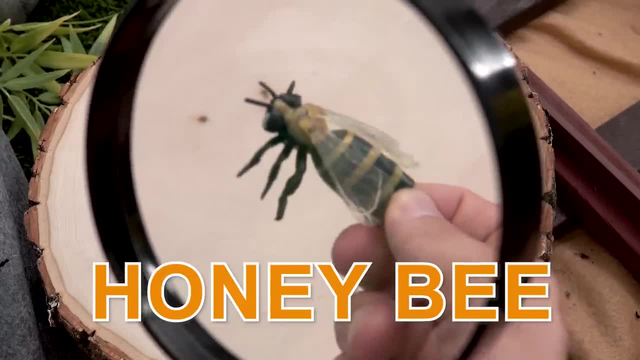 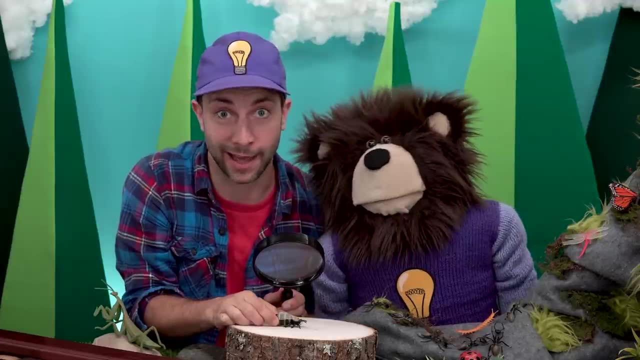 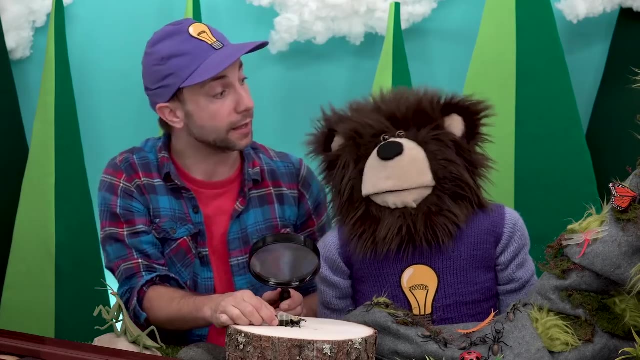 are really important because they help other plants grow by pollinating fruits and vegetables and flowers, And they make honey. That's right, Honeybees make honey. They live in hives, or you can call them colonies, And honeybees are really. 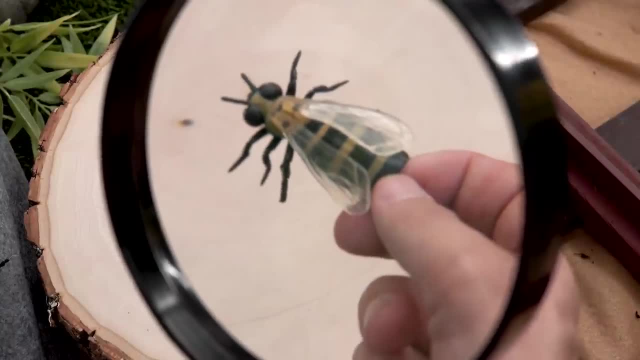 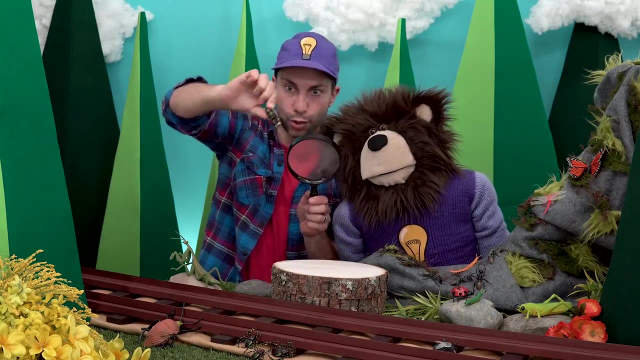 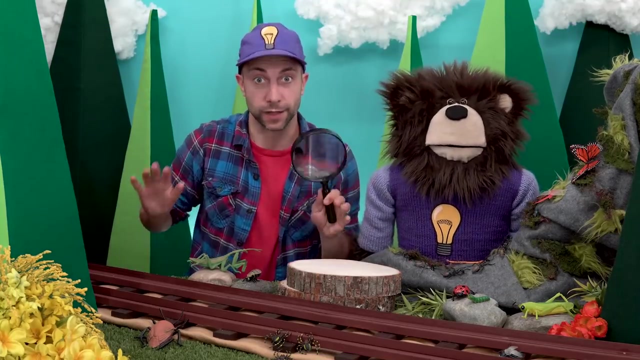 good flyers. They can flap their wings up to 200 times a second. Wow, That is a lot of flaps. Buzz, Buzz, Buzz, Buzz. You know what time it is? It's time to dance. This is where we stop. 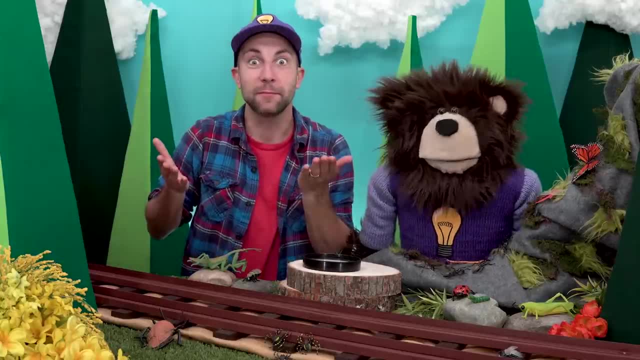 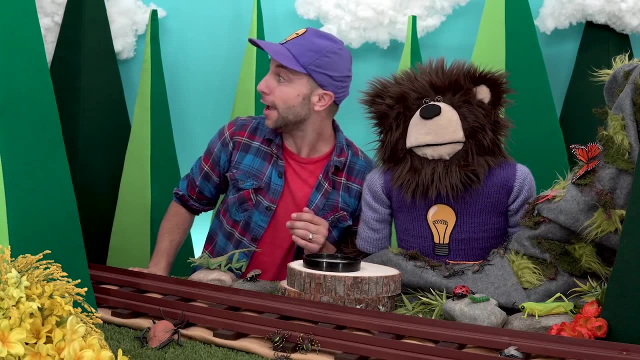 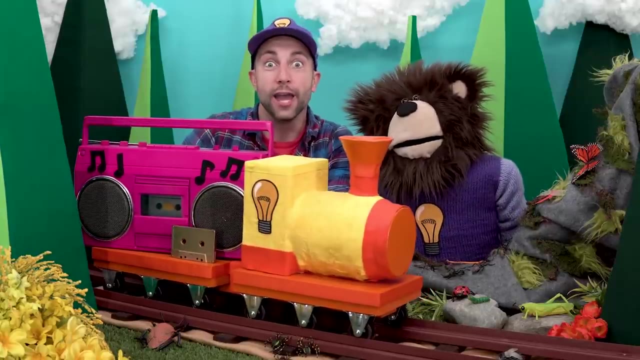 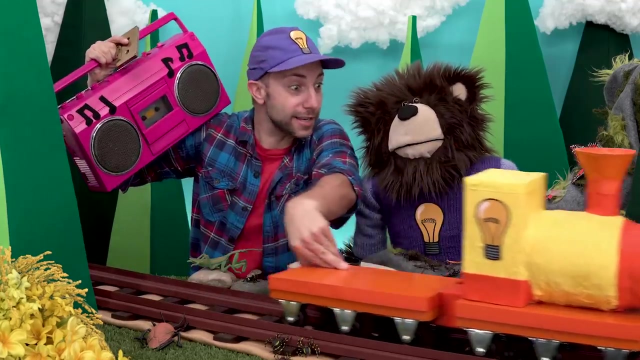 what we're doing. stand up and dance. You can do whatever dance move you feel like doing. It's the Idea Train. It's Pinky the Boombox. Hi, Pinky the Boombox. All right, Thank you, Idea Train. 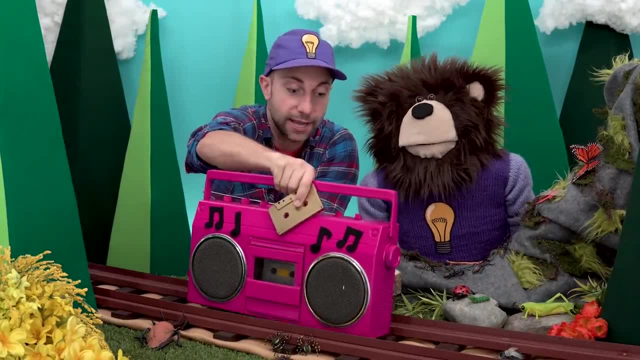 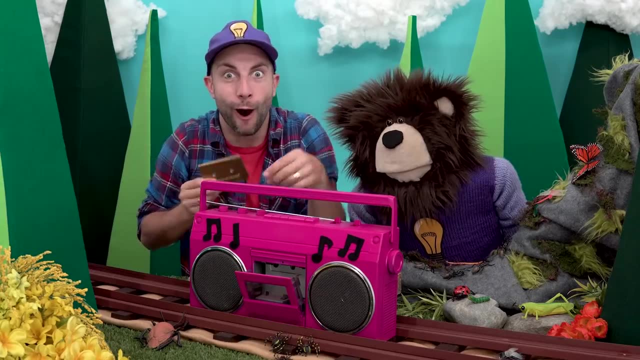 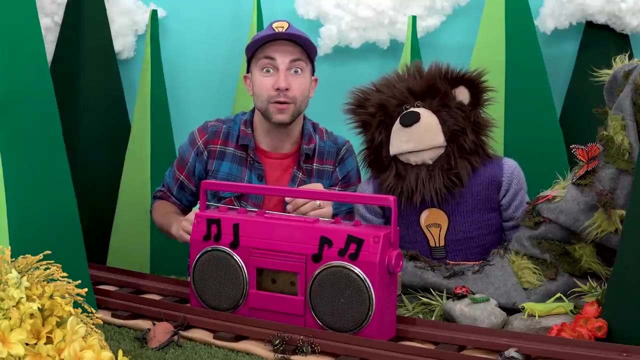 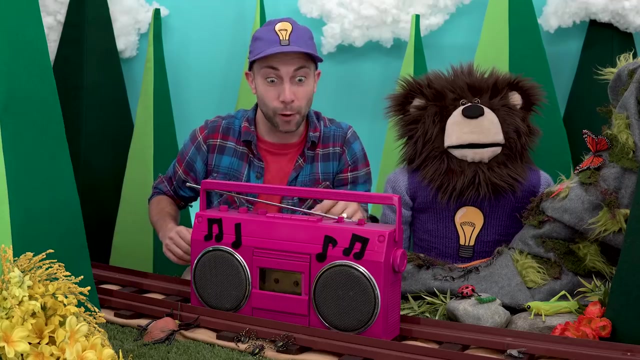 Pinky, the Boombox plays our music. We take this golden cassette tape and put it in here and close it, And we push the button with the triangle on it, the play button. Are you ready to dance? Yes, I'm going to push the button. 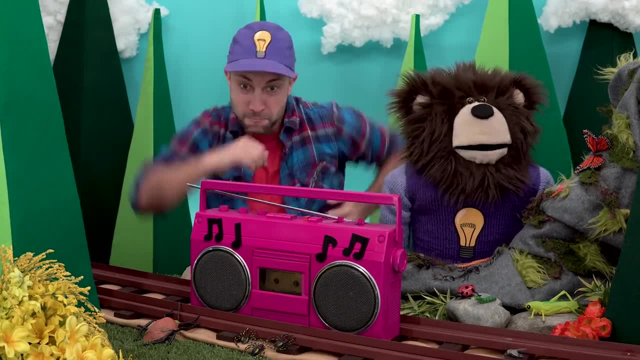 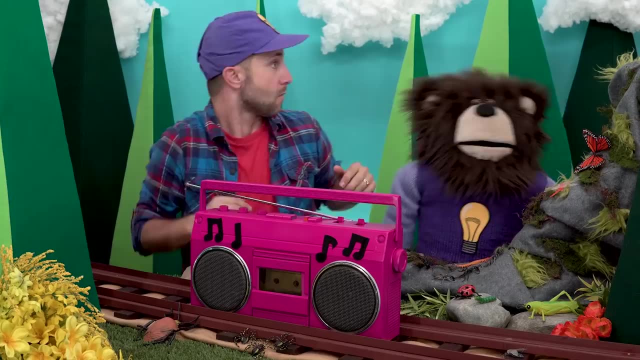 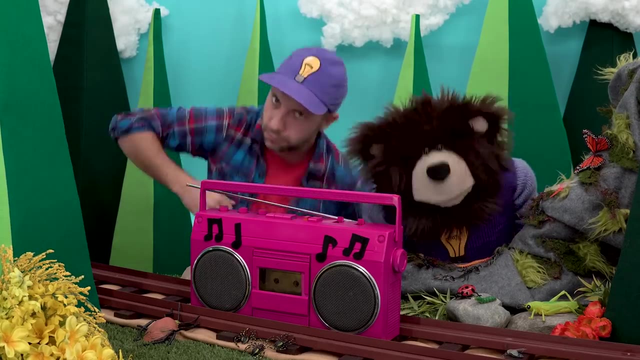 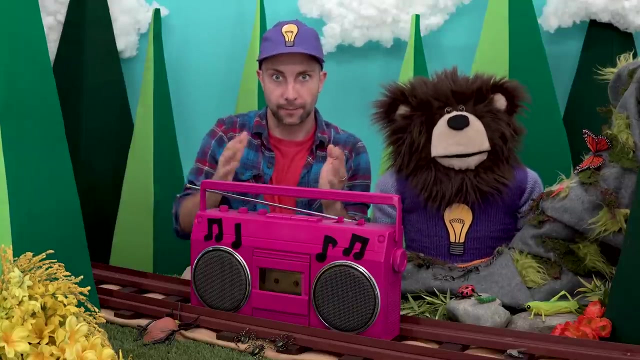 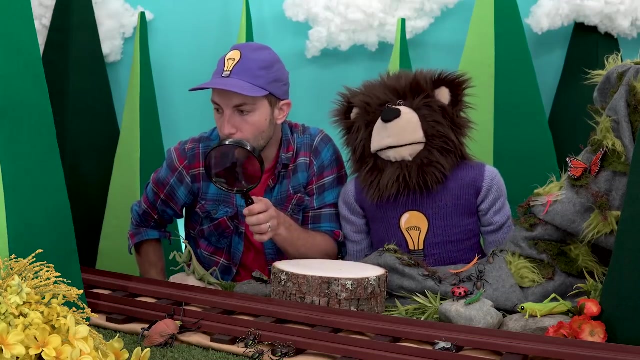 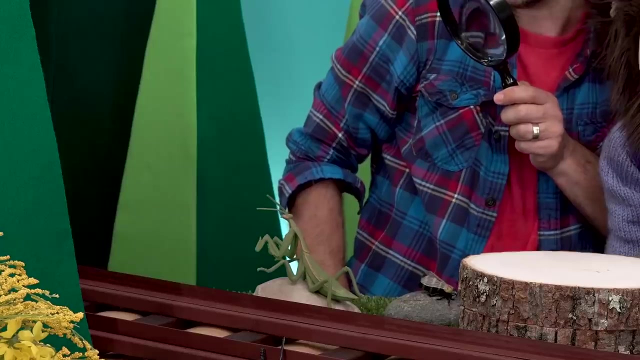 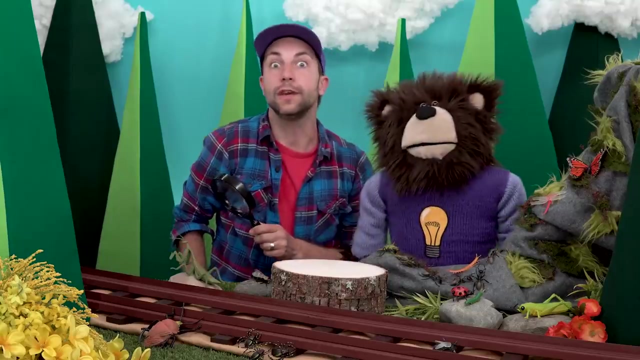 now. Whoa, That was a lot of fun. Okay, Let's get back to what we were doing. Okay, Let's keep looking for more bugs. Mayta, I see a praying mantis right over there on that rock. Do you see that? 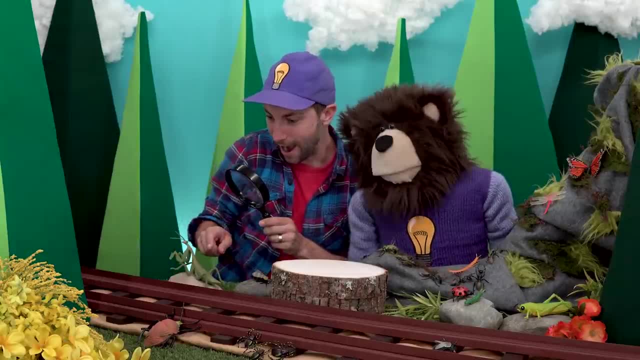 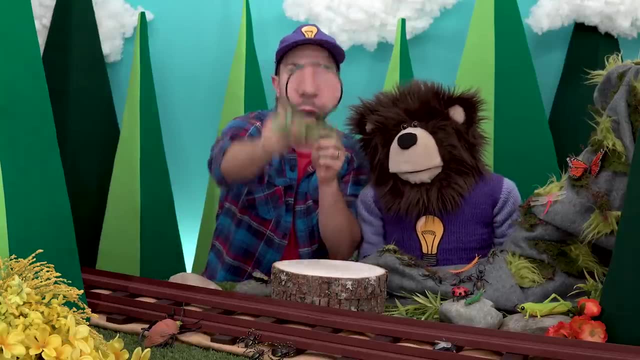 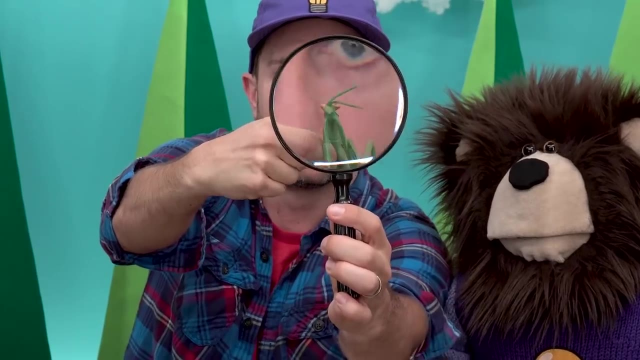 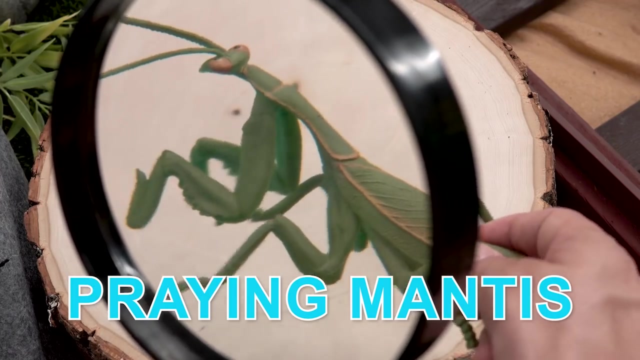 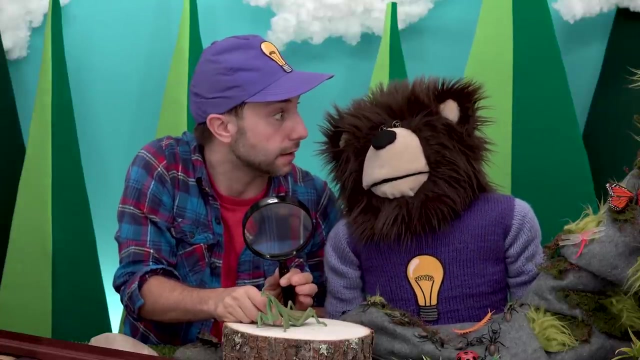 praying mantis. Wow, Look at this guy Boing, Boing, Boing, Whoa. Take a look at that, Whoa. A praying mantis is very agile. It can jump from one limb to another limb of a tree and it can bounce. 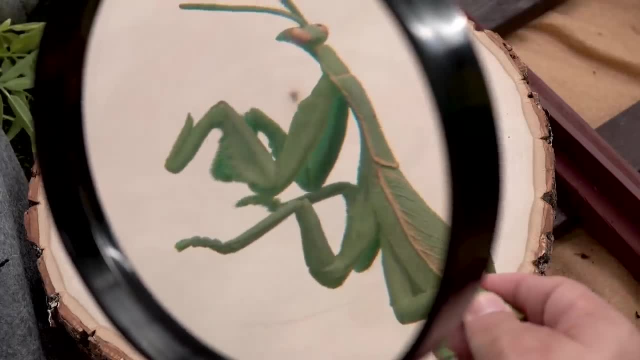 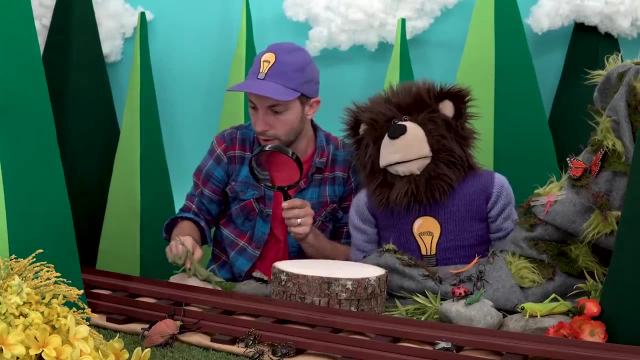 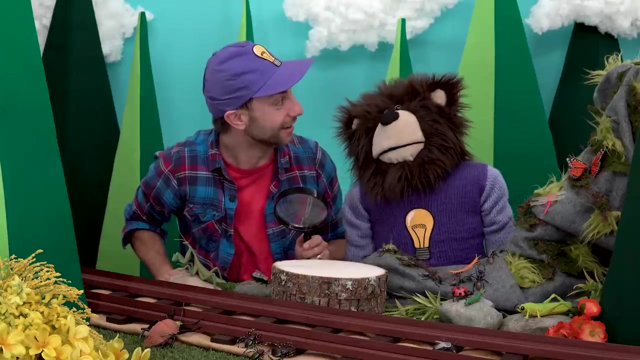 Kind of like a kitty cat And some people think a praying mantis is very, very smart. Hmm, Boing, Boing, Boing. Wow, We sure did find a lot of bugs, didn't we? Mayta, Did you have fun looking for all those bugs? 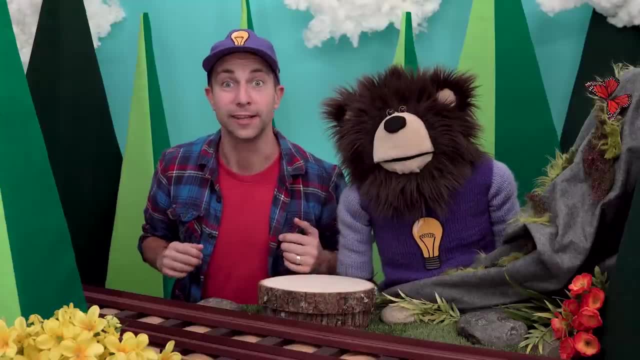 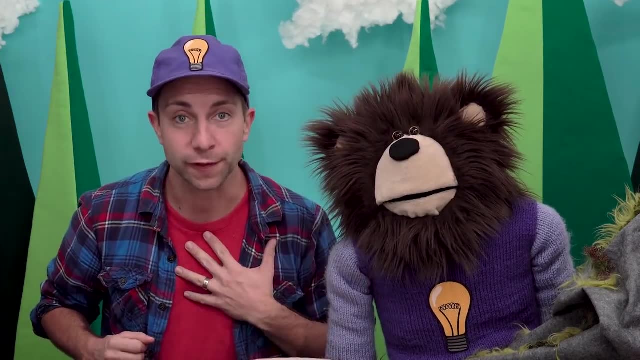 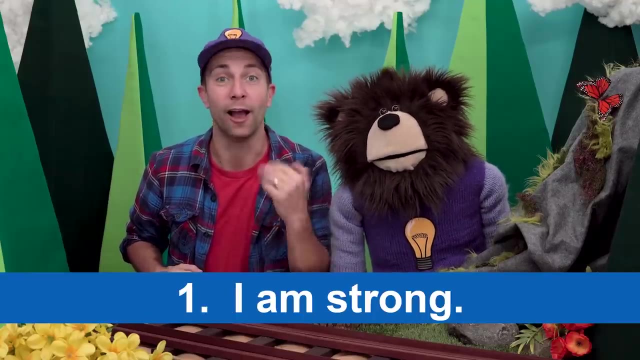 You did. Before we go, let's say five good things about ourselves. Do you want to do that? I'll go first and then you repeat what I say after me. Number one: I am strong. Number two: I am helpful. 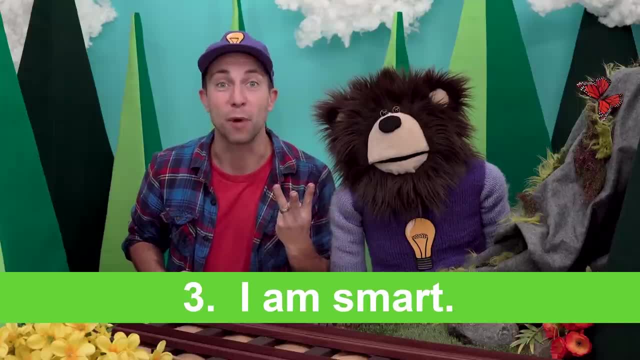 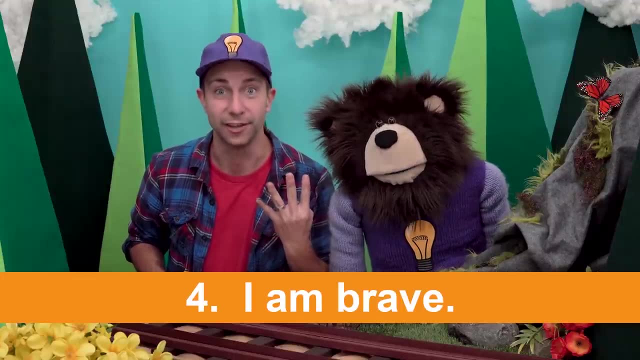 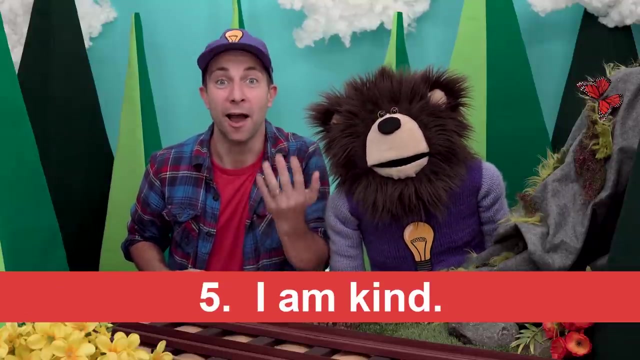 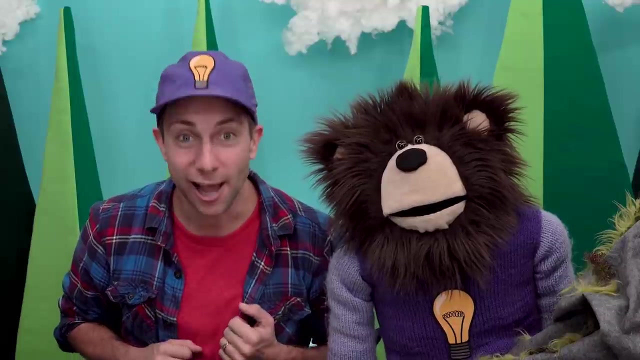 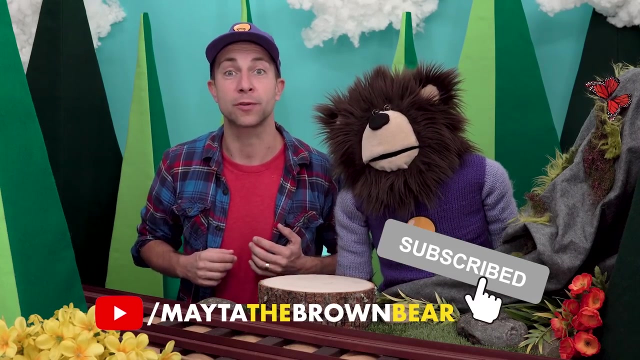 Number three: I am smart. Number four: I am brave. Number five: I am kind. That was great. Wonderful job, Grownups. remember to follow us so you know when we post a new video, And please support our channel by subscribing.